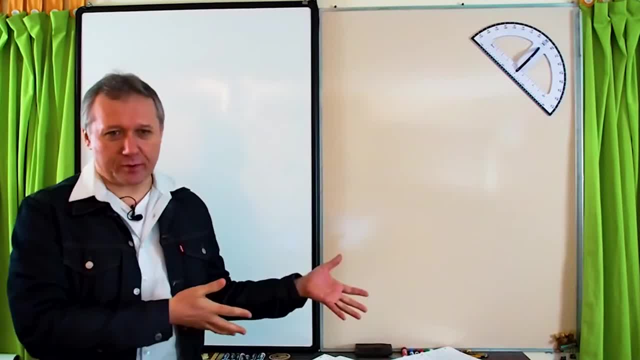 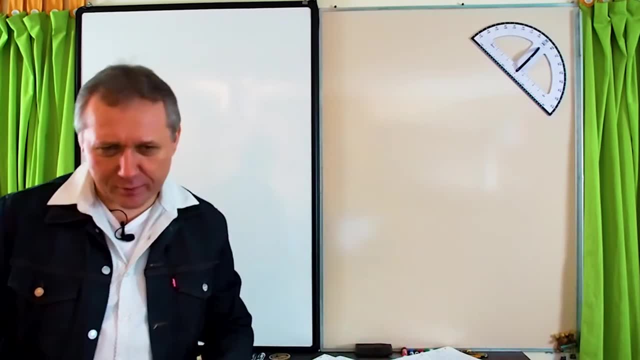 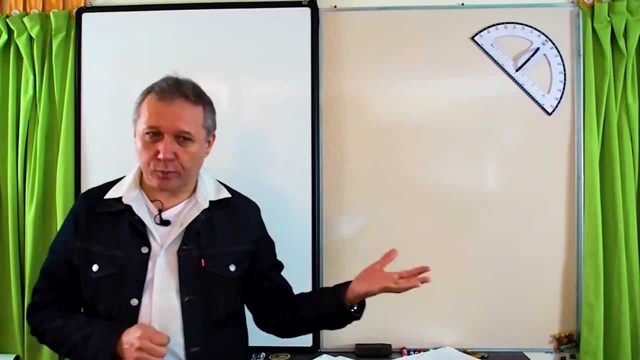 So we will derive here the major formula right, And then we will just grab it and use it in the Lagrangian formalism right, With small adjustments right, Not that significant right. So I'm sure that at some point you'll learn calculus of variations. 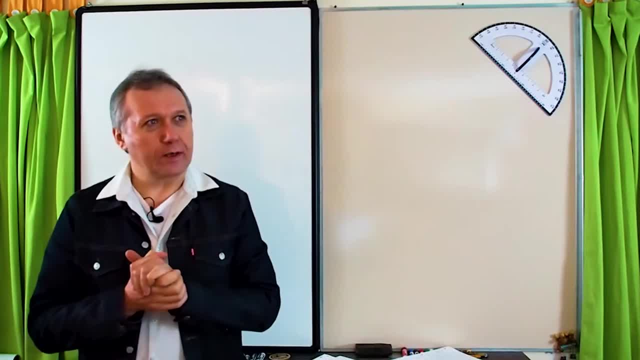 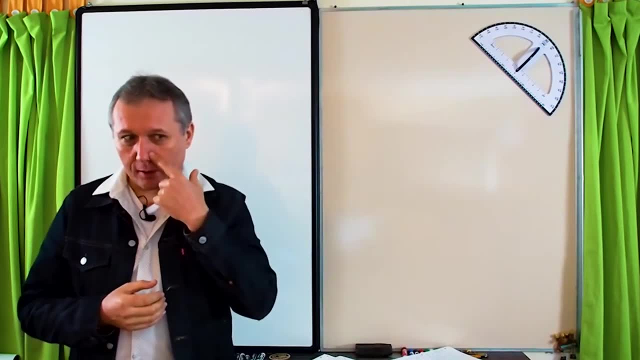 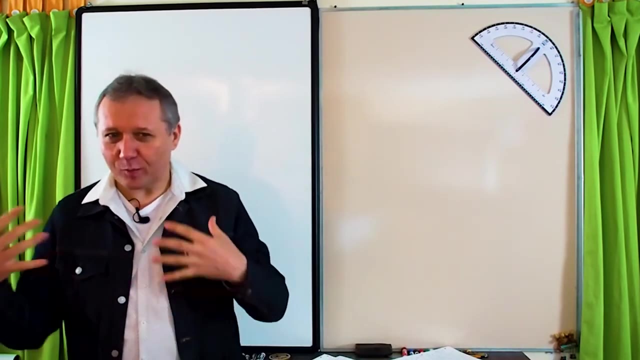 in your, one of your, maybe- calculus classes- Actually, I need to find out where right, But I remember myself it was the second year right the university And we were quite fascinated by this completely different approach right, Really different from normal calculus right. 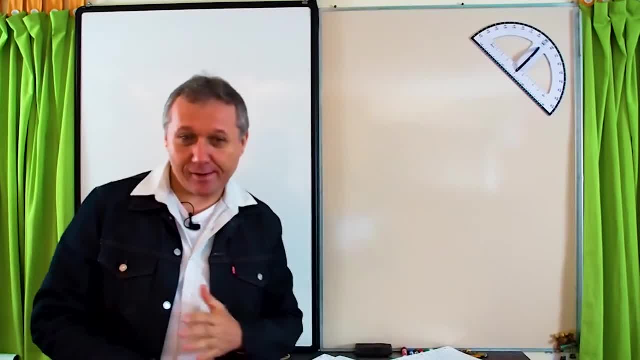 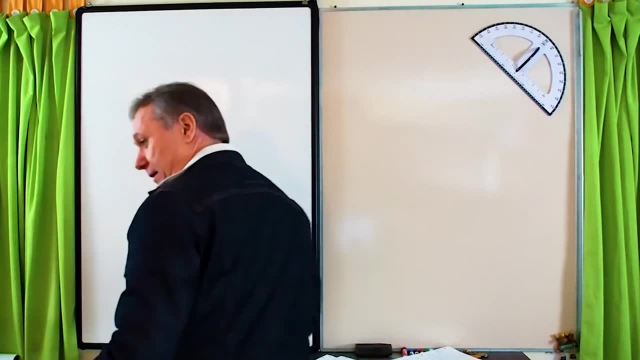 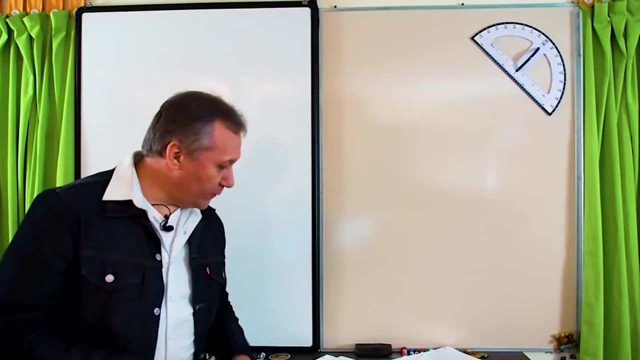 It was so new, It was so, you know, refreshing, even right. I remember we were impressed by this, But anyway, right. so let's, I'll write the title: calculus of variations. and before before, before I write down the goal of calculus of variations and so on. 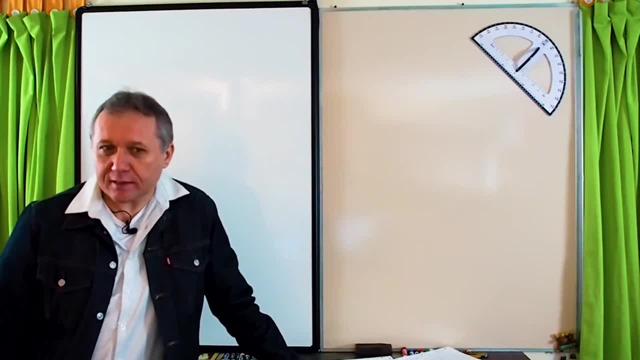 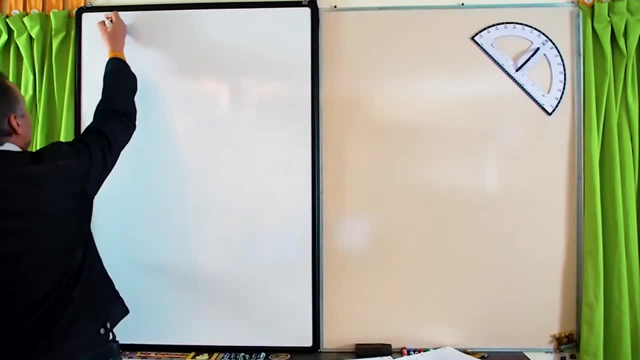 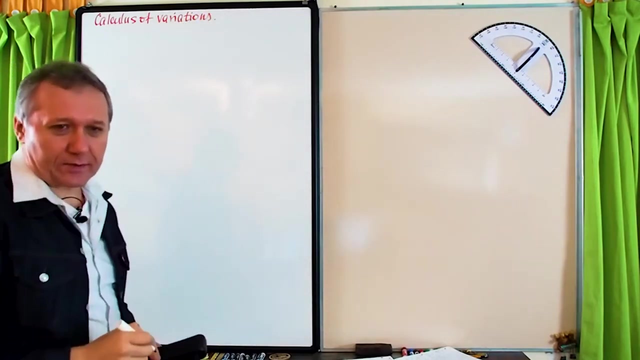 let's look at a couple of examples in order to actually see the goal right, On sort of on real examples. But first, of course, let me write down the title. So calculus of variations. It's chapter six. probably I should write it down also: chapter six, right? 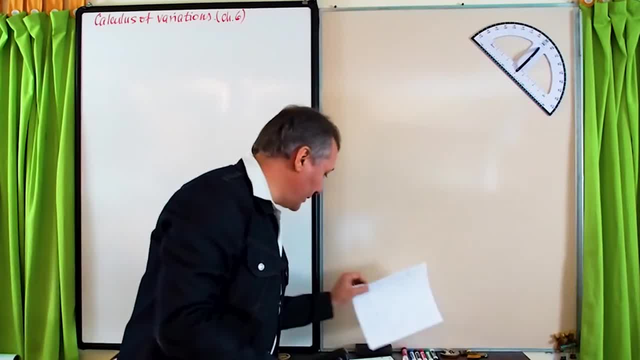 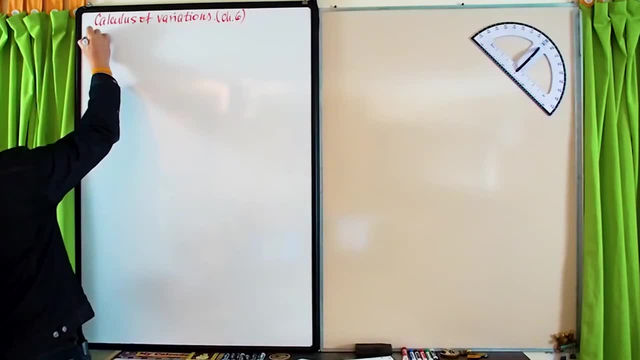 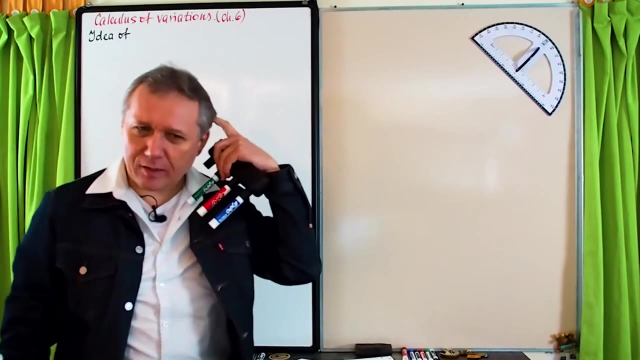 And all right, so let me. all right so, idea of calculus of variations. All right, so let me write idea of you know what calculus of variations. since I'm I'm going to use it from time to time. let me abbreviate it. 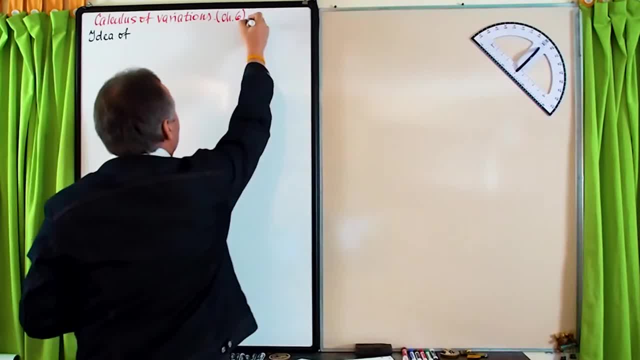 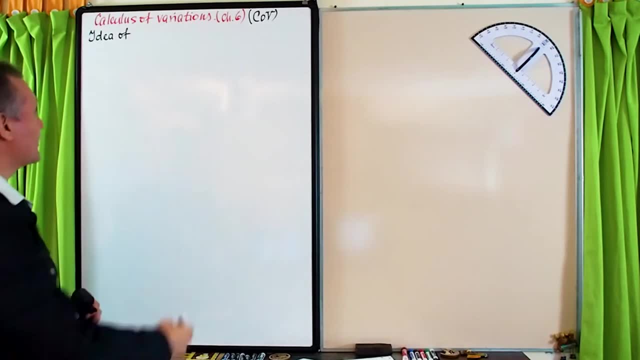 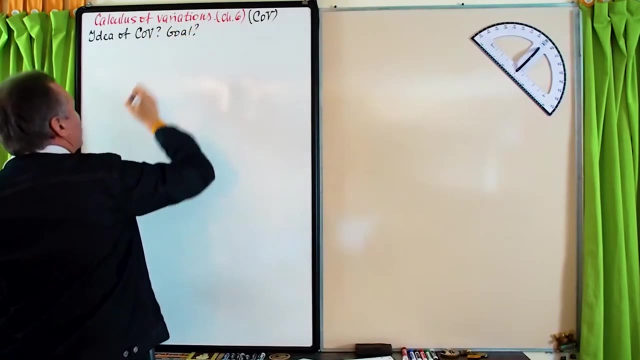 Okay, It's not universal abbreviation, but COV- calculus of variations. So idea of calculus of variations, right? So basically like a goal, What's the goal of COV? And let's look at a couple of examples. as I said, 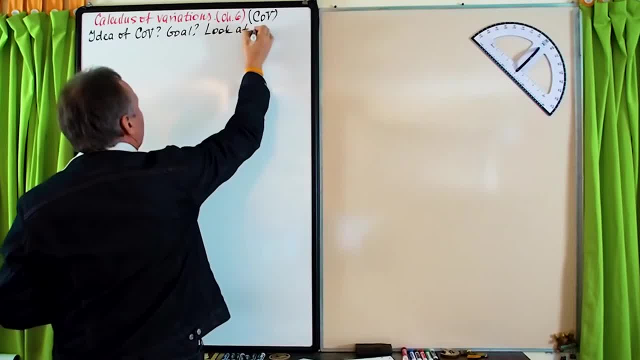 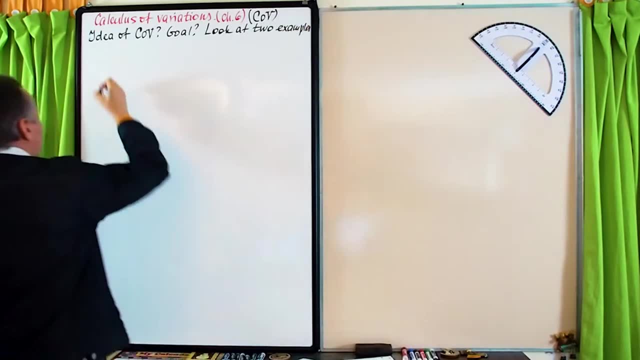 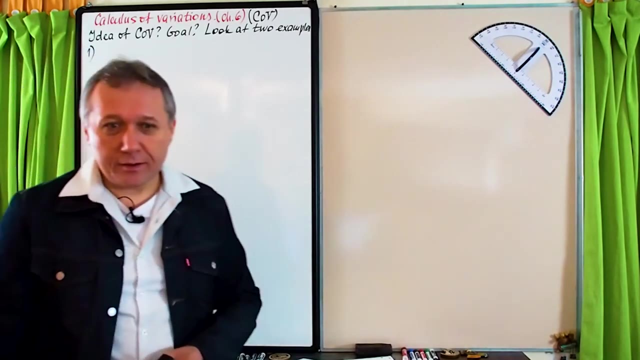 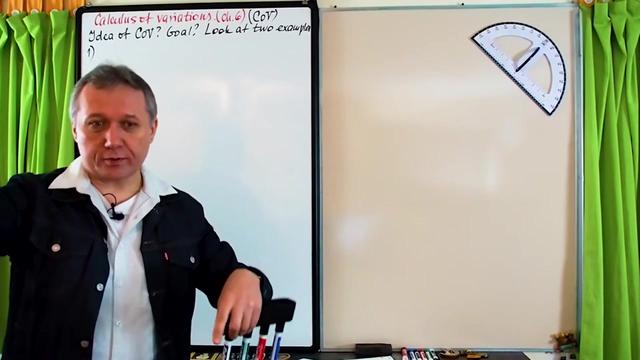 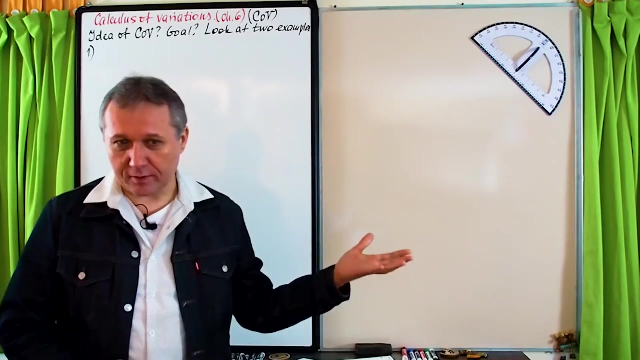 All right, look at two examples. Should I label it number one? Yeah, Okay, Number one. Let's imagine this situation. So you have plane right, flat, two points. What is the shortest path between these two points? Of course you can say, come on, it's obvious, right? 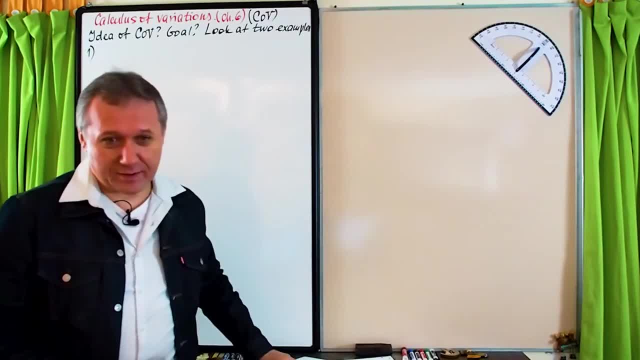 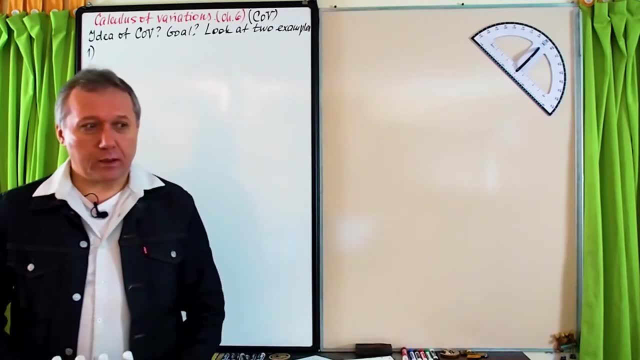 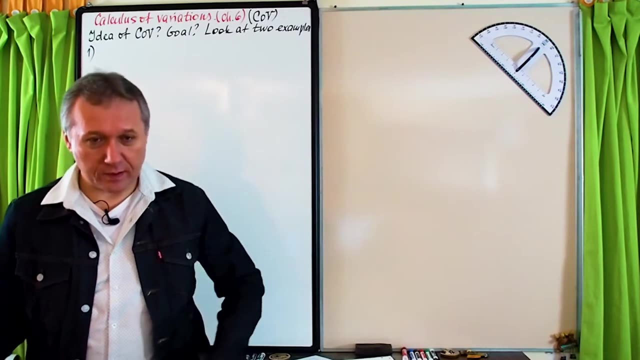 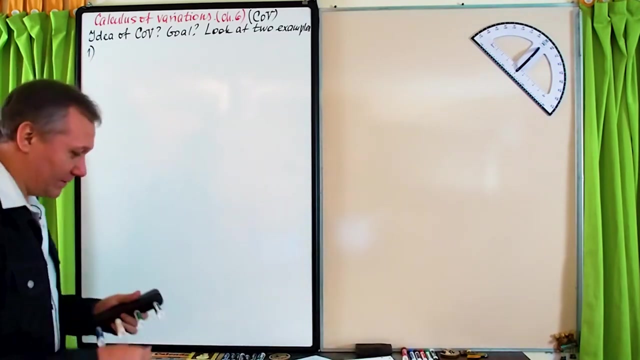 Yeah, We have that situation in our everyday life, right, But we need to develop a tool which can be used to find, to solve problem like this and problems similar to this. right, Some mathematical tools which wouldn't be based on our everyday life experience, right? 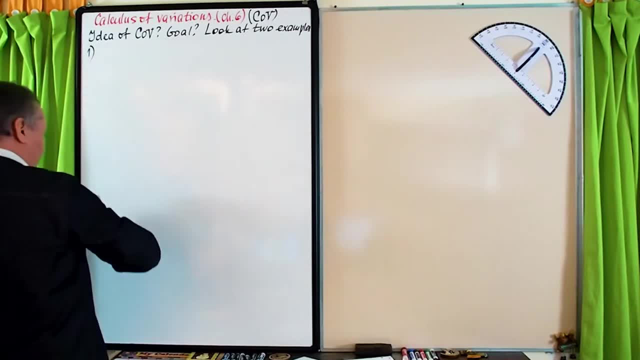 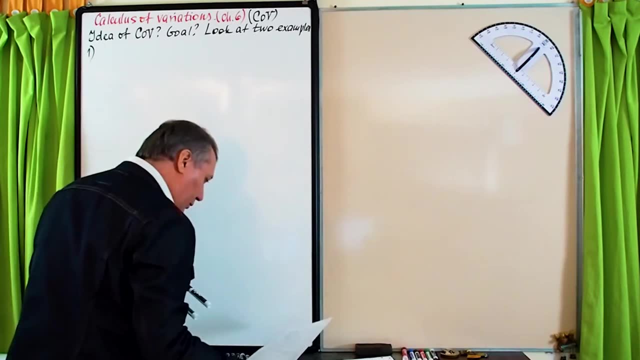 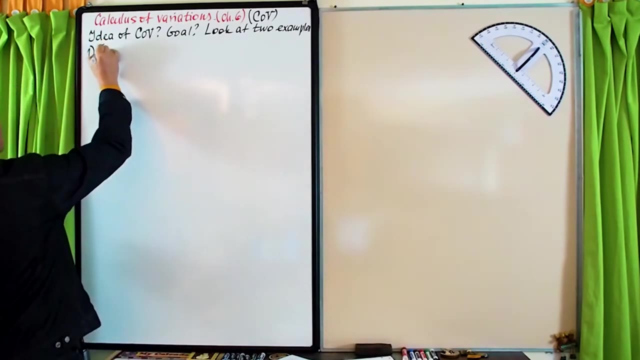 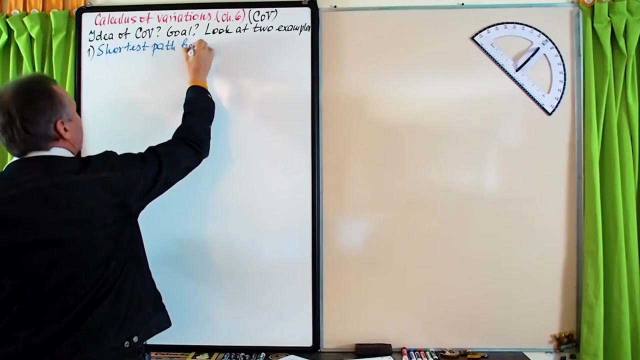 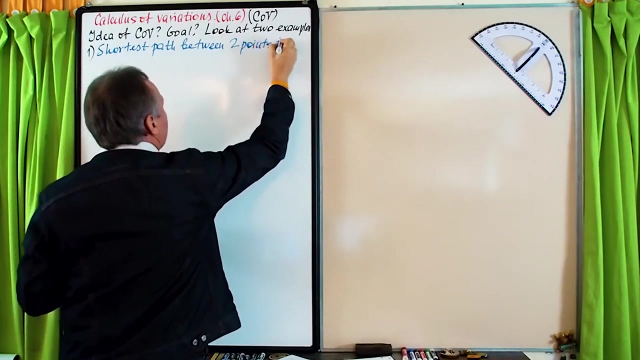 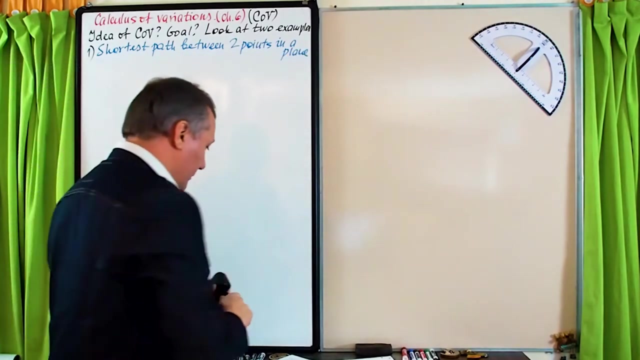 Okay, So the shortest path in the plane between two points. All right, So should I. Yeah, So, the shortest path between two points. So let's imagine in a plane two-dimensional situation. right, Okay, So let's draw the situation. 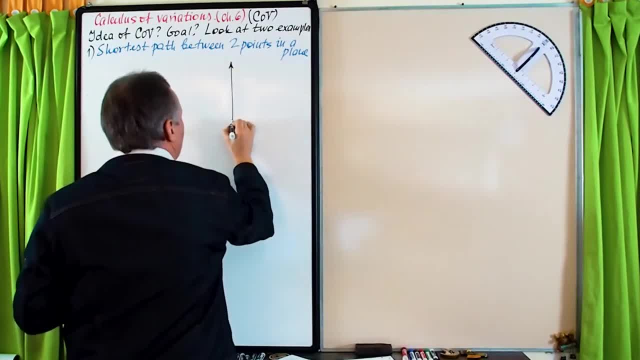 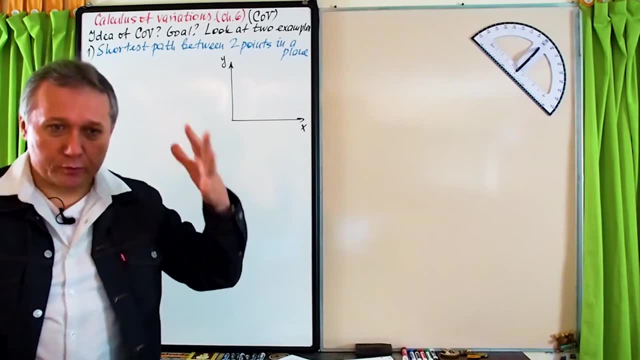 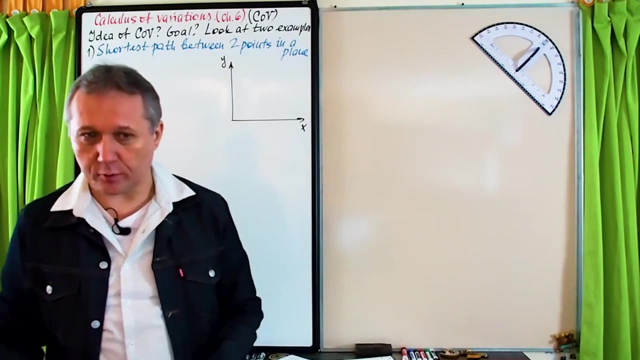 All right. So let's say x, y and every time if you have a problem like this, of course you have a beginning, you have end. End points are fixed right. You know your beginning, You know where you want to be and you want to find the shortest path. 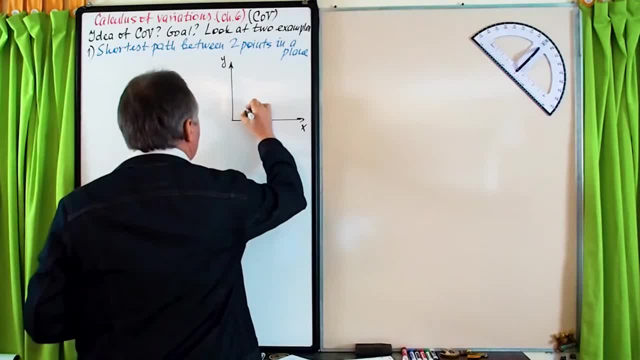 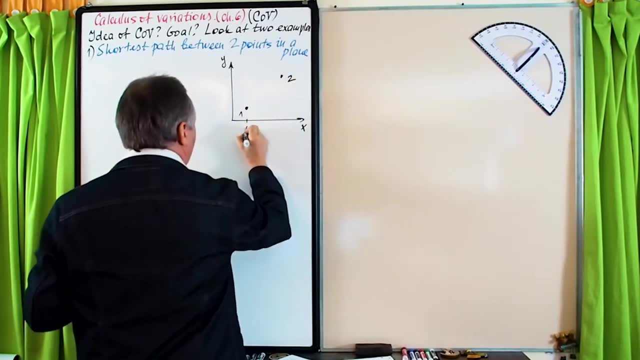 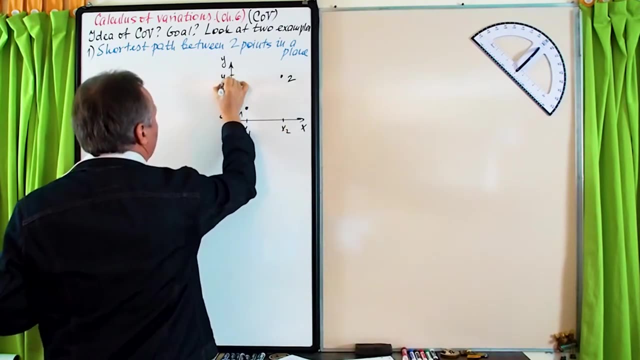 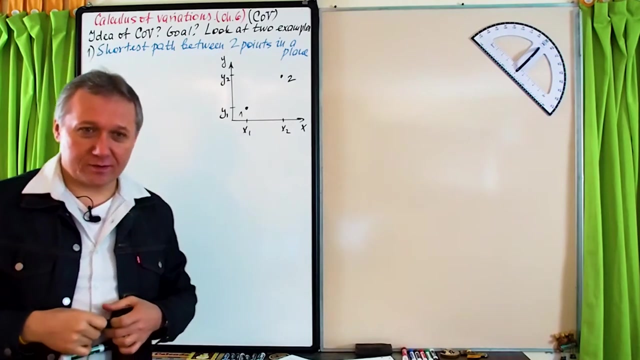 path, so the endpoints are fixed. so let's say, this is initial and this is point 2. of course, this will be X 1, this will be X 2, this is Y 1, Y 2, right, and we basically need to find the path with the shortest distance, right? okay, so how? 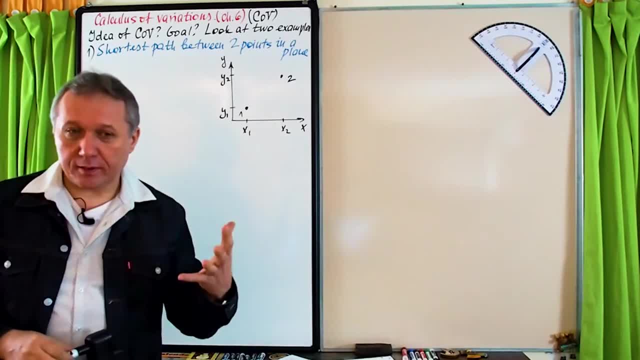 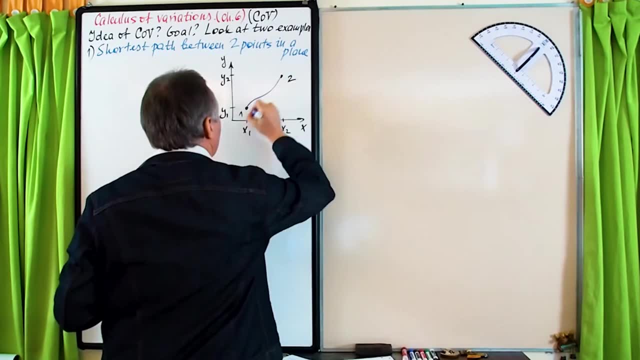 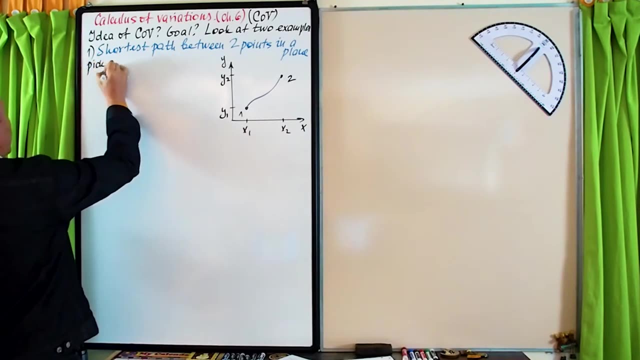 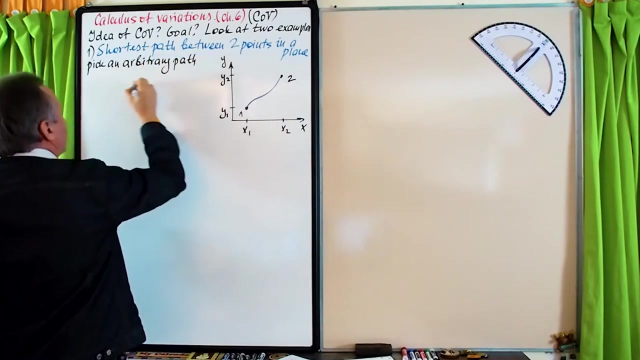 should we start it? let's pick a completely arbitrary path. completely arbitrary, right? so let's say: this is the any path. pick an arbitrary path. let's say Y as a function of X two-dimensional situation. it's basically a yes or no function of X two-dimensional situation. it's basically a yes or no. 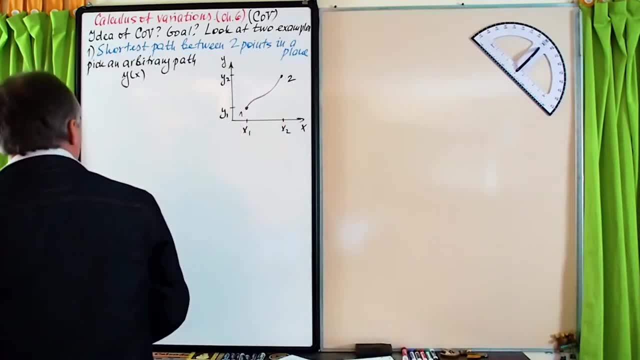 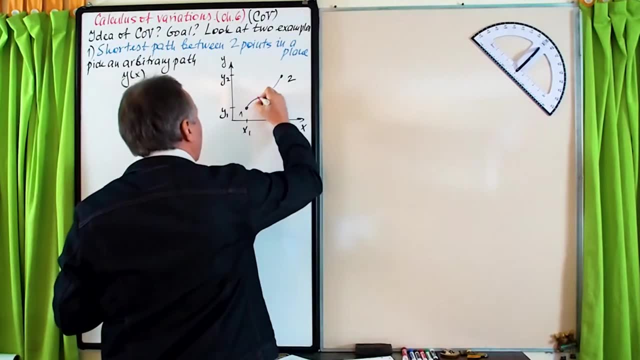 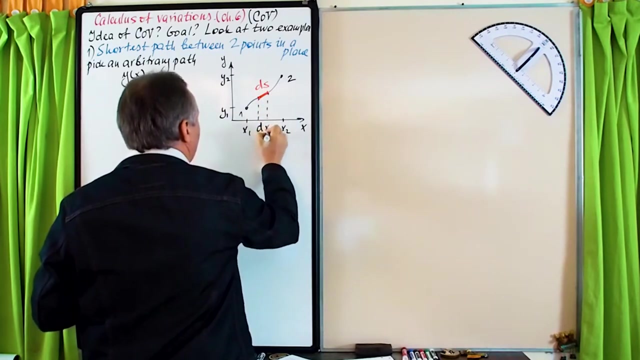 equation over some arbitrary line: Y is a function of function of X. and then what? of course we need to take infinitesimally short section of this path, right? so let's say DS, right of course, which has components DX and dy. and of right. so let's say DS, right of course, which has components DX and dy, and of course we can write the element of: 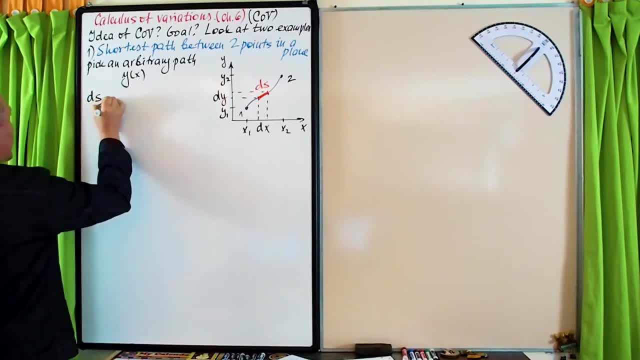 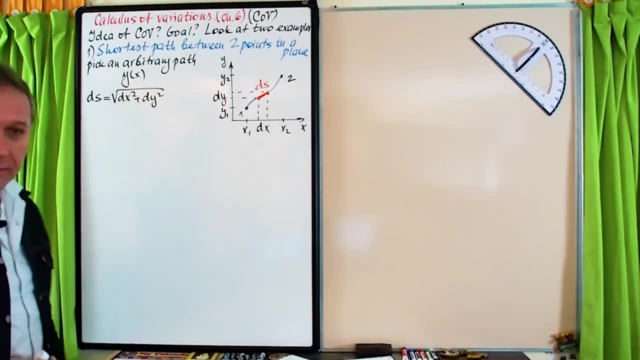 course we can write the element of the path DS easily as square root of DX, the path DS easily as square root of DX, the path DS easily as square root of DX. squared plus dy squared. okay if this is squared plus dy squared. okay, if this is squared plus dy squared. okay if this is length of DS. then if we want to calculate, 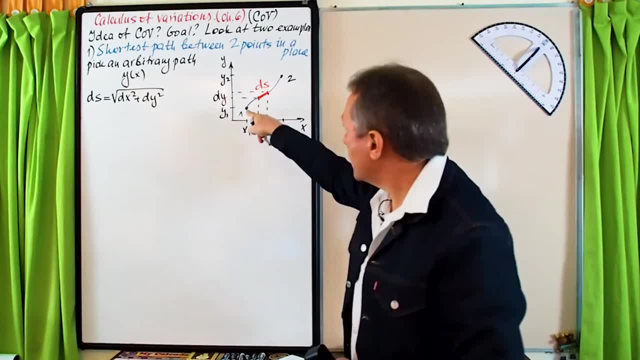 length of DS, then if we want to calculate length of DS, then if we want to calculate the total distance between these two, the total distance between these two, the total distance between these two points using this line, this path, and of points using this line, this path, and of. 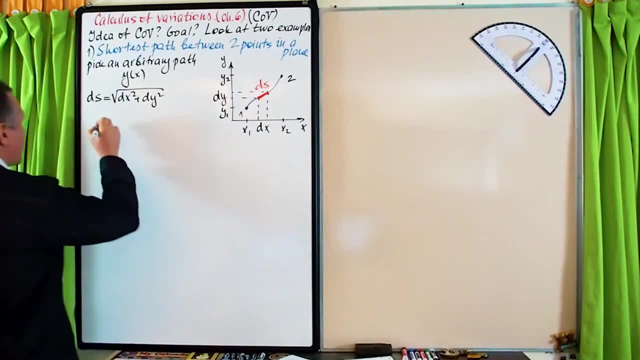 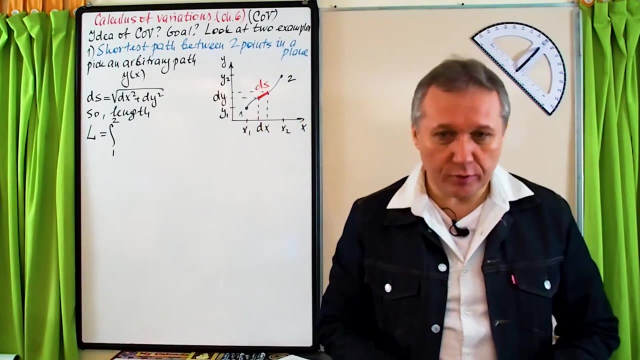 points using this line, this path, and of course I think I use L yeah, so course I think I use L yeah, so The length will be L equals, of course, integral from the first point to the second point. Right now I don't know which variables of integration I'm going to use. 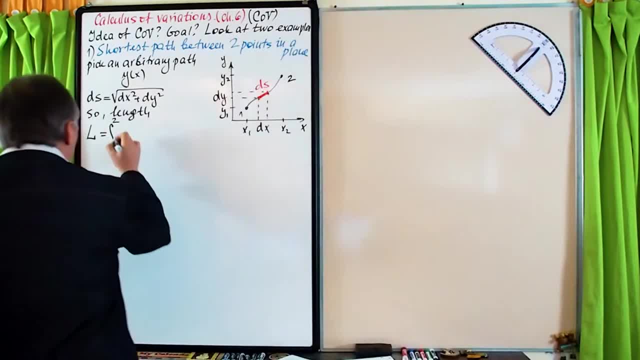 Variable of integration. so I just put 1 and 2. And it will be, of course, ds. We need to integrate that, Okay. so now of course, it will be integral of square root of dx squared plus dy squared right. 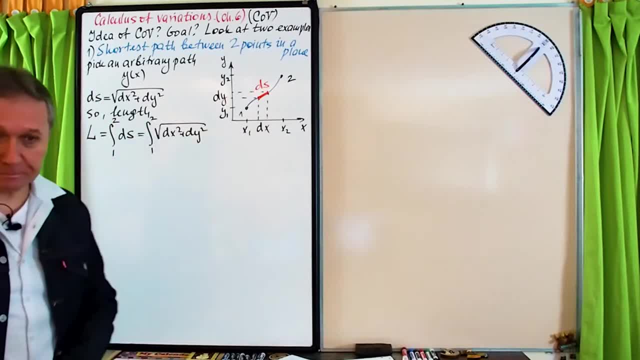 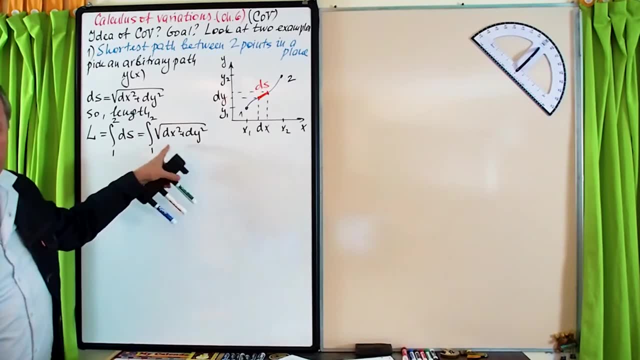 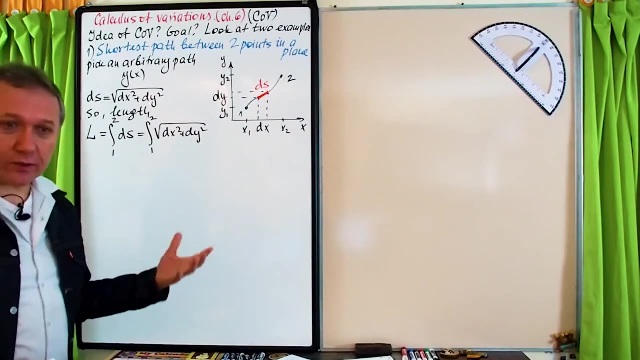 Still 1, 2, because right now we still have two variables, x and y. I still haven't made a decision about which variable to use, right? So, in order to make a decision, so now I have to pull out of this square root sign: either dx or dy. 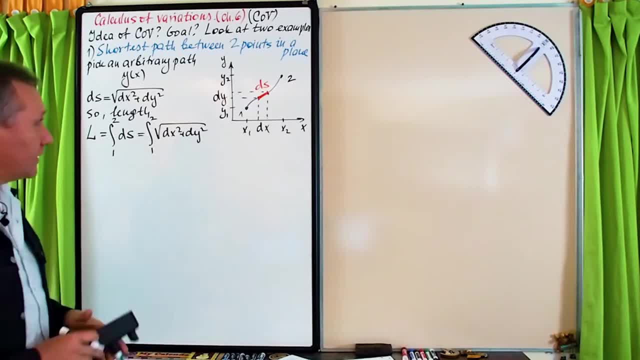 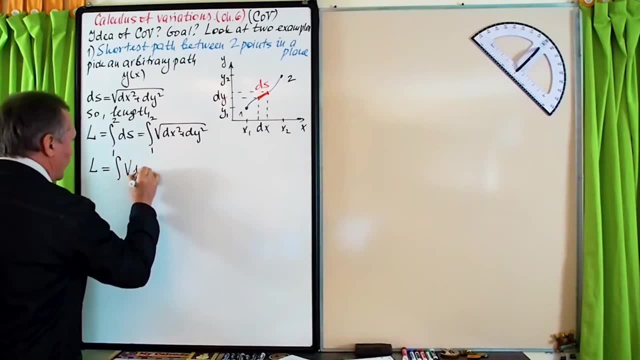 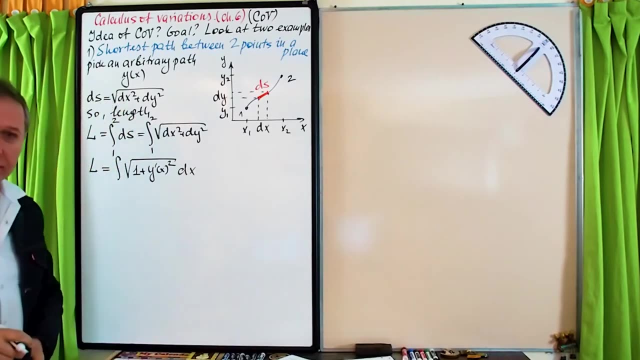 Let's take dx outside right, And in that case we will have All right. L equals integral square root of 1 plus y prime of x squared dx. So in this case, you see, I took dx outside. As a result, I have here dy over dx prime. you see prime n squared. 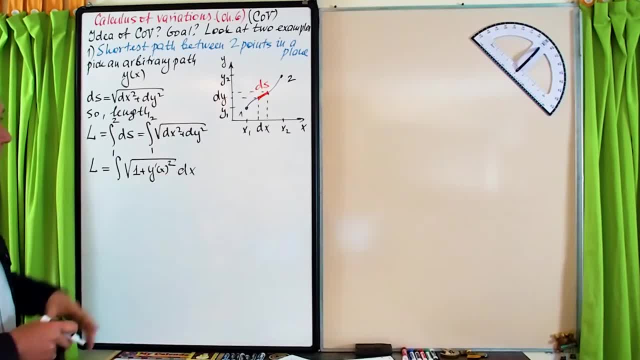 So now, yeah, we have one variable of integration, x. So now I can write from x1 to x2.. So that's what we have. Let me frame it like this. And now again, what's the goal? 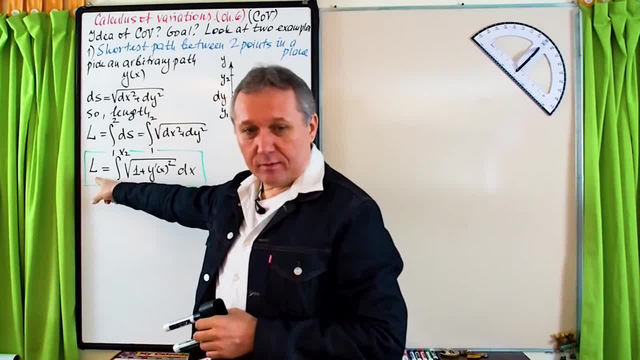 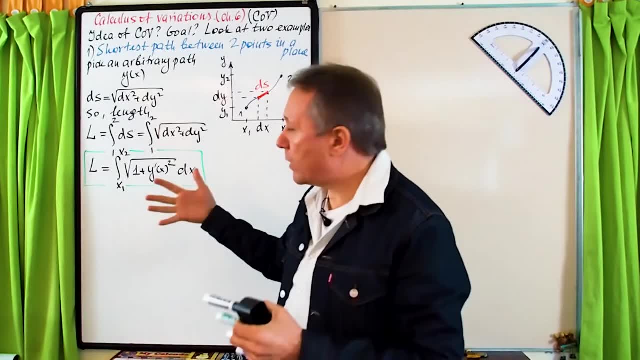 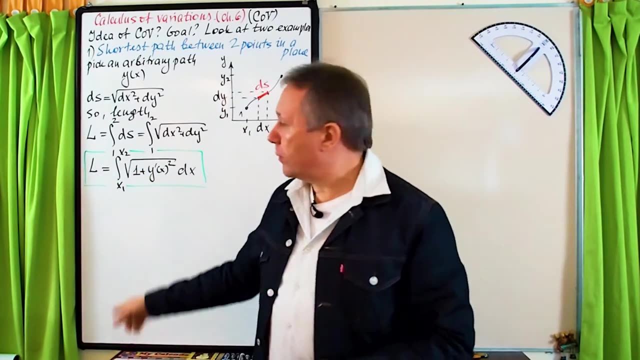 The goal is to make this, to minimize this right. We're trying to find the shortest path. So basically, by looking at this, you can say, yeah, we have almost everything, We have endpoints given right, We have an integrand, except for we don't know the true path. 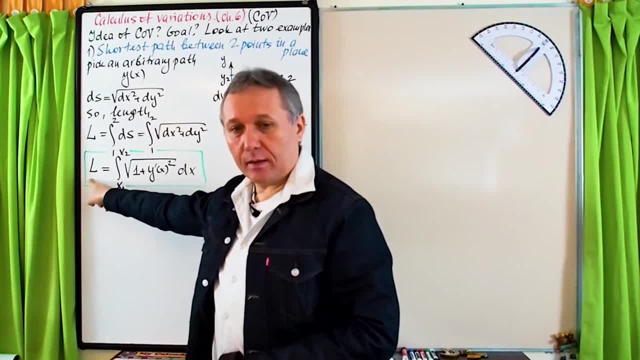 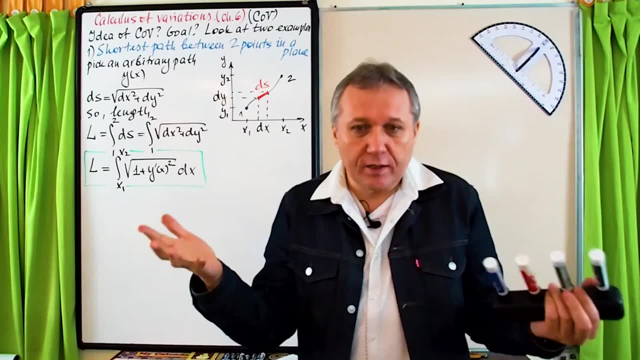 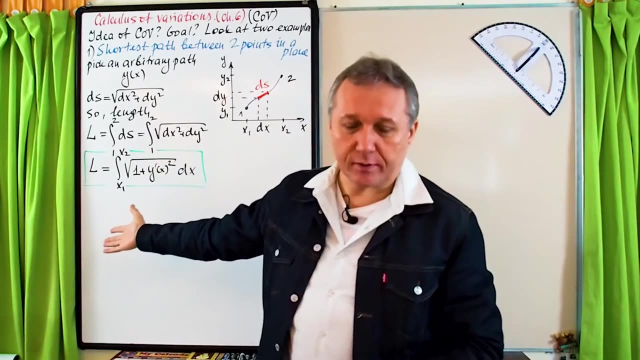 The true path which makes L minimum. So everything is given except for what is actual, correct path. the true path, which is y, is a function of x, because right now we just pick an arbitrary path. But of course we need to find that single, unique path. 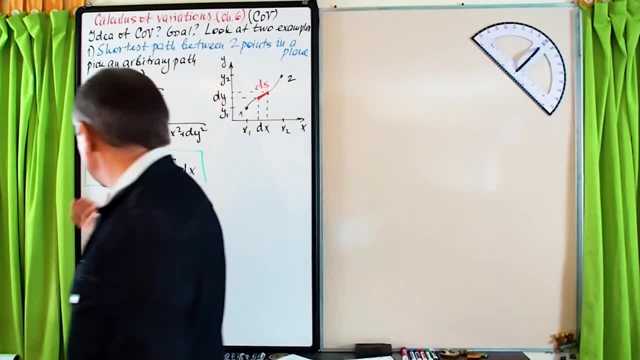 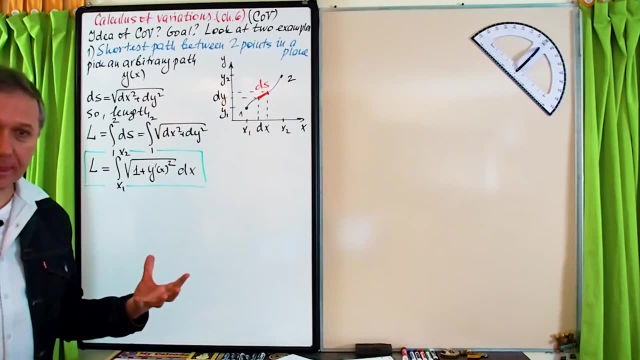 which is going to minimize this distance, this distance, right? So basically, we need to. we need to develop a tool which can be used to find the true path. y is a function of x which makes this minimum, But of course, we're going to develop a tool which is going to make this stationary. 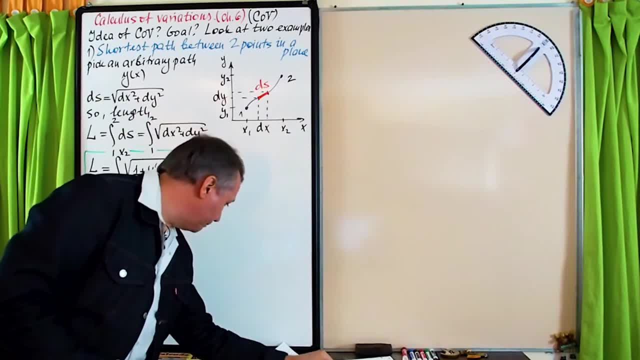 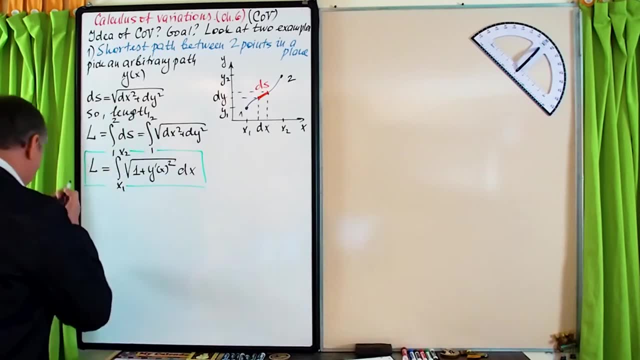 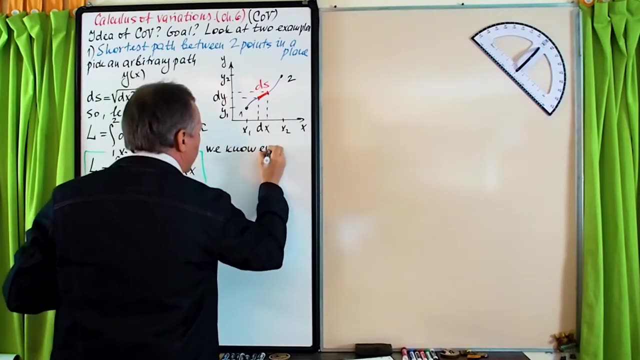 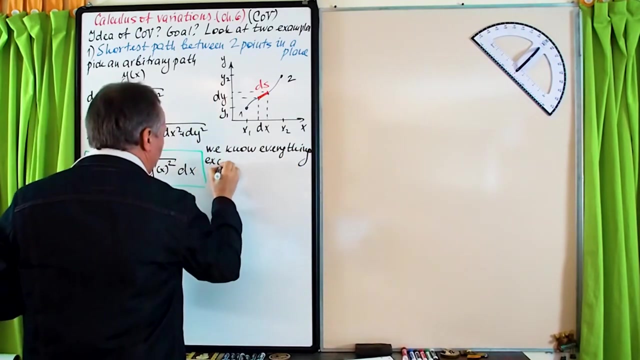 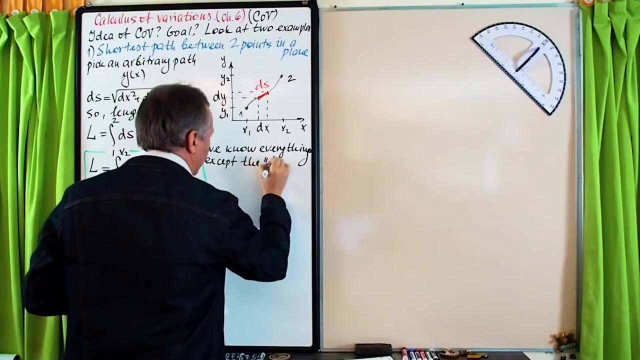 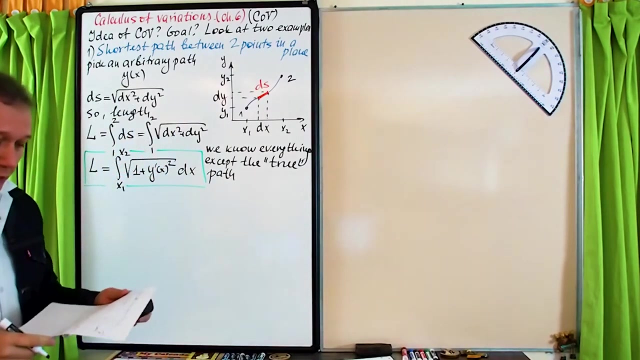 But we will talk about this later. All right, so now let me So, let me write. So here we know everything, everything except except the true path. the true path to make L minimum, to make the distance L. 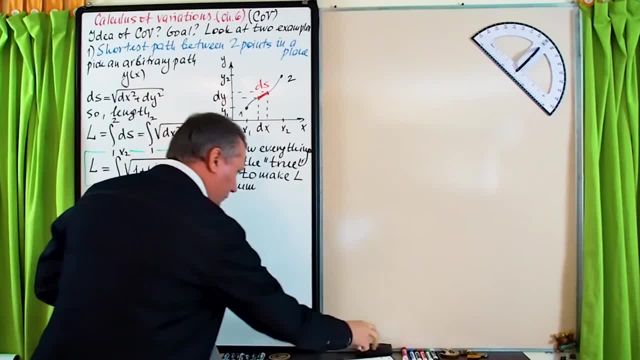 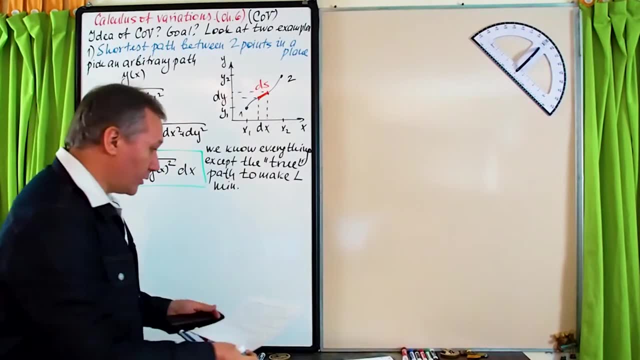 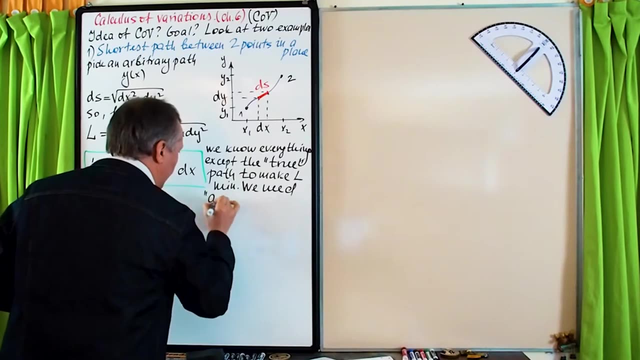 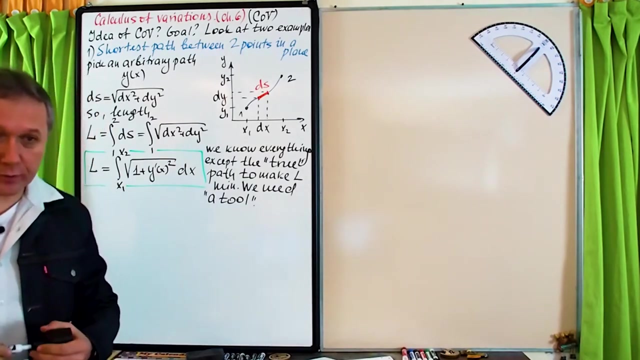 wait, let me just abbreviate min minimum. Okay, so we need a tool. So we need a tool kind of tool. Of course we will derive it, But for now, you see what we need. We need to find some. 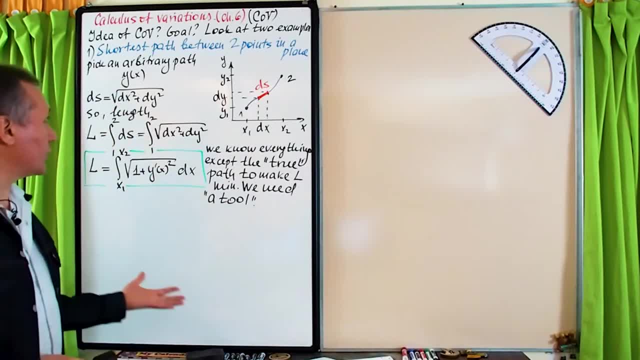 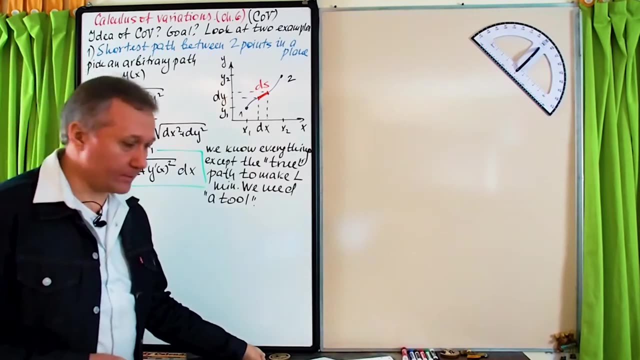 we need to have some procedure which will allow us to find the true path, us to find this y, so that in this integral l, so that l is minimum, l is this integral right, so this l is uh, minimum. there will be situations where, uh, you can have to maximize, but in our 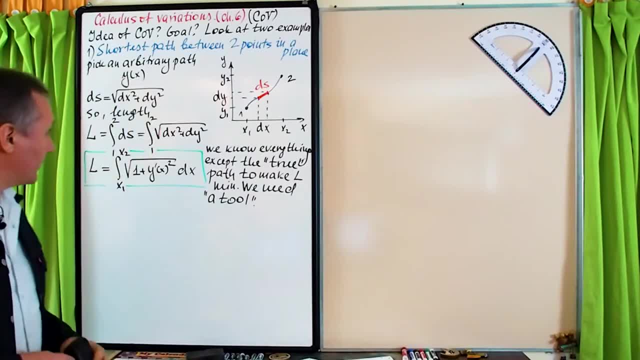 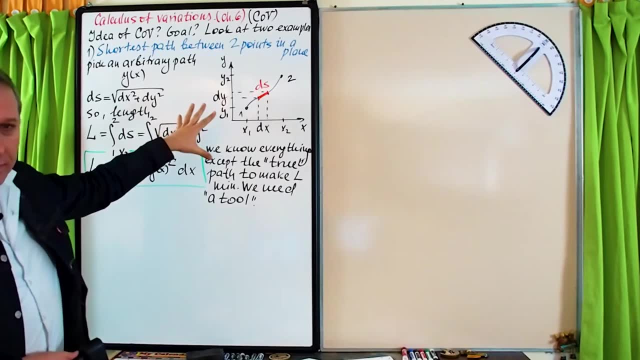 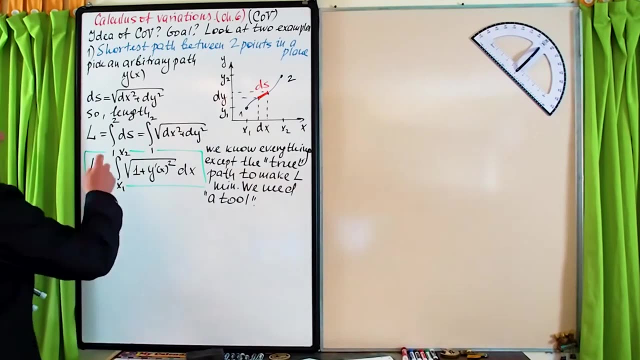 cases, or most of the time, we are going to search for minimum. so that's one, one example. we're going to finish it all right, so we will leave it behind for i know, 20 minutes, um, develop the tool, and then we'll get back to this example. the second example: so, uh, what if? uh, fermo principle. so you know the. 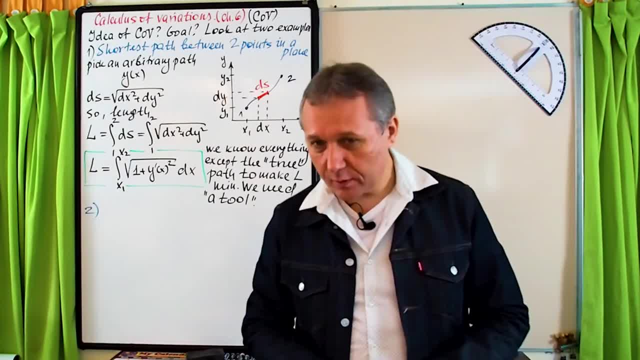 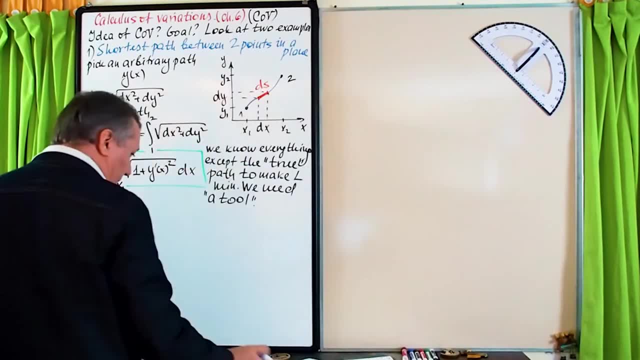 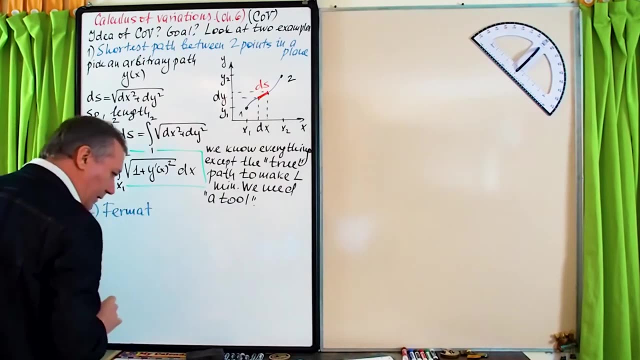 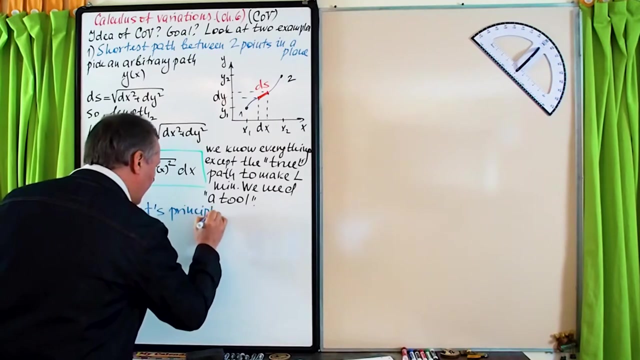 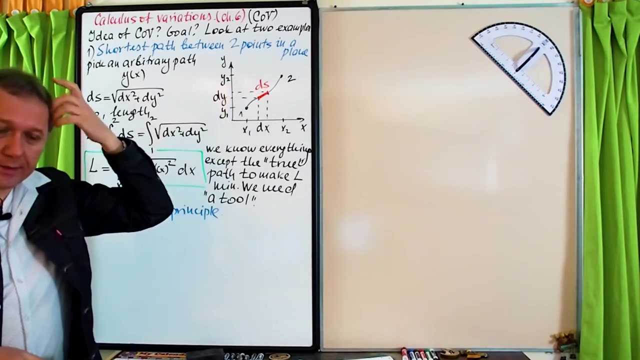 light travels between points, trying to minimize what, of course, travel along the path. minimizing time: right, okay, fermo principle, all right, fair, ma right, the yeah principle, basically, uh, again, two-dimensional situation: right, so you have x and y. uh, initial point, final point. right, so you pick some arbitrary path. okay, let me. 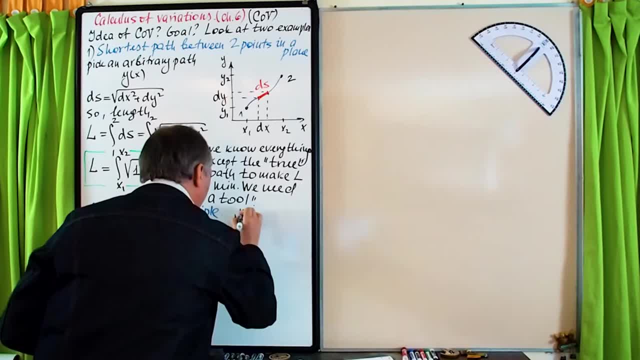 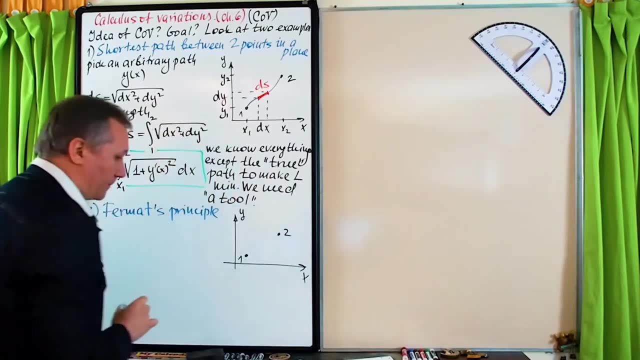 uh. redraw basically the picture again. it will be y, okay, uh, x, uh, point one, point two: again the same story. you will pick uh, some uh. every time you will pick some arbitrary path. all right, right now, it's not, of course, it's not going to minimize time. 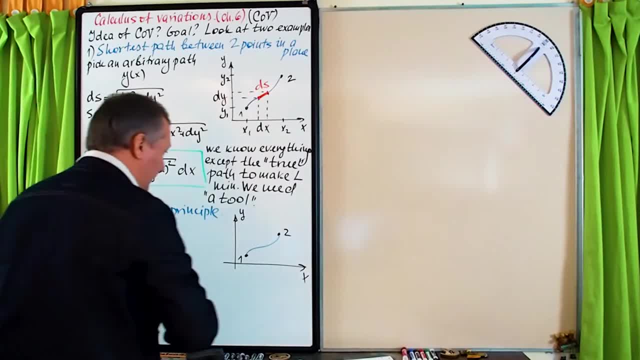 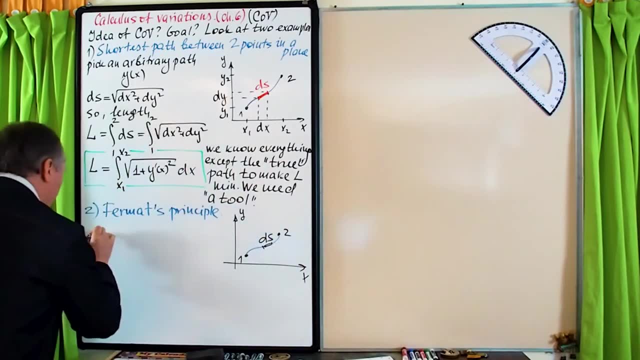 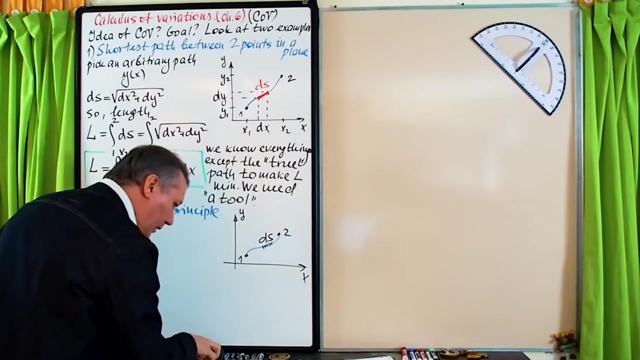 when we set up the problem right, uh again, you will take uh ds, right. and so now, uh, instead of minimizing distance, distance, now we are going to minimize time. so now, um, so tau- i think i label it tau- um, yeah, so it will be integral of dt. 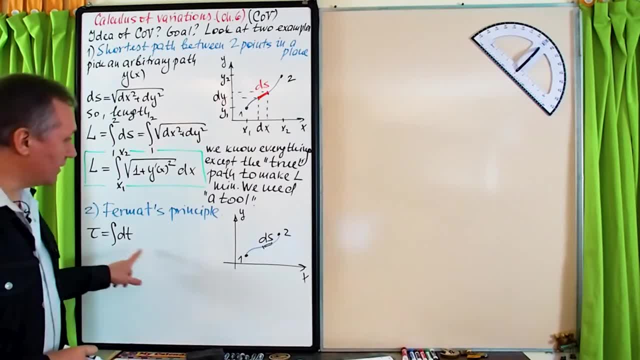 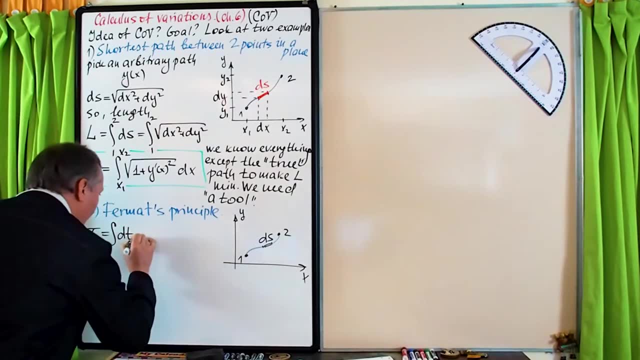 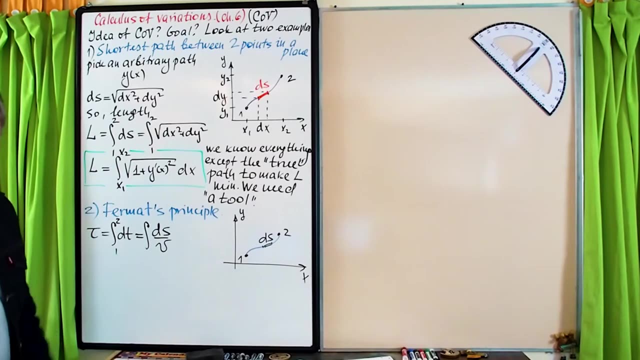 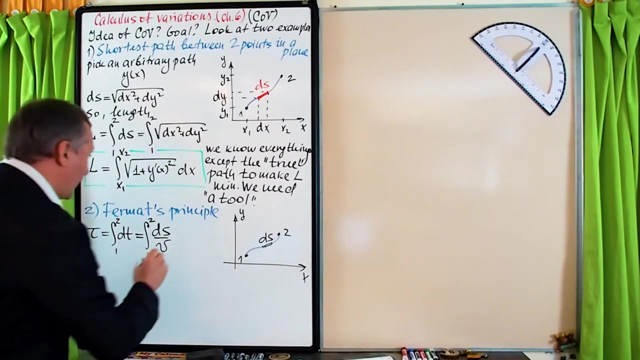 right, so basically dt. it's a time to uh to cover this ds, right? so it will be, of course, uh. from one to two, integral of ds divided by v, simple math, i mean simple physics, again, from point two point, from one to two. synchronize to two. all right, uh, ds. 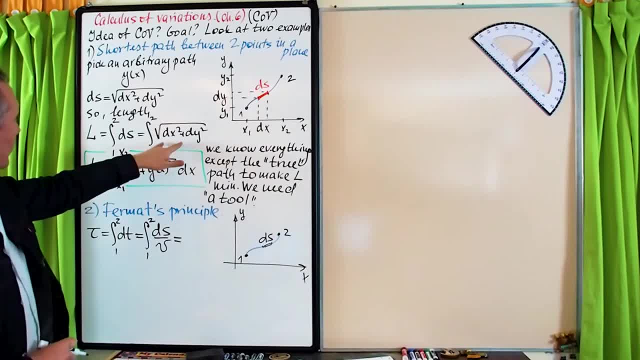 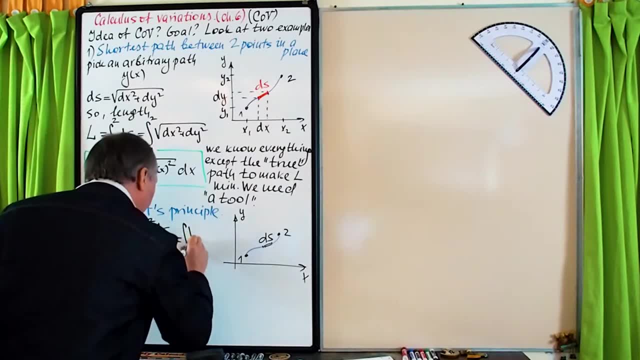 uh, we know we can. we already wrote down ds over here. right again, if you take dx outside, okay, let me write it. so first, dx squared plus dy and left d horn is equal. so that's some explanation to greater aaren했던. so i will take this outside. all right, so that's nice. so if you have 20 points and we are getting 90 points here, so 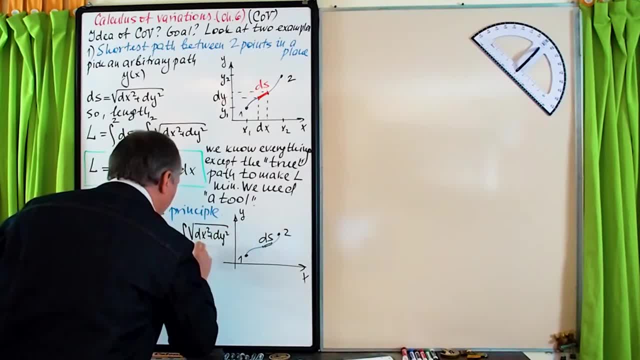 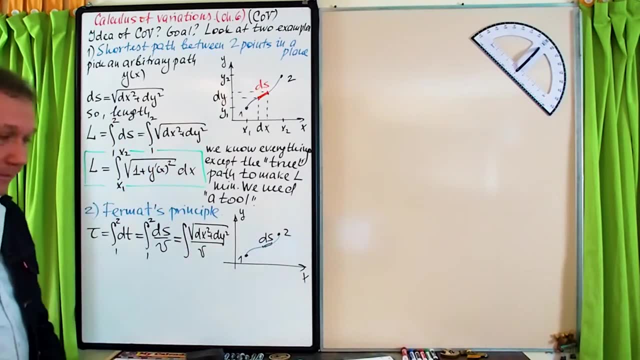 dx squared plus dy squared right and divided by. okay, let me write first v And now. so how can we write v? Of course we know the index of refraction, which can be a function of x and y in the most general situation. 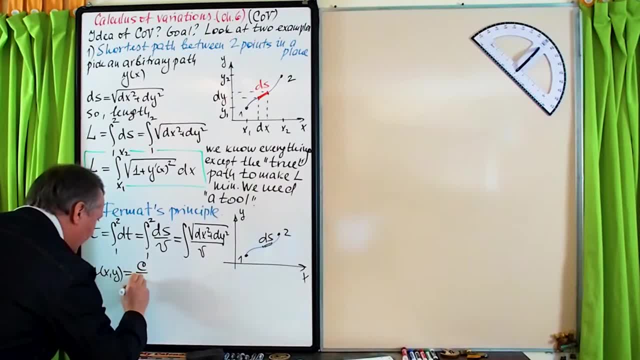 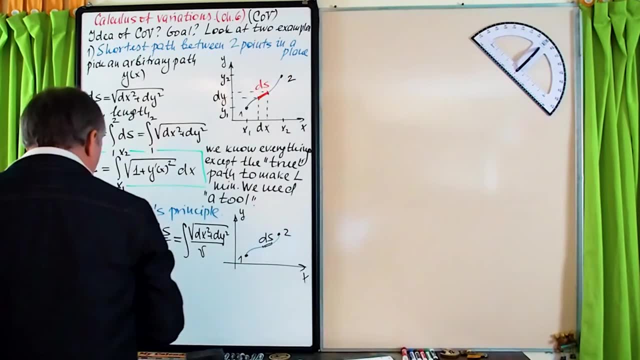 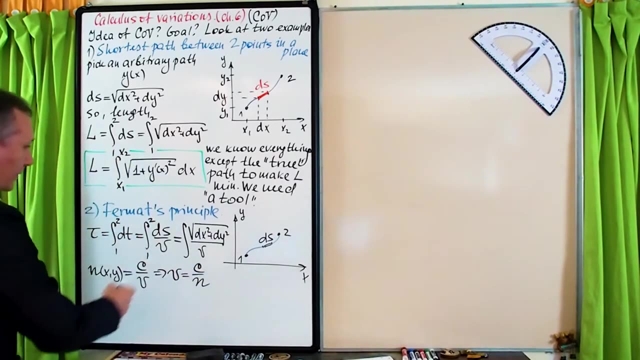 Of course it is introduced as c speed of light divided by the velocity of light right, So v will be c over n right, So we'll plug it. As a result, tau will be equal. 1 over c will be downstairs, so I will take it outside. 1 over c integral. 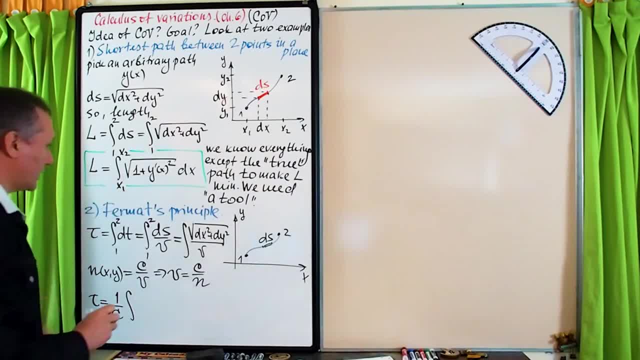 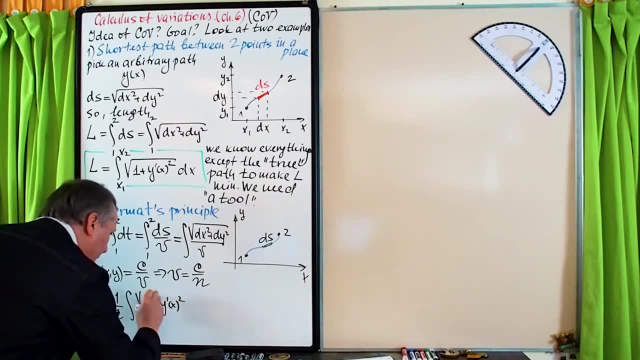 Now I will take dx outside, like we've done here, I've done there. So it will be square root of 1 plus Y, prime of x squared. Then n will be also upstairs. Let me write n as a function of x and y and dx. 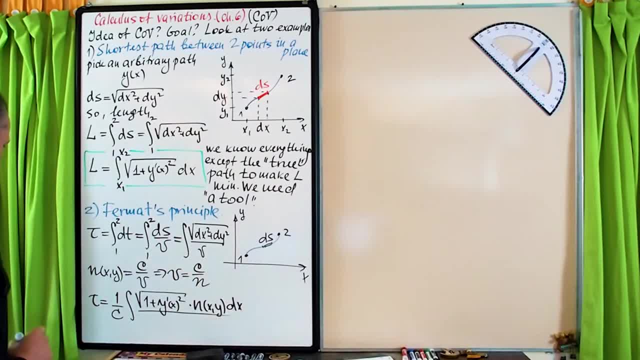 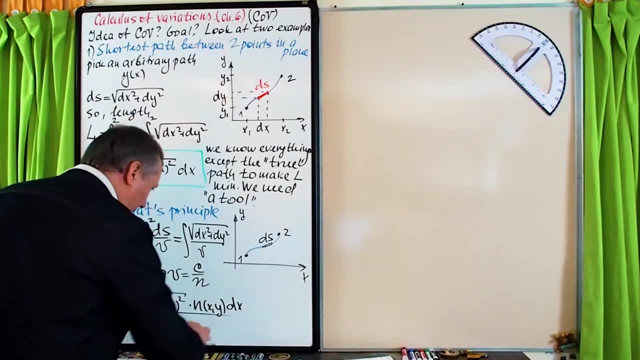 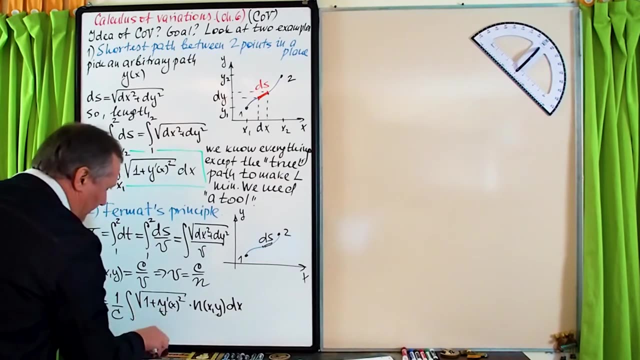 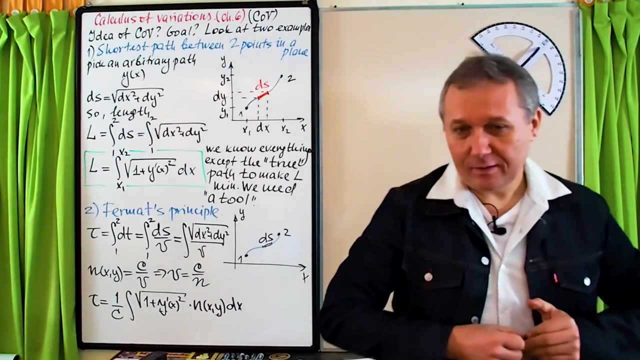 And divide it. That's it right. C yeah, yeah, So nothing, there's no division. I took c outside, I took it outside already. Okay, So that's the integral in this case. So here we minimize distance. 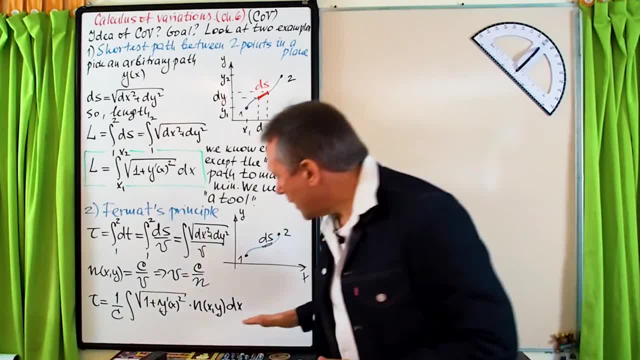 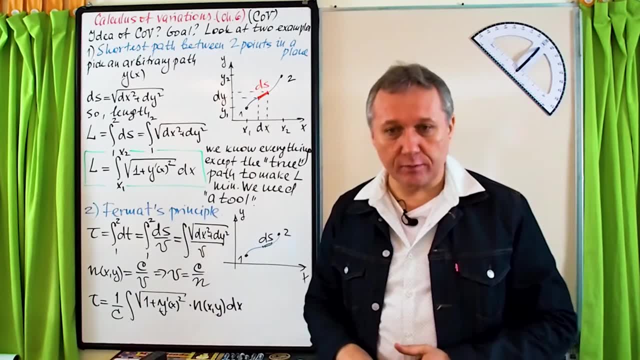 Now we're minimizing time to minimize time And again the same story. Everything is known, like what I wrote here, except for the true path: y as a function of x. Right now, we picked an arbitrary path, but of course you need to optimize and find the true path. 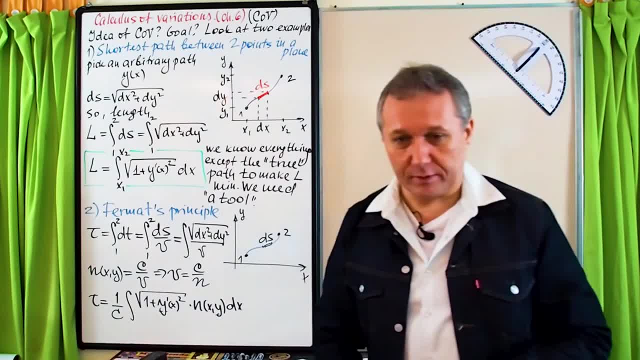 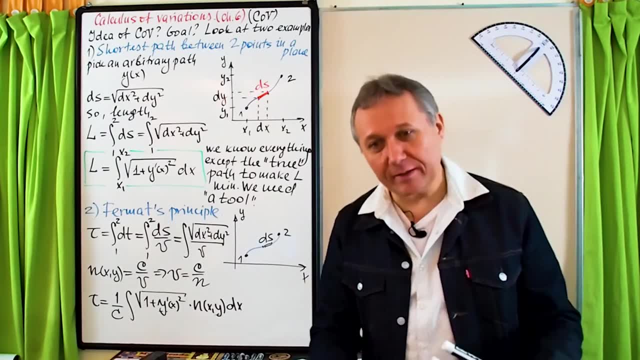 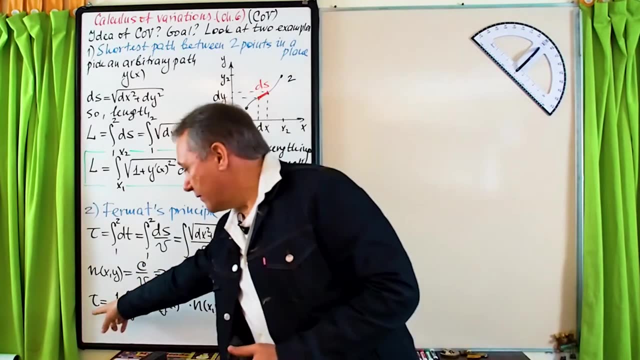 which is going to minimize the travel time, right. So the second example: again, we need a tool so which can be applied, used to find the true path and which would guarantee that this the value of this integral here, or there will be minimum right. 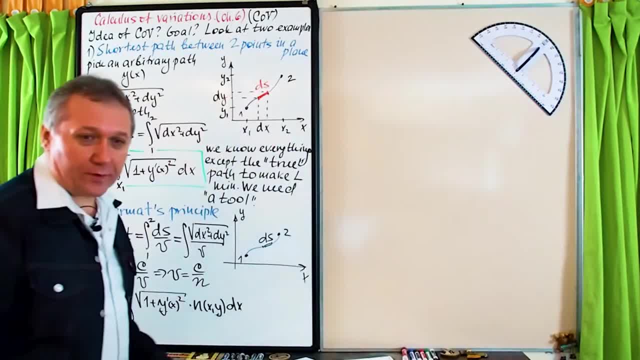 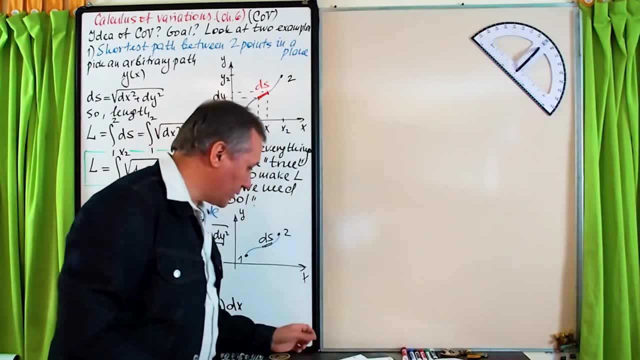 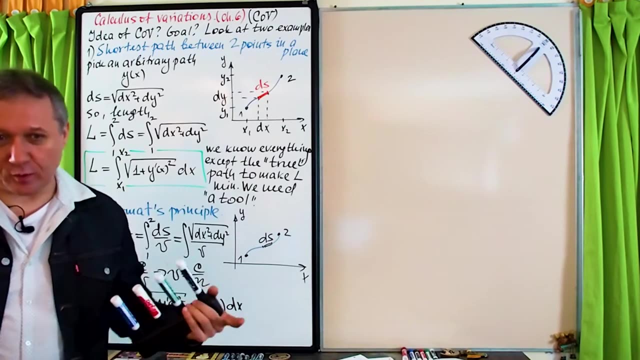 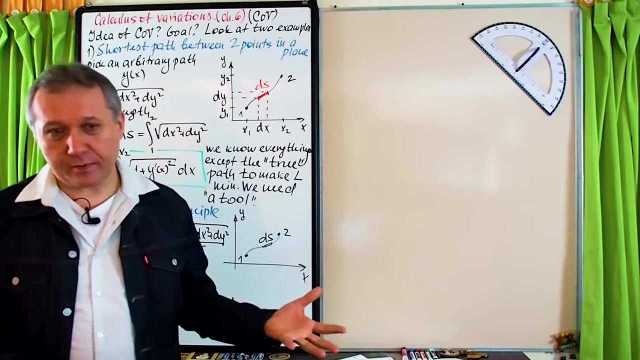 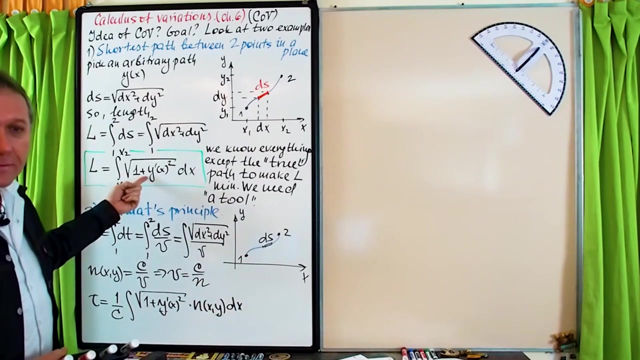 So that's the goal of calculus of variation, using this example, As you can see, And now let me write. So the calculus of variation, sort of like a precise definition of the goal of calculus of variation, is about. calculus of variation is about finding extreme values of these integrals which we are going to call functionals. 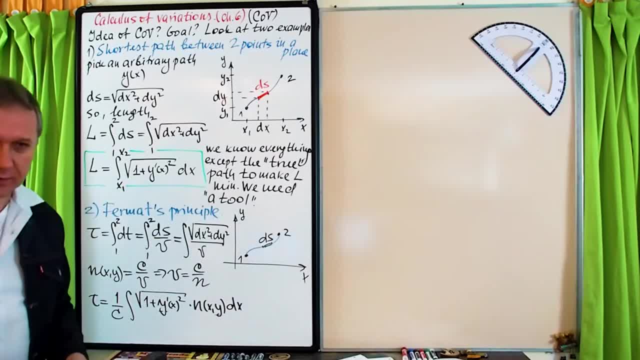 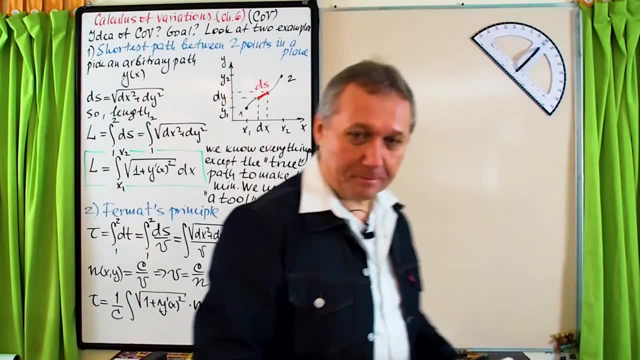 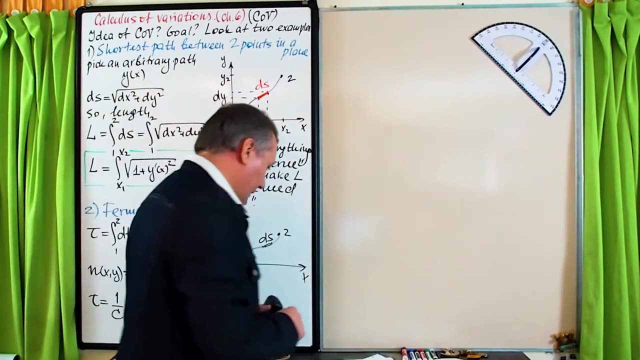 I will define in a second function, Functionals, right? Basically, these functionals, like quantity, are presented in an integral form, right? Okay, so let me write a strict definition of the goal and then we will start working on the tool which we need to find this true path. 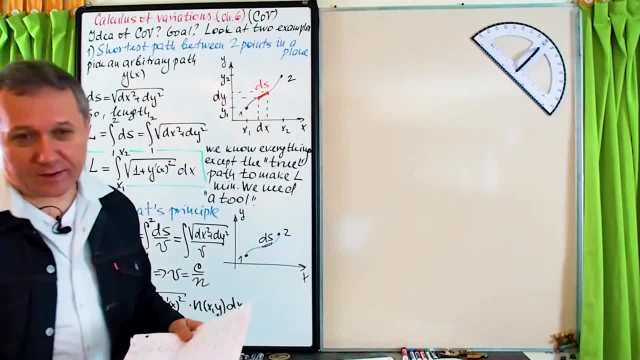 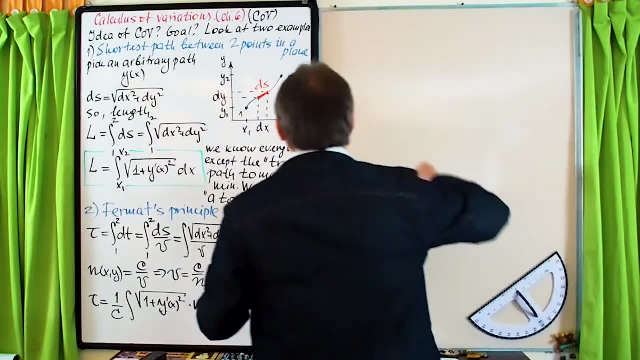 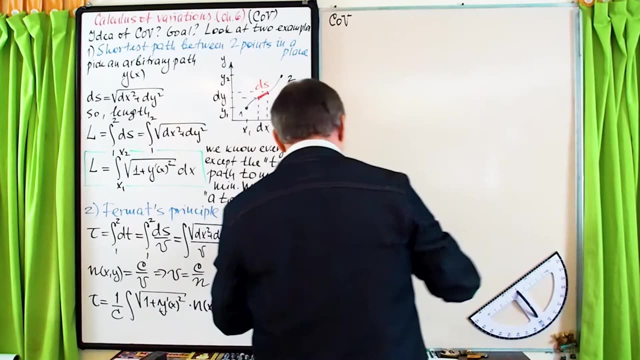 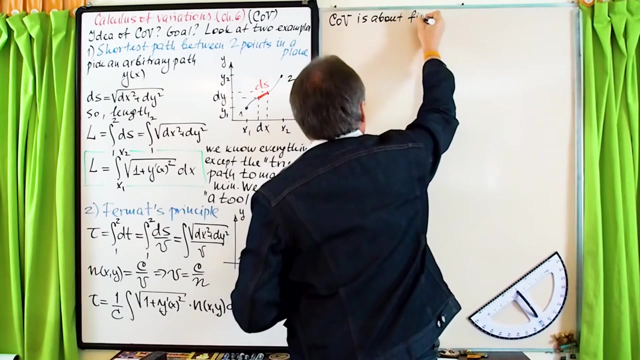 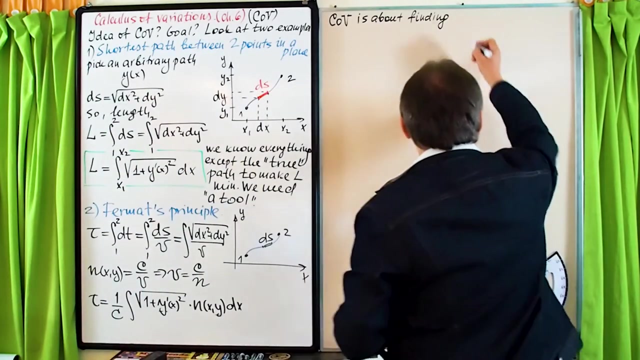 Okay. so the calculus of variations is about finding extreme values, as I said, of functionals. So let me take this down. So C-O-V, again, calculus of variations is about finding extreme values. Okay, Okay. 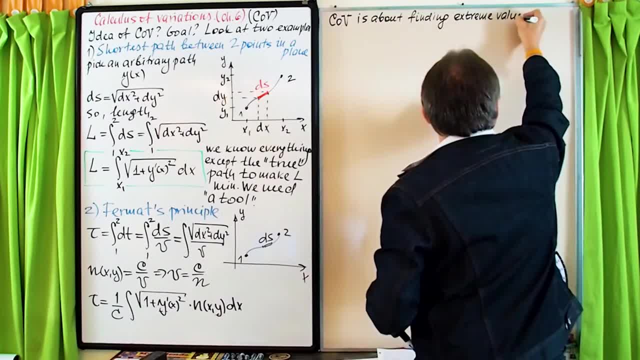 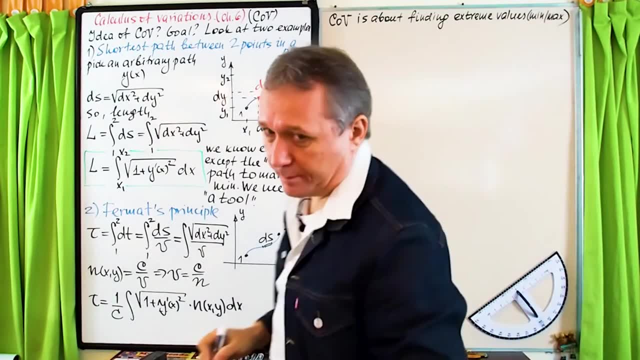 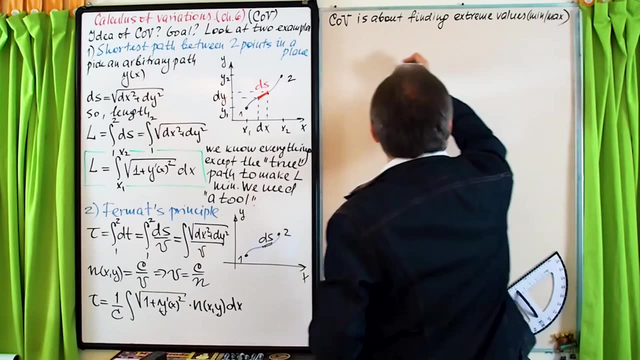 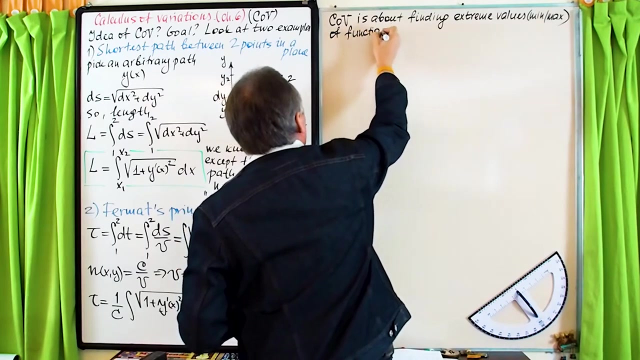 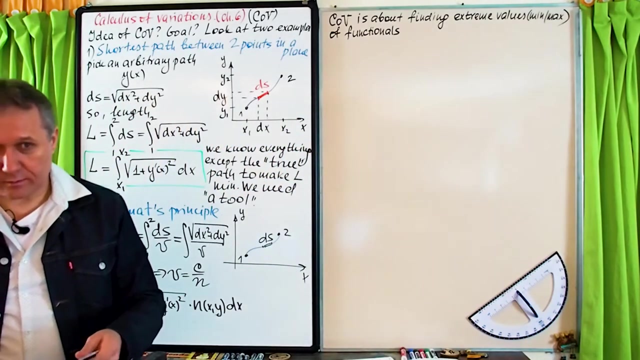 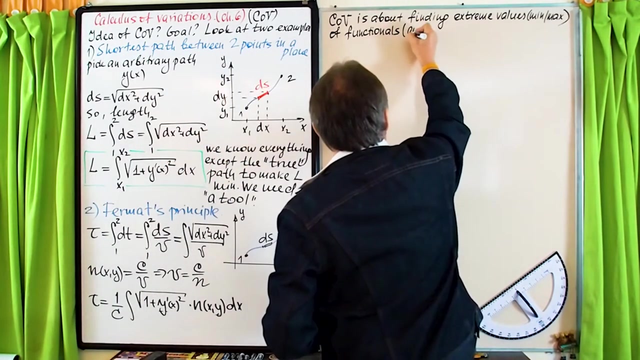 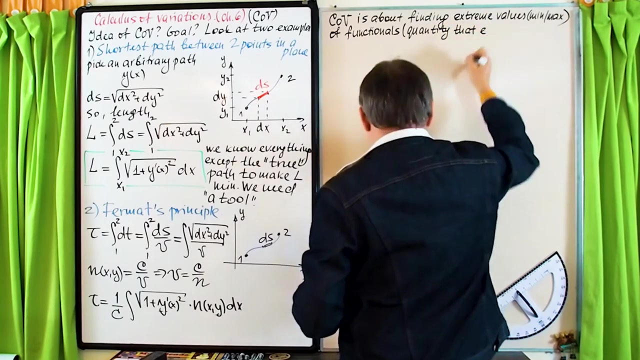 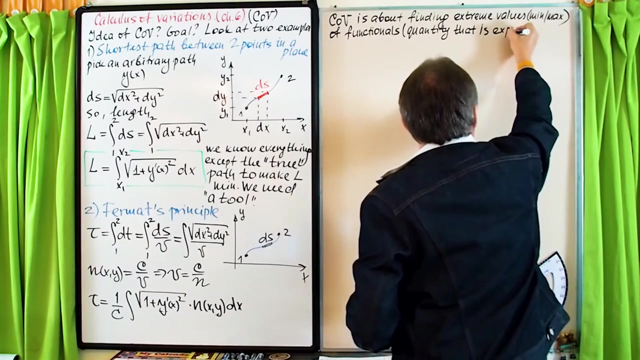 Okay, Okay, Okay me write: yeah, extreme values, so it can be mean minimum, can be maximum. extreme values of functionals, all right, of functionals, basically quantities that are a quantity that is expressed as an integral, so, and that is that is expressed as an integral. 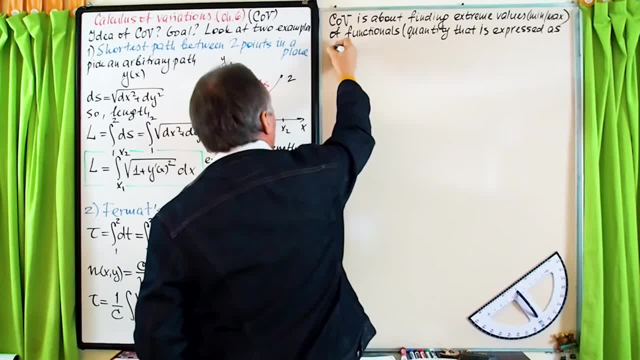 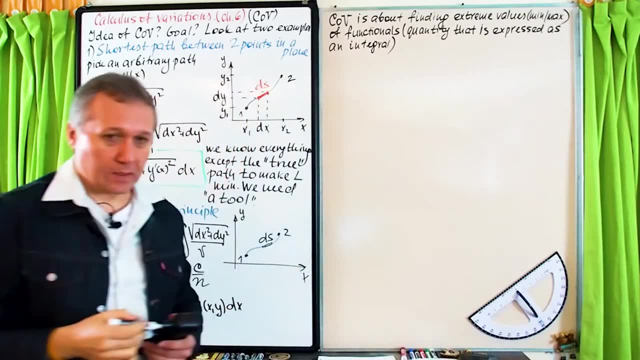 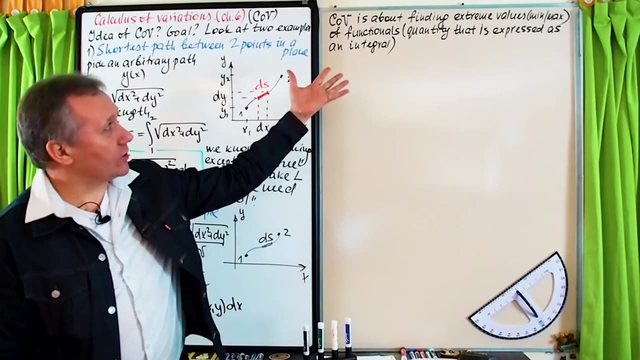 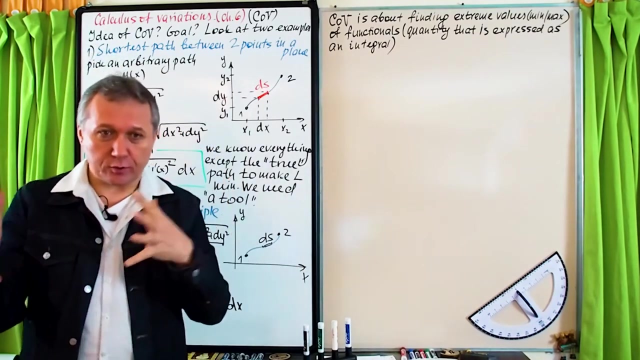 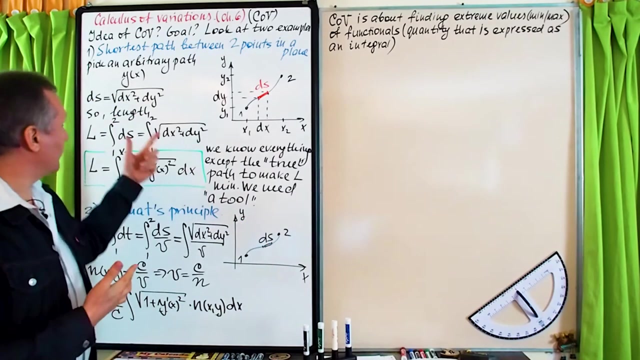 all right, and the major difference, um, and the major difference between functions and functional. on purpose, they change the name sort of function, but now they added al functional to distinguish between these two mathematical ideas. so in a function, what do we have as inputs? for example, y is a function of x, it's a function. 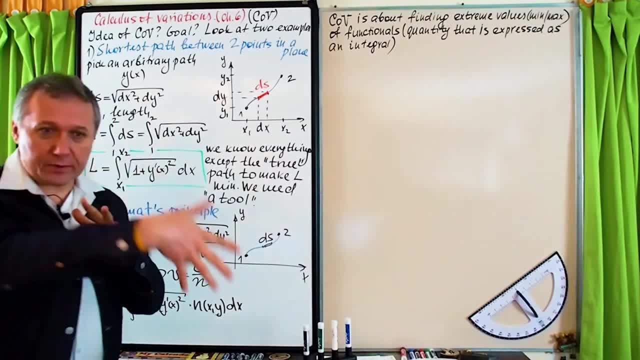 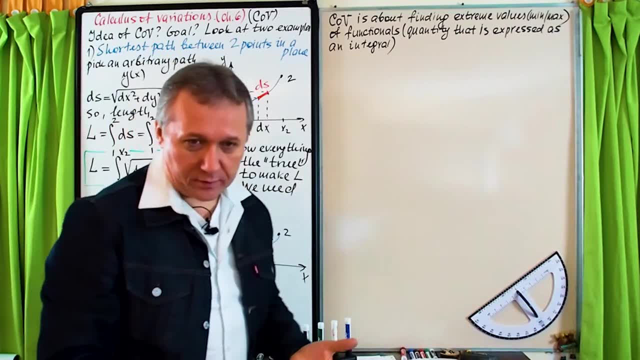 so now, inputs x numbers, outputs y's also numbers, so numbers in numbers, out in a function of x. it's a function of x, so it's a function of x, so it's a function of x, but we have functionals. what do we have functionals like in this case? so what do we have as inputs? 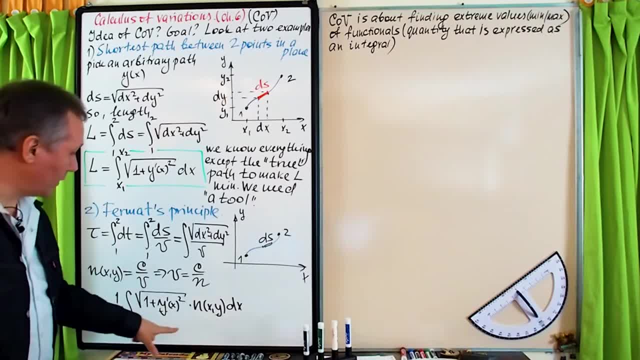 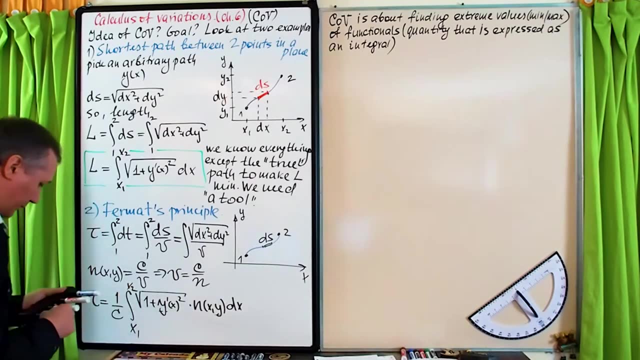 we have functions n as a function of x and y, then y prime, right? so, Mister, as inputs, we have root for the answer functions as an output, because these are definite integrals. oh, i forgot to put the limits from x one to x two, right. so inputs, functions, outputs, wood and their numbers rightrose, and we don't have to keep. 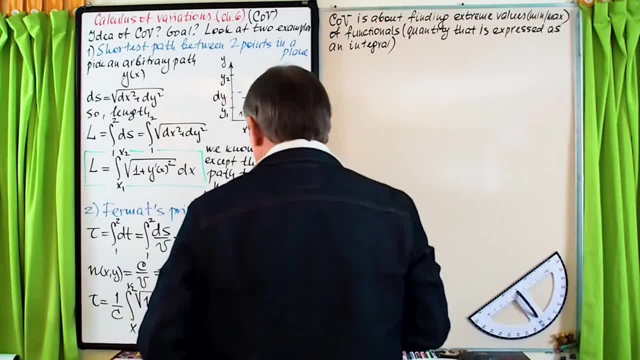 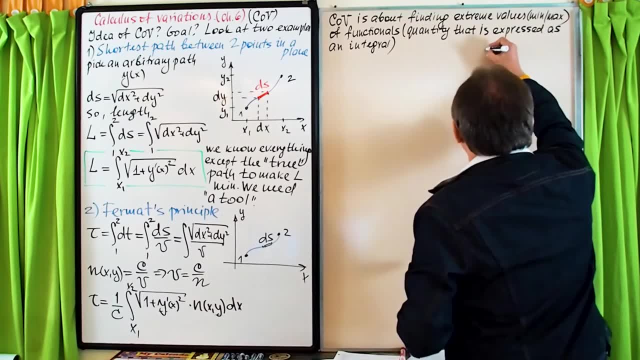 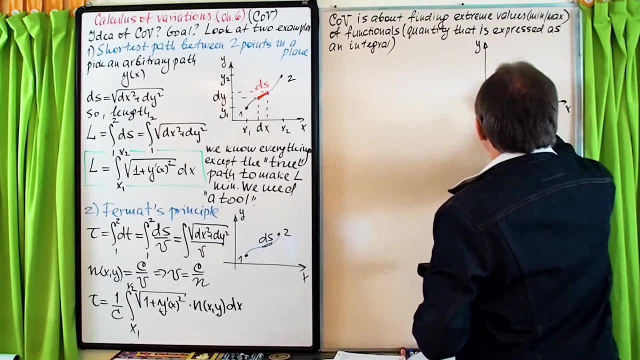 it in order to know them right kanssa. let's say, we can't know them. every force right? so what's okay? so and and, uh, sort of graphically. usually, uh, something like this is drawn: so let's say this is y, this is x. let's say: this is initial point, this is the final point. 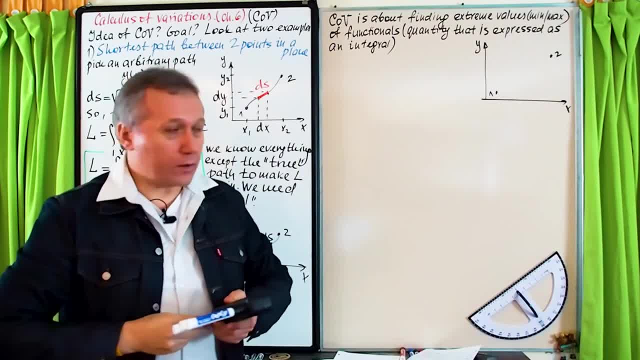 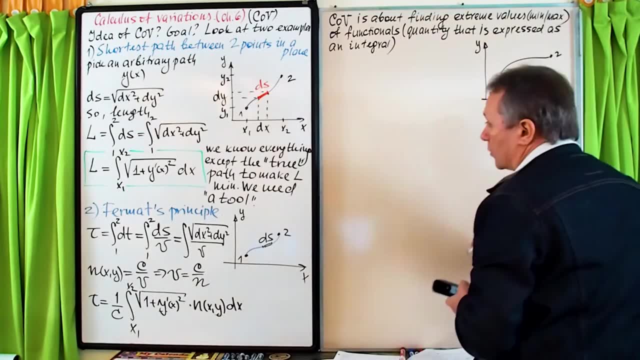 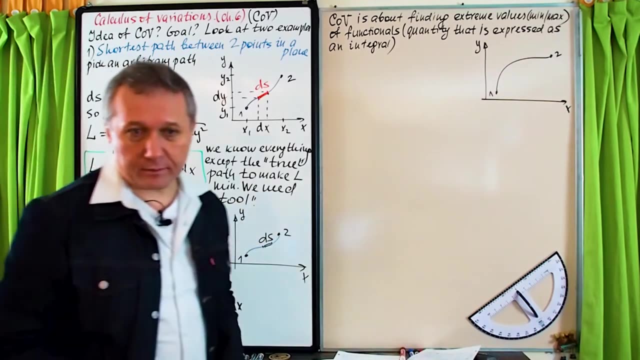 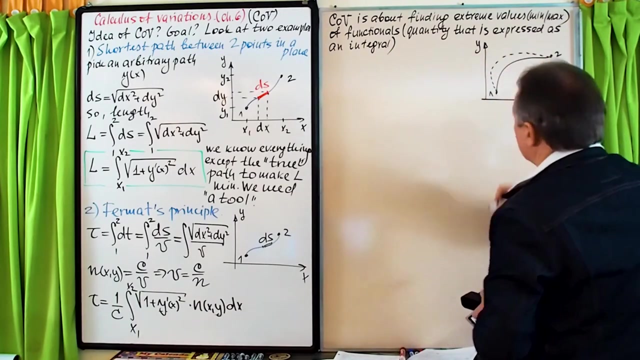 one and two. and so, uh, what does it mean? so you take an arbitrary path, for example this one, and you calculate it, let's say length or time, let's say you get some number, whatever five, then you will change this path, for example to this one, but again endpoints are the same because, according to your problem, you have initial. 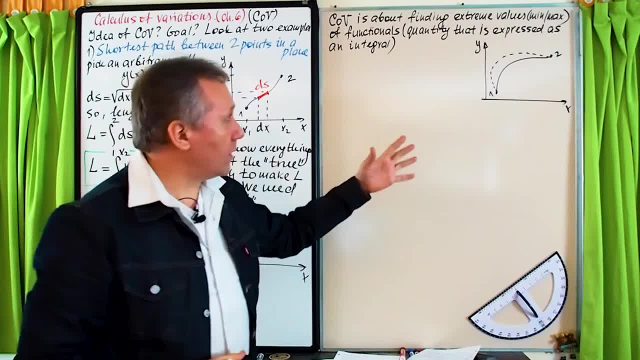 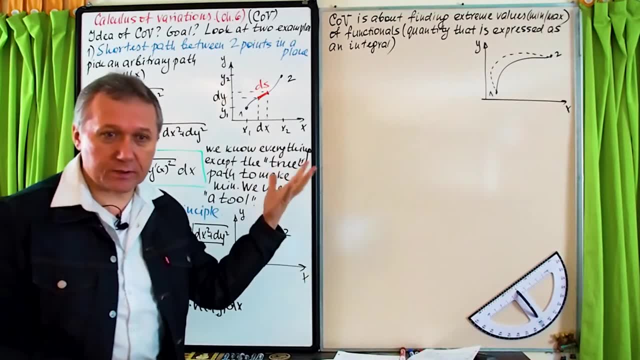 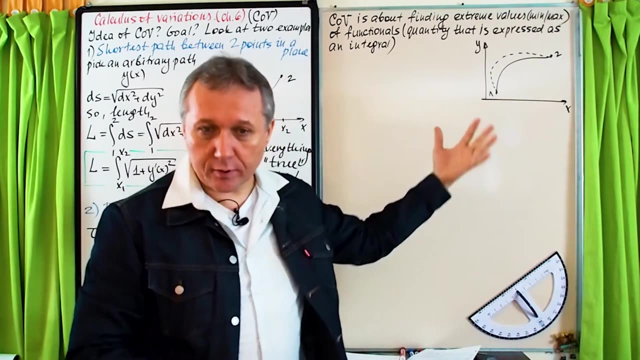 and the final point: right endpoints are fixed. you change, uh, you just change this path to this one and you calculate the value of the formula. let's say now, instead of five you got six. damn it, I'm getting. we're getting a lot, it's getting bigger. but let's say we want to minimize, so I'm moving in the wrong direction. so you change the. 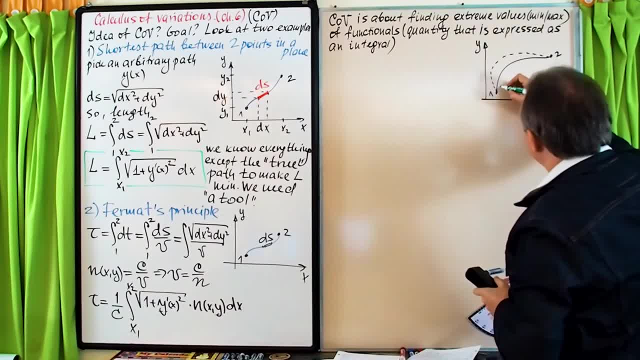 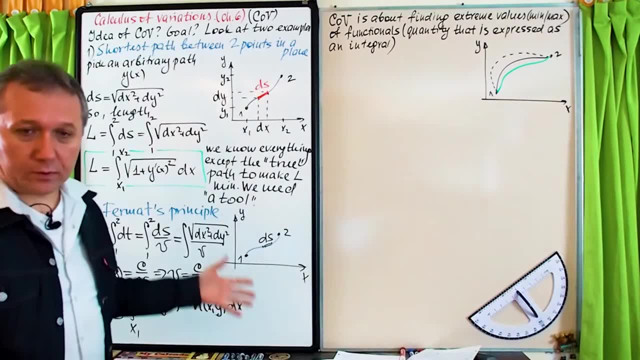 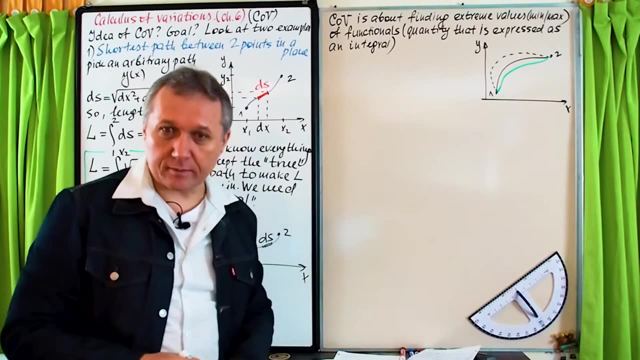 direction. and now you'll start looking, for example, you will change your path to this one. calculate l or tau at over that path and let's say you will get now three. okay, we're getting uh towards minimum, so it's better, right? so then, uh, you'll keep moving. now let's say you look at: 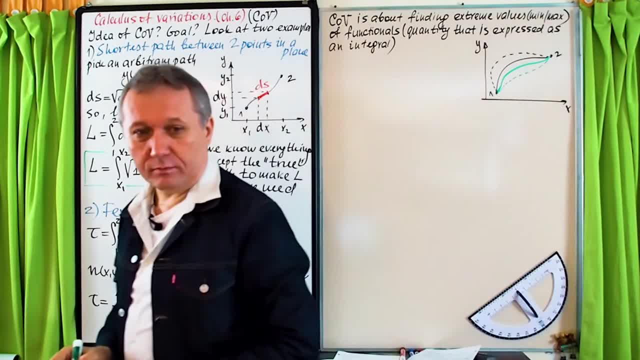 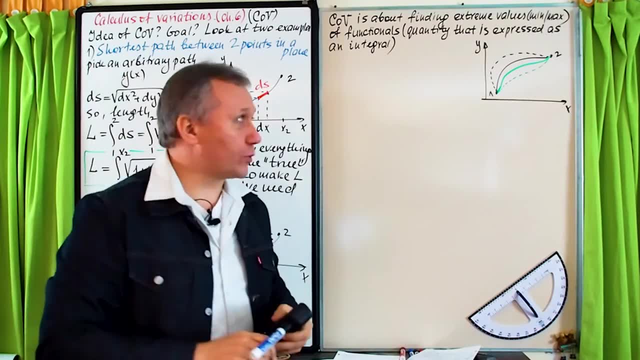 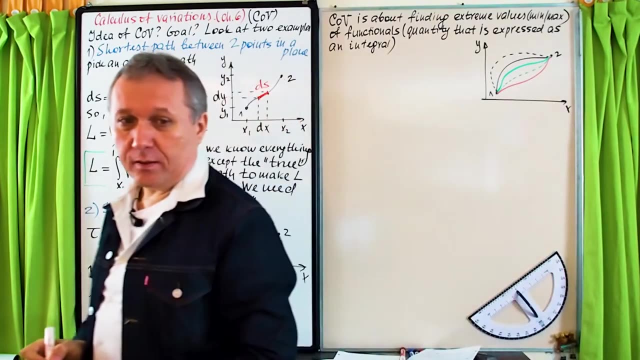 this path. let's say you got, I know one. okay, we're still decreasing, so it means you keep, you have to, you keep moving that way, so you keep probing and probing me. let's say at some point, let's say over this path, not some point, over some path, let's say you'll get, you got, I don't know. point two: 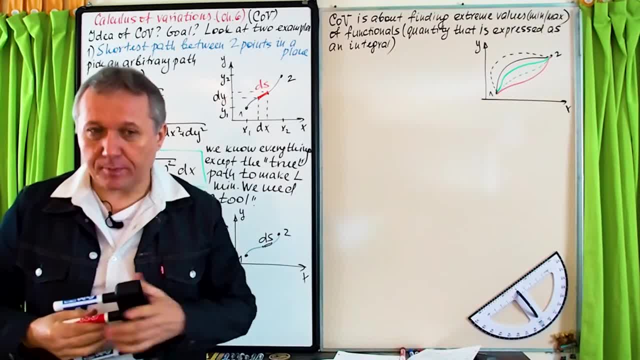 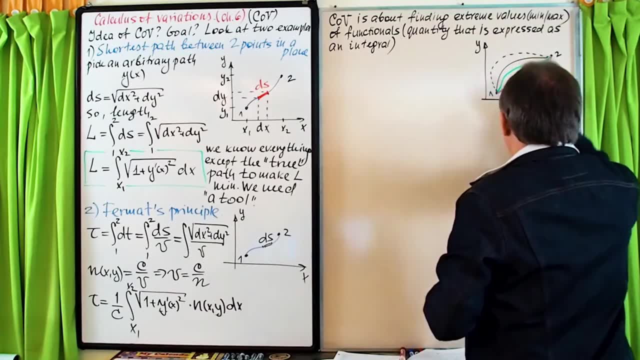 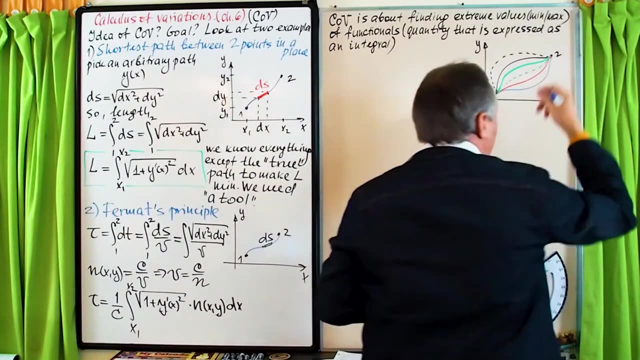 I'm just making it up, and if you pass that, if you pass this path, and uh, your value, the value of uh, l or tau, start increasing. so now let's say now, uh, here we had, um, I know, as I said, point two, and now the next path. 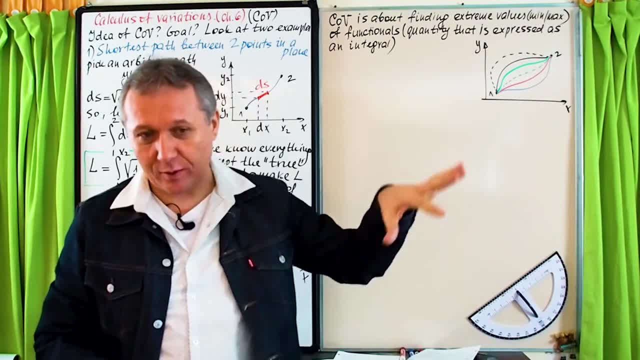 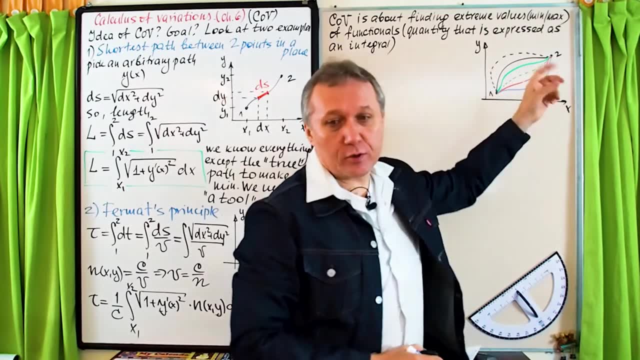 it will be, let's say, maybe 0.5, and you see, now the value of uh- functional- starts growing. so it means that this will be the true path which is going to minimize. so that tool which we're going to develop allows us sort of like 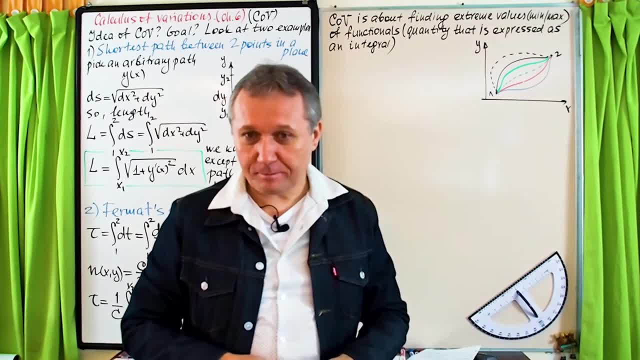 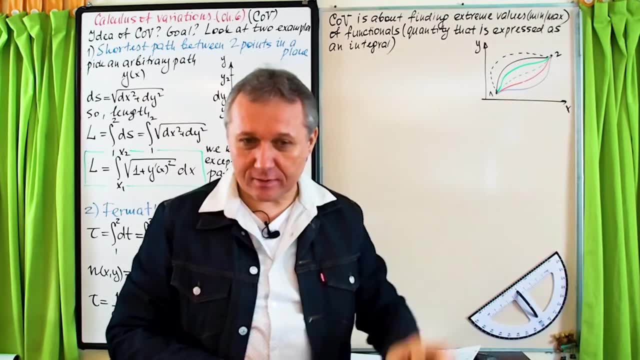 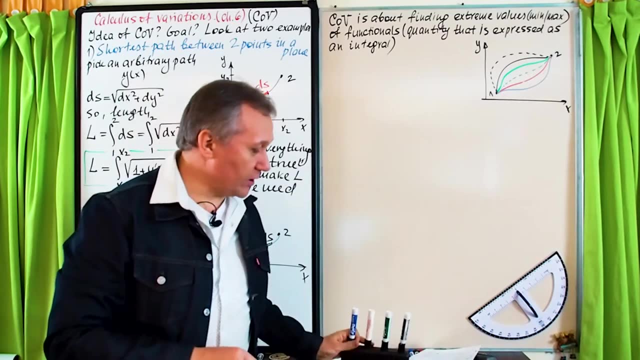 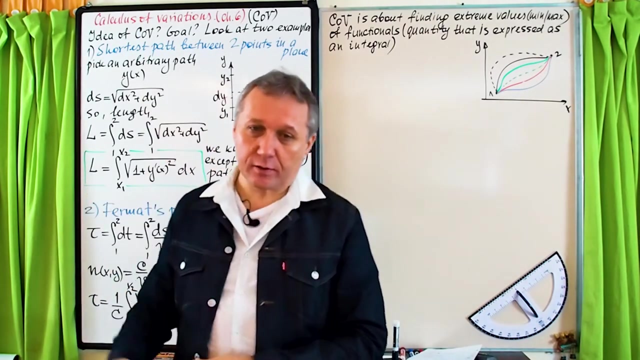 to uh change this path searching for the minimum right. so you move this way, okay, it's increasing. move this way: it's increasing again, okay, so this is seems to be like a minimum right. so that's what calculus operation does it? just uh change your path searching for the minimum value of uh functional, whatever functional. 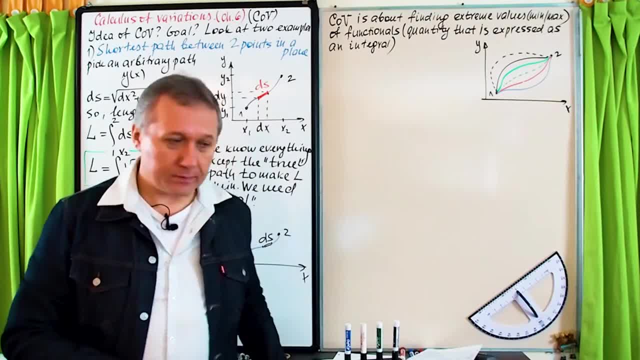 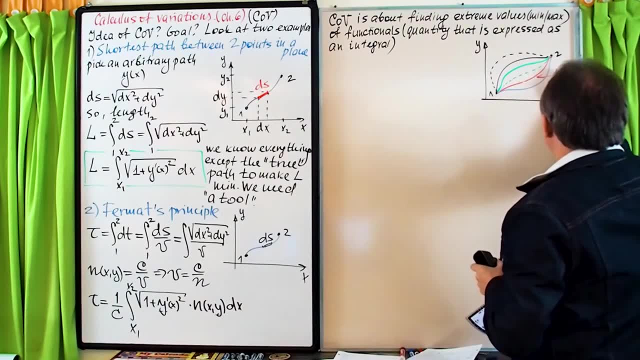 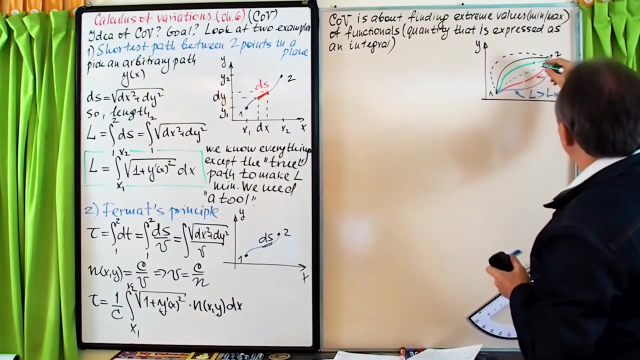 is in your uh problem, in your problem, right? okay, so let's let me show that. for example, this is: gives us l minimum and uh, this path. let's say it's a l larger than l minimum. then again, over here as well, I can say that l is larger than l. 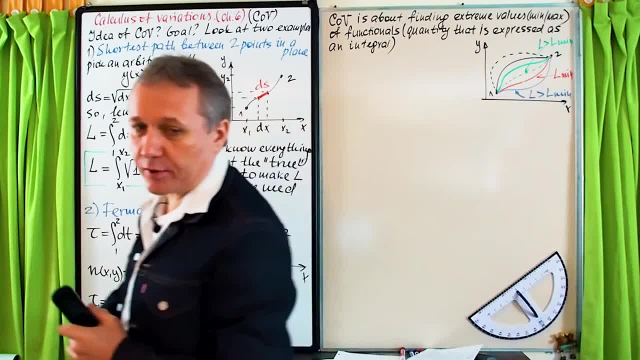 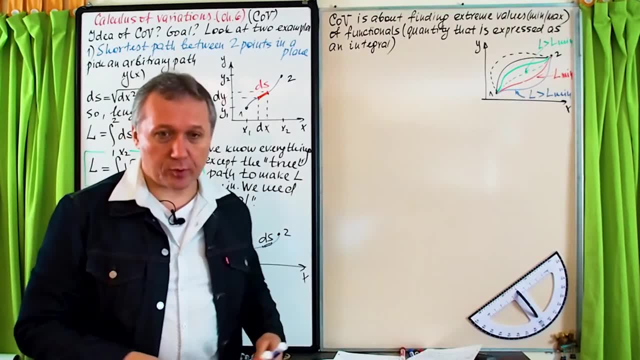 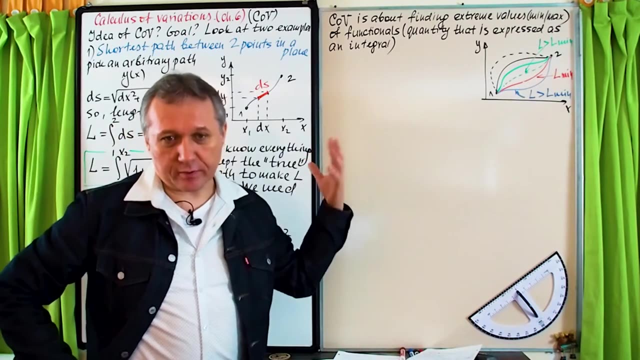 right. so I want to correct this by changing this. so l is larger than l. so that means l, which is less than l, or not l. and this path is larger than l, right. so l is larger than l. so l is larger than l, so it is a minimum, right. so that's what calculus of variations does. it allows you to find the path. 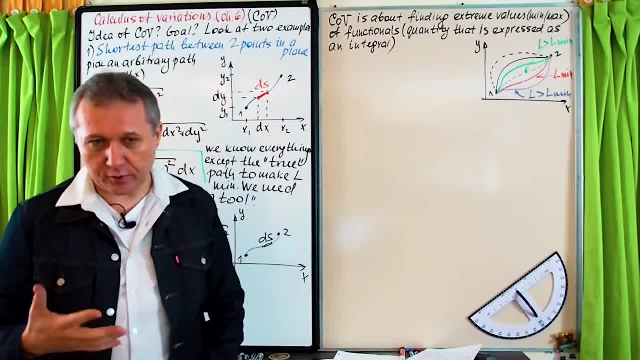 along which a certain functional functional view- problem uh- is minimum. but of course in general we will see when we start deriving that we can guarantee we will be able to guarantee not the minimum value but a stationary value, so it can be minimum and or maximum, but you will see in most of the actual. otherwise we will not see the actual value but it will be a stationary value, so it can be minimum or maximum, but you will see in the most of the actual. 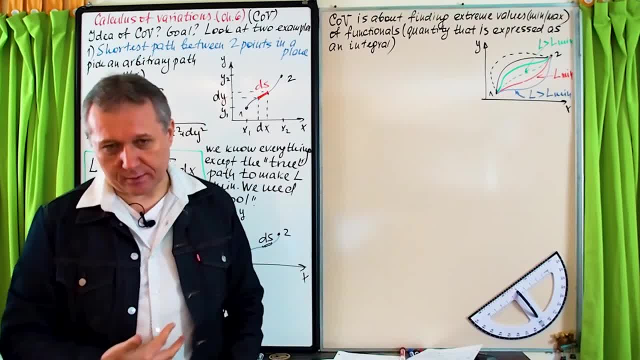 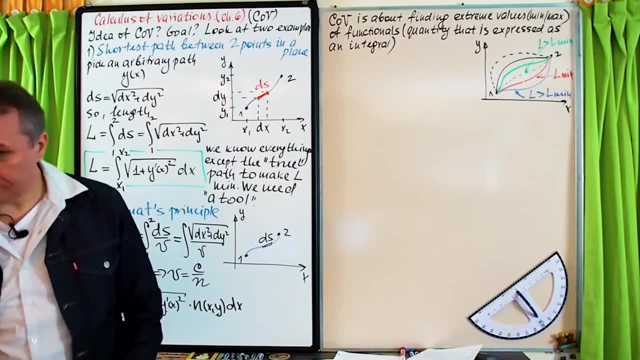 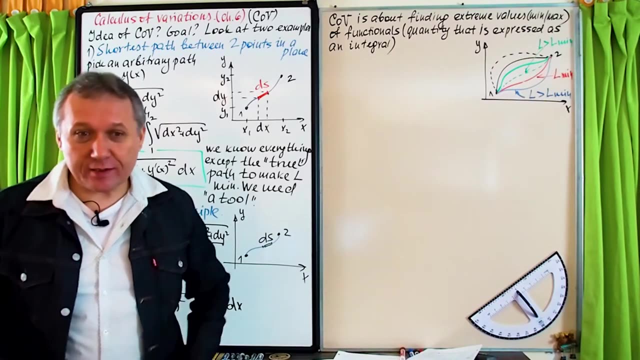 of our problems. all the time we will have to minimize, right, So we'll have to find the minimum value of something along a path, right So that's the introduction into the calculus of variations. So now I want to give a more or less clear picture. 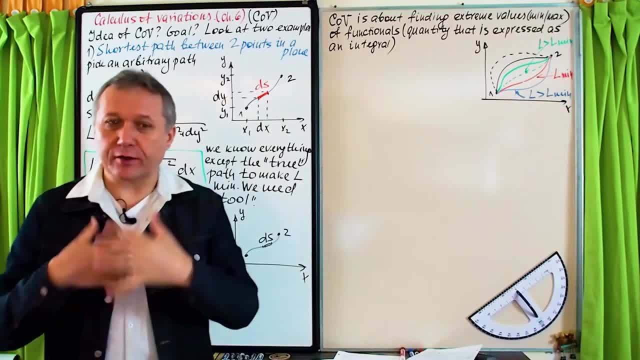 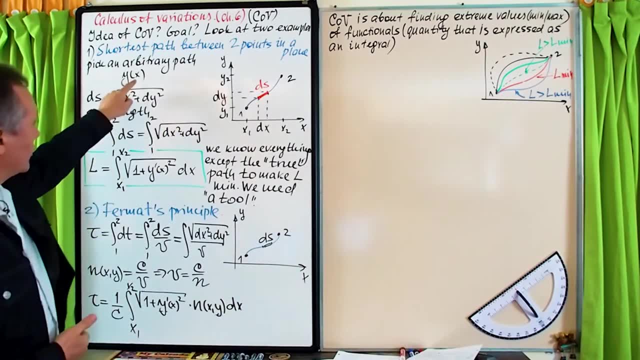 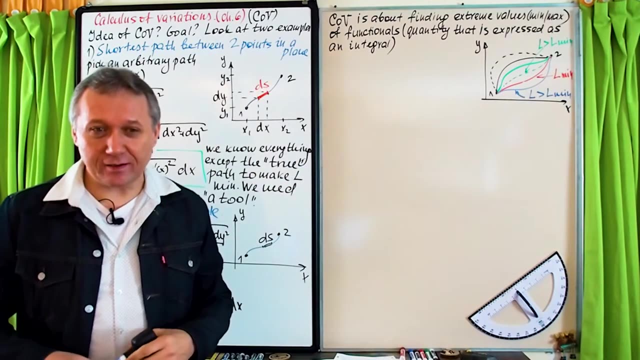 And oh, you should have a clear picture already. We just refreshed it right. And now let's derive. start deriving the tool right, which we need to find again the true path making this functional stationary. Okay, so the title. let's derive what is called the Euler-Lagrange equation. 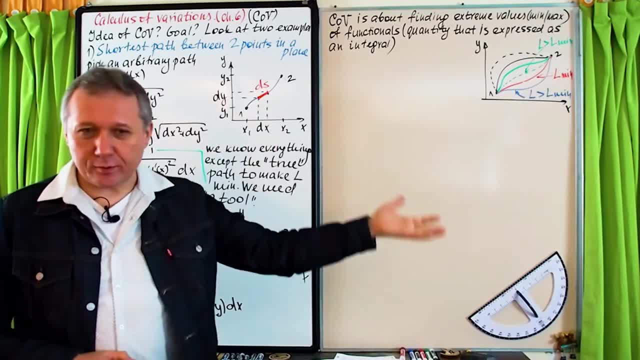 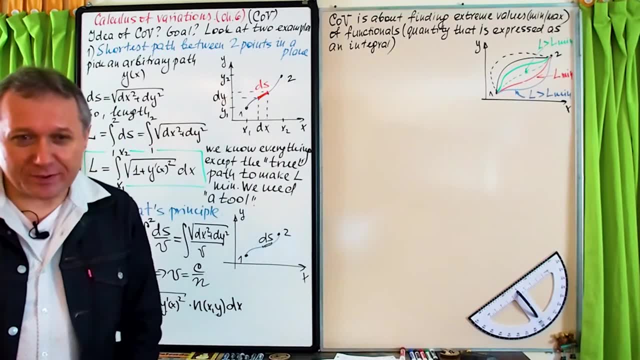 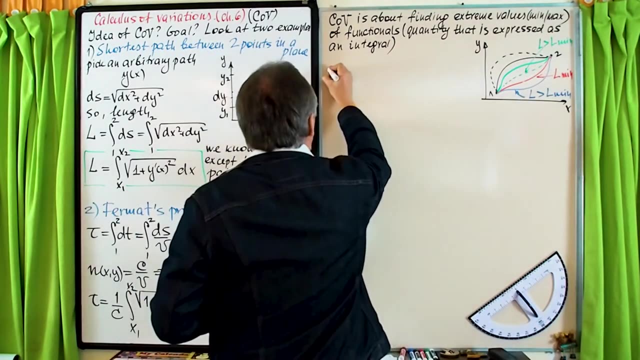 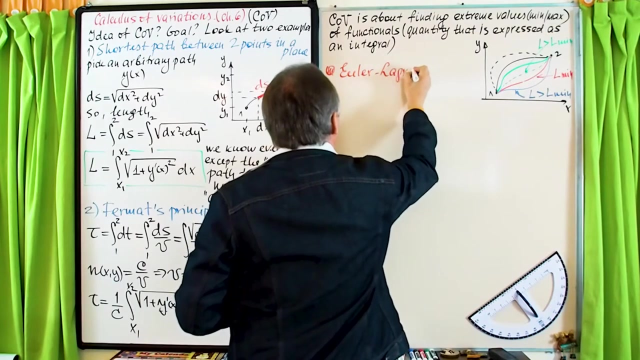 Different pronunciation of Euler right, Euler, Euler. I've heard different, I don't know which one is correct. I heard this pronunciation so I'm trying to use that. Okay, so now the title. Okay, I will put a new bullet and Euler-Lagrange equation. 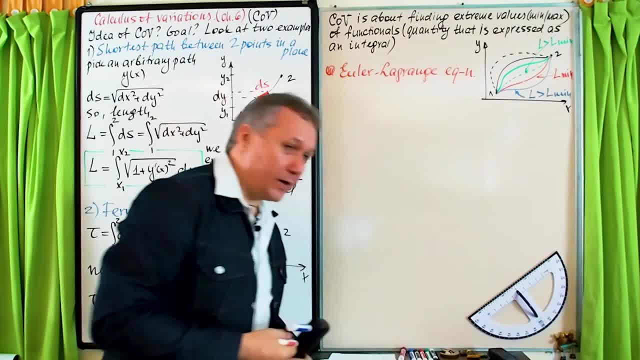 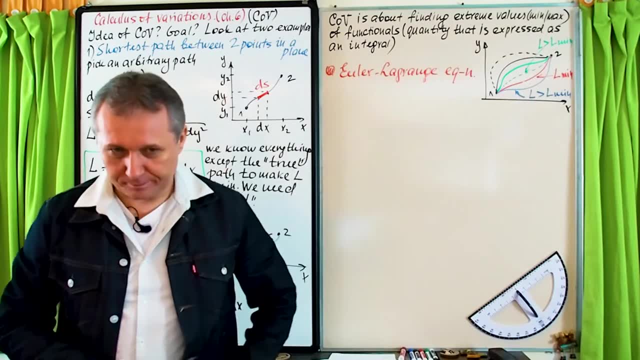 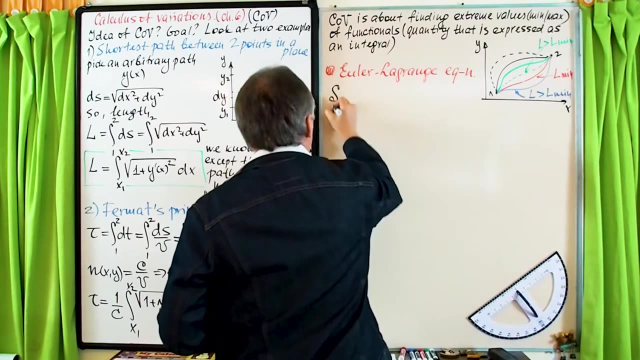 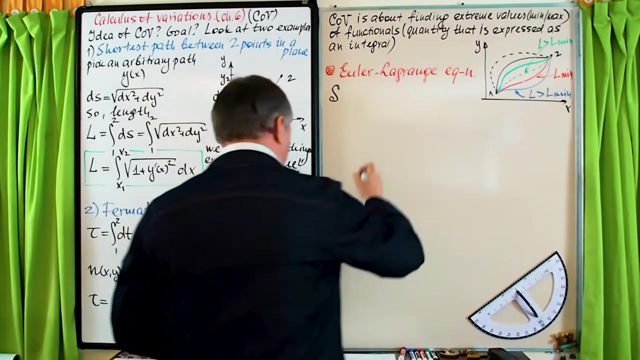 All right, Okay, so let's assume that we have a completely, just completely arbitrary functional. So let me write it So: S. so here we have L, here we have tau. Let's just call it in general S, which is a function of Y, and that is a function of X. 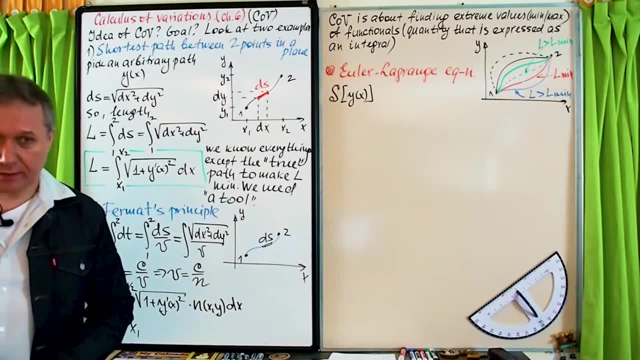 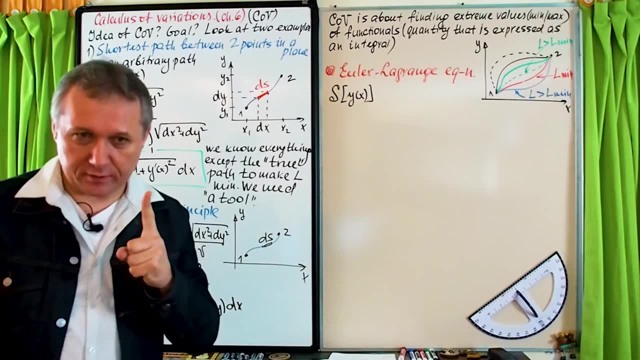 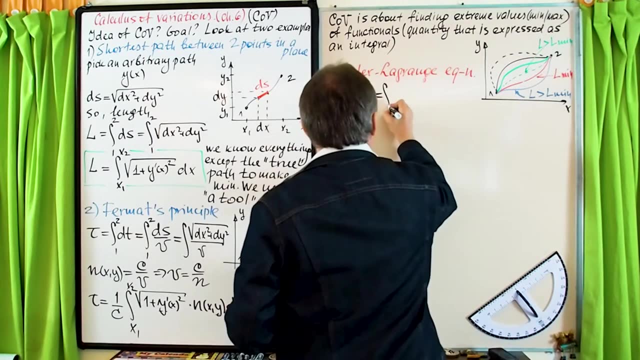 Again, the major difference between functionals and functions that are in a functional inputs are or in a functional Functionals. inputs are functions. Okay, let me write that Now. first let me complete the functional and then I will state that. 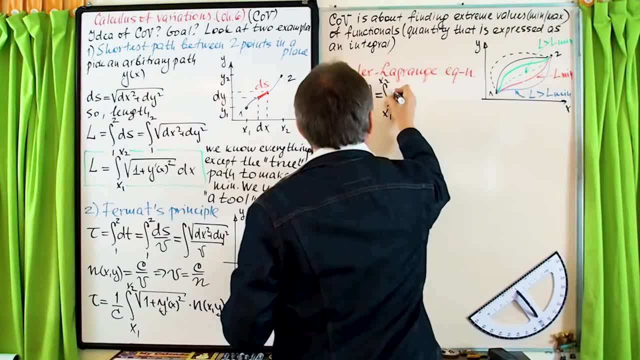 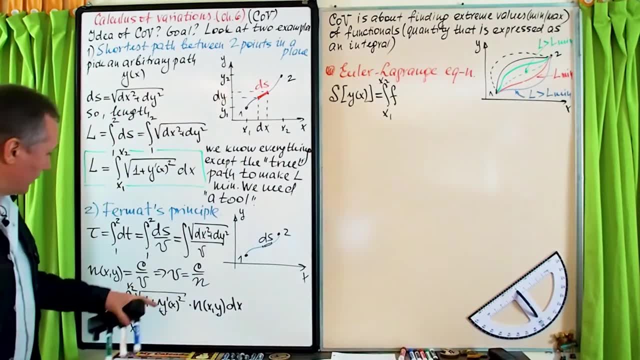 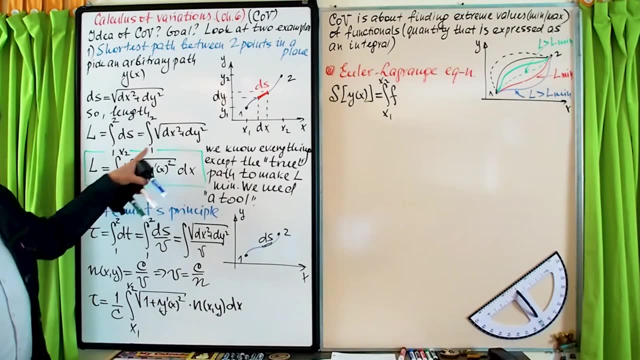 So integral, from some X1 to X2, and some integrand F, like in this case, F was this square root times N as a function of X and Y, so that is F. In this case, F is that square root. 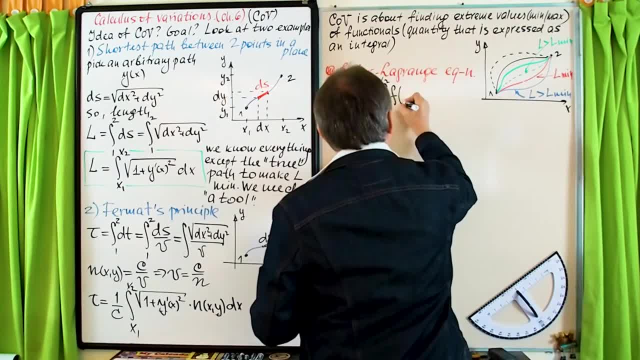 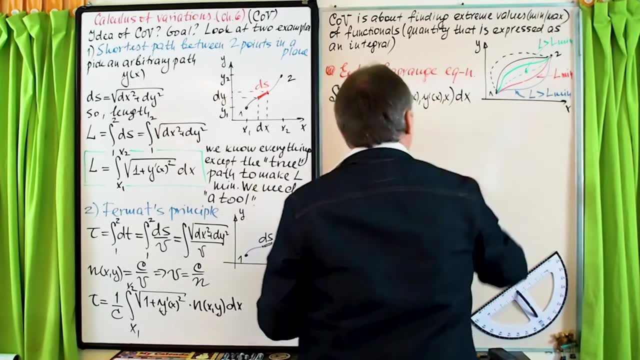 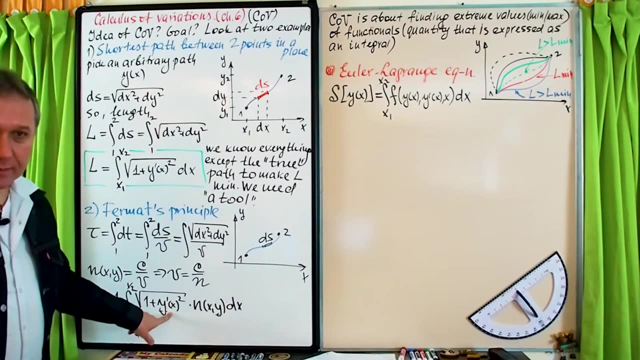 So some integrand which Can be a function of Y, Y prime, and X itself, the X. So you see, sometimes you can have Y primes, You can have Ys which are functions of X, and you can have X. 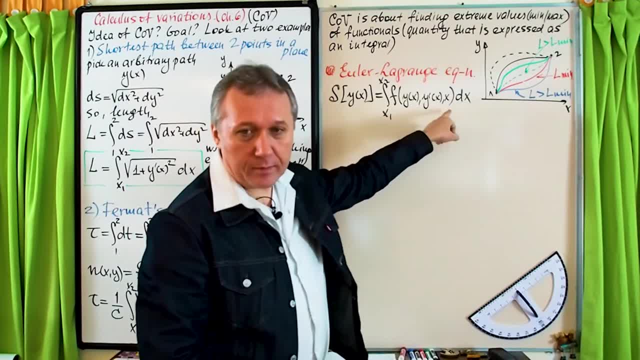 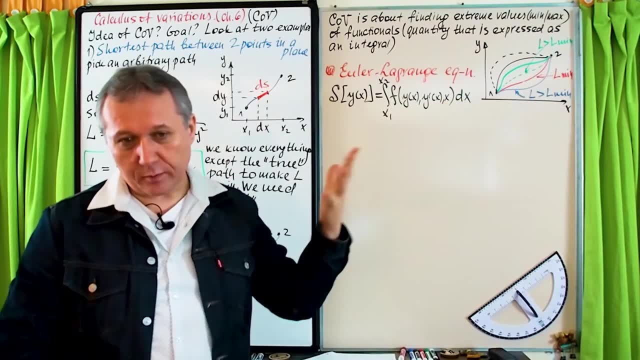 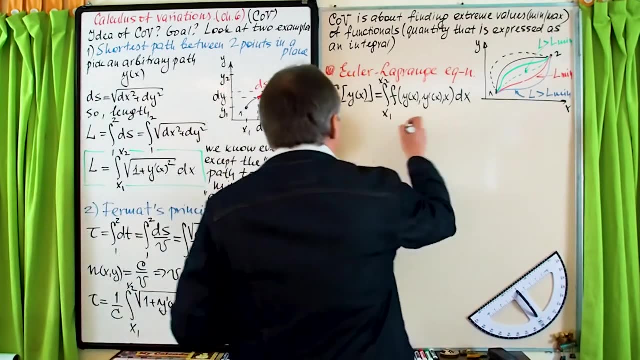 So I combine them all- Y, Y, prime X- And we assume that our variable of integration is X, Although we can have sometimes different variable of integrations. I will talk about that when we start looking at examples. Right, so that is a functional. 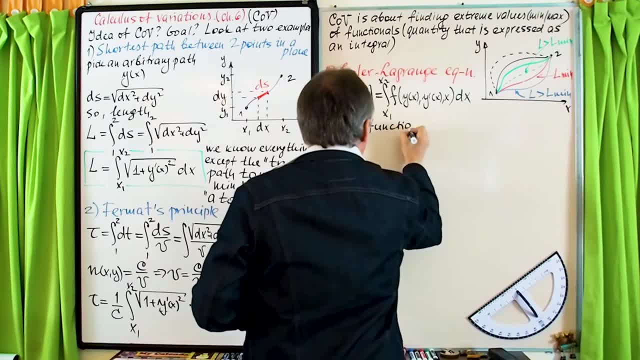 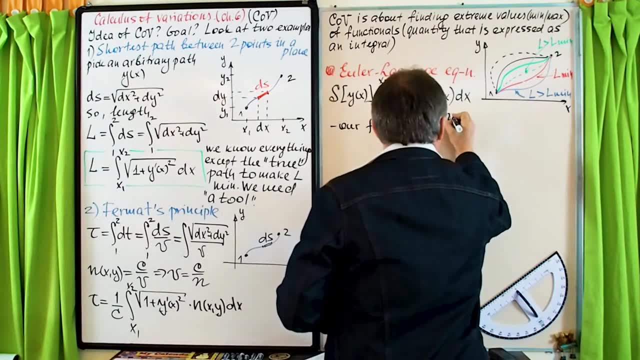 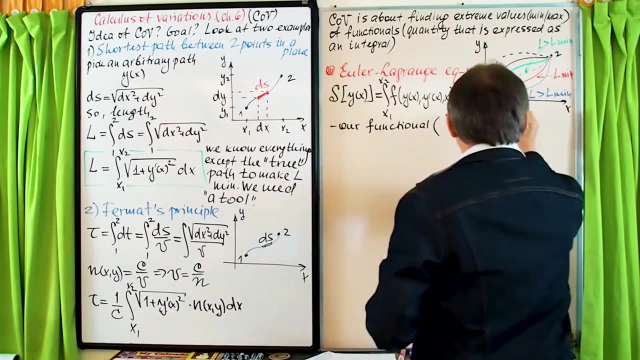 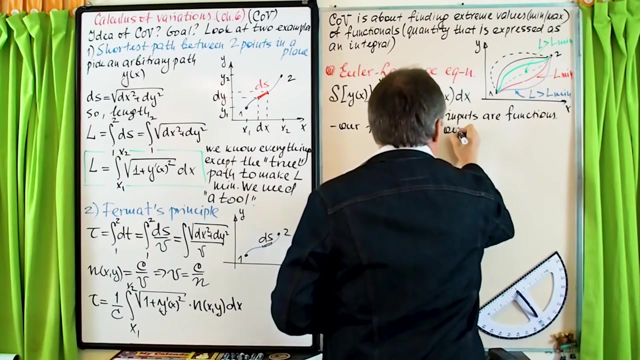 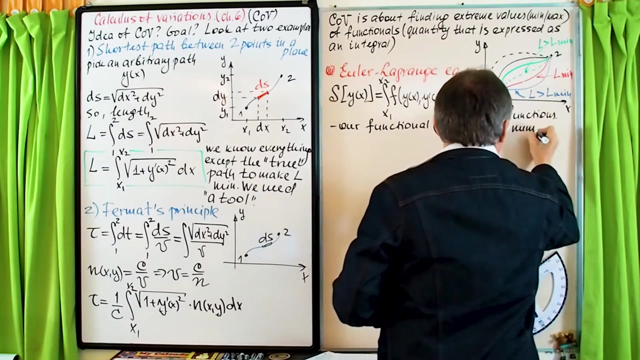 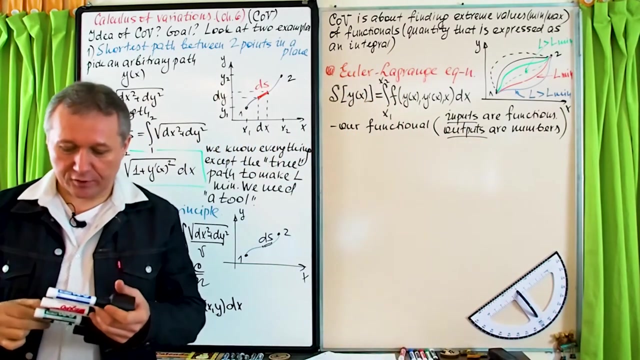 Our functional. And now I will emphasize that inputs are functions, output numbers. All right, inputs are numbers. Wait, inputs are functions, Outputs are numbers. So that is the major difference between function and functionals In a function: numbers in numbers out. 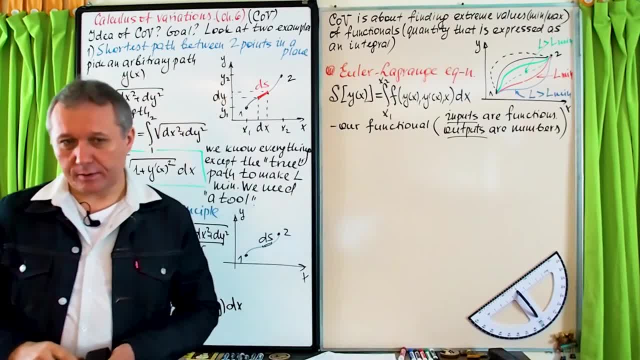 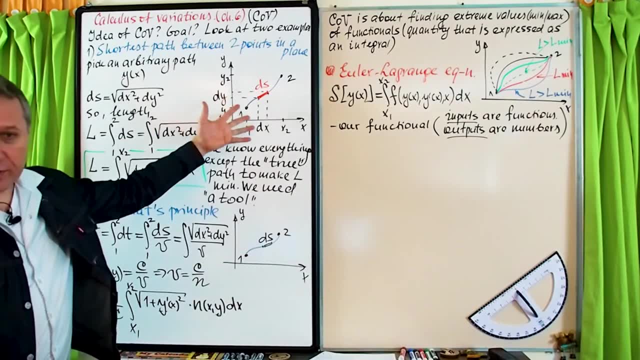 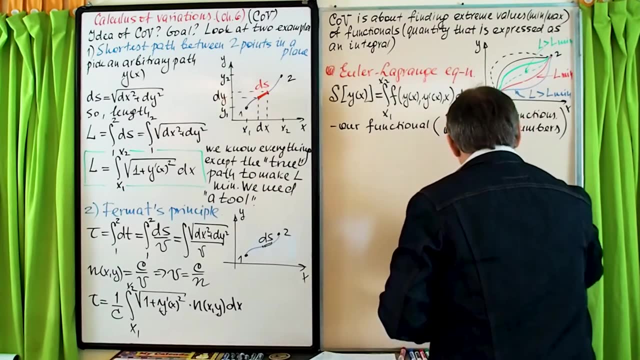 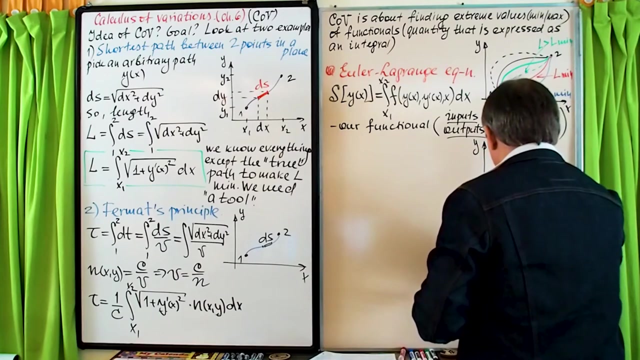 Here functions in a number is out. Okay so, and now let's imagine some completely arbitrary situations, Some initial point, final point, right? So let me draw it here. So Y, X, and let's say this is point one and this is point two. 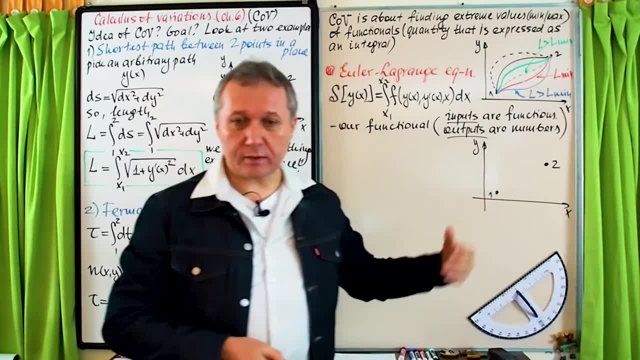 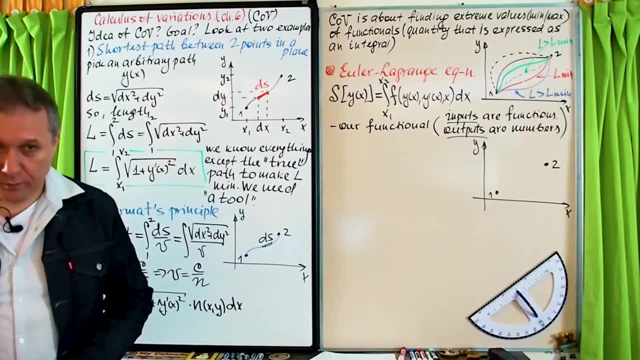 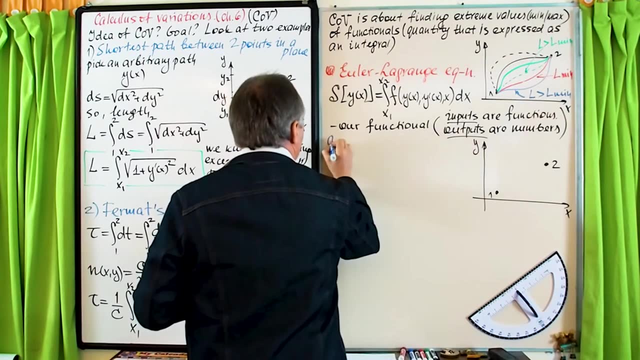 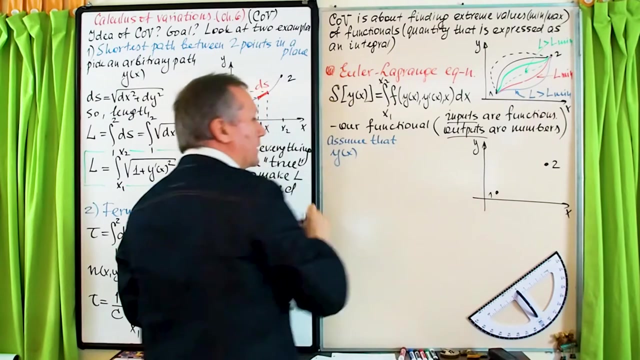 And again, and some functions, function is given on this in this space. All right, two-dimensional space in this case. So now let's assume- Okay, I will write, assume, let me use. So let's assume that Y as a function of X is the true path. 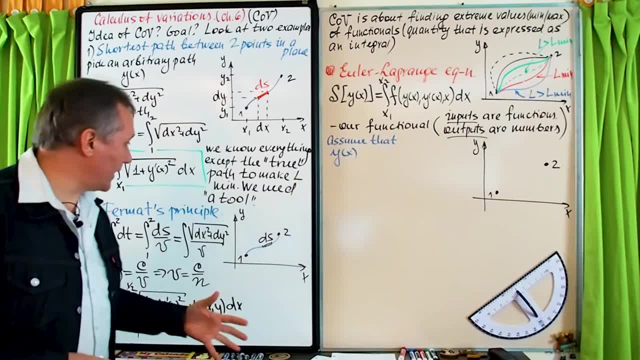 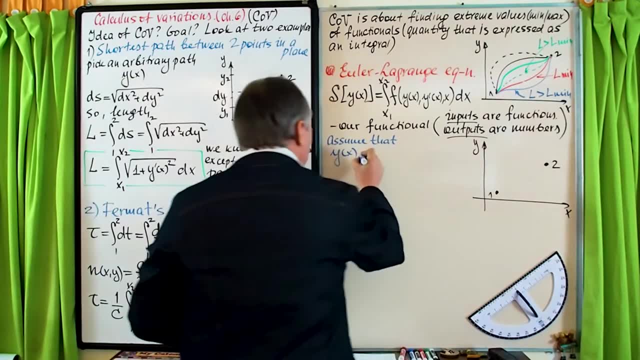 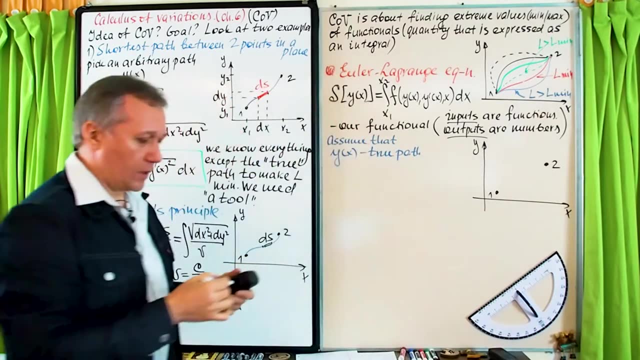 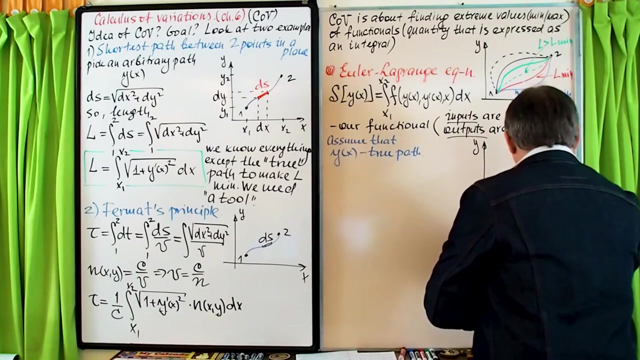 Let's assume that we know Y as a function of X is the true path which is going to minimize Our functional S right is the true path. Okay, let me draw this true path using the red color right. So that is Y as a function of X true path. 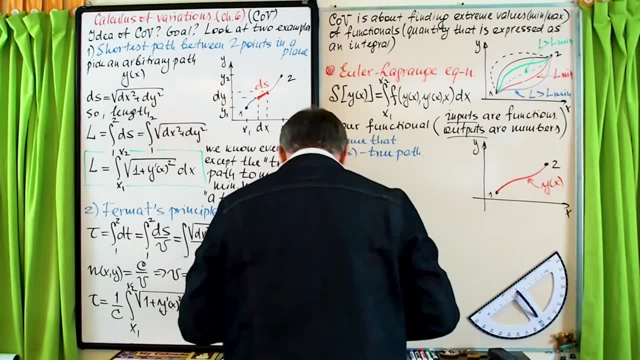 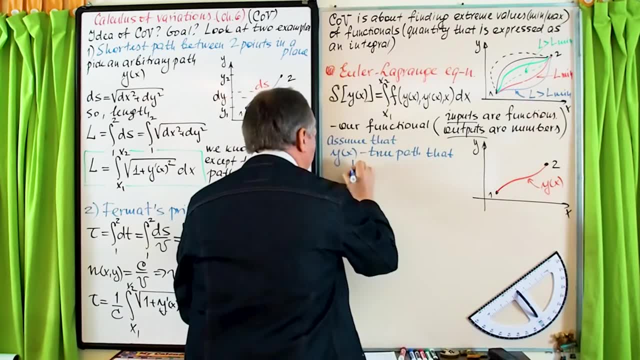 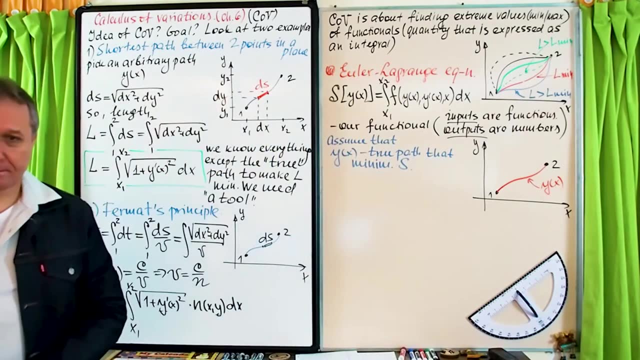 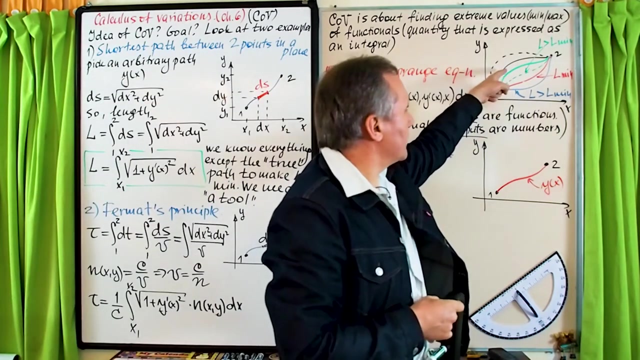 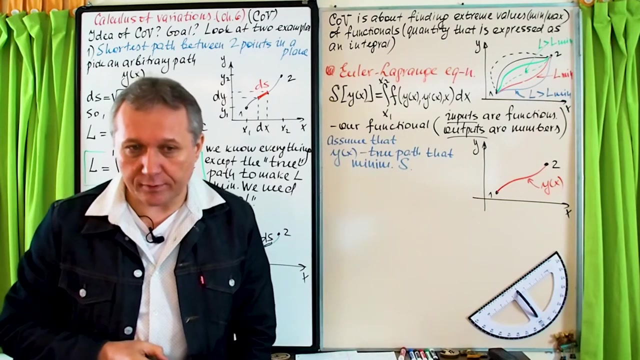 All right, Let me maybe emphasize the true path That minimizes, minimizes, minimizes, S. Okay, now let's construct a variation. Basically, this, this path, basically this path, are variations of the true one. So now let's construct a variation, or we can call it a wrong path. 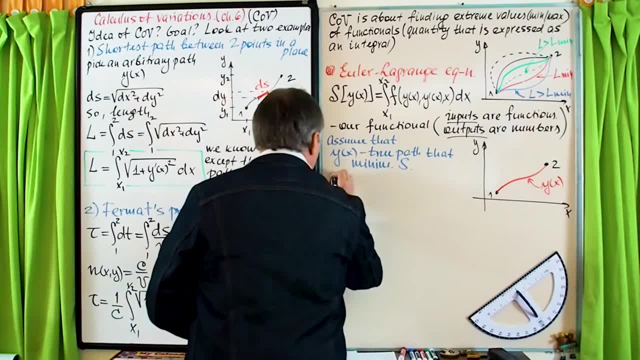 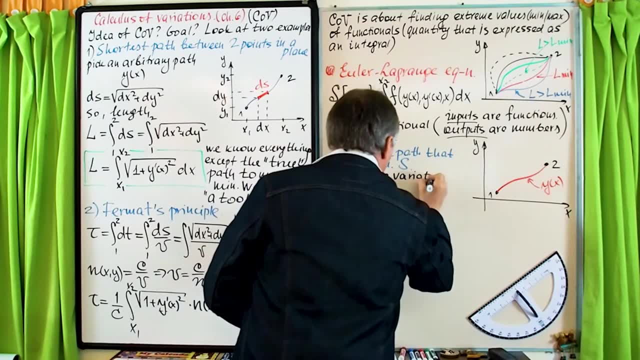 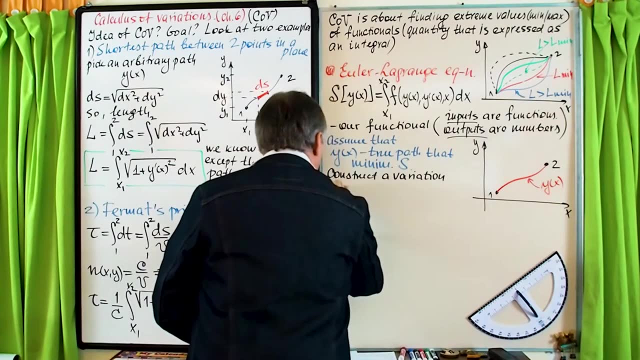 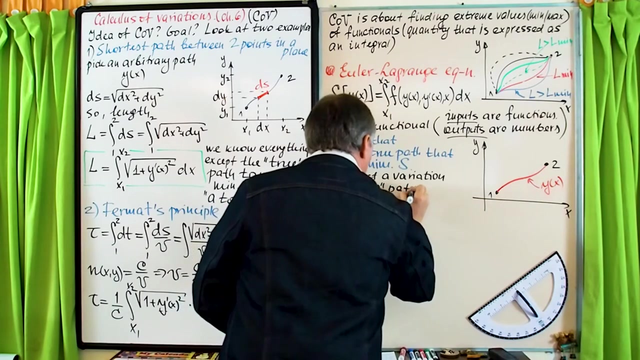 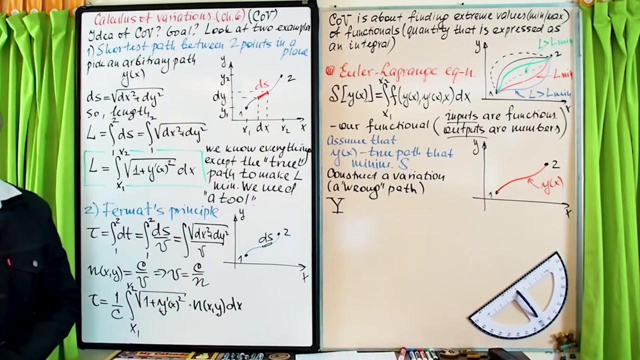 Now Let's construct a variation. A variation, That's why it's called calculus of variation. Let's construct a variation, Basically a wrong path. And let me call it: Y capital Still is a function of X, Right, It's just a wrong path. 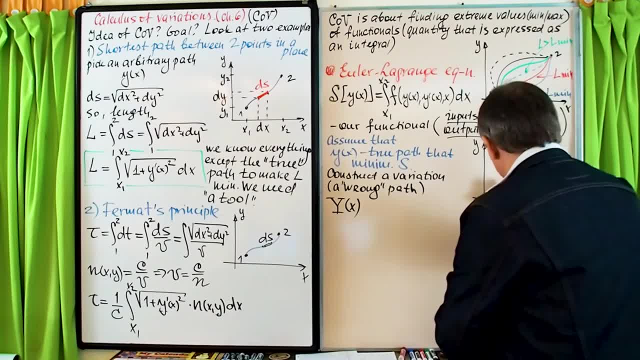 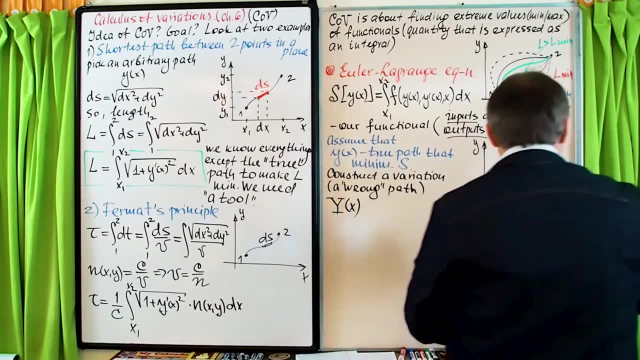 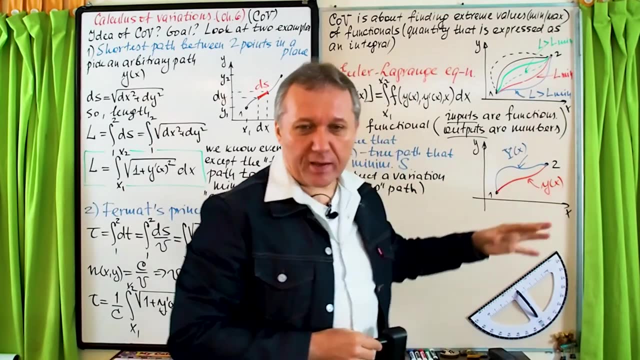 Okay, let me use some blue color, for example. Right, So this is our wrong path. Y, capital is a function of X, And we are going to construct it in this way. We are going to distort the true path just slightly. 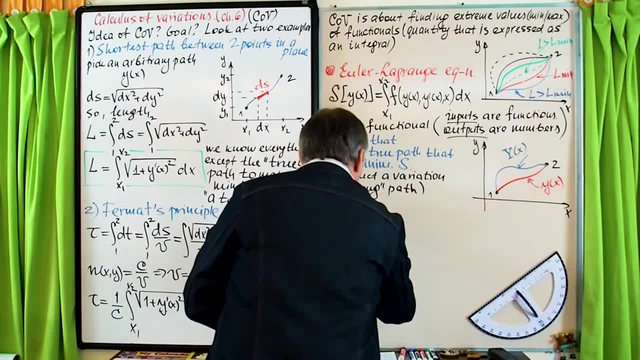 Right, So we are going to construct it in this way. Okay, So we are going to take the truth. We are going to construct it in this way. So we are going to take the true path. Again, it's basically a variation of the true path. 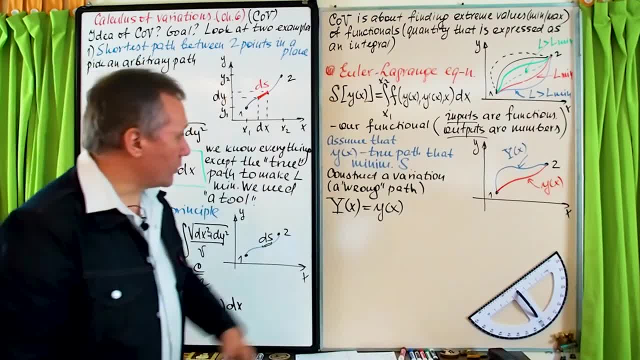 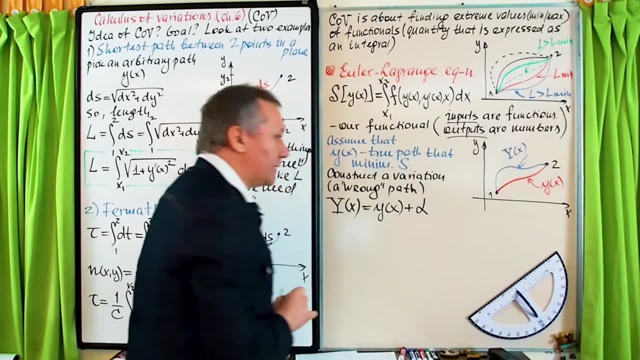 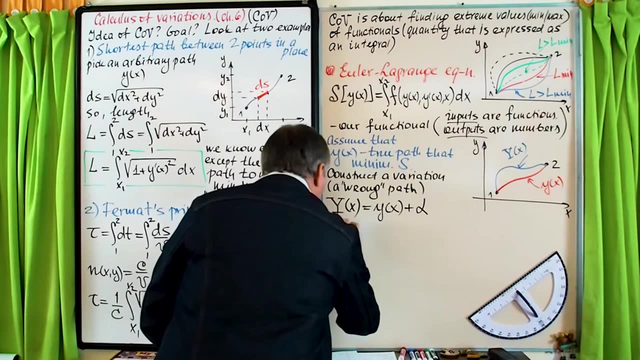 Slightly change it, Slightly distort it. So the true path, right Here And plus, since, as I said, we want to distort it slightly. so let me introduce a small parameter: alpha, Real Right. Alpha is the real and small parameter. 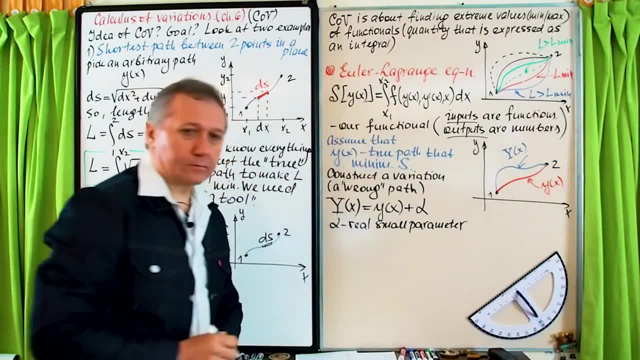 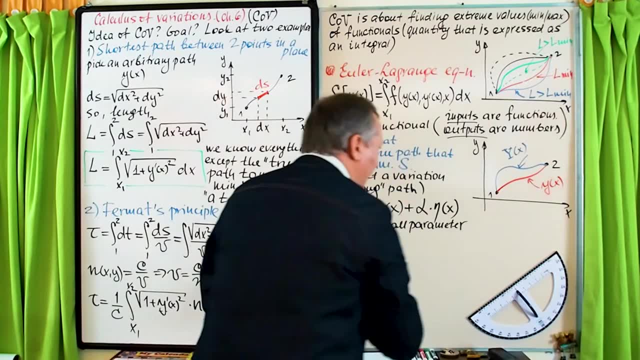 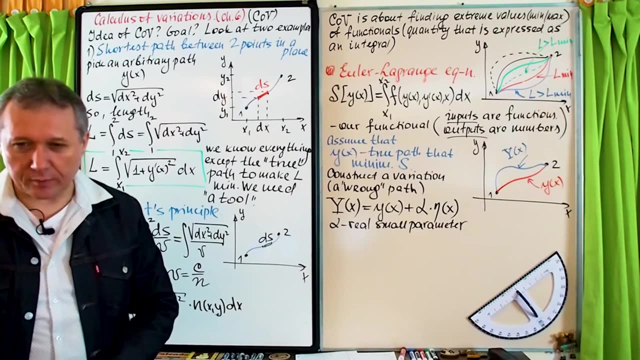 And let's multiply this small parameter by an arbitrary function, eta. It can be any but well-behaved function. What does it mean well-behaved? It means that, yeah, it's continuous and you can differentiate it as many times as you want. 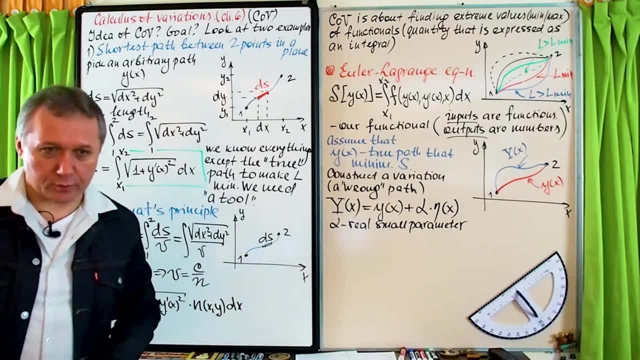 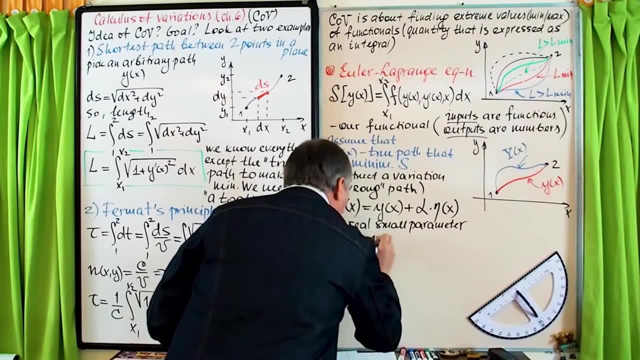 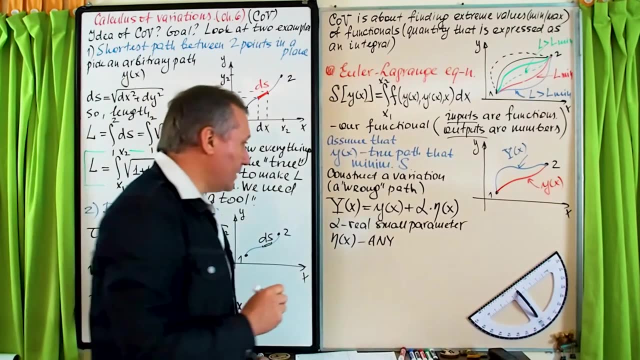 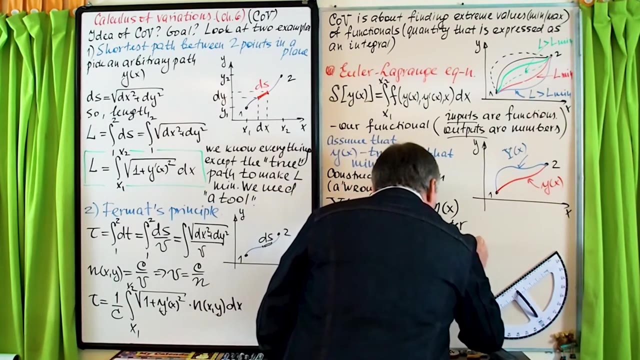 So well-behaved, good-looking, so whatever adjectives you want to use, So eta of x, eta of x, and I will emphasize any- It's a key word- any. You will see at some point why Any well-behaved function, well-behaved function. 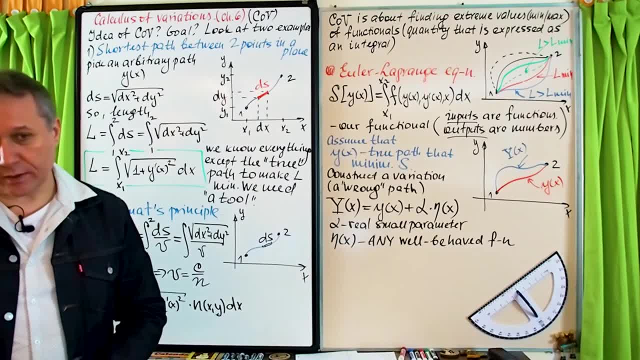 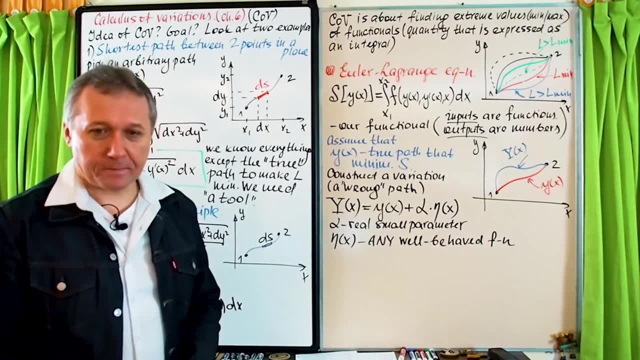 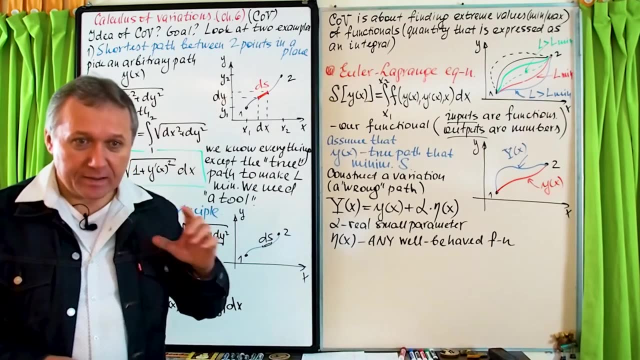 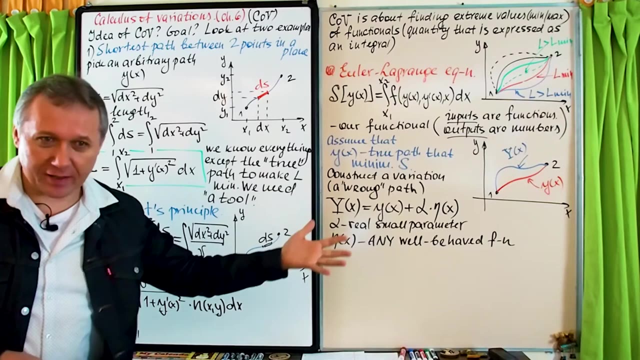 Again, it means that it's continuous and you can differentiate it as many times as you want. Okay, what else do we have to impose on our function? eta? Very important. It doesn't matter, like in all these examples, which path you take: wrong, correct, true, right. 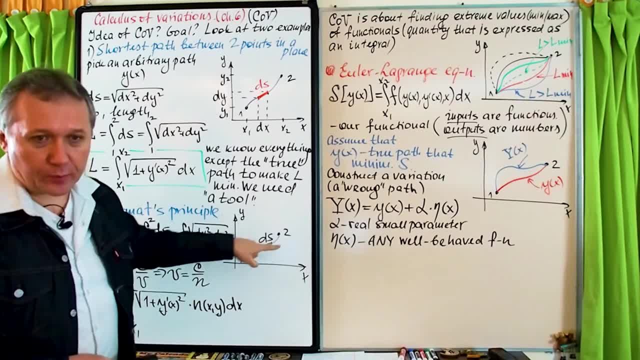 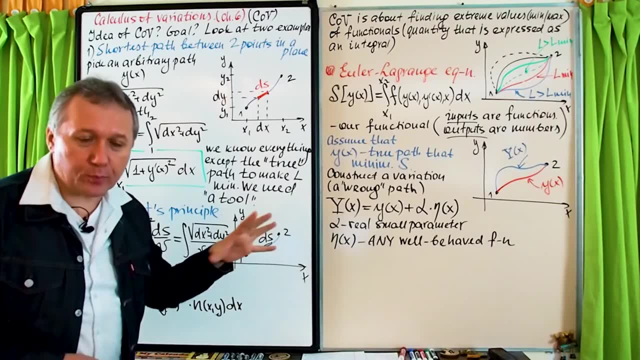 Every time, all paths go through the endpoints, Because you know, in your problem, you want to be here and you want to be there. The endpoints, The endpoints are fixed. You cannot change them because in that case you change the problem. 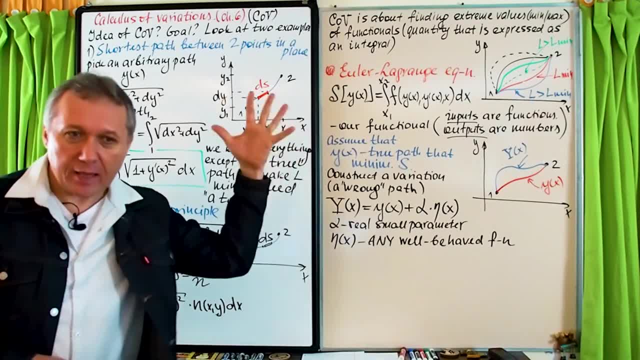 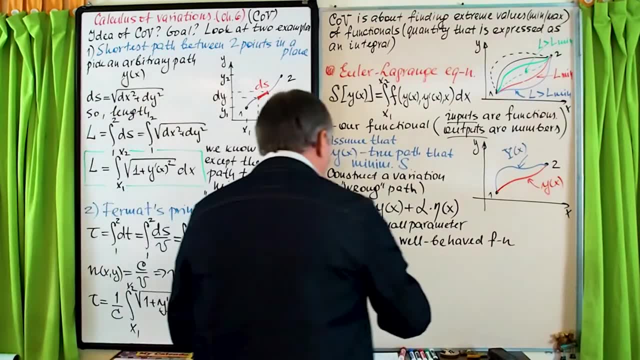 You want to solve a particular problem. so it means that endpoints are fixed, Otherwise it will be a different problem, right? So endpoints are fixed. Okay, as a result, so it means that y capital at endpoints. Okay, let me write. 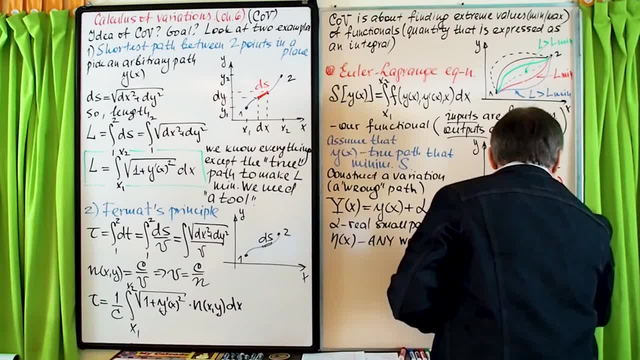 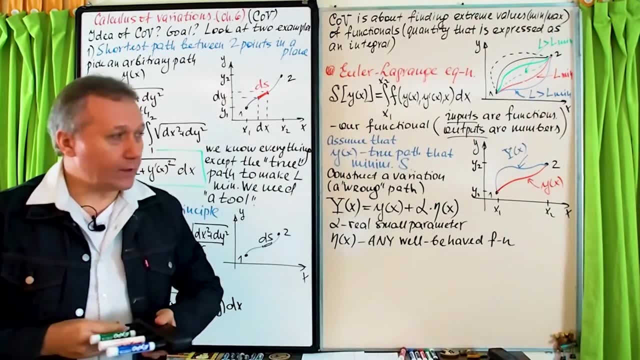 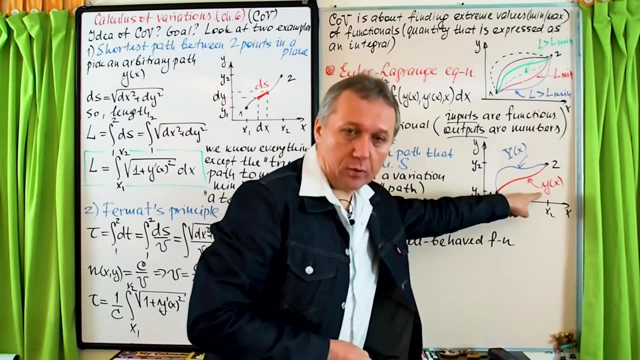 So this is x1, and this is x2.. This is y1.. This is y2.. So the value of y at y capital at x1 must be equal to the value of y small at x1, because they meet at that point. 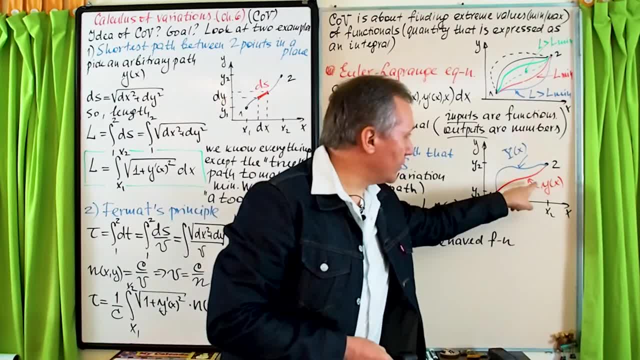 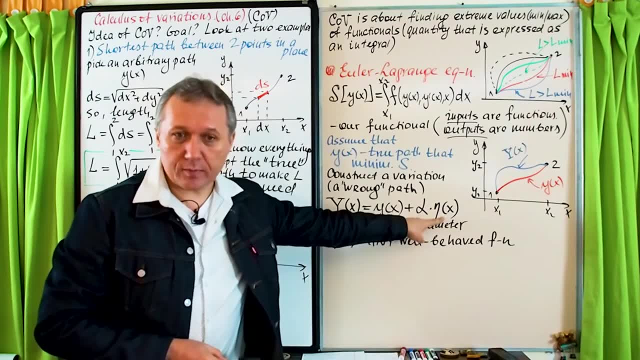 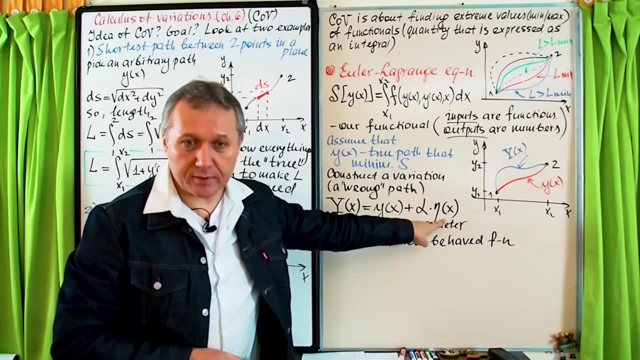 And also at that point, y capital at x2 must be equal to y small at x2.. So in order to make that happen, so eta at the endpoints must be equal to zero right. So value of function eta must be zero. 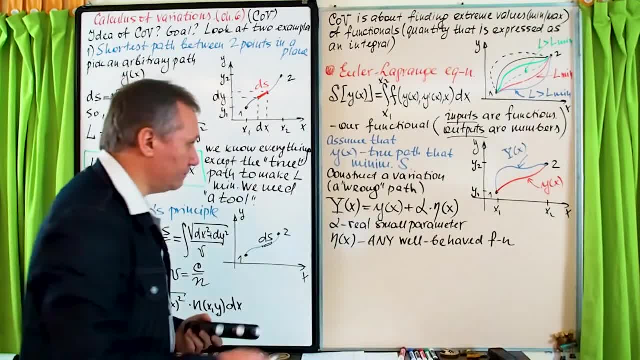 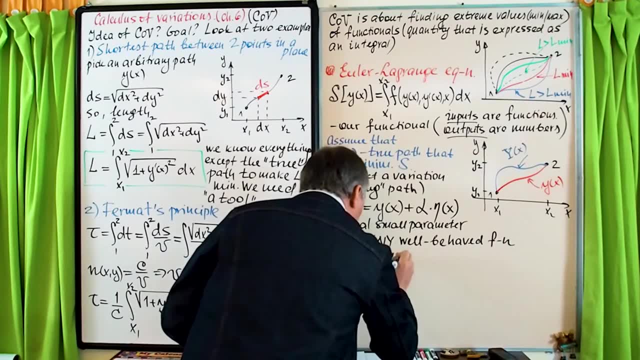 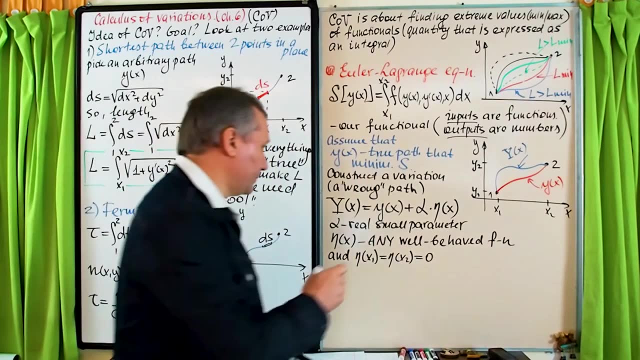 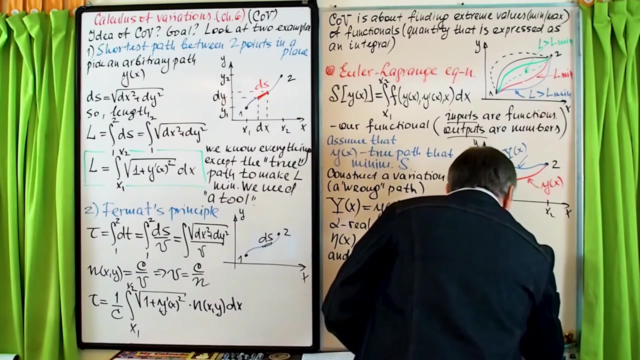 At the endpoints. We have to demand that, And eta at x1 equals to, eta at x2 equals zero. All paths must go through the endpoints. All paths must go through the endpoints. Endpoints, They are fixed, Endpoints are fixed. 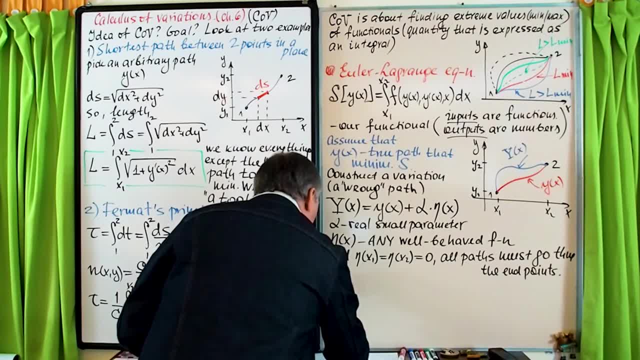 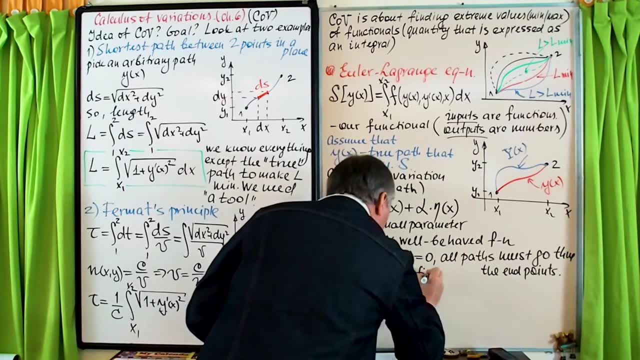 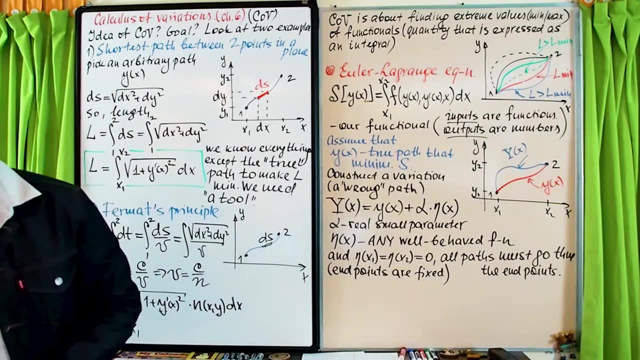 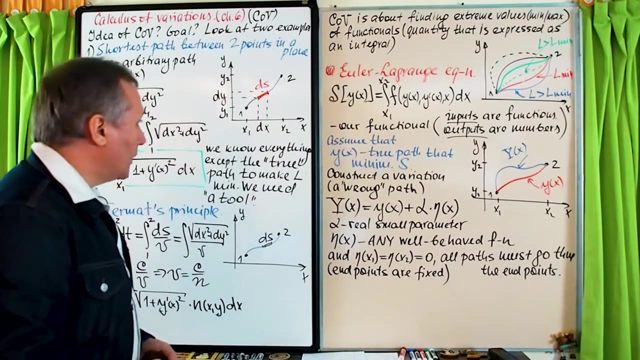 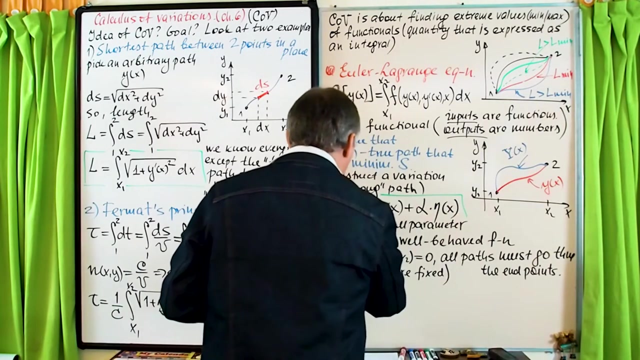 Okay, maybe I will write So endpoints are fixed, As I said, otherwise it will be a different problem. All right, Okay, so these are preliminary steps. Since I will use it from time to time, let me frame it so that it will be easier for me to spot it. 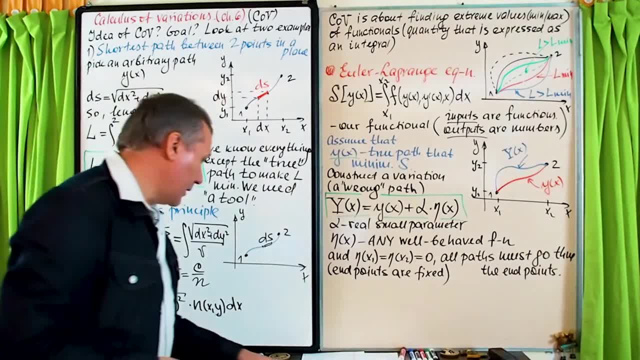 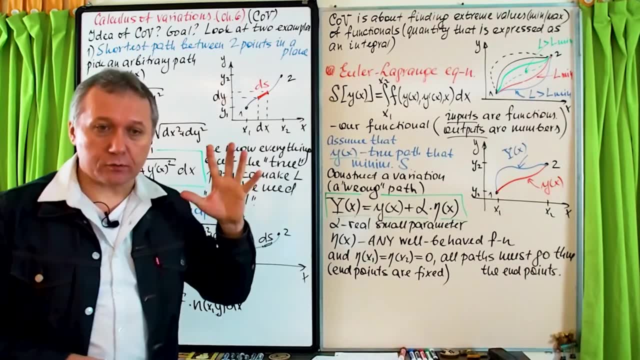 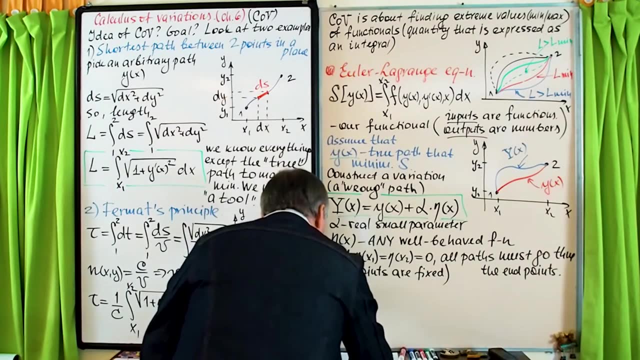 This is the true path, right? Okay? so these are our introduction, And now let's evaluate our functional at the wrong path, Why not, Right? So? So I will basically now this sort of like: stating the problem and now let's start massaging it. 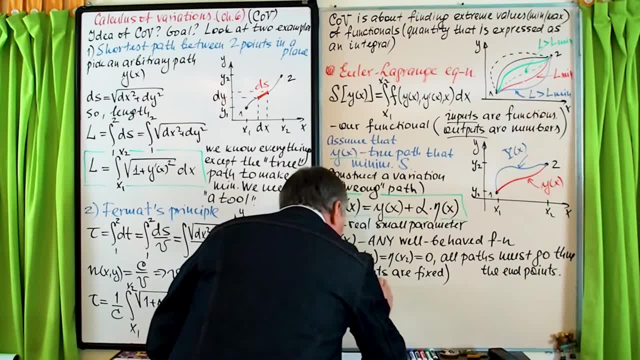 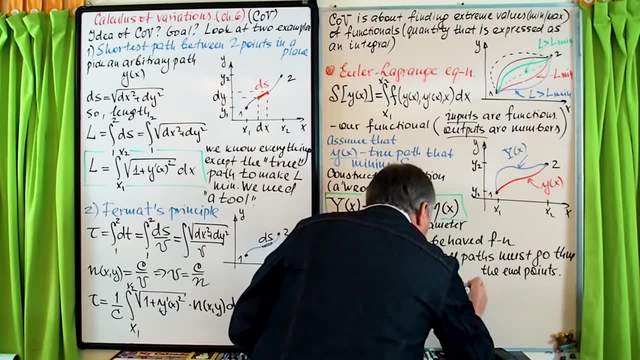 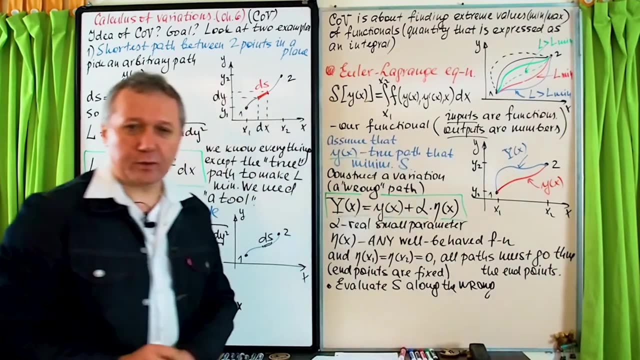 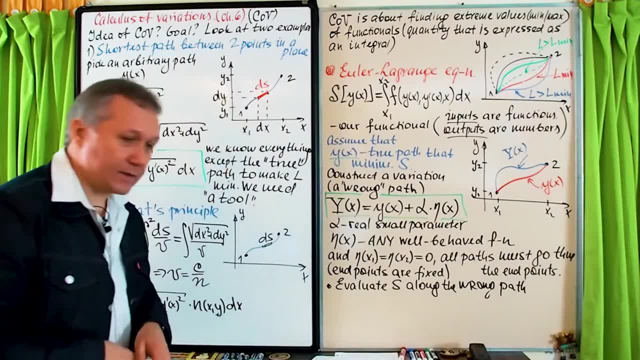 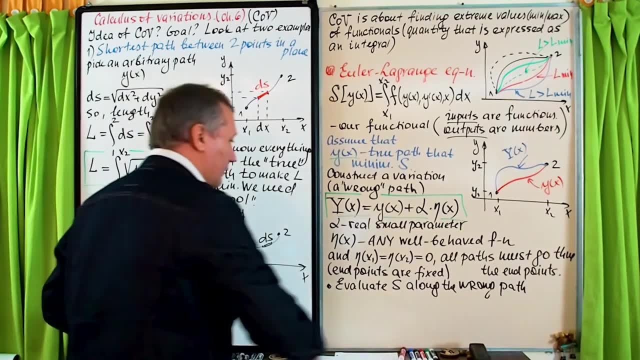 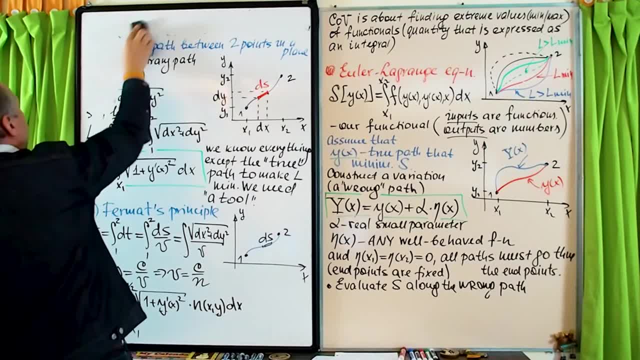 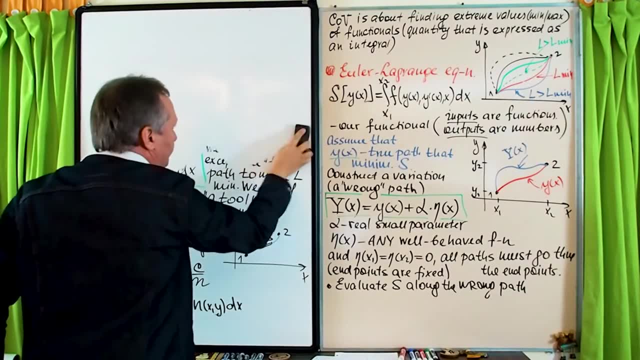 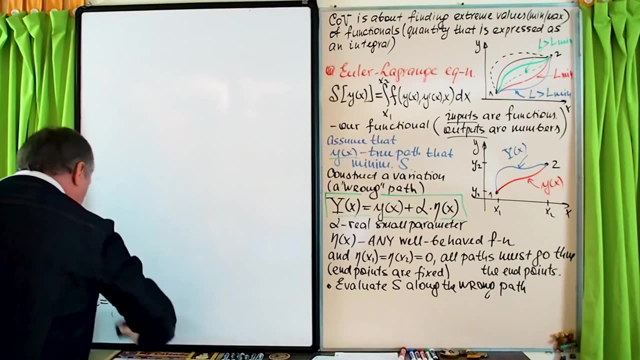 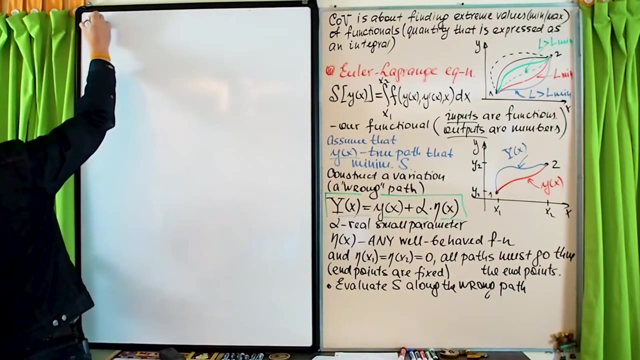 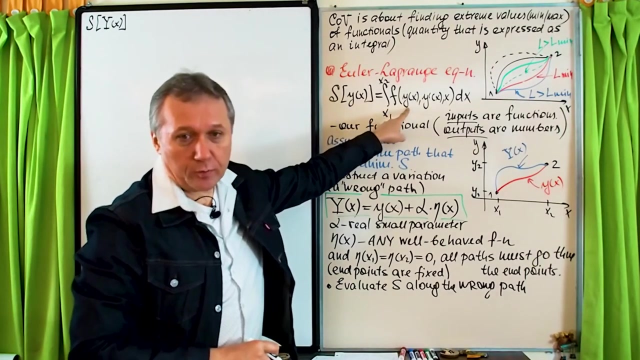 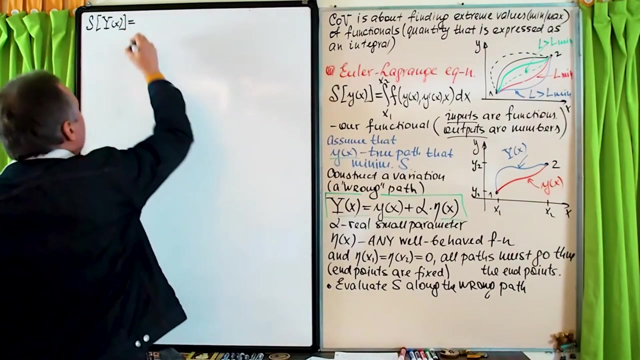 Okay, we'll see, So evaluate. So it means that S evaluated along the wrong path. So Y capital, So it will be integral. but now instead of Y small, we have Y capitals, Right, So integral from X1 to X2.. 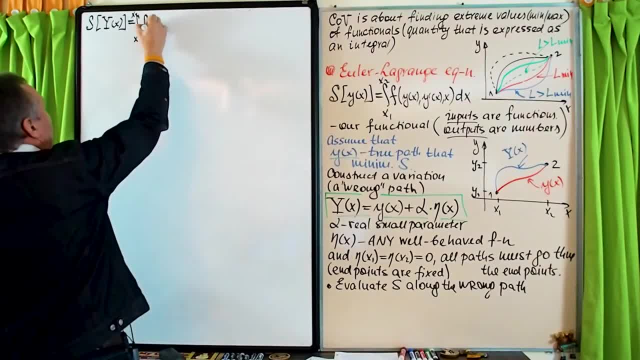 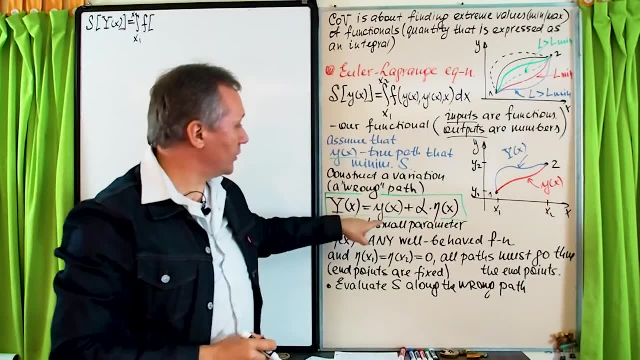 And you know what, In order to save a little bit of space, let me write F, And I'm not going to write Y capital, Y prime capital. I will write it immediately in terms of Y, small and eta. So here we'll have Y capital, Y prime capital. 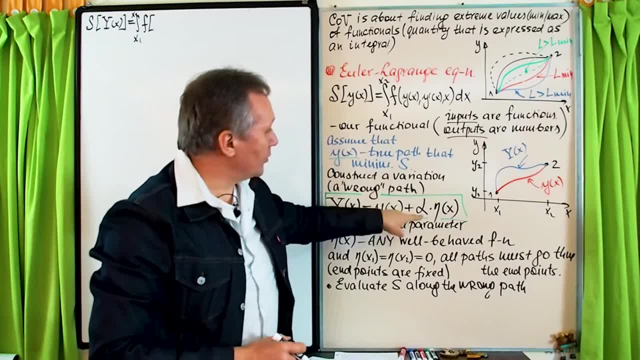 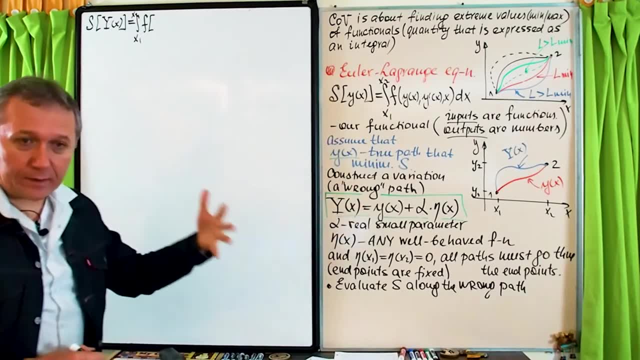 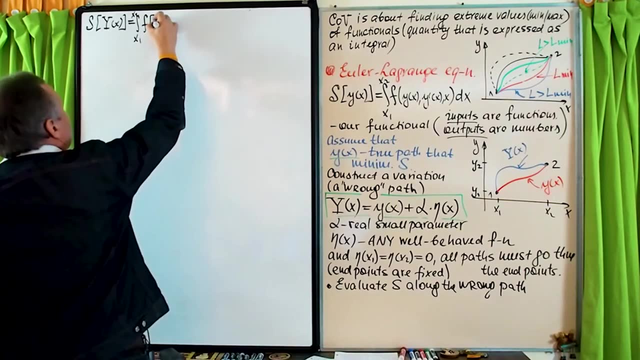 But I can write immediately. So it will be here Y small plus alpha eta, And here we'll have Y prime plus alpha eta prime. So it will be which way? Yeah, So Y plus alpha eta, Then Y prime plus alpha eta prime and X right. 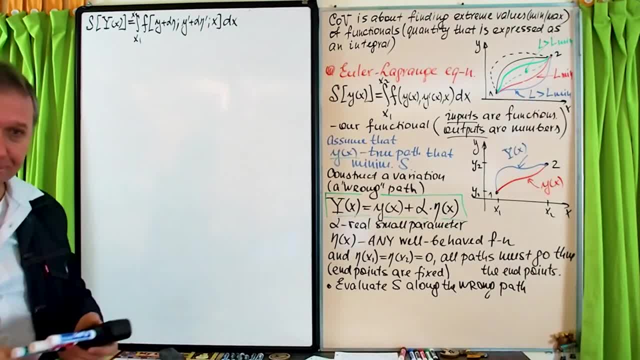 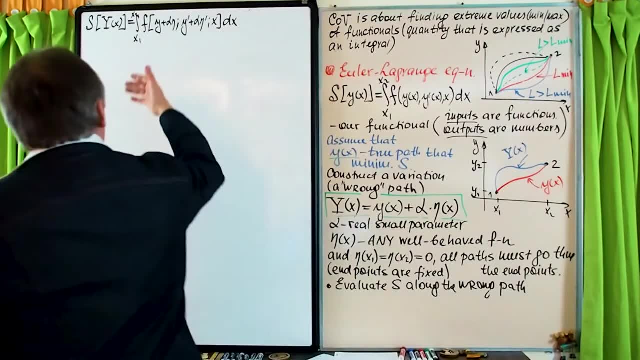 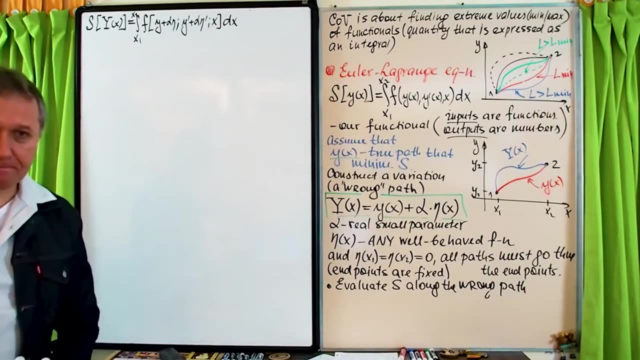 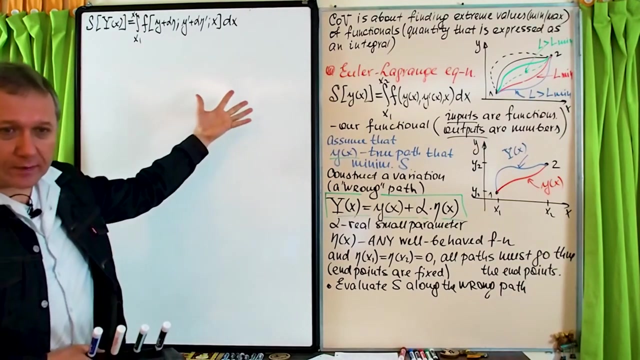 And DX. So now, what are we going to get if we integrate it through? You can still see it. Yeah Right, So it's an integral over X, Definite integral. So upper and lower limits are given. 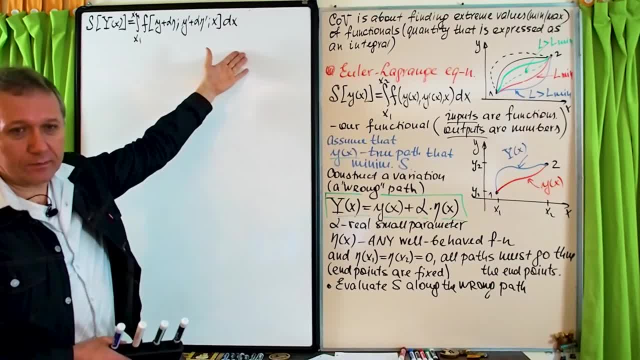 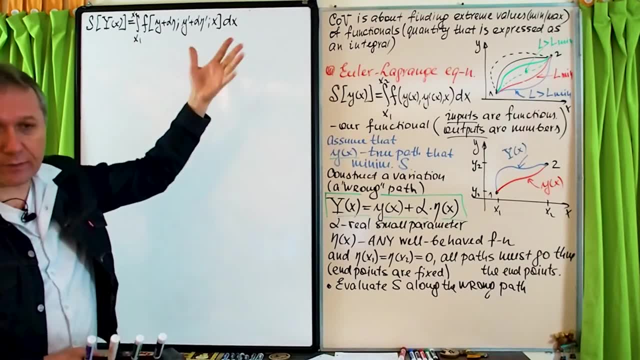 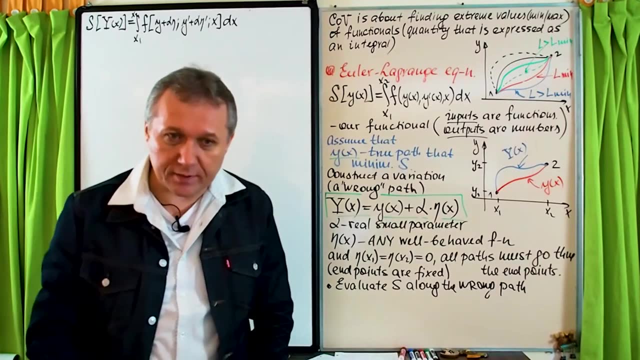 Some numbers. So if you integrate it, X will be integrated out, So X will not be left, It will not be here. Of course, Y is a function of X also. So everything will disappear except what. Everything will be turned into numbers, except what. 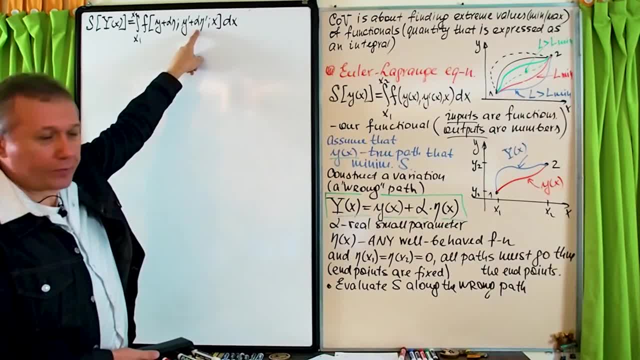 Except our newly integrated. So alpha will survive through this brutal integration. So it will be. at the end There will be some numbers and alpha present And we haven't imposed any significant restrictions on our alpha, except for its real And small, yeah, but 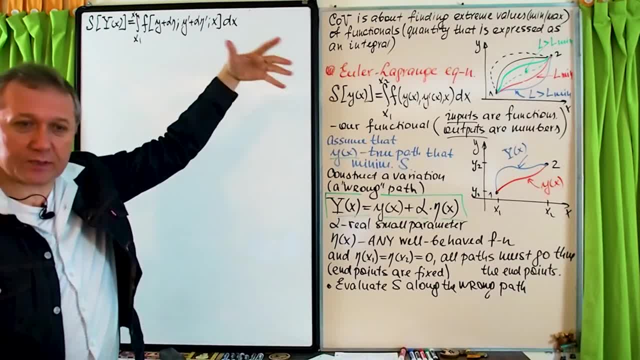 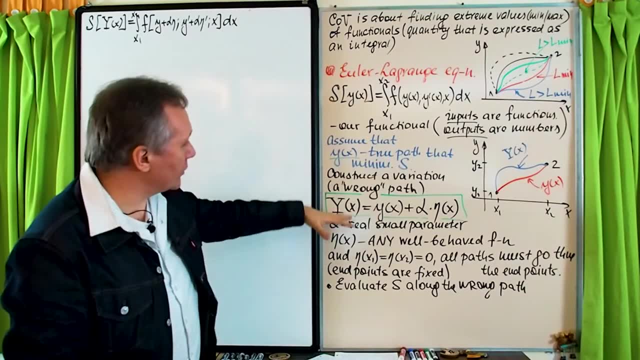 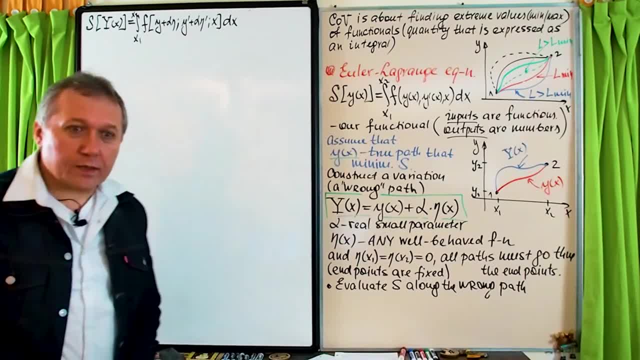 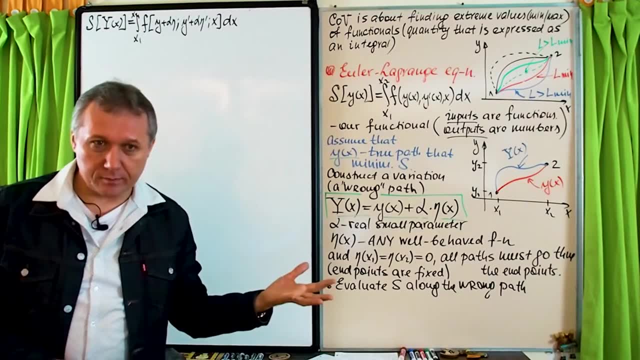 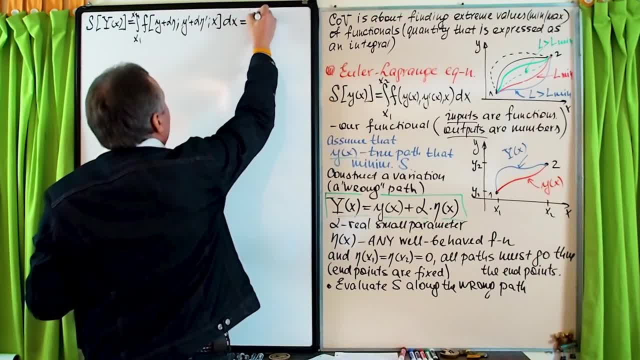 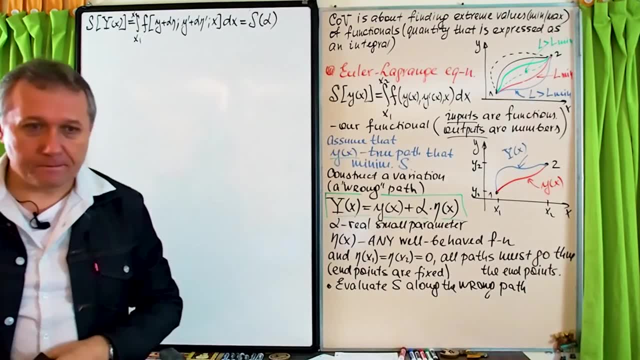 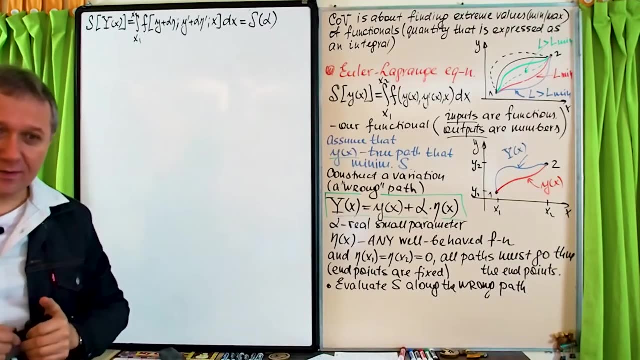 So I can write these, that this will be some new function, S as a function of alpha, So now I can start treating my alpha as a variable. So now I will—I will- have just a normal rainbow根号. 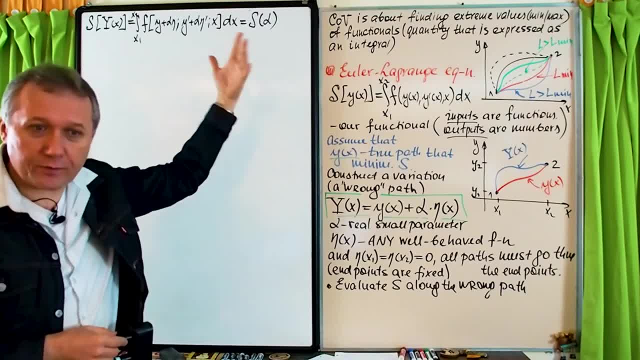 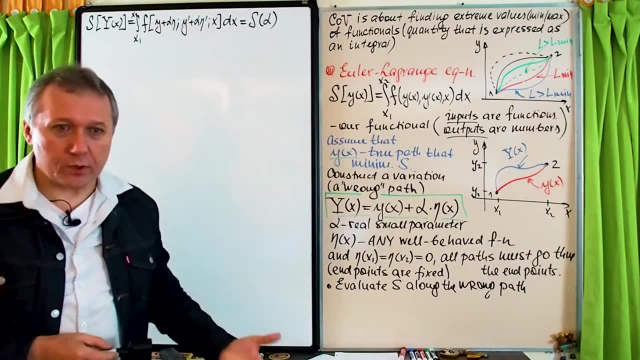 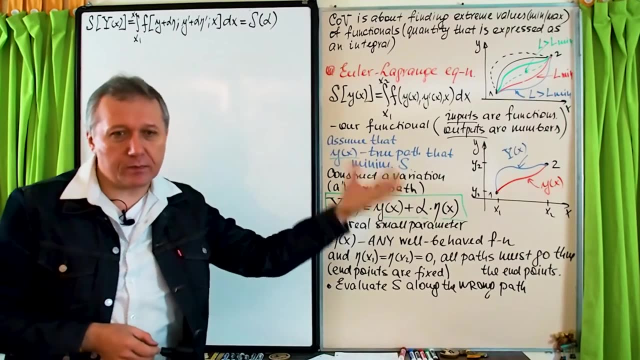 That's right. regular function function of alpha. S is the function of alpha, So I'm not going to have any. some weird functionals, right? Because we have no idea how we can treat those functionals, How we can find that, how can we minimize them. 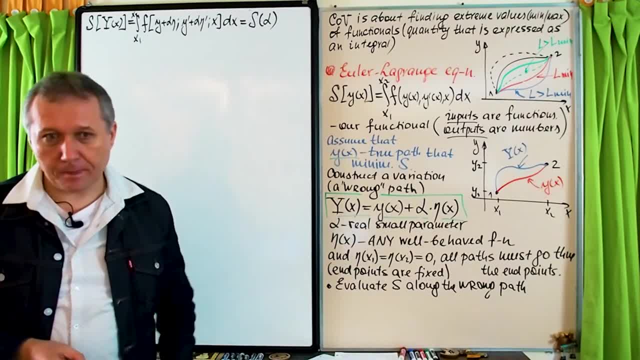 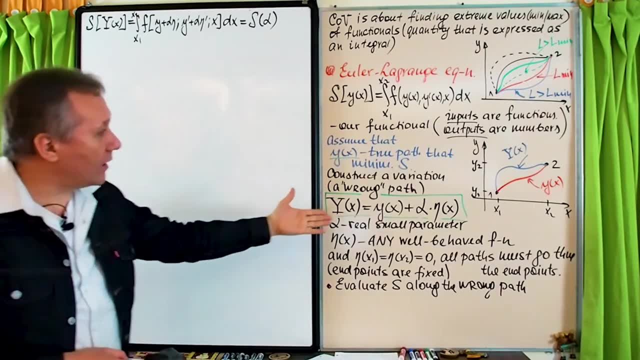 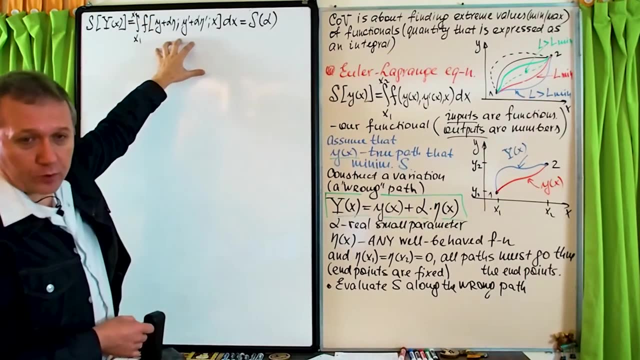 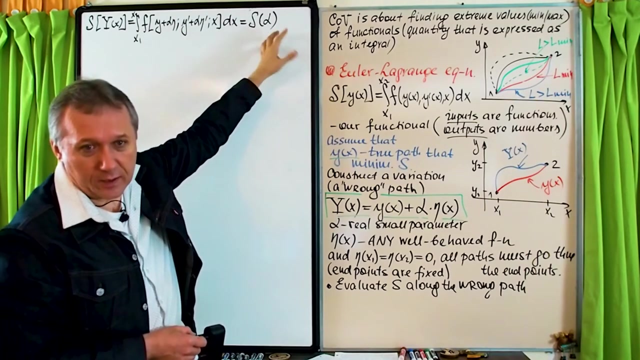 So far we have no idea about them, not much. But by doing this, by introducing artificially this parameter alpha now we're basically switching, moving from some weird world of functionals into the regular world of functions, And in this case it's a function of one variable alpha. 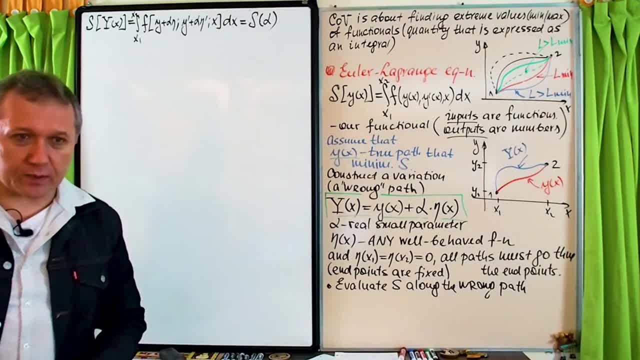 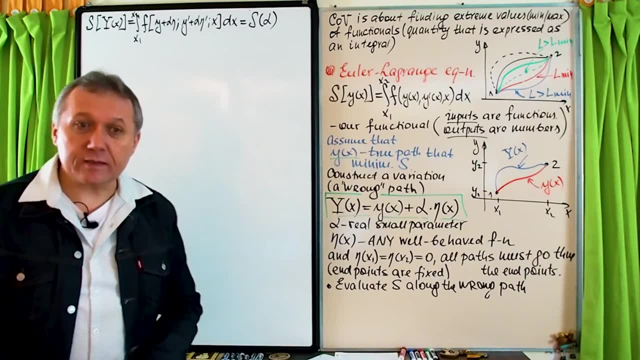 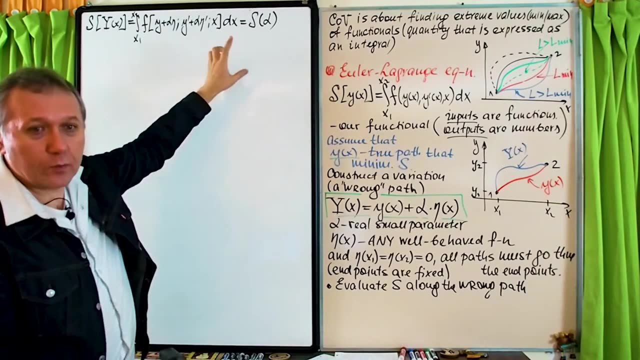 We have tons of tools from calculus one, calculus two, which can be used to analyze this function. This is probably one of the most important steps. By doing this, by By introducing this alpha and analyzing this way, we're switching from the strange world of functionals. 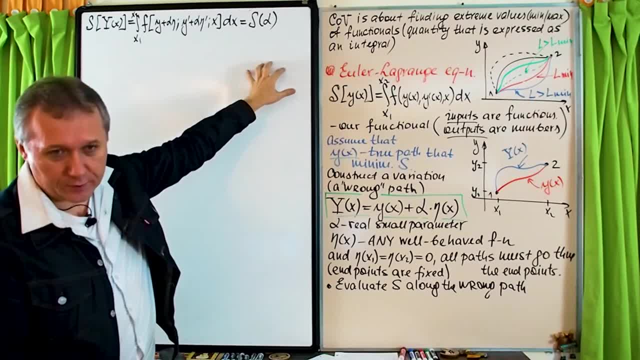 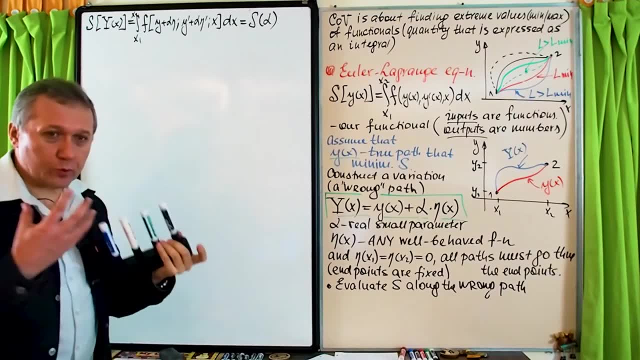 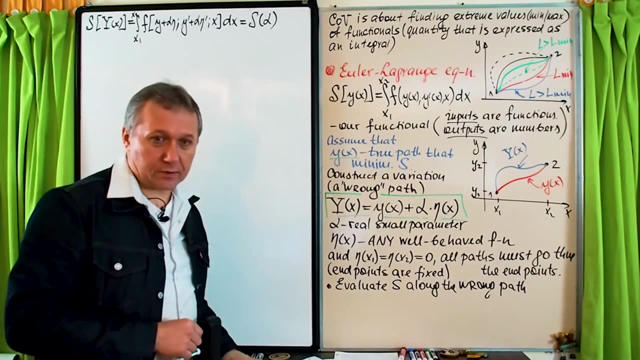 to a normal, regular world of functions. Okay, So this is probably, in my opinion, one of the crucial pivoted points in this derivation, And then the rest will be regular calculus, right that have to be applied. that has to be applied. 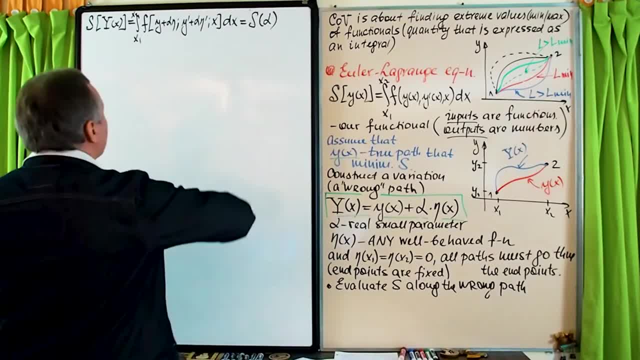 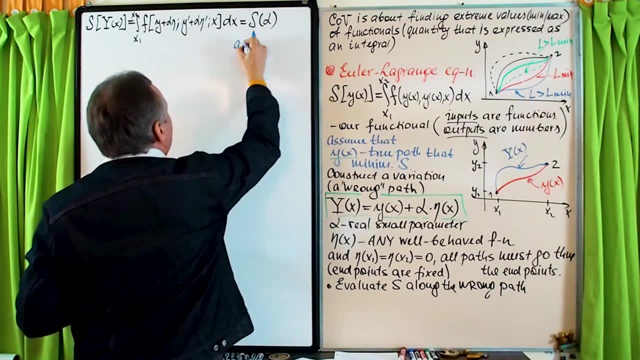 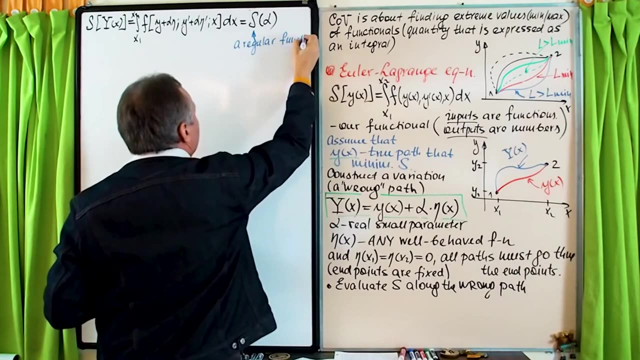 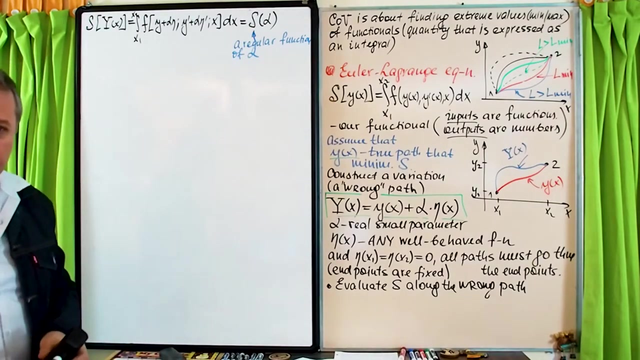 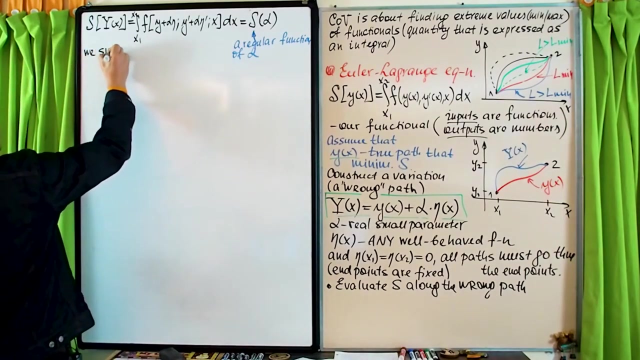 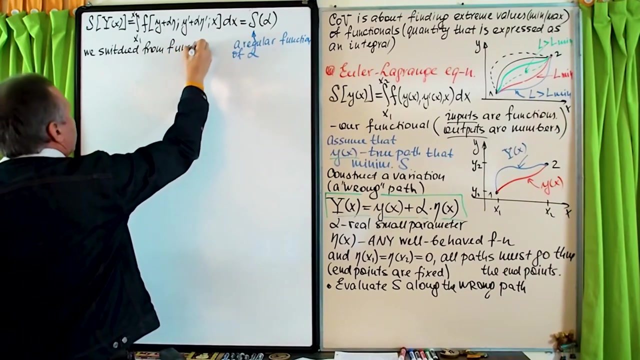 All right. So now, let me emphasize on this. So here we have a functional, And this is just a regular function of alpha, regular function of alpha. So we switched, So we switched, We switched, We switched from functionals, from functionals. 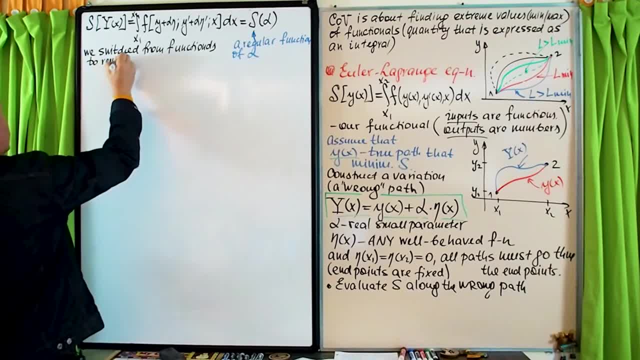 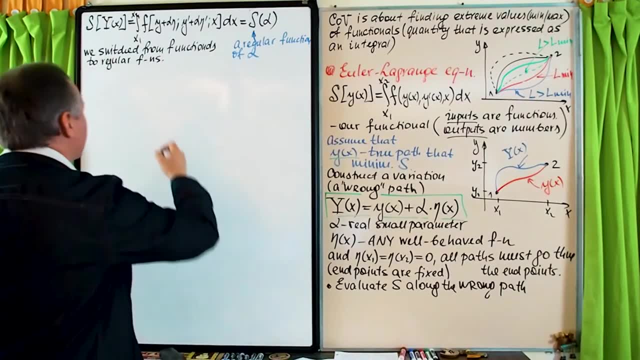 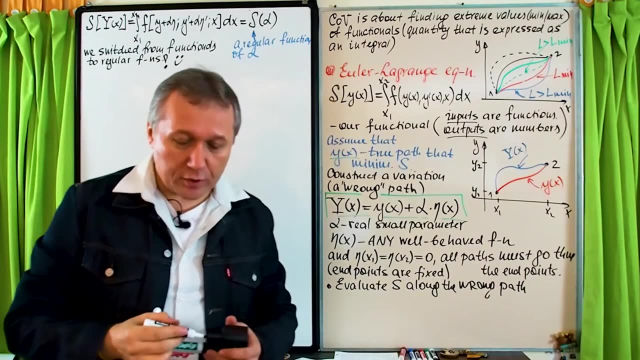 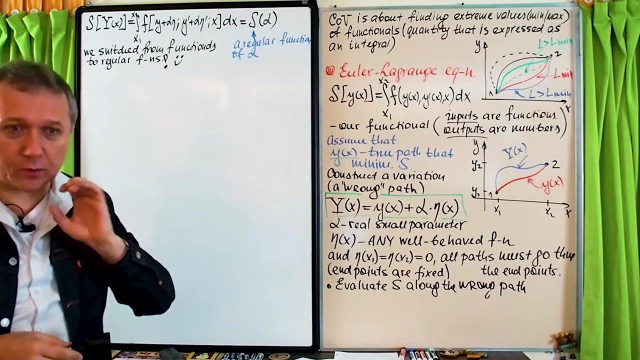 to regular functions. Okay, let me put an exclamation mark and happy face. Okay, what else now do we know about this function S, Which is the function of alpha? What else happens Now? we have also an important piece of information which we need to realize. 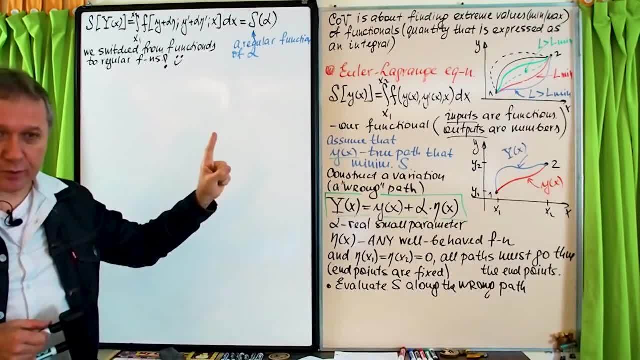 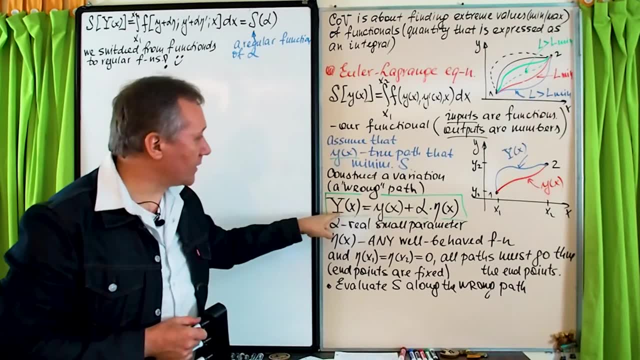 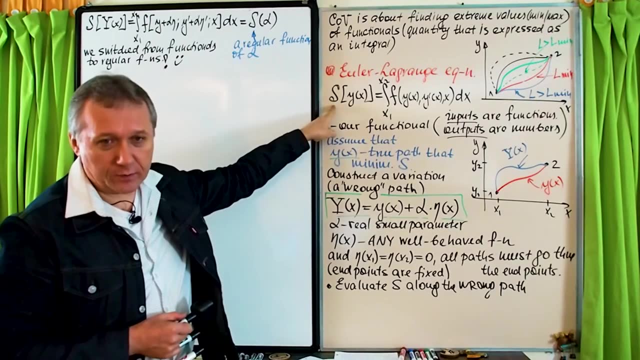 What happens when alpha equals to zero? When alpha equals to zero, alpha equals to zero. this, of course, zero in our wrong path turns into the true path. What happens with our functional when we are on the true path? It becomes minimum right. 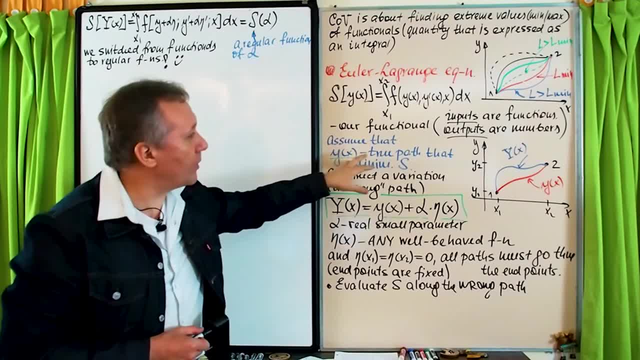 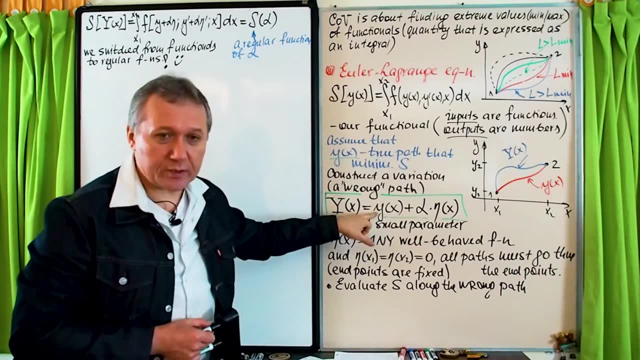 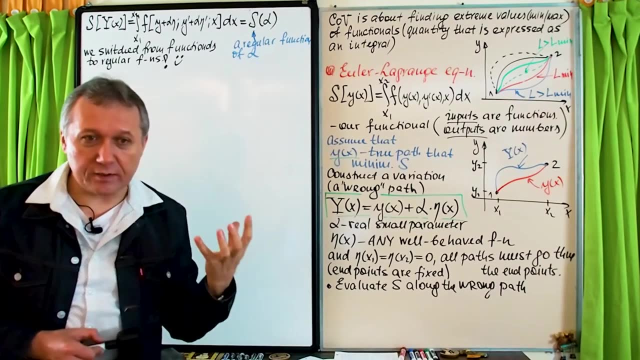 That's what we assume, that y as a function of x is the true path which minimizes s. So when alpha equals to zero, y capital equals to y small and s is minimum. So at alpha equals to zero, our functional is minimal. 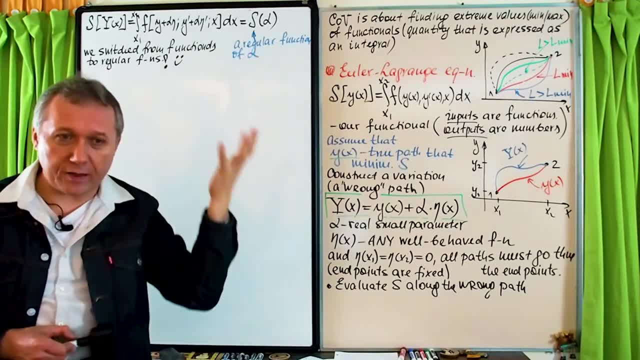 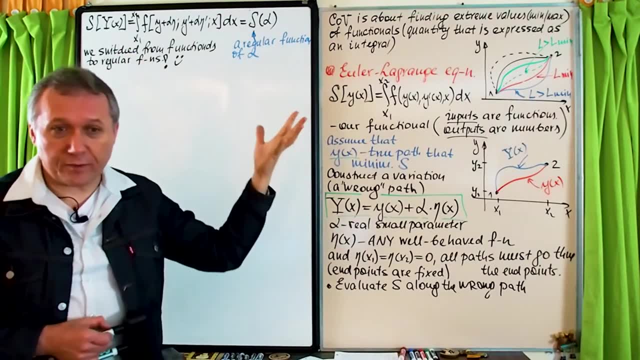 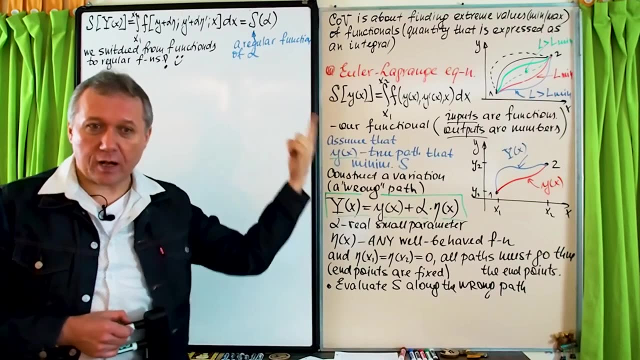 Our function in this case is a function We switch to function. Our function reaches minimum value. So now, on top of the fact that we switch to normal functions, now we also know one additional piece of information: That, at alpha equals zero, our function is minimum. 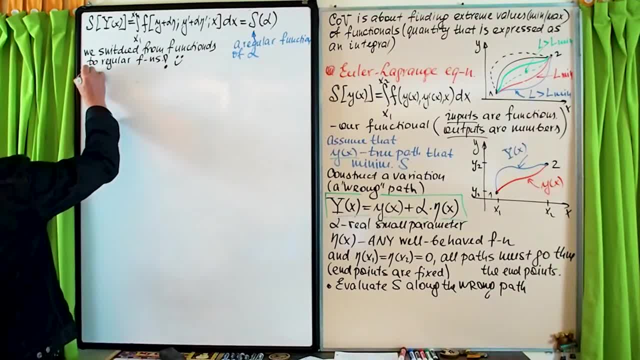 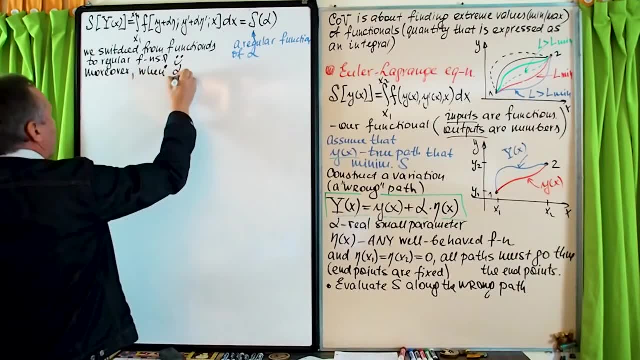 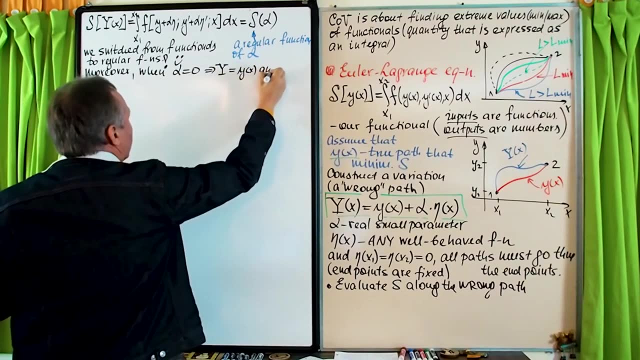 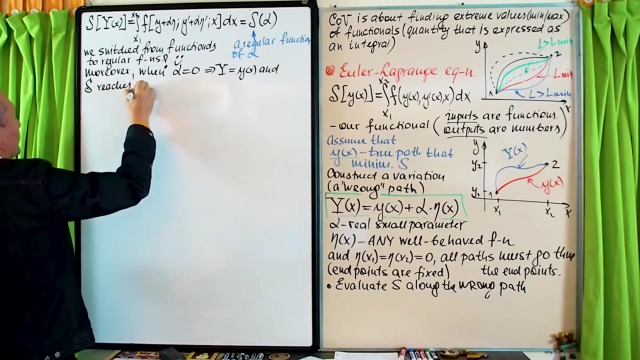 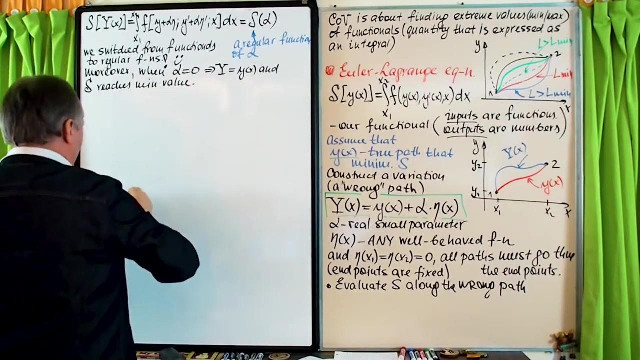 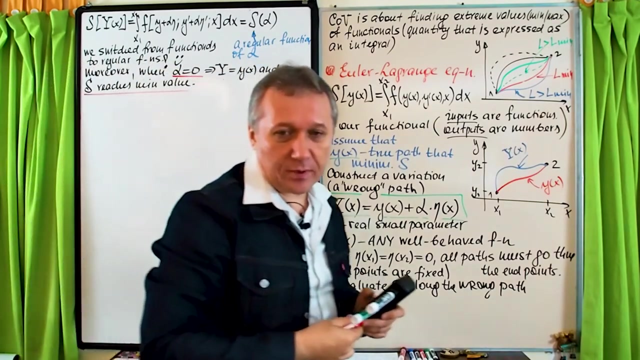 Okay. so, moreover, when alpha equals to zero, y capital equals to y small and s and s reaches minimum, When- okay, let me- alpha equals to zero and s reaches minimum value. So now, this statement will allow us to dive deeper. 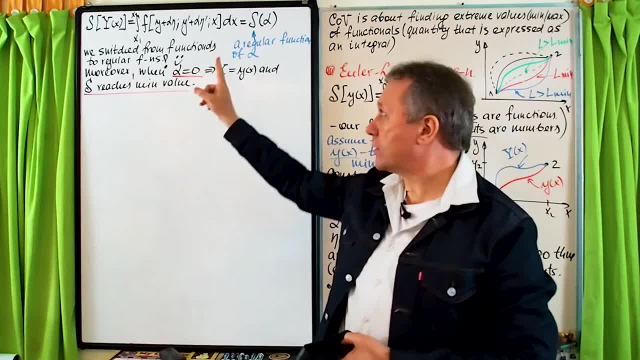 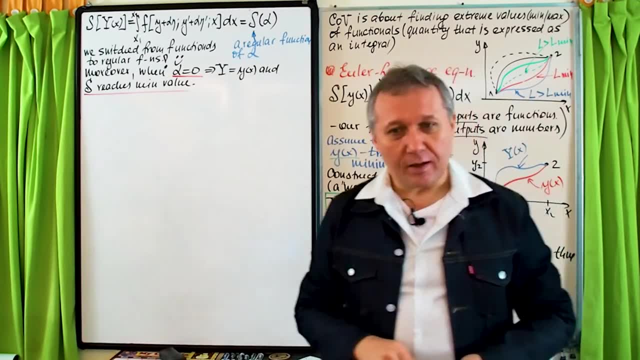 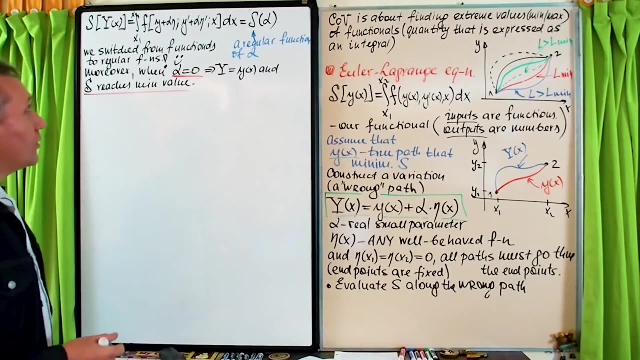 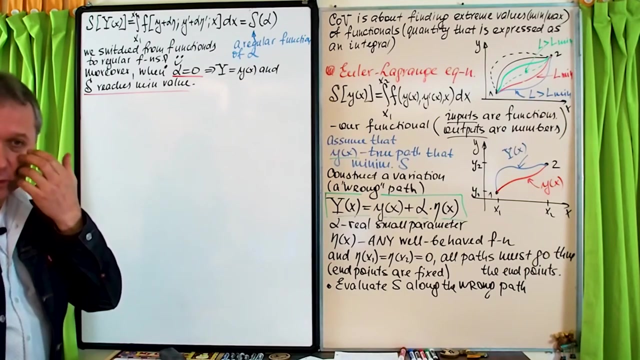 And get what we wanted. So first we made it, made a transition to normal functions, and now this piece of information will allow us to continue through the derivation right. So, and we know what, how we can find the first step in a search for minimum points. 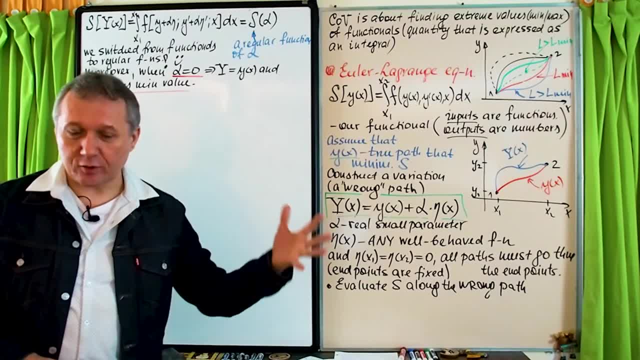 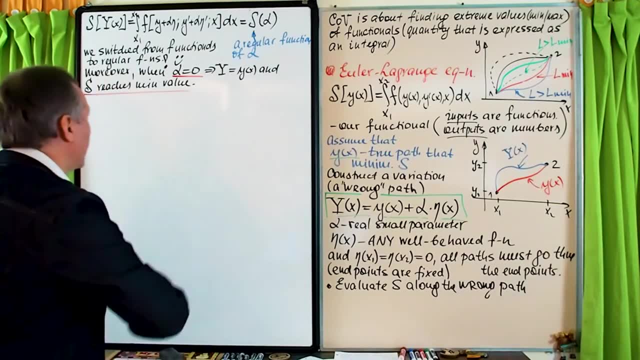 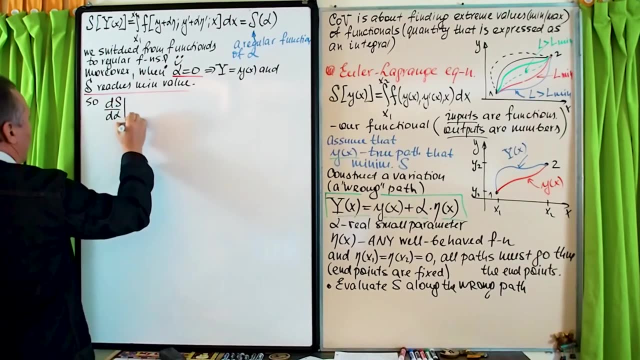 First you need to find the stationary points right. You need to first differentiate. You need to first differentiate function with respect to the variable right And equate it to zero. It's the first step, right. So ds over d. alpha when alpha, yeah, when alpha equals zero equals to zero. 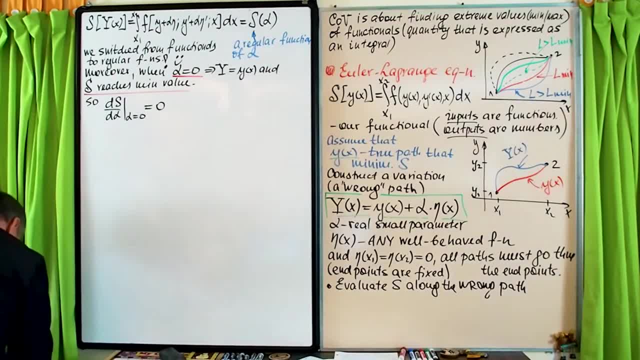 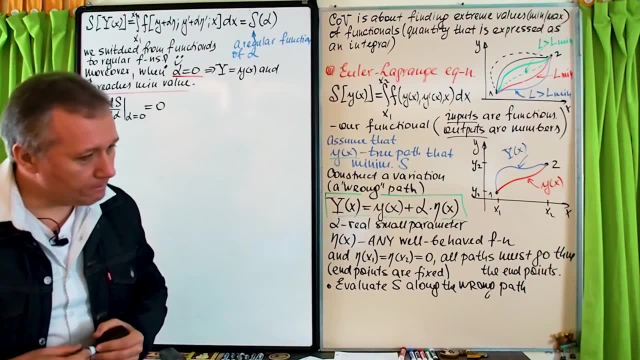 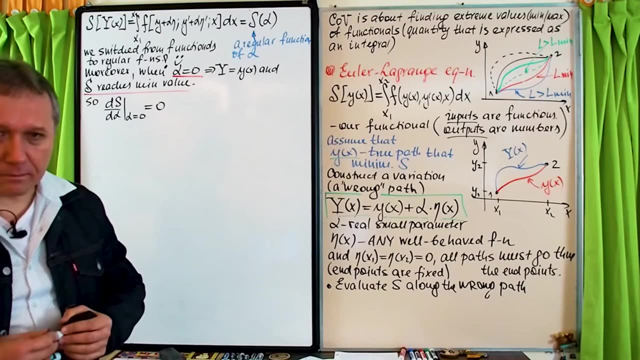 Right Stationary point, Oops. So the reason behind actually having this alpha over there Is like we're kind of guessing at a wrong path and with this alpha parameter we can kind of constrain our solution such that it'll actually be the correct path. 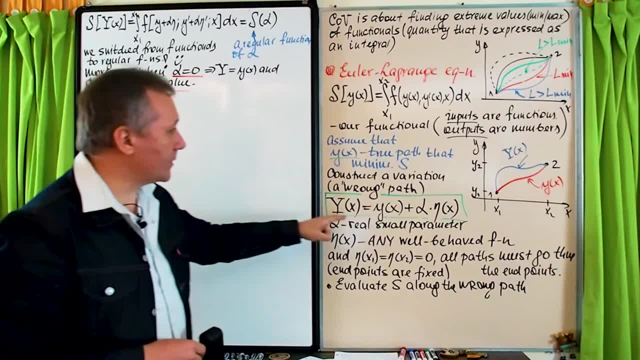 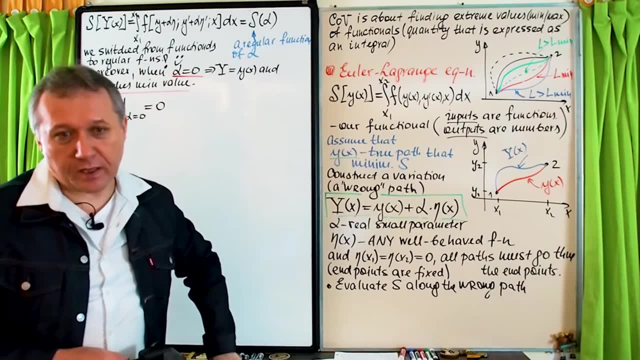 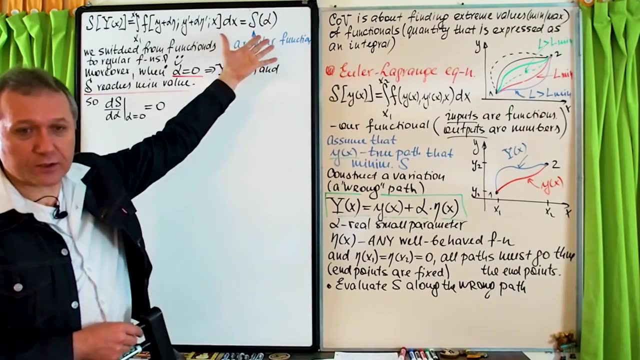 Is that kind of Yeah, So when alpha equals to zero, as I explained, yeah, alpha equals zero, so this disappears and that, with that parameter, our wrong path becomes the true path. And of course, the state, the functional is minimum and of course, since we're getting this function out of the functional, of course the function will be also minimum. 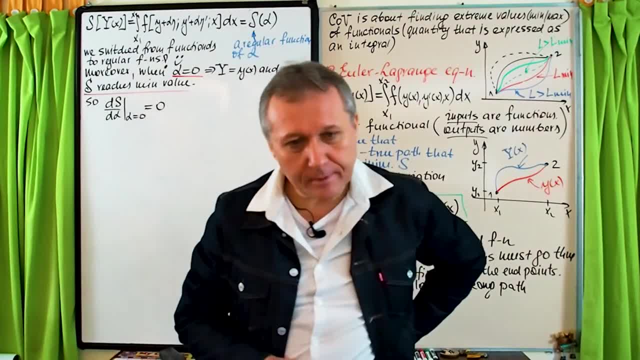 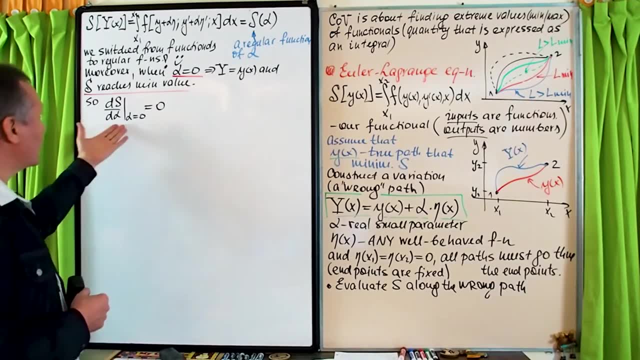 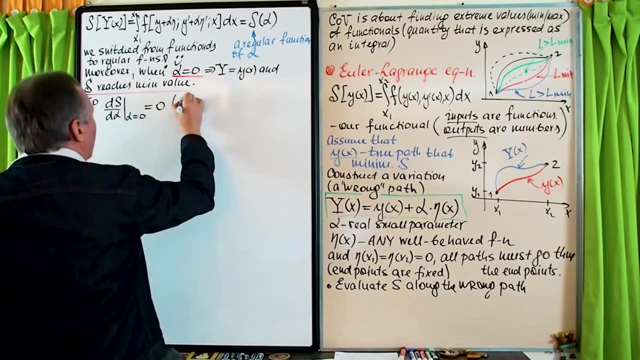 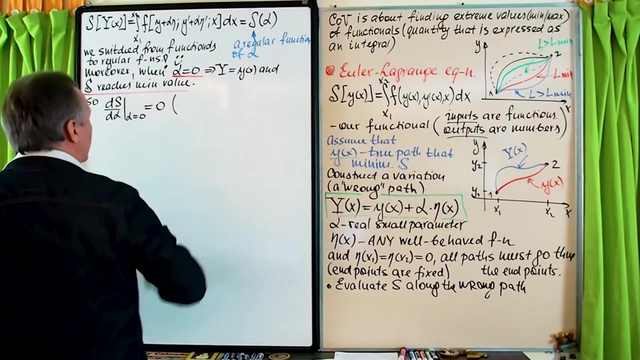 Right, Yeah, That's the correct statement, absolutely Okay. And as the first step of searching to search for minimum points, of course you need to search for stationary points, So let's use it. So a search, oops. okay, let me just write for stationary points. 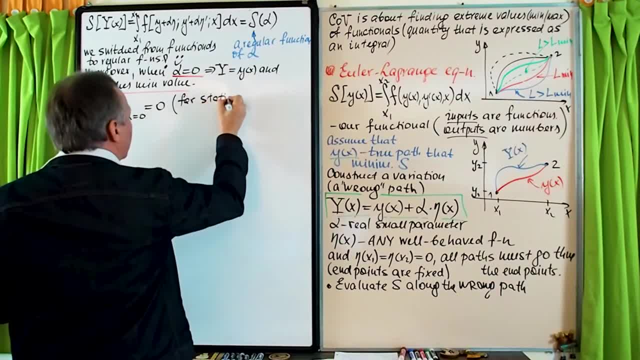 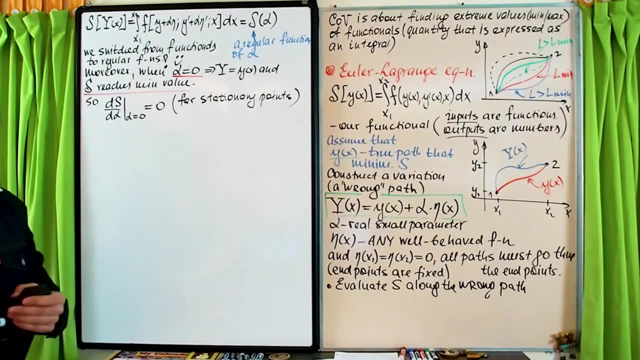 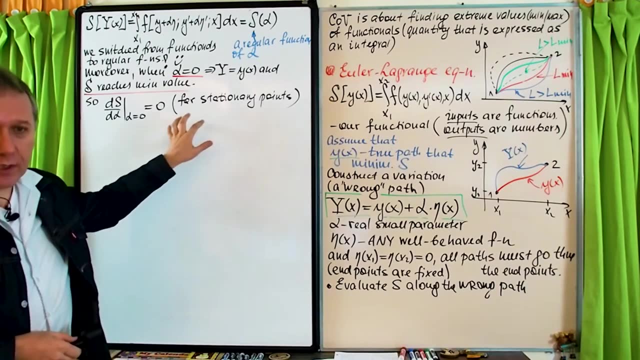 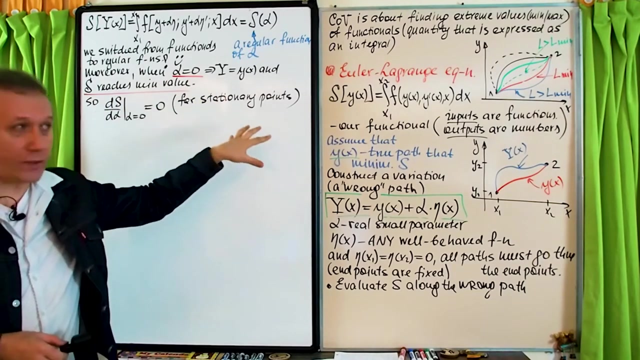 For stationary points, For points, Right, Okay, So, as a result, okay, let me sort of jump ahead. So we are using conditions for stationary points, right, Although this goes much deeper: it tells us that the value of S will be minimum. but what we use, we use this stationary condition. 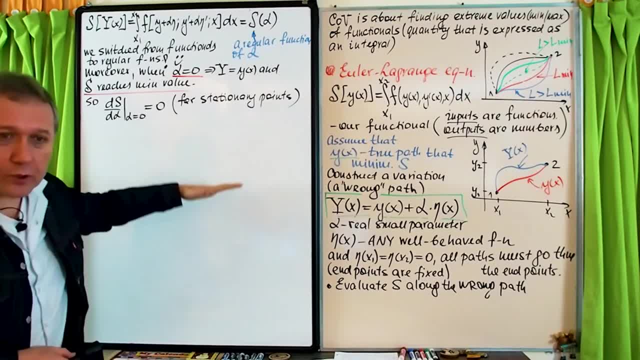 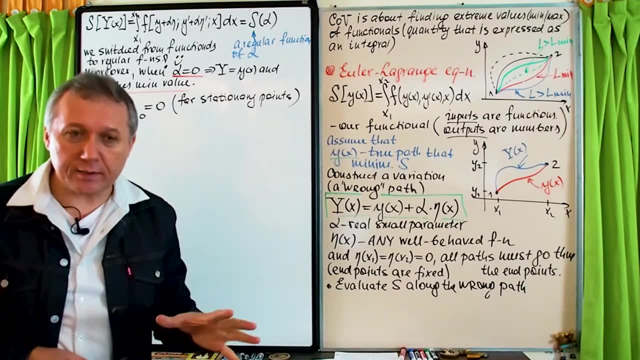 And now, using this stationary condition, we are going to derive the tool which we need right And, as a result, that tool is not going to be in the right position. that tool which will be derived can guarantee, only can only guarantee that. 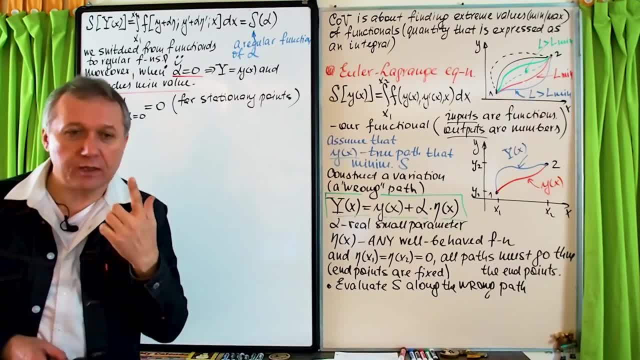 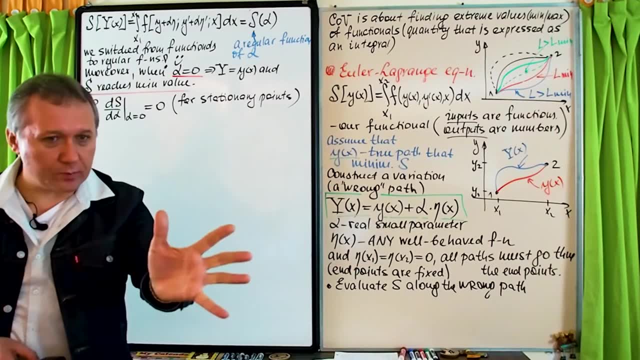 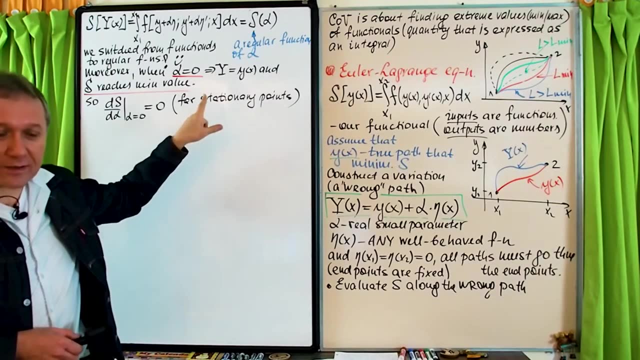 your functional is going to reach station. it can be stationary. it cannot guarantee that will be a minimum. so it can be a minimum or can be a maximum, right, because again, stationary, stationary conditions cannot guarantee that, guarantee that it will be a minimum point. it can be minimal and maximum. 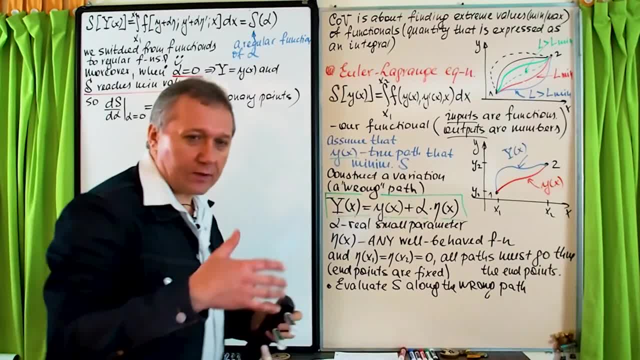 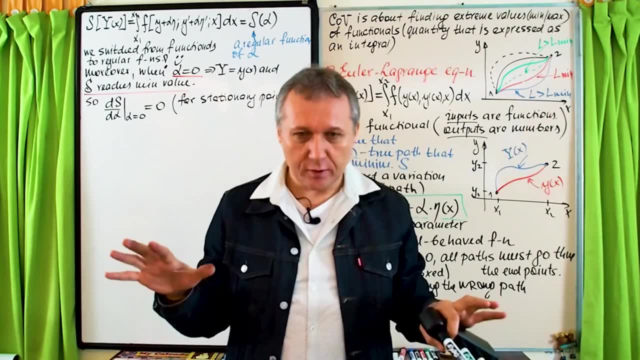 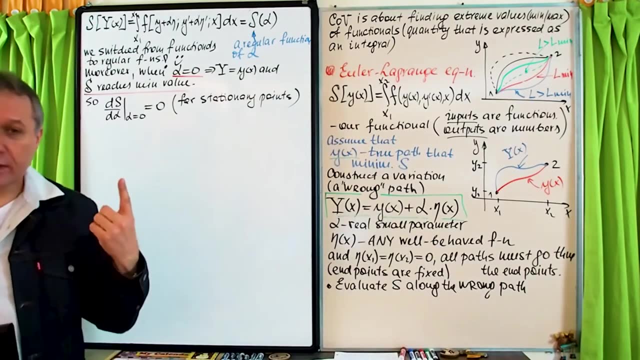 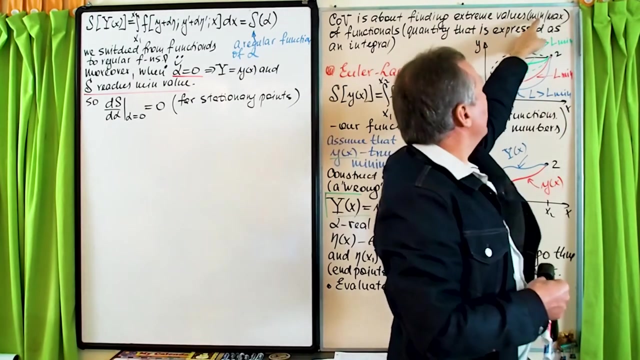 right. so in order to prove that the value of the functional is going to be minimum, you have to do some additional step stuff. we're not going to do that, so every time in calculus of variations we use this tool, which guarantees only the stationary value. that's what. that's why I wrote here: extreme values mean max. 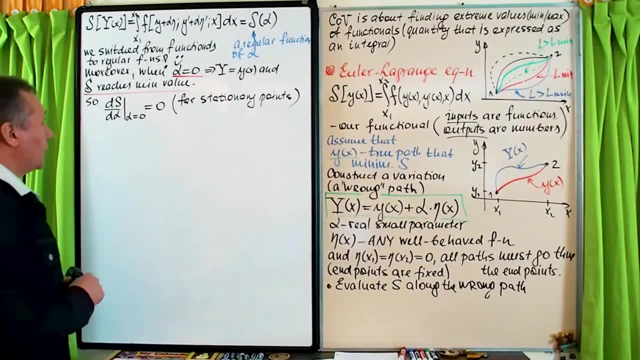 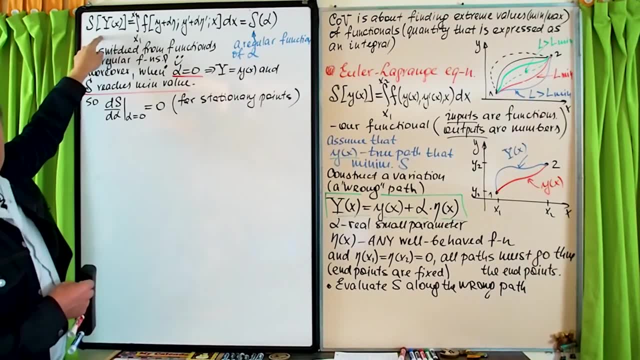 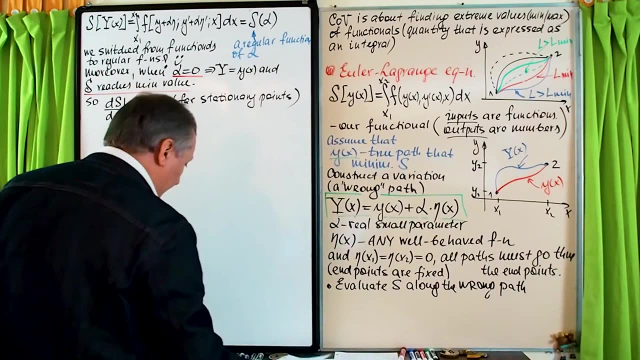 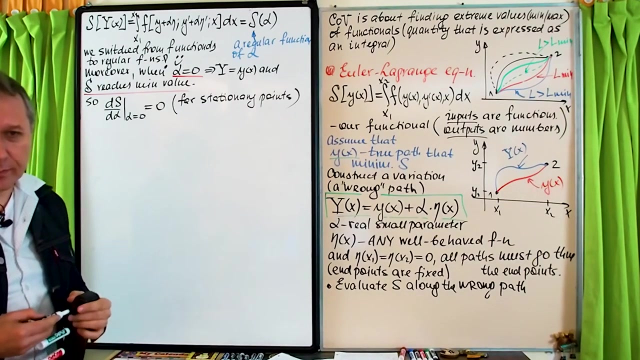 right or functionals. okay, so now let's differentiate our functional this, let's differentiate along the wrong path, right and and. so, in order to differentiate integral, let's recall Leibniz rule. I remember it was, I think, in the freshman year when I was in. 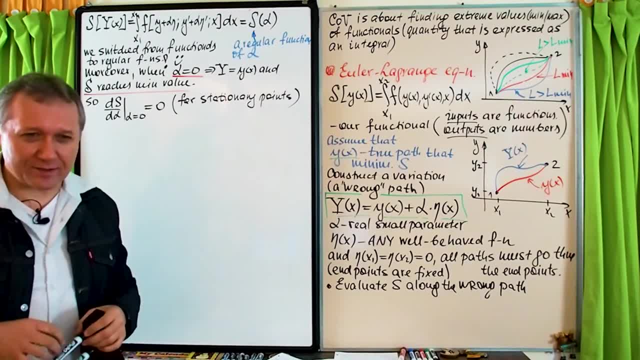 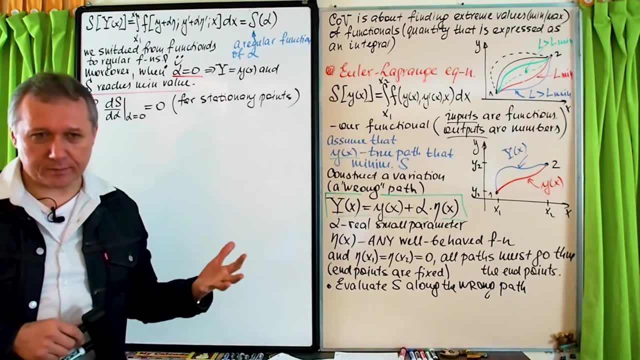 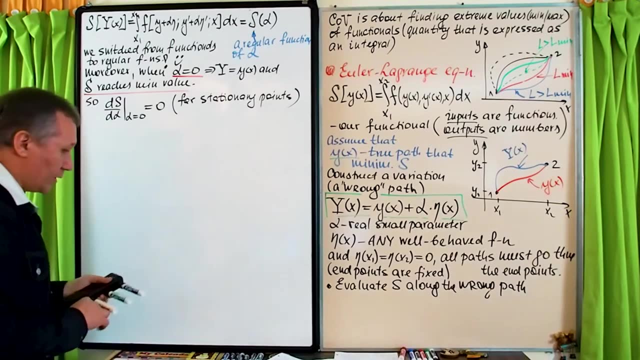 freshman year I remember I was practicing: we derive, we had to derive everything. so we derive this Leibniz rule- how to differentiate- and an integral where the upper limit can be a function of X, lower limit can be a functional effects in integral can be a functional effects. so let me just write down that Leibniz rule. 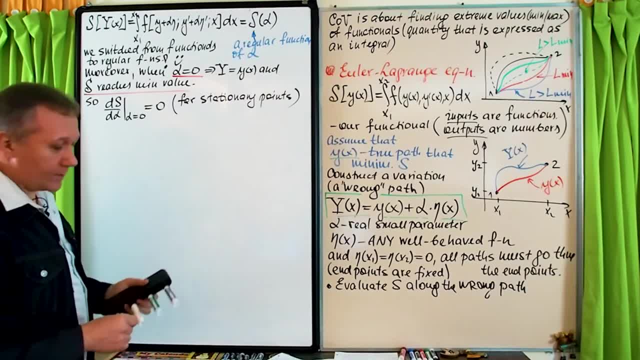 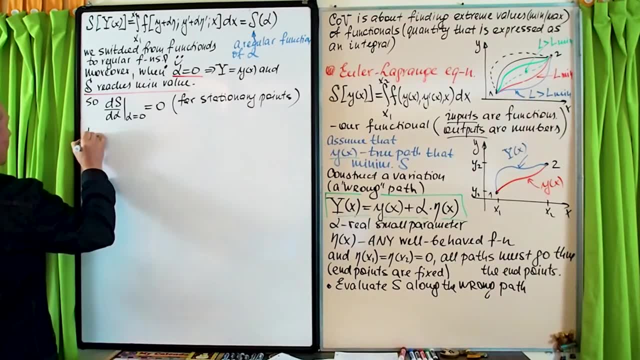 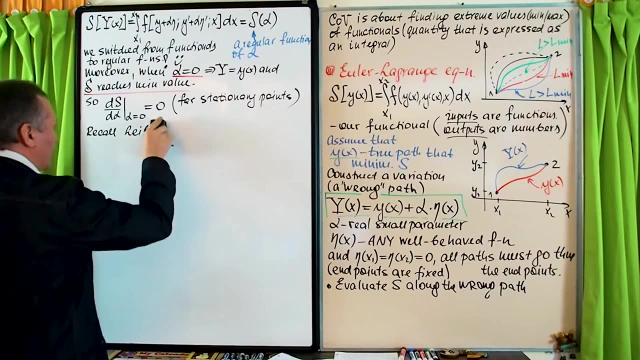 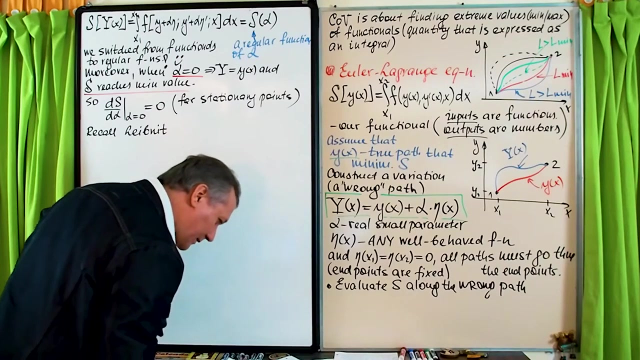 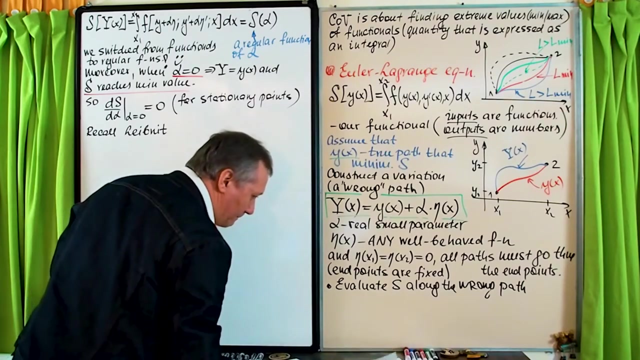 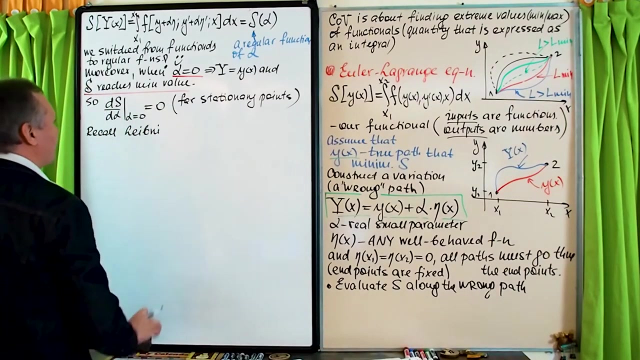 and then we will apply it for our particular case. okay, so small digression, recall Leibniz rule: it's good. okay, I don't trust live need. I think that was the correct spelling. no, no wrong Z at the end, just Z at live needs rule, right. so what does it tell us? 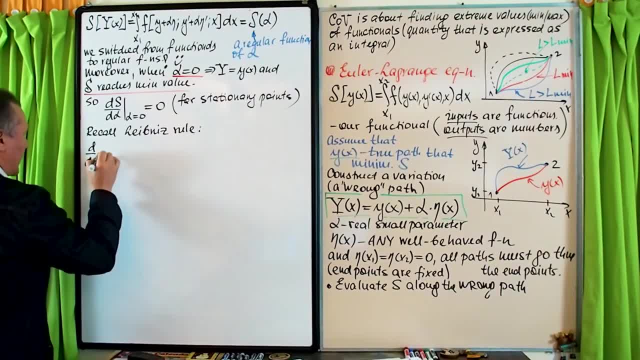 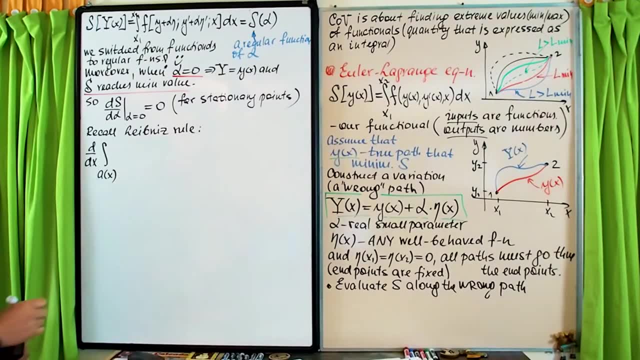 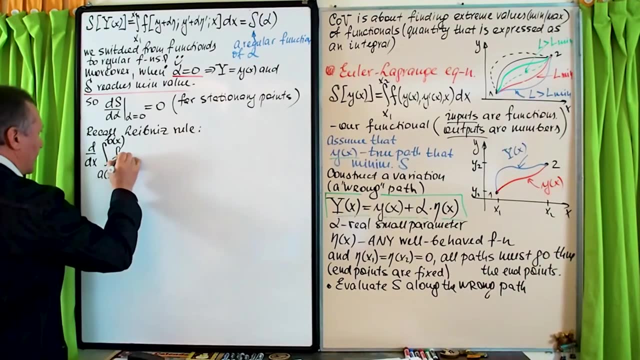 so if you have D over DX out of some integral, which is a function of lower limit as a function of X, a as a function of X, upper limit, B as a function of X, then integrand, which we eroded, F, which is a function of X, and we wait alpha. 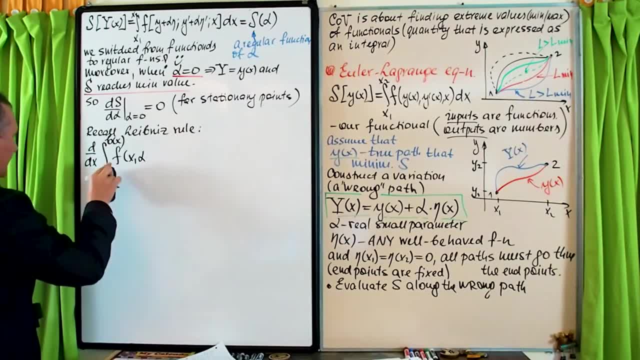 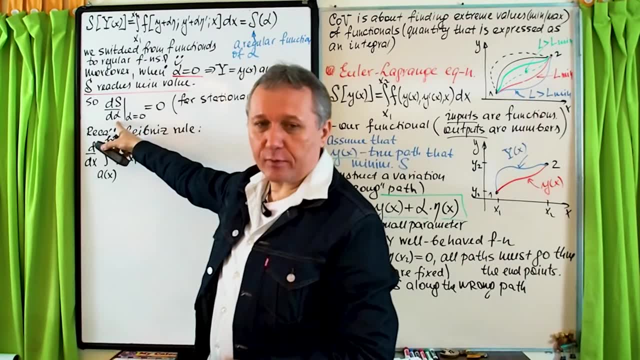 alpha, okay. okay, I need to use my notes more, so instead of X, I use alpha, so let me change. also, since we are going to, here here, integrate or differentiate with respect to alpha, let me also use here: instead of X is alpha. again what I'm I started writing, it's not wrong at all. 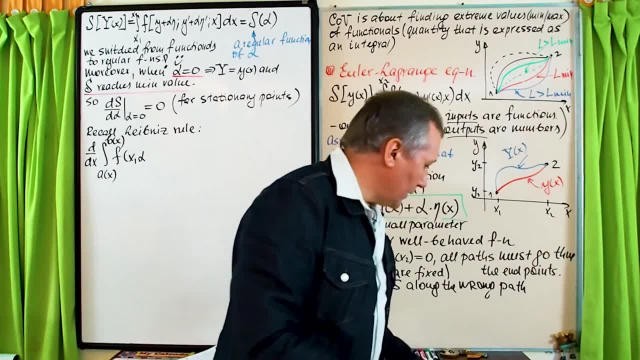 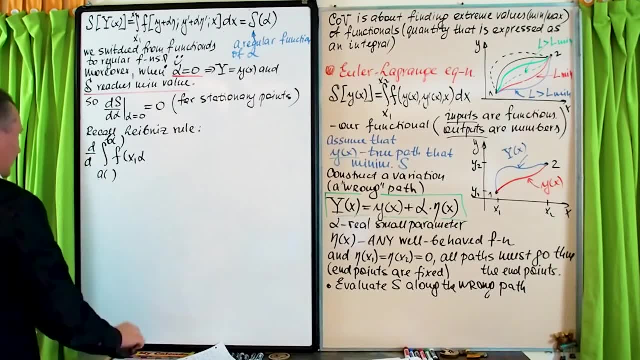 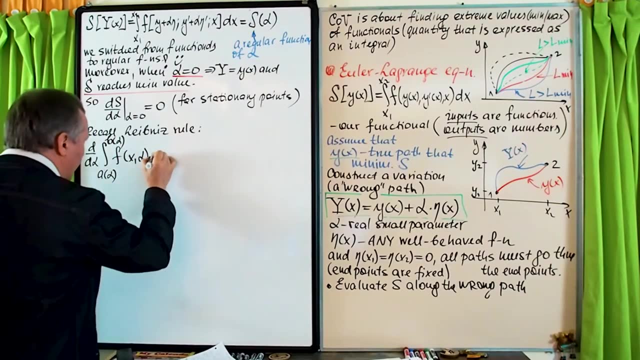 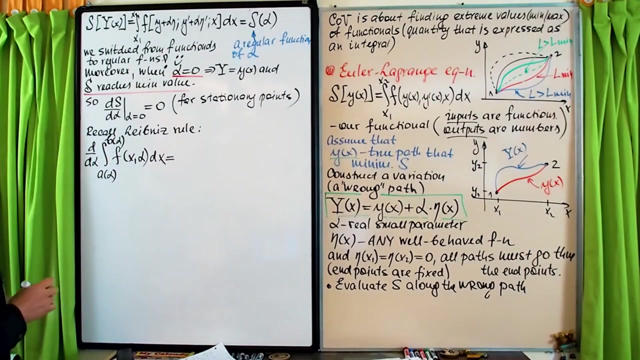 all right so in order just to be consistent all right so let me change to alpha since I haven't moved that far alpha alpha alpha and so it will be alpha alpha alpha right and D X okay so according to that rule on the same law I'm going to integrating or思 � Field F is the 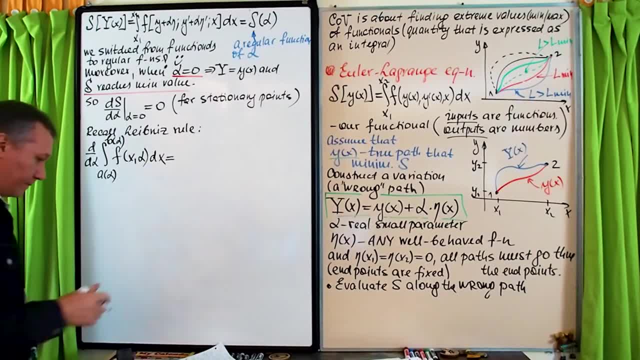 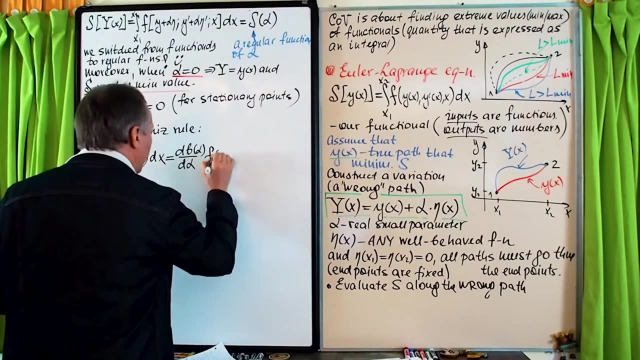 meaning of alpha, alpha and I have I already. plus it's evidence in the preschool problem of: okay, THY is N F, I. okay, now I have my higher up here again, it's gonna be 0 to alpha. what is alpha and what's that? values in the equation f of alpha 1, 2 and 4: you, you, you. 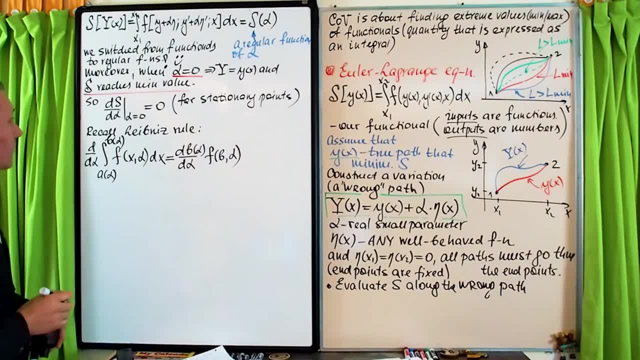 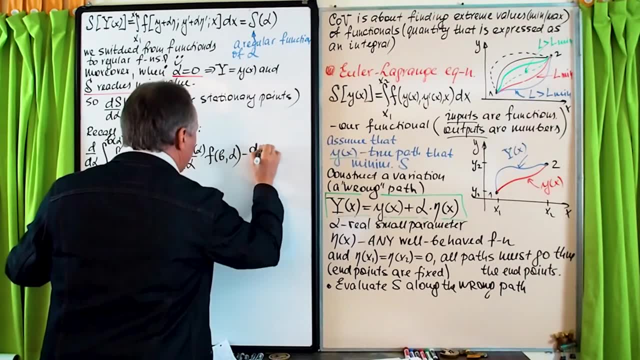 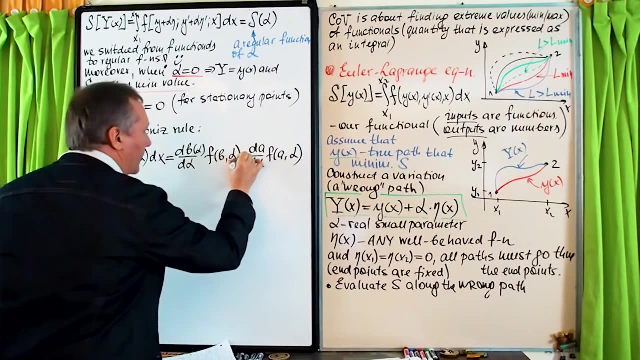 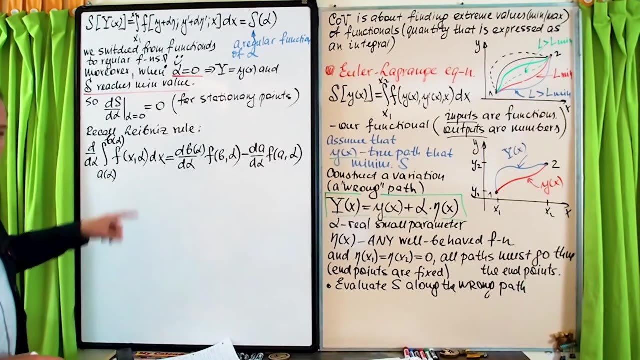 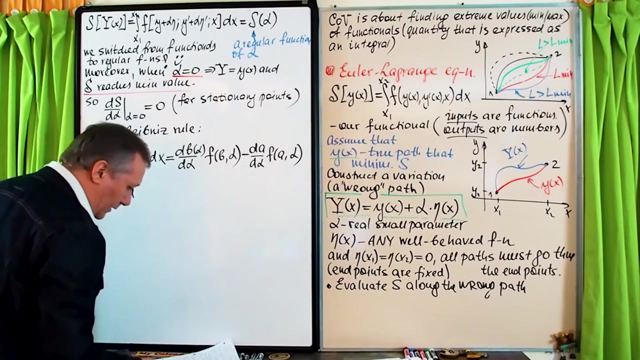 alpha, then minus the same with the lower limit, minus dA over d, alpha, F, A alpha and then plus integral over partial derivative of F, So plus integral from x1 to the limits, still So partial derivative of F with respect to alpha right and dA. 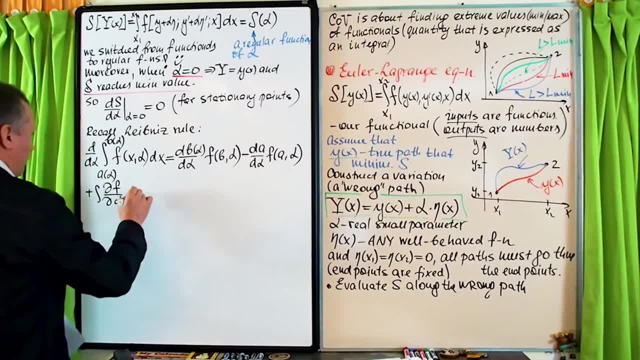 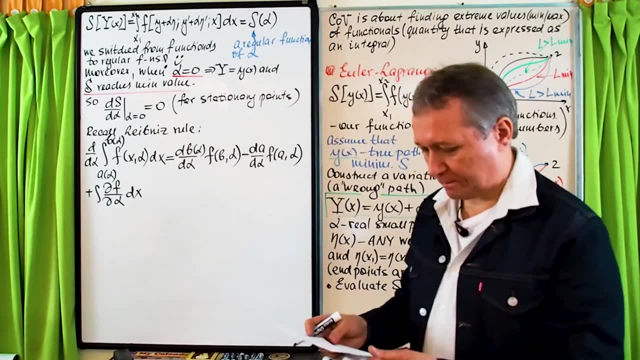 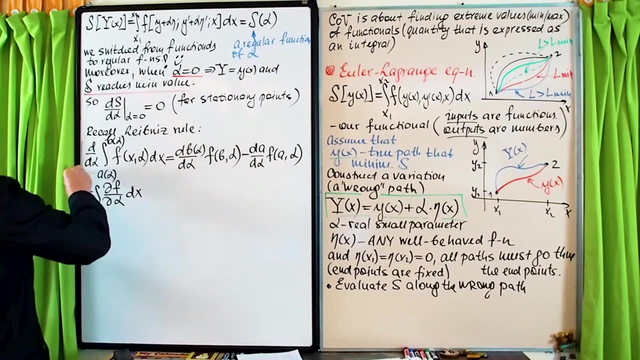 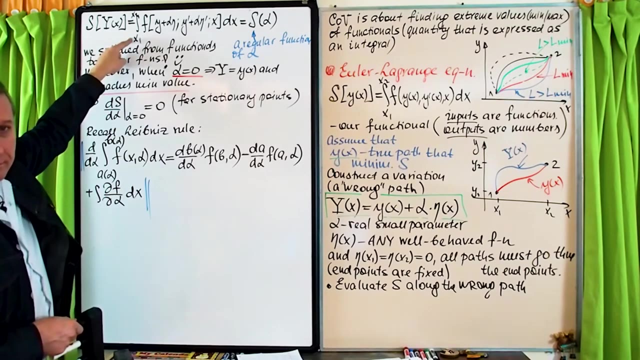 Okay, so now in our case, in our case, let me sort of frame it- In our case, upper limit number- I mean upper limit, lower limit is number right. so this and this will be zero. So we just need to differentiate with respect to alpha, because here that's what we do. 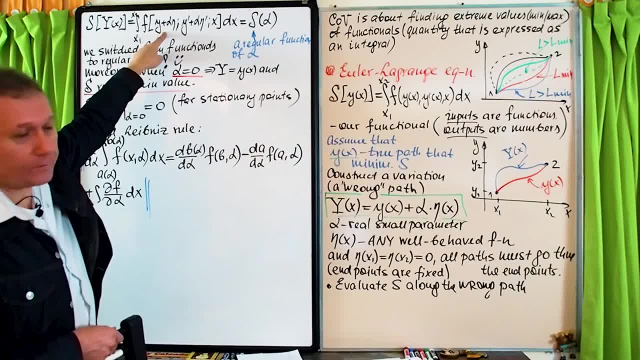 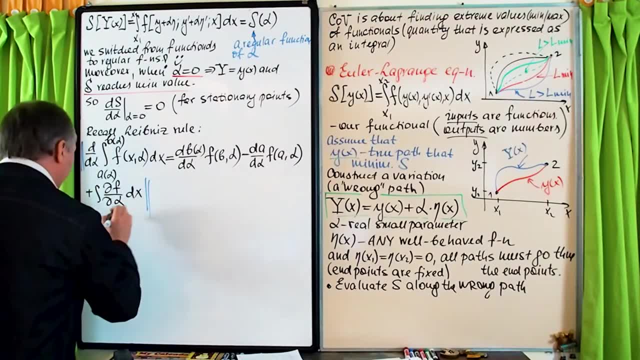 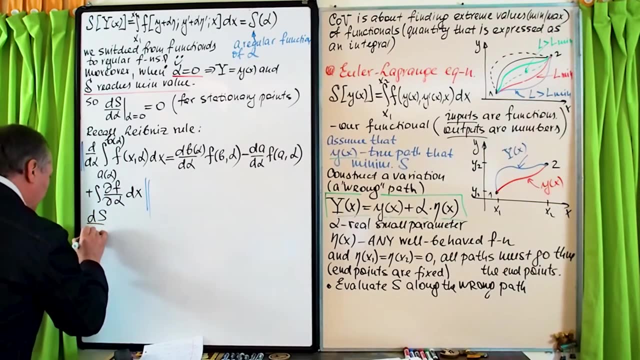 dS over d alpha. So we'll have to differentiate with respect to alpha integrant and equate it to zero. So in our case, so it will be- dS over d alpha will be equal integral from x1 to x2, right, so partial derivative Should I? yeah, let me write first dF over. 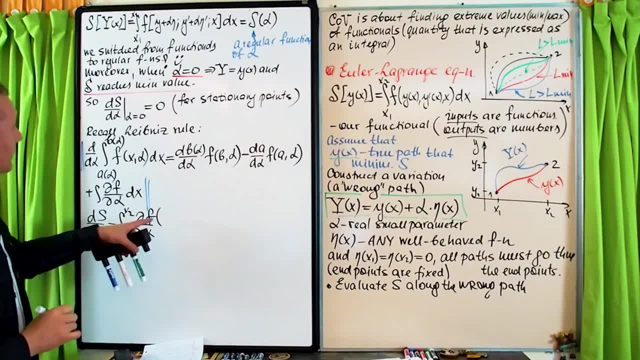 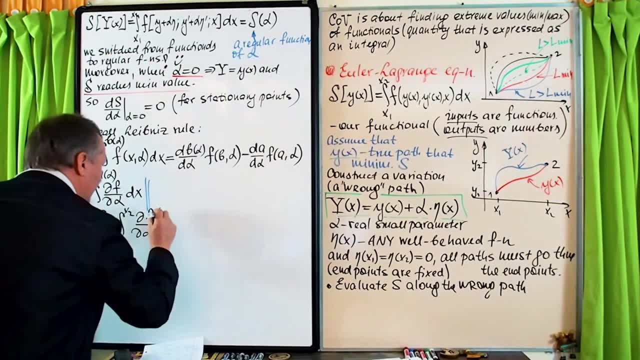 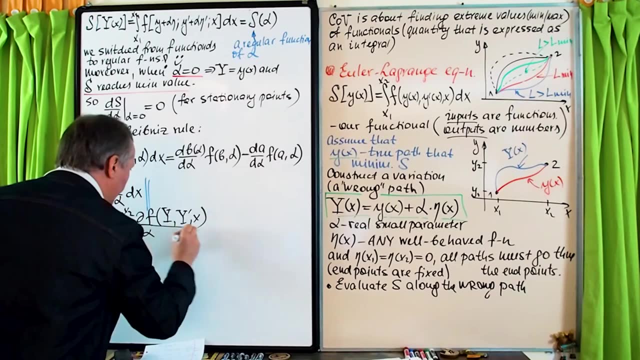 d, alpha and F. again, we're integrating, evaluating over this y capital. so let me write y capital here, Prime and x right. So now I just combine: this is y capital, this is y prime capital. 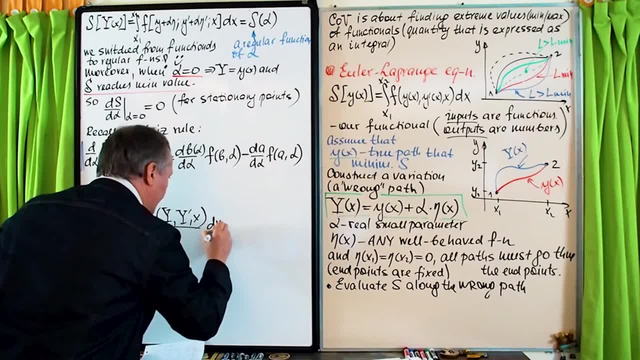 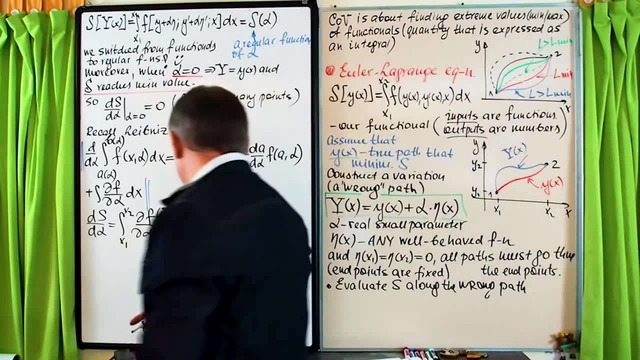 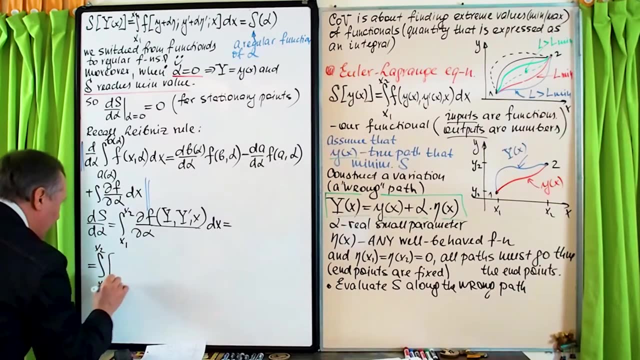 x, dx, right, dx, dx. Okay, so now, just using simple rules of differentiation, we can get. so it will be integral from x1 to x2, let me open the square bracket, so it will be dF. 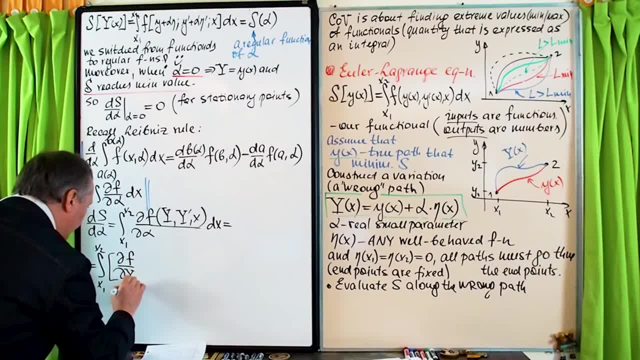 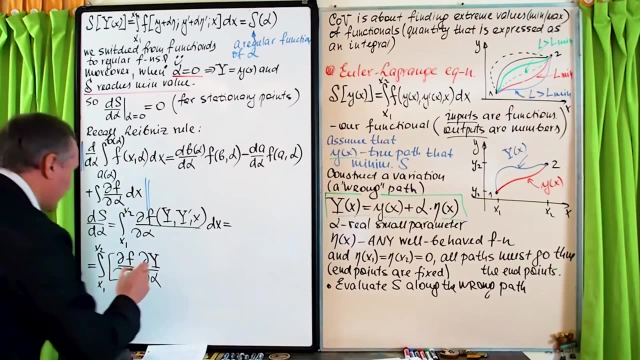 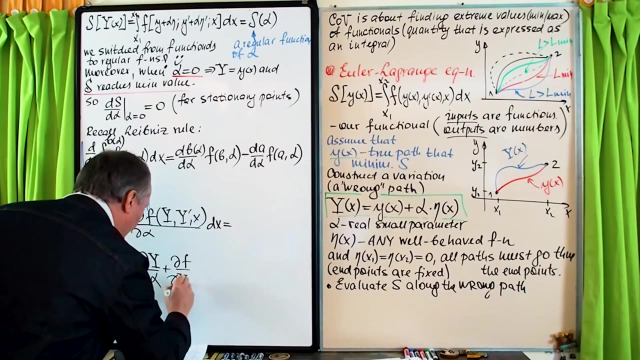 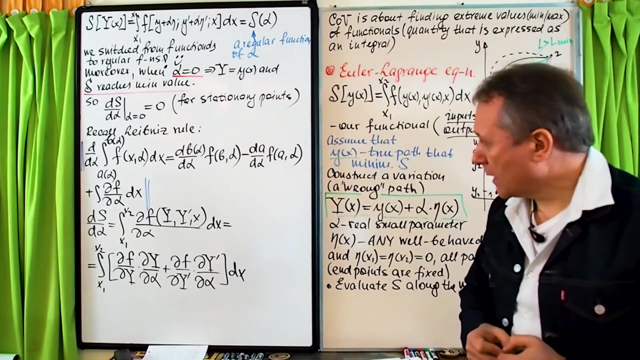 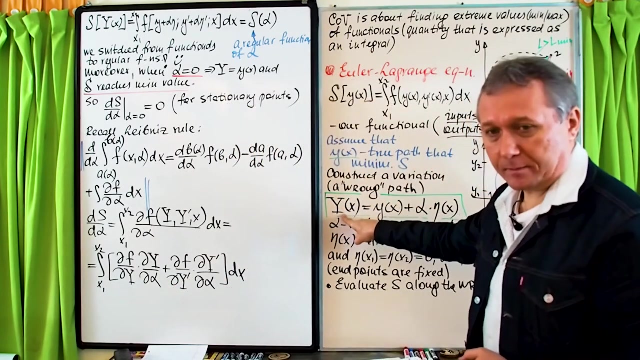 over d y capital, then partial derivative of y capital with respect to alpha right, this complex function, then plus partial derivative of F with respect to y prime and d y prime d alpha and dx. So the easiest part probably: d y capital over d alpha, So d y capital over d alpha. 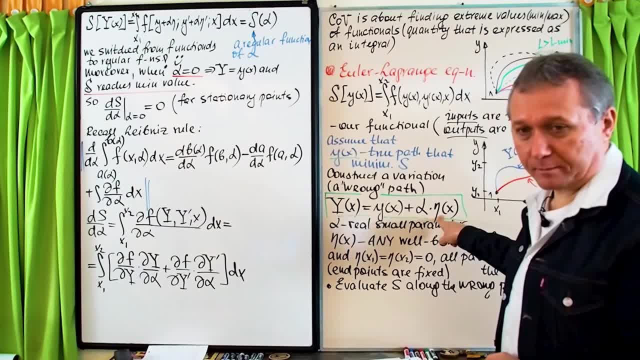 again partial derivative, It will be eta Right. That's why I framed it, because I knew that at some point I would have to search for that. so d y capital over d y, or y prime over d, alpha over the alpha prime, and巨 prime which equals 10 times d x. 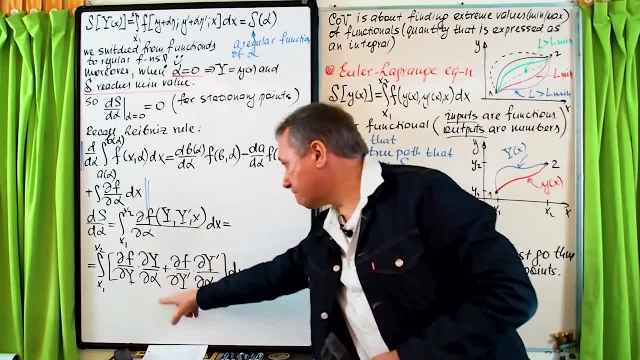 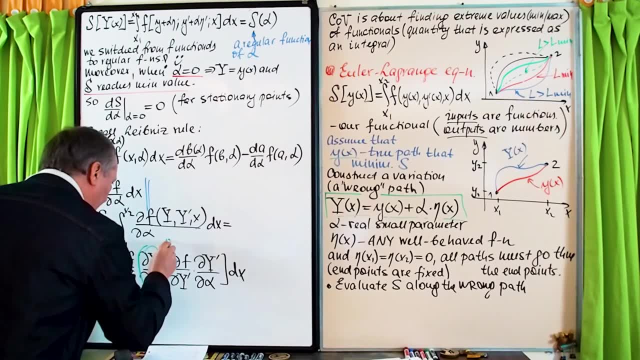 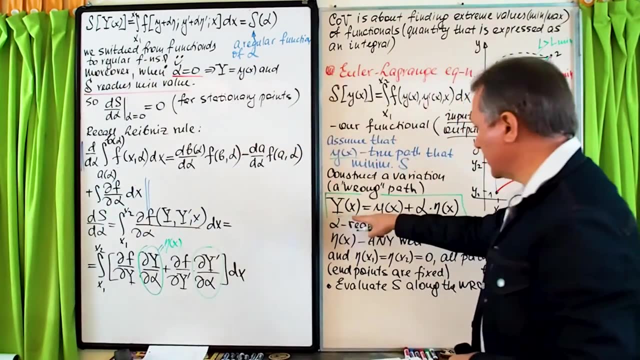 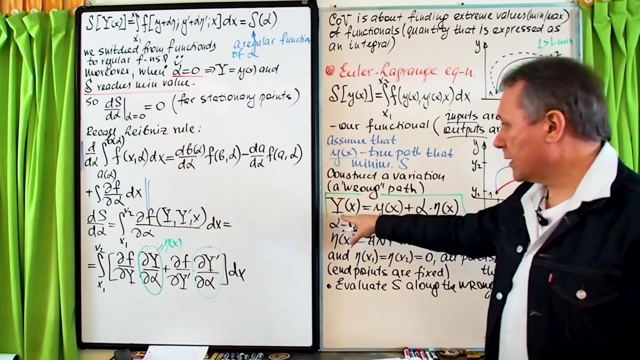 over dy, or y, d, d alpha, So just eta. So this is just eta as a function of x. Then this: if you differentiate this with, if you differentiate, if you take a prime right, prime, prime prime, So dy, prime over d alpha, again it's a. 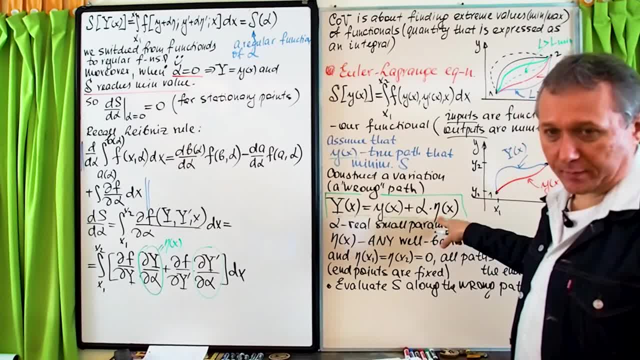 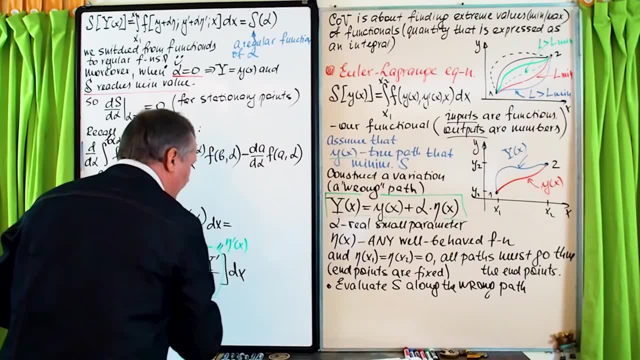 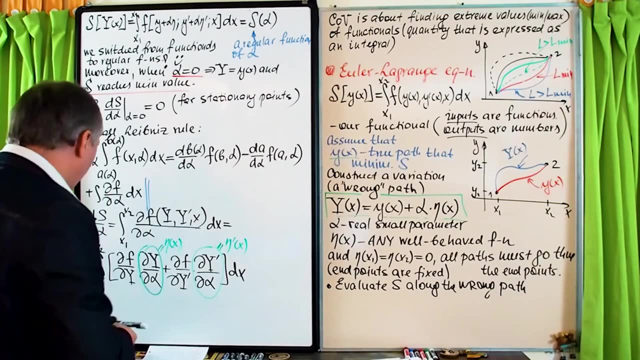 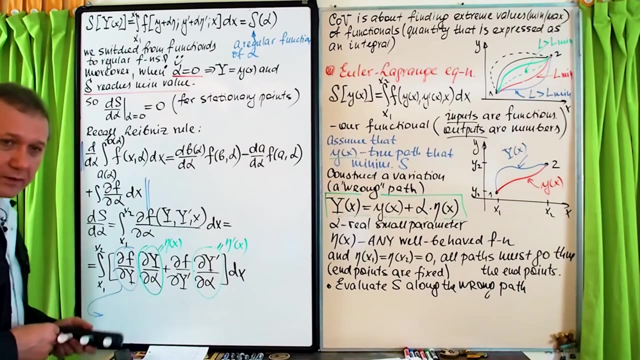 partial derivative. so you'll get only eta prime. Eta prime is a function of x. It's a derivative with respect to x prime. Okay, so now this dx over d, df over dy prime. Okay, so now let me take care of this term over here. 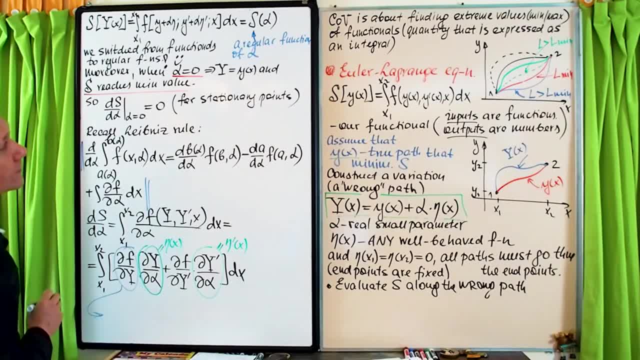 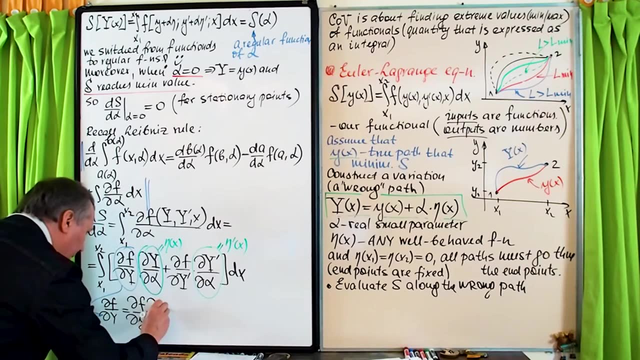 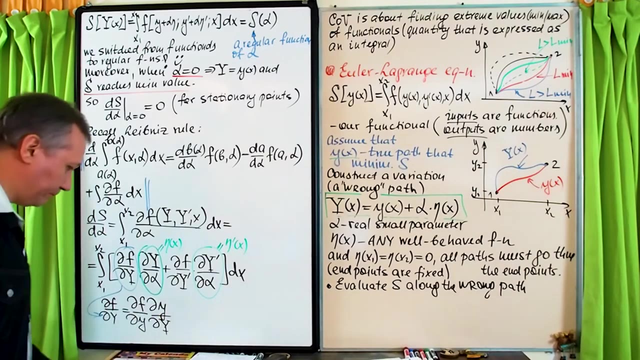 All right, So I hope I can squeeze it. All right, So df over dy capital. So I can write it like this: df over dy small and then dy small over dy capital. All right, So now dy capital. 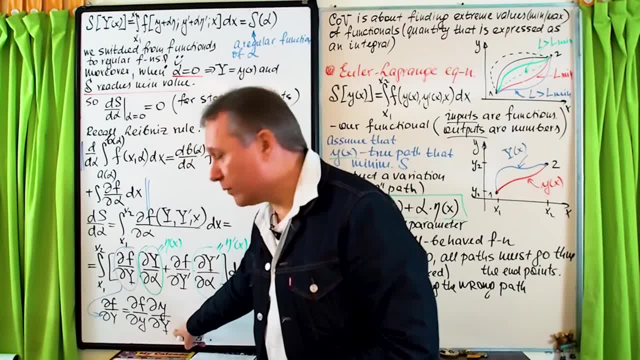 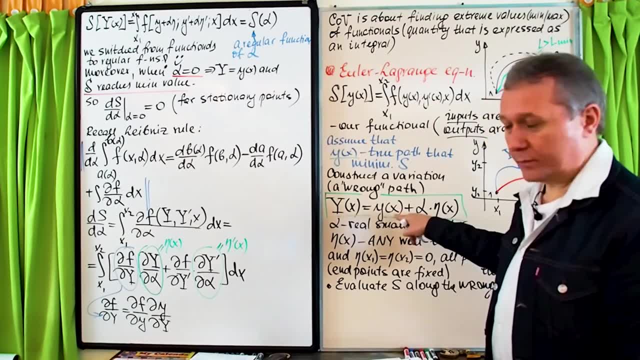 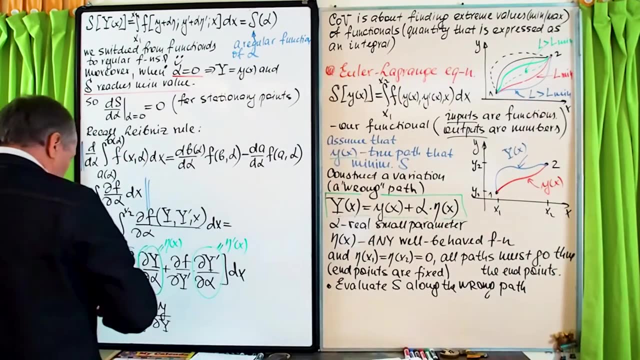 Well, again, partial derivative with respect dy small over dy capital right Again, look at this: y small with respect to y capital. it will, you will get one partial derivative right, So it will be one. So this is just one. 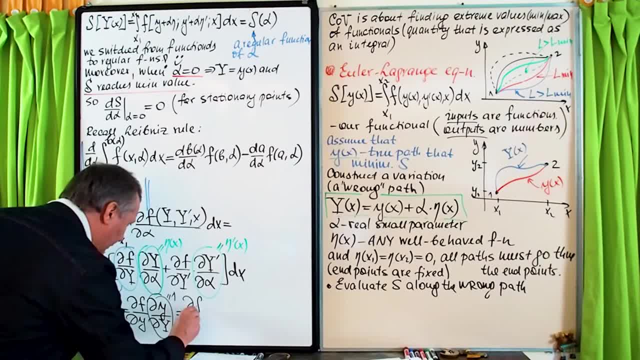 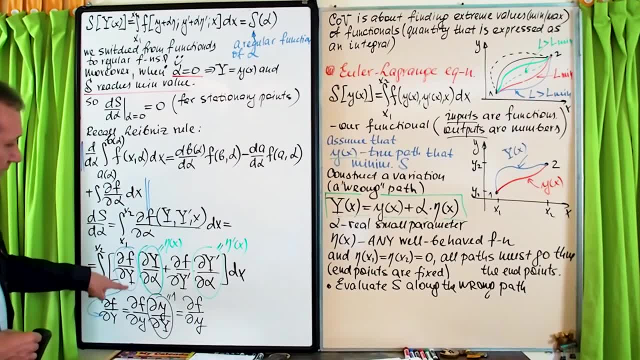 As a result, this is equal to the partial derivative of f with respect to y. So this is df over dy small And very similar. this will be df over dy small, right? So here it's exactly the same. 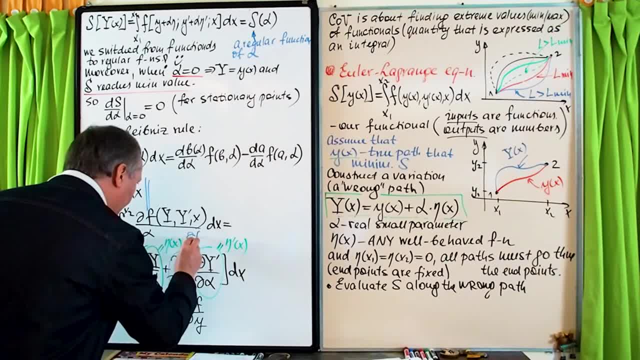 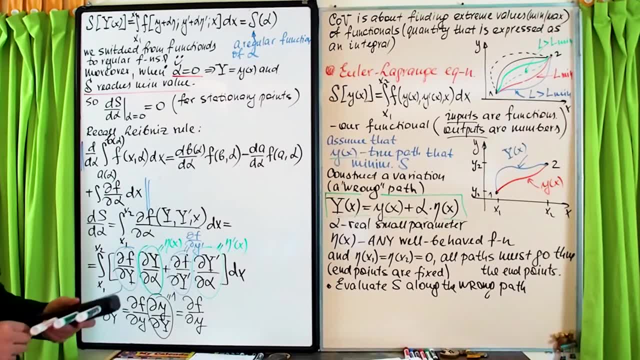 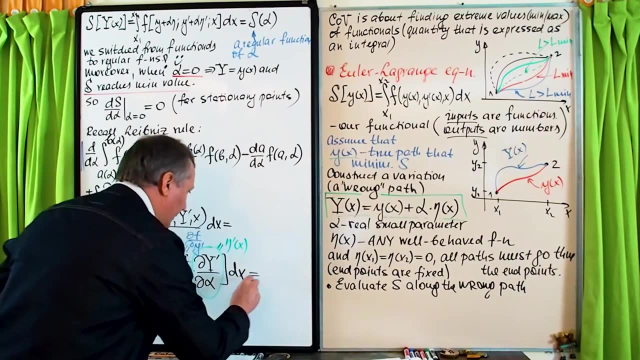 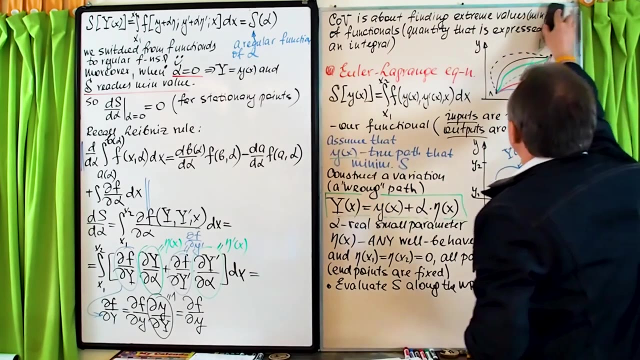 So this will be equal to partial derivative of f with respect to y prime: Yeah, y prime. Okay, so now let's rewrite. Okay, So let's rewrite it over there with all these replacements, All right, Yeah, I think I can erase this. 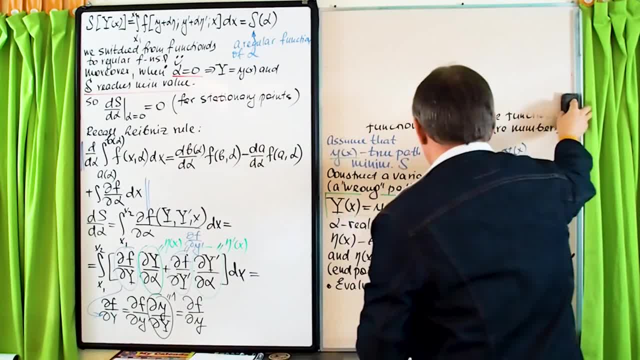 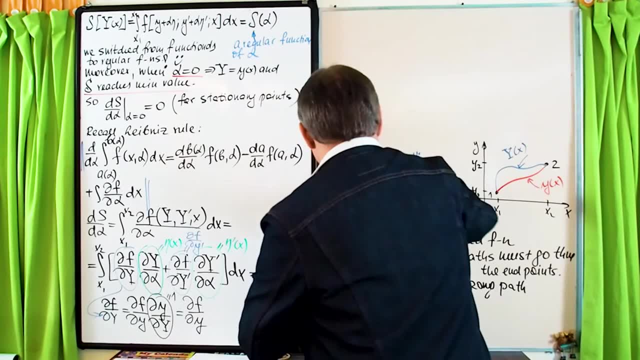 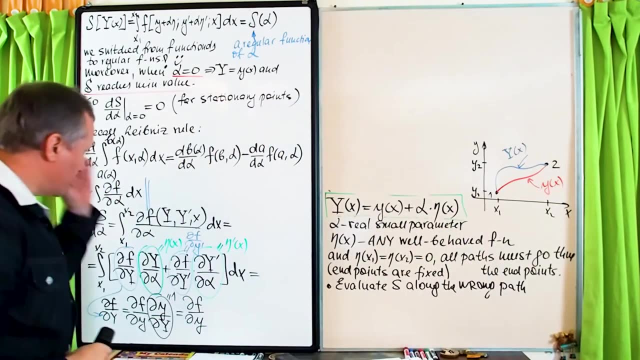 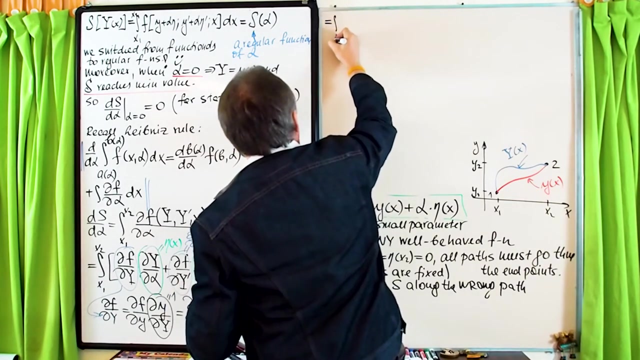 Okay, up to this point, I still need probably try to keep the picture as much as I can- And this Variation: Okay, so let's rewrite it So it will be equal to integral from x1 to x2.. 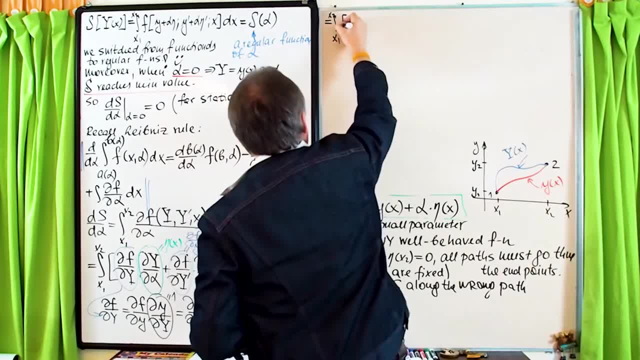 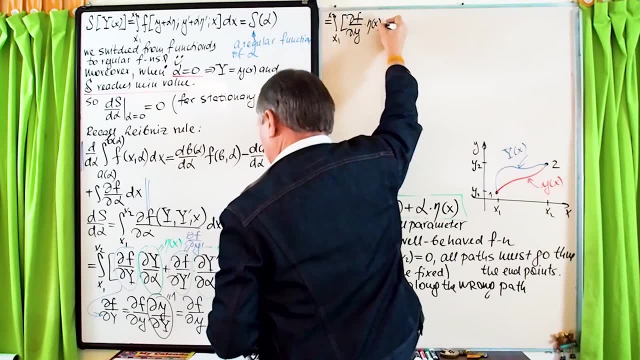 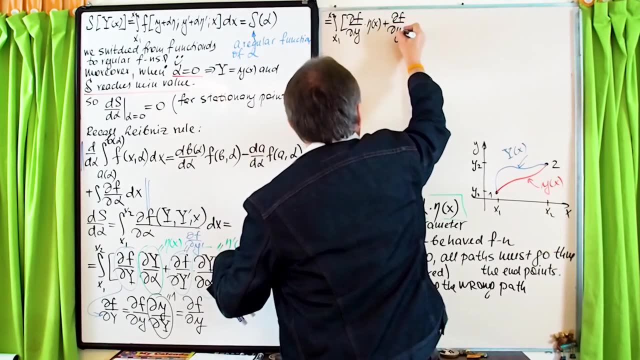 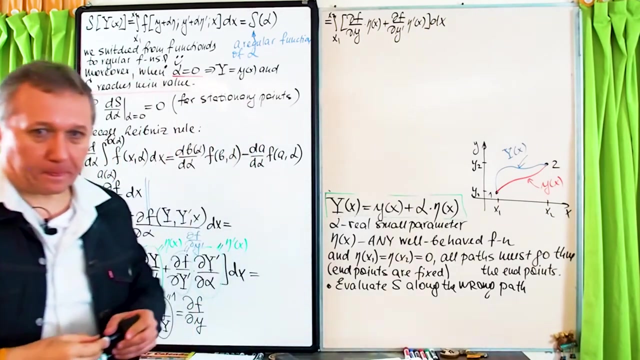 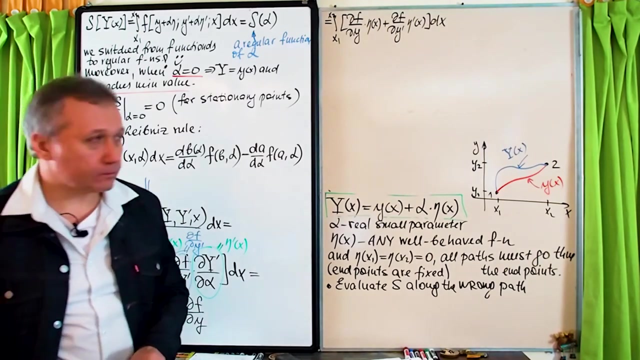 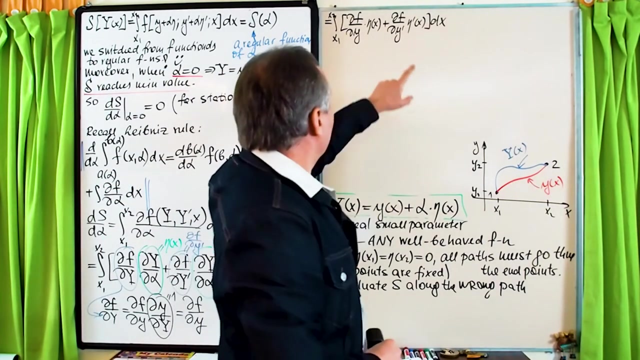 This is okay. df over dy eta as a function of x. Then plus, This is df over dy prime, eta, prime as a function of x and dx. Okay, almost everything looks great, except for eta, eta prime. Let's get. 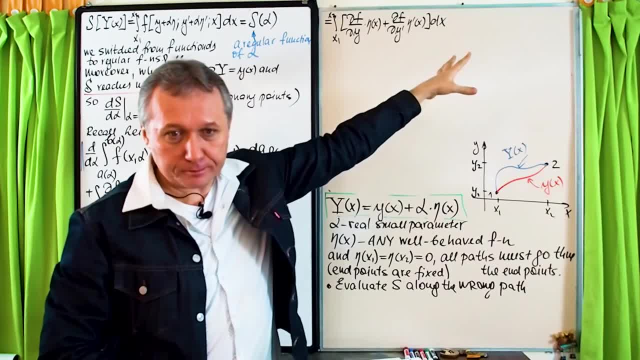 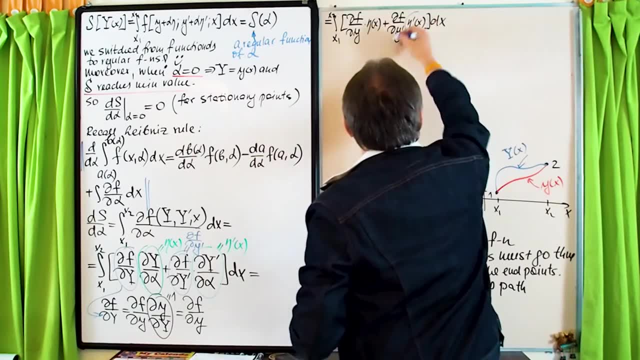 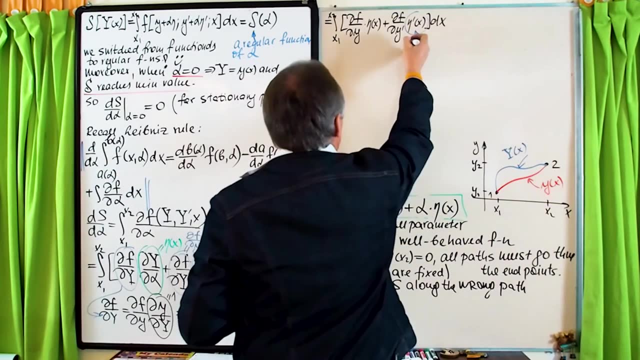 Let's try to get rid of that prime in the second term, right? So let's take care of that prime. So, in order to do that, of course we can integrate by parts the second integral, right? So let's take care of that here. 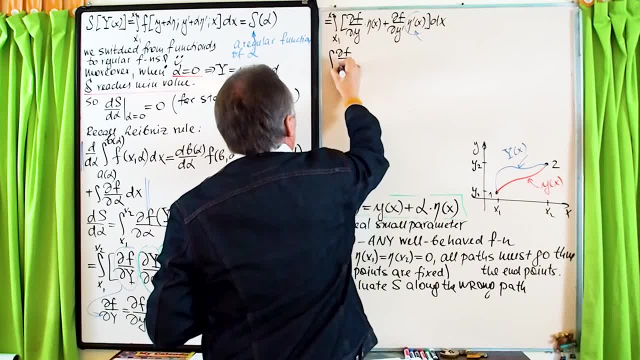 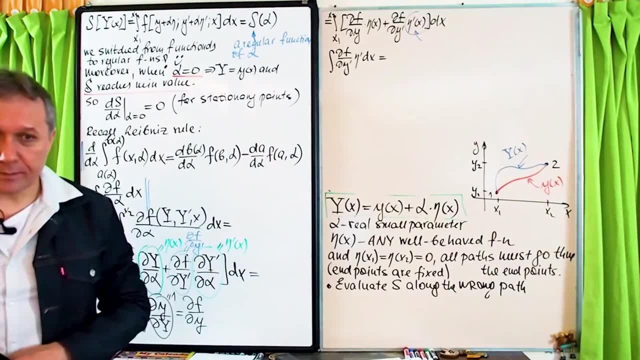 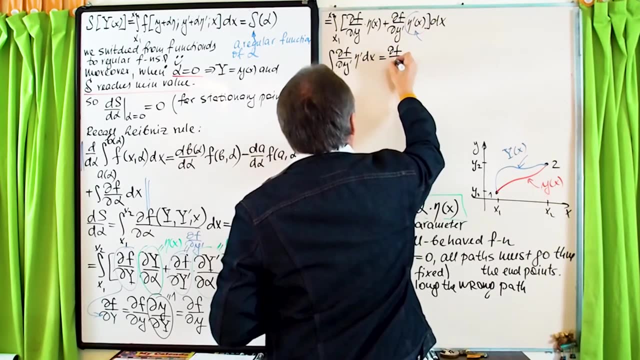 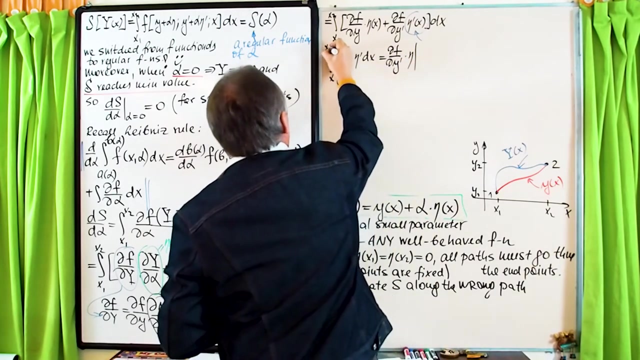 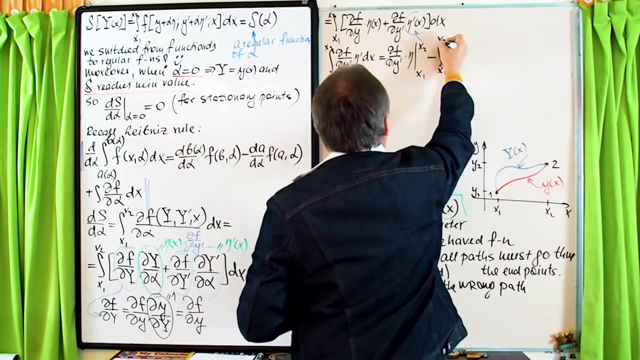 So it's integral of df over dy prime eta prime dx. Of course it will be equal Just by parts. So it will be df over dy prime eta right And limits x1, x2 minus integral from x1 to x2.. 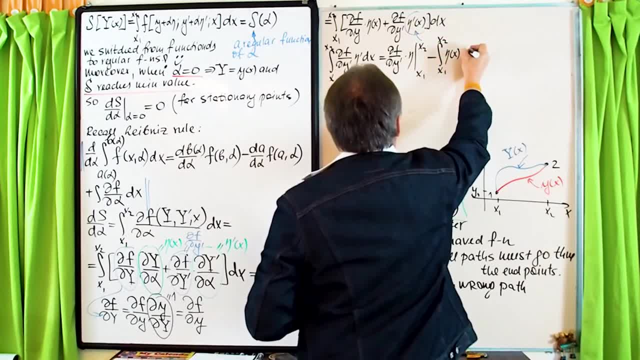 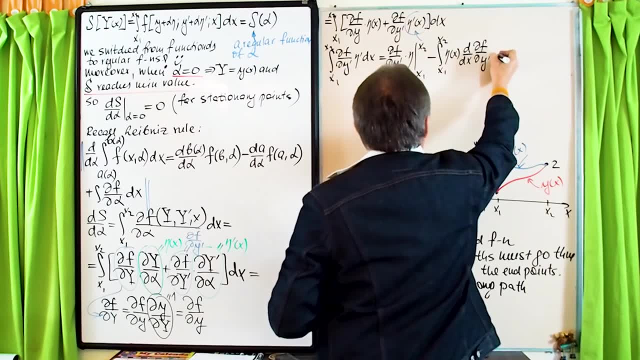 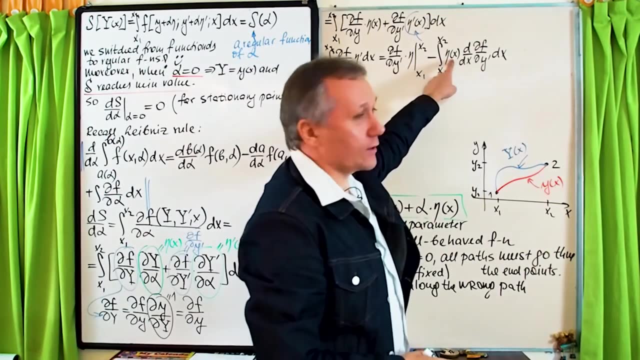 And now it will be eta as a function of x And we will have d over dx, Partial dx It's a derivative of f with respect to y prime, dx Prime it's a d over dx. So here now we have function eta without derivation. 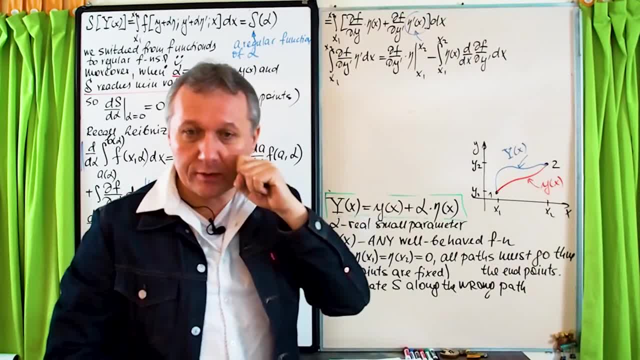 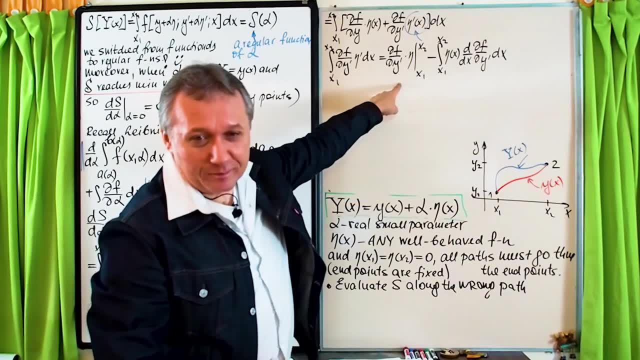 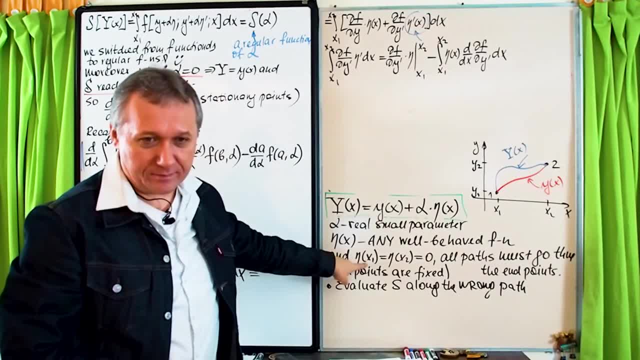 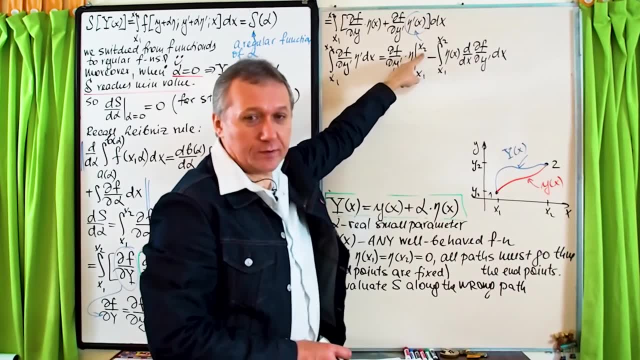 Eta, Eta. It's an arbitrary function and we demanded this. The value of that function at the end points must be zero. So eta at x2 is zero and eta at x1 is zero. So that is zero. 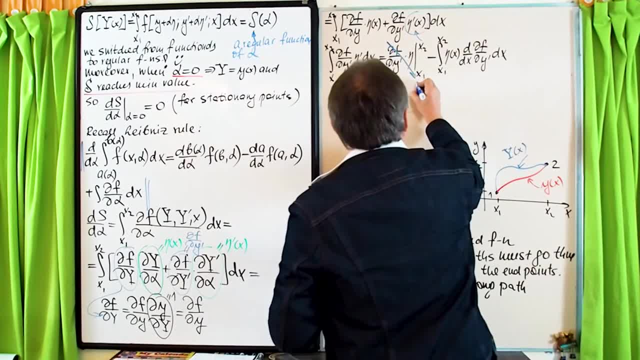 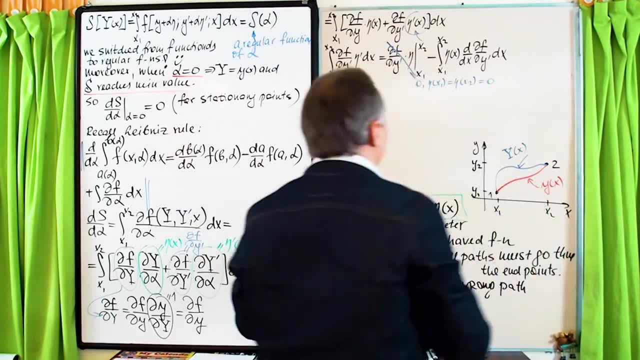 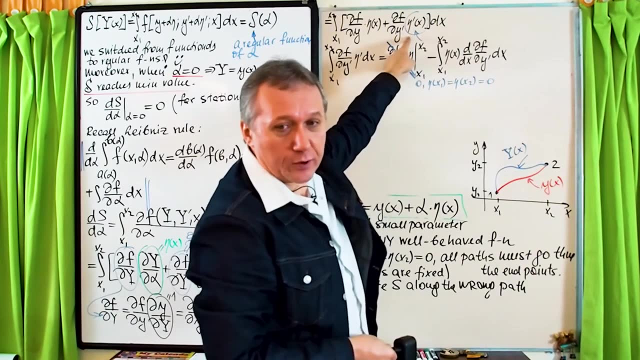 So let me dump this. So this is zero, since eta at x1 equals to eta at x2 equals to zero. So, as a result, we have only that integral And now we have eta here, so we can bring it back to this expression and this eta, and 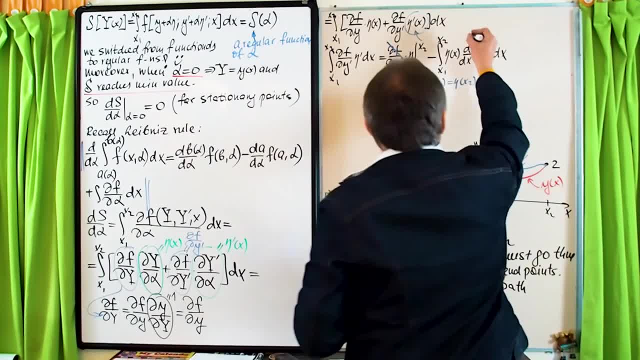 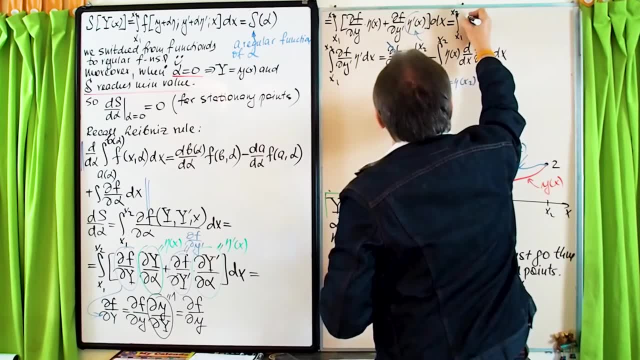 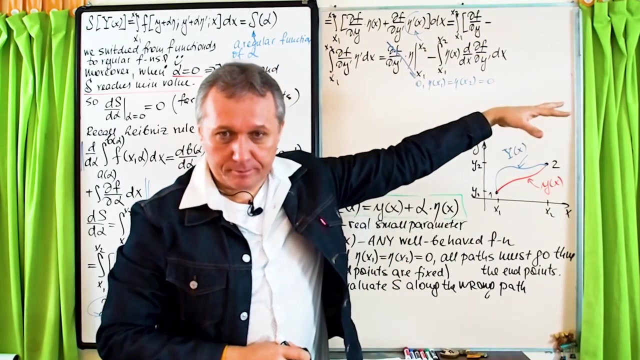 this eta can be factored out. So now let me continue this. It will be integral from x1 to x2.. So first I will write this partial derivative of f with respect to y, Then Then, Then eta will factor out. 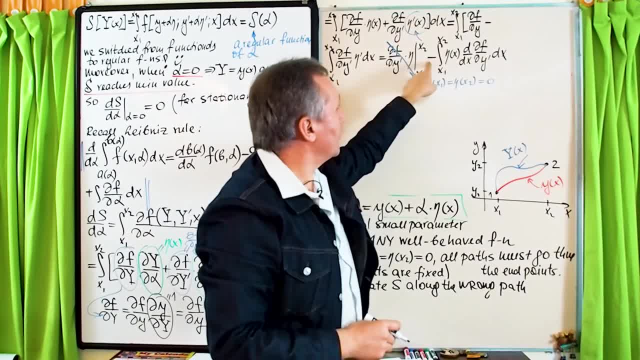 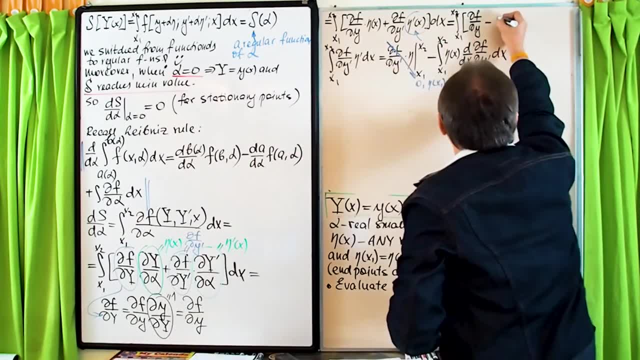 So that's why I didn't write this eta. So now let me write this. So it will be minus d over dx, df over dy prime over here. So it will be minus d over dx partial derivative of f with respect to y prime. and now eta. 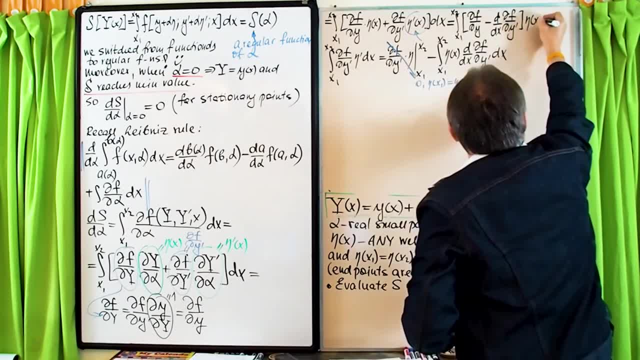 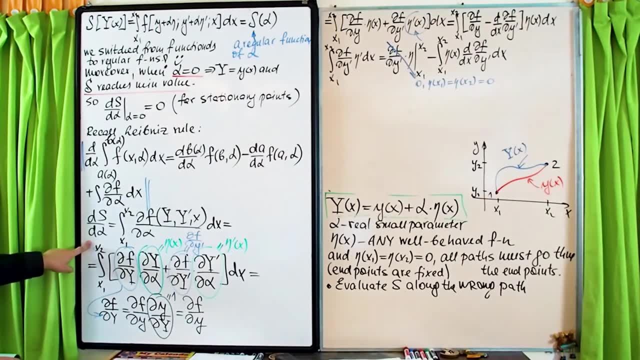 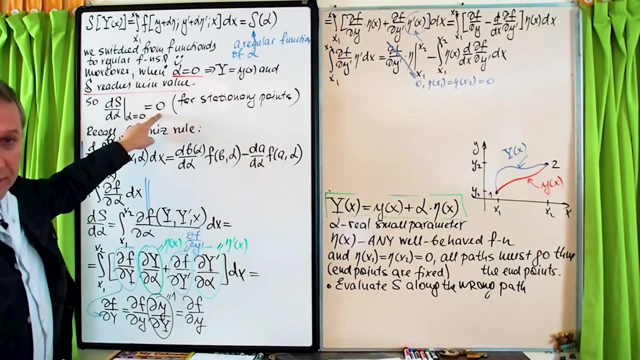 Eta here, eta there. So eta is a function of x, dx, Whoo And again. so what? We started with dx over d alpha, all right, from ds over d alpha. And this ds over d alpha is zero, all right. 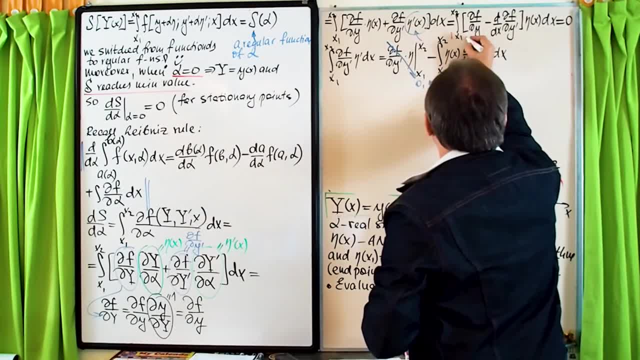 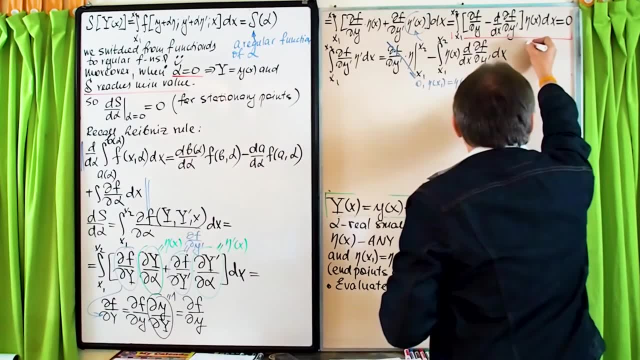 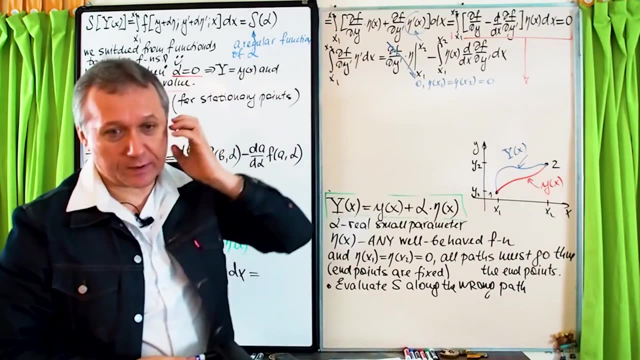 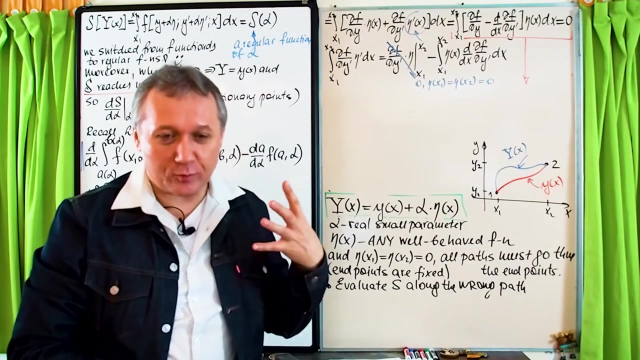 So now we need to look at this carefully, right? so this part- Okay, let me show that I am going To move over here. I mean, get the conclusions out of that expression, all right. So obviously you see that what we need to get, 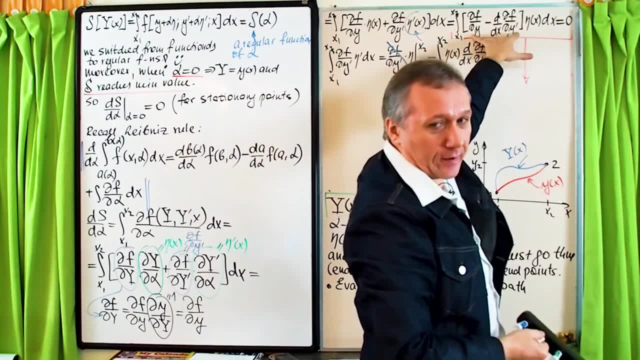 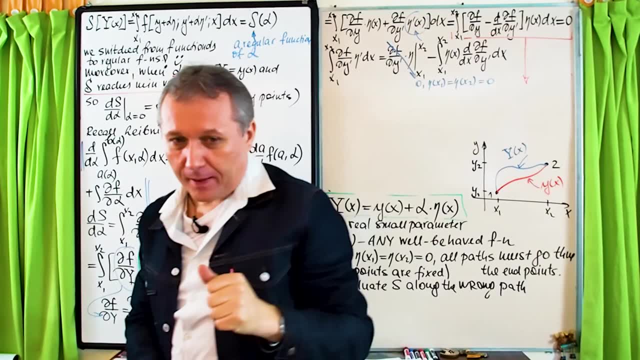 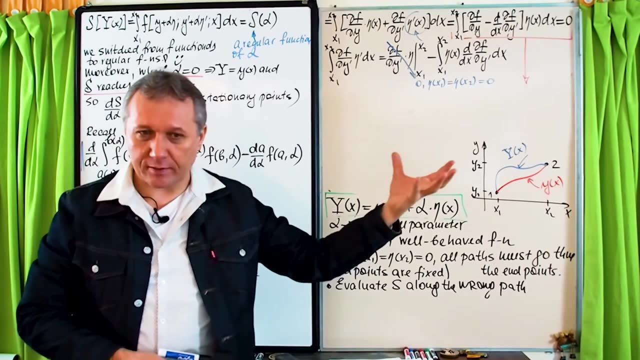 We need to take this bracket, extract it and call it zero. right, Because it equals to zero. But but which magic words do we have to pronounce a say first before we can? We can extract that bracket and call it zero, and that will be our Euler-Lagrange equation. 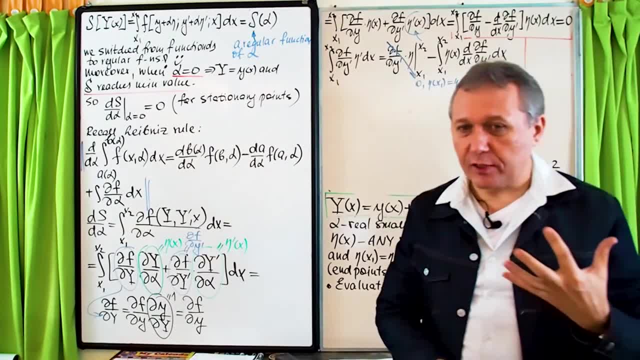 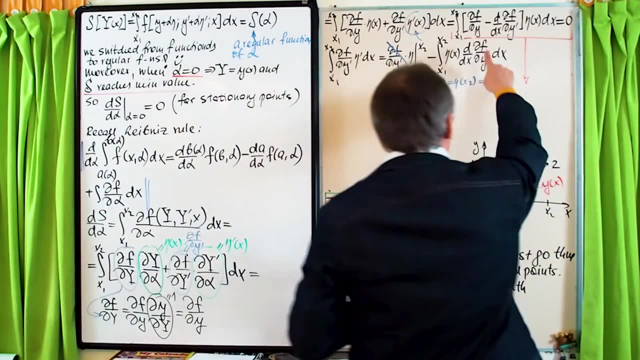 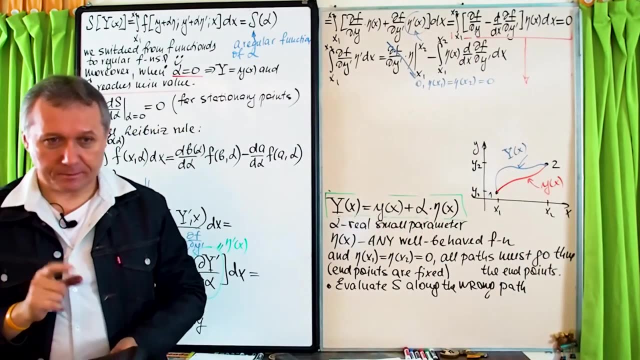 From the mathematical point of view. this must be justified. this extraction of that bracket, of that integral, Why can we take this bracket and call it zero? And the key word is: you see what I wrote. I even capitalized Our function, eta. 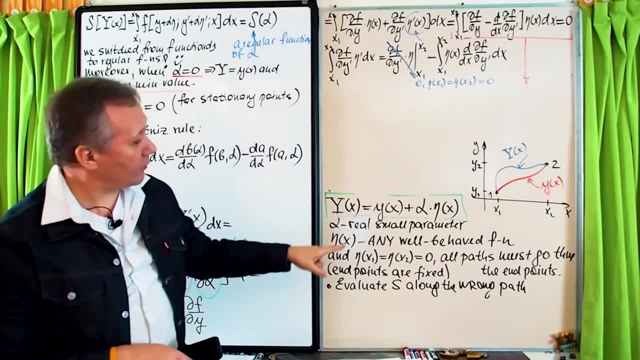 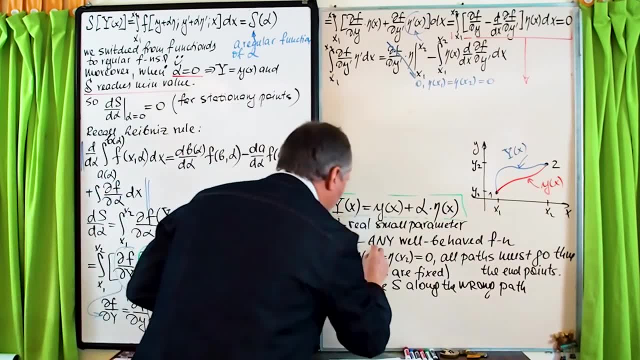 Our function eta, Which is over there, you see, just outside of the bracket. Our function eta is any, a well-behaved function, but still key word is any. It can be sine, it can be cosine, it can be tangent, it can be exponential, it can be. 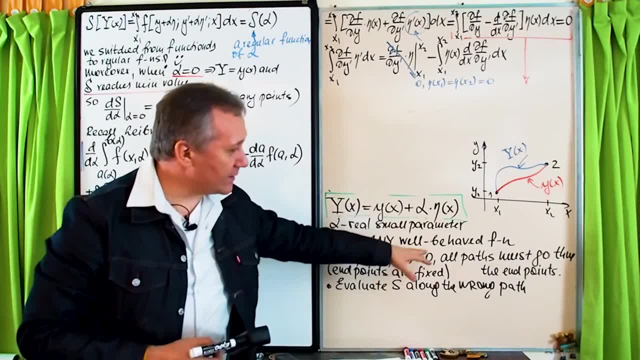 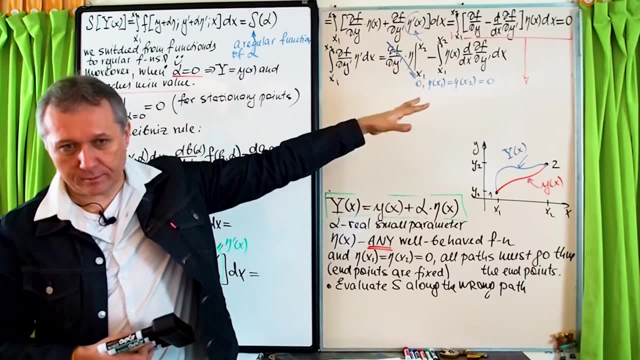 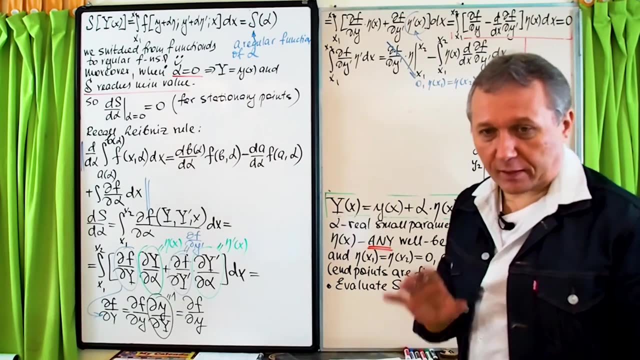 basically any function, of course, if it satisfies this and well-behaved. So if that must be true for any eta, it means that this can be correct Only when this bracket is zero. So right now the key word is: any right. 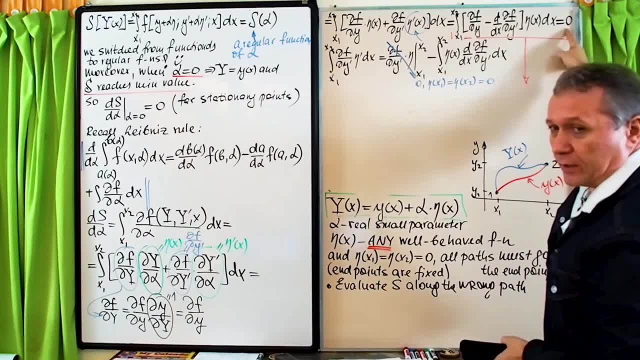 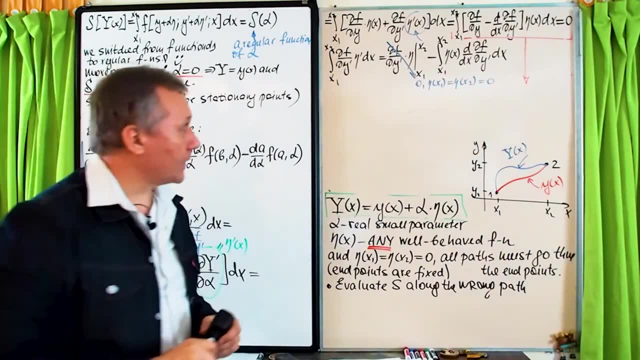 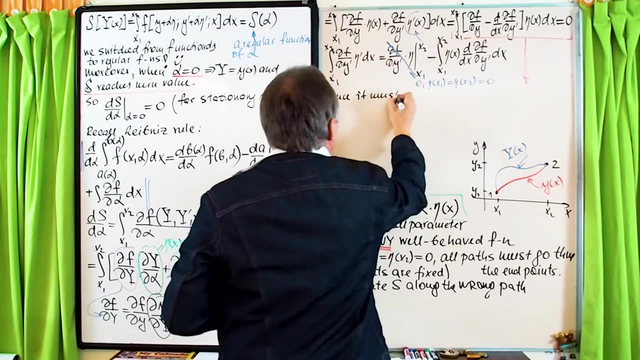 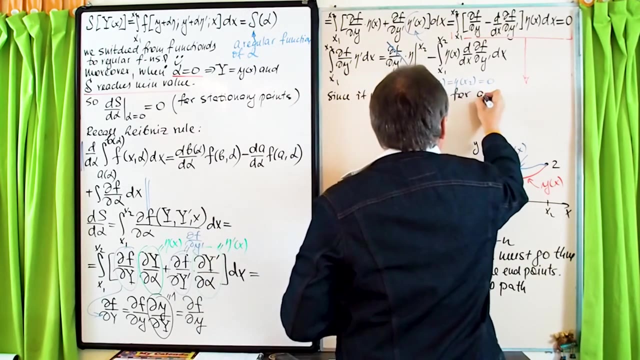 So it must be true, It must be equal to zero in any for any eta. So it means that that bracket must be equal to zero. So, okay, let me write, Since it must be zero For any eta as a function of x. 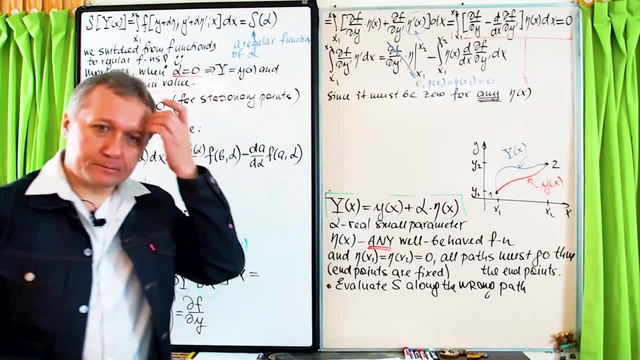 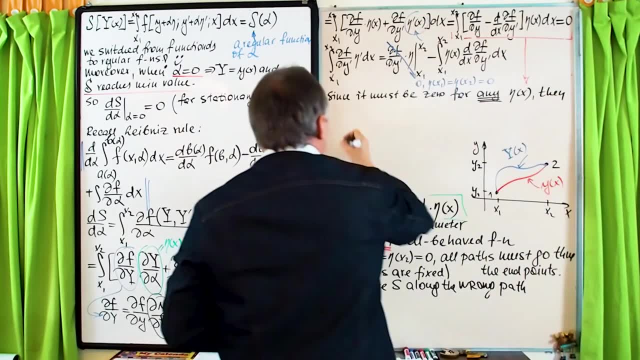 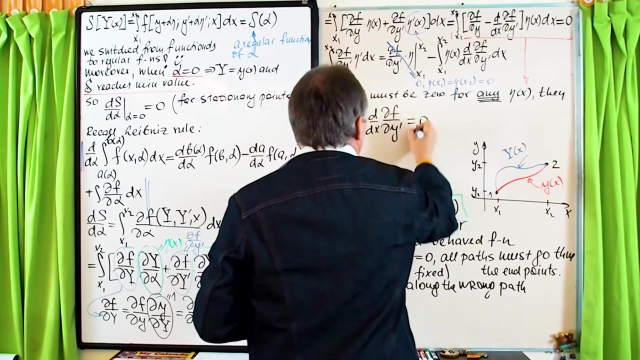 Again that I'm analyzing this right For any, Then where we can extract that So we can write: So: partial derivative of function f with respect to y minus d over dx out of partial derivative of f with respect to y, prime equals to 0.. 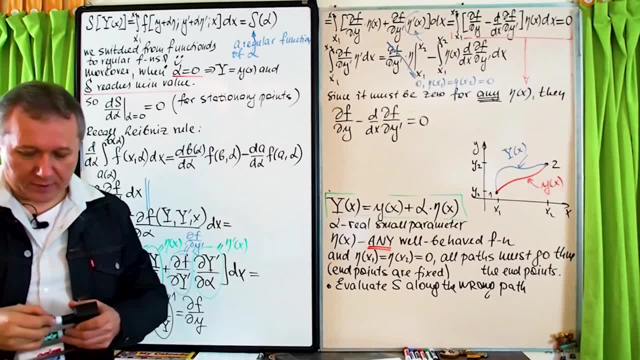 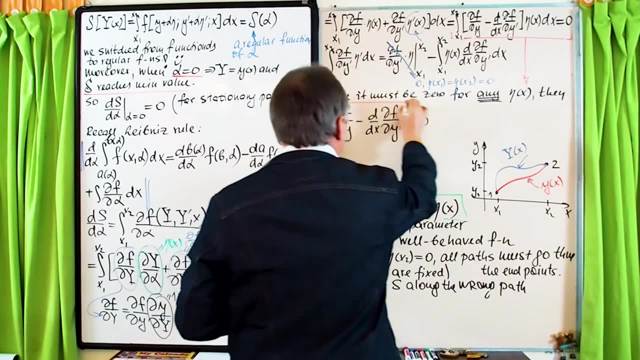 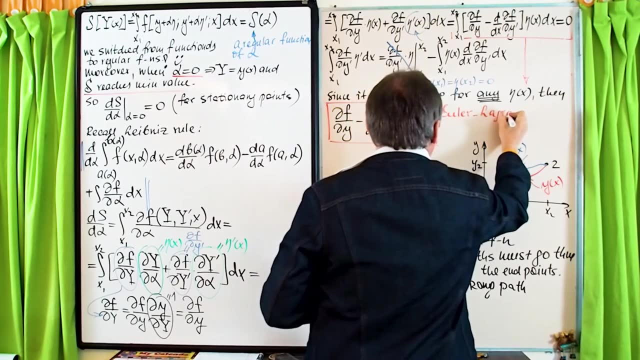 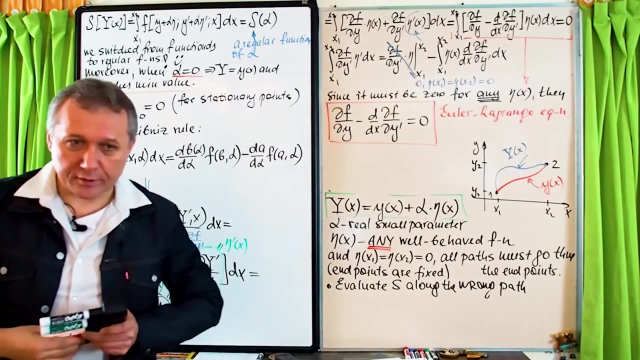 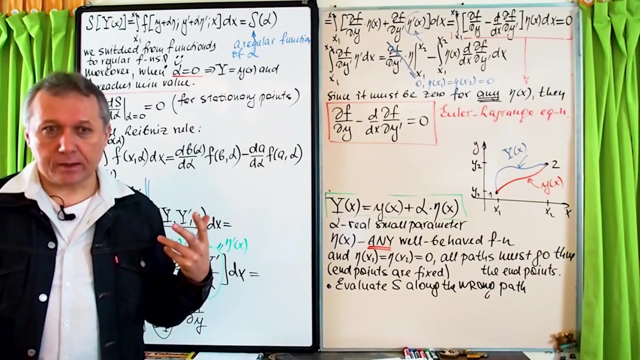 So this is the tool. This is Euler-Lagrange equation. So let me frame it: It's a second-order differential equation. So what is an output of this differential equation? second-order, It's a function eta. Oh, you ate. 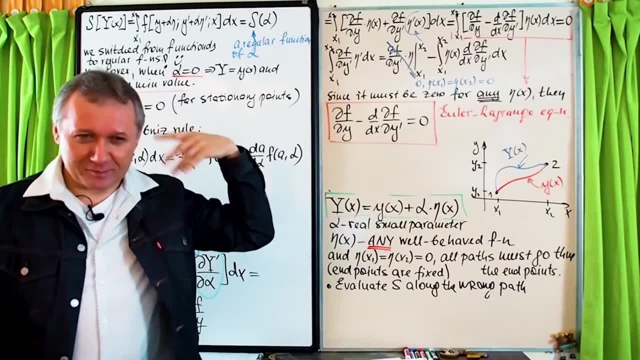 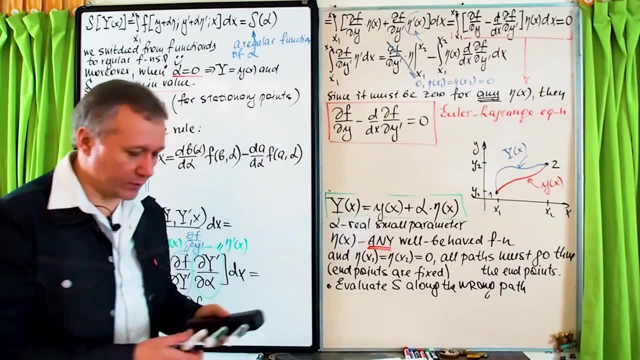 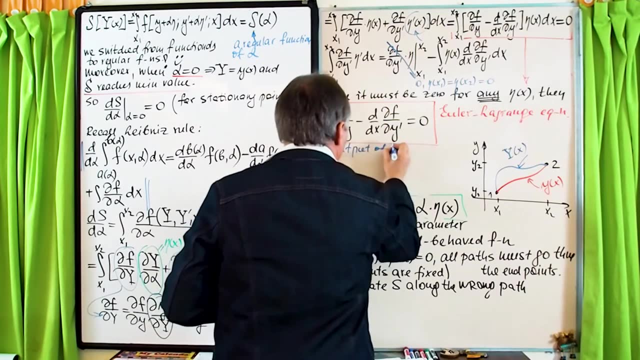 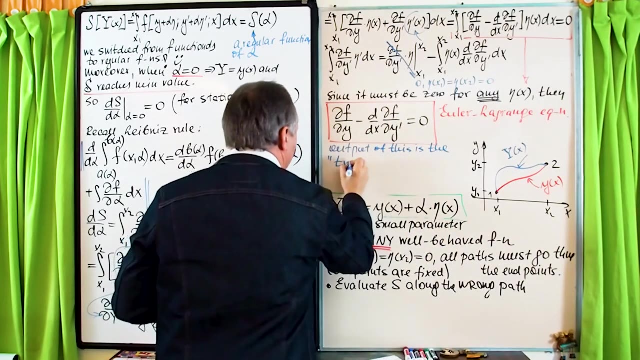 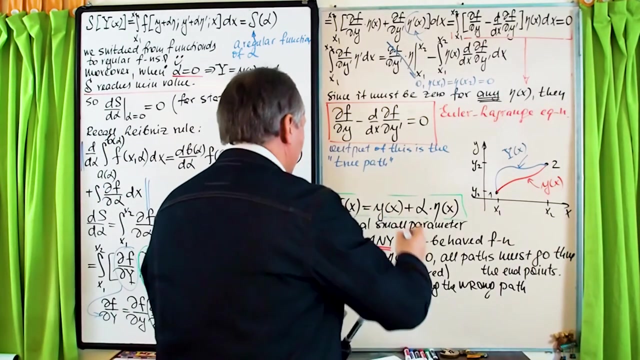 Damn it. I've been pronouncing eta so much. So function y. y is a function of x, which is the true path. So the output of this is: is the true path to the true love right, Which is y as a function of x. 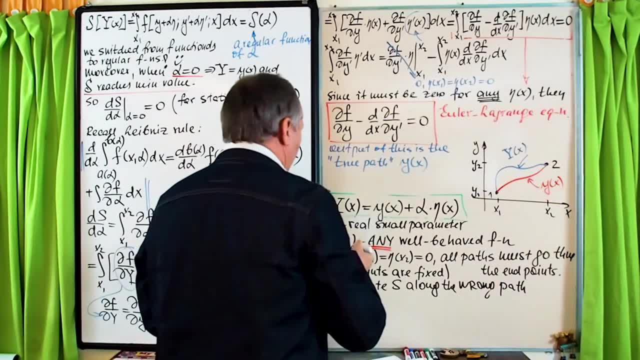 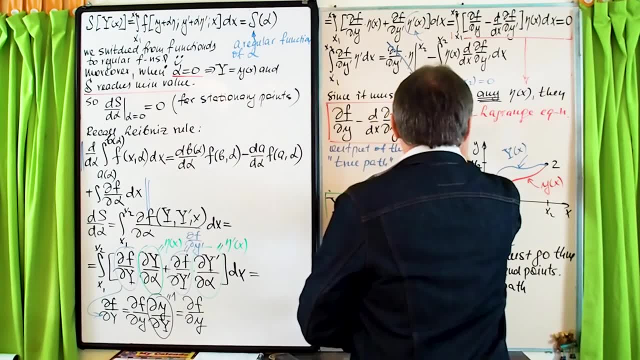 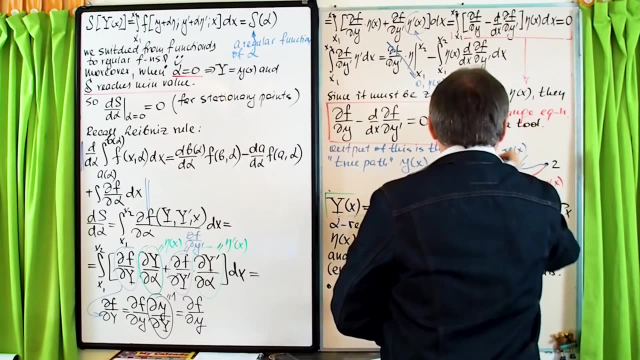 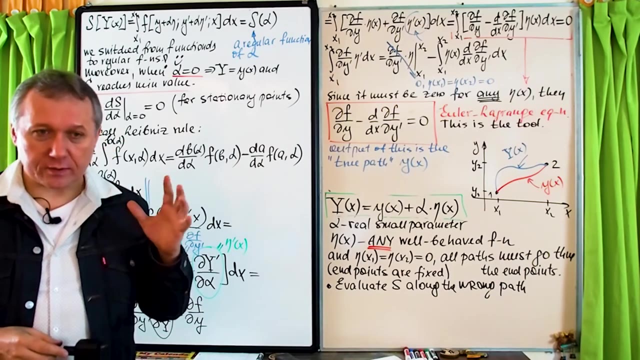 So that is the tool. Okay, So, okay, let me write. So this is our tool, This is, this is the tool which allows us to find the true path, which is going to make Okay. and now I have to again emphasize on this. 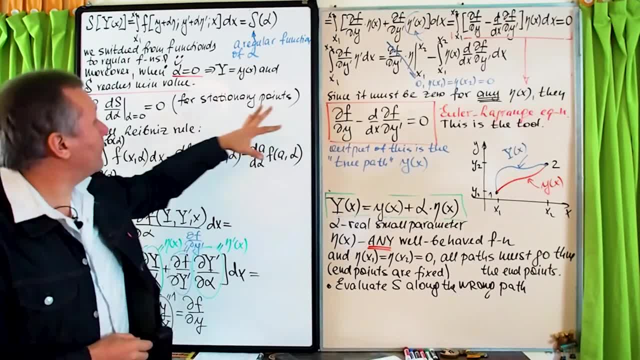 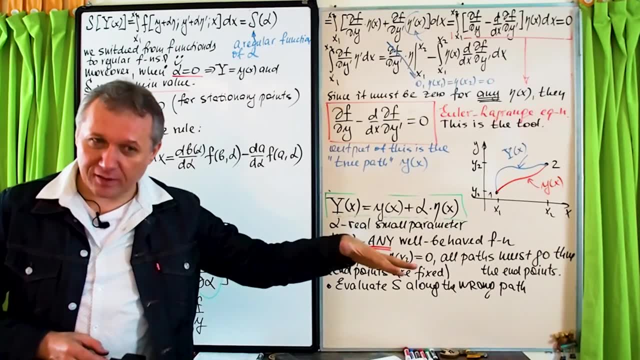 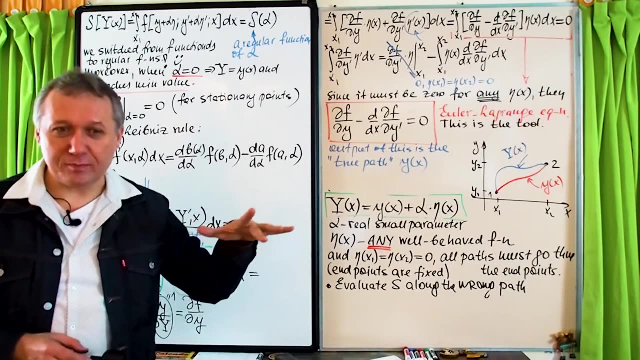 This condition is not going to guarantee that our integrand s reaches minimum. It can guarantee that it will be stationary, So it can be min, can be max, But in all the problems which we are going to discuss it is going to reach minimum value. 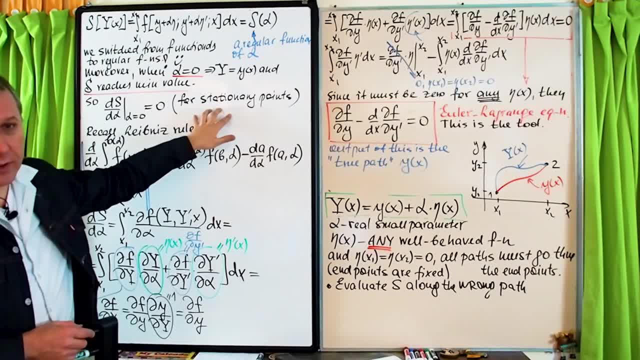 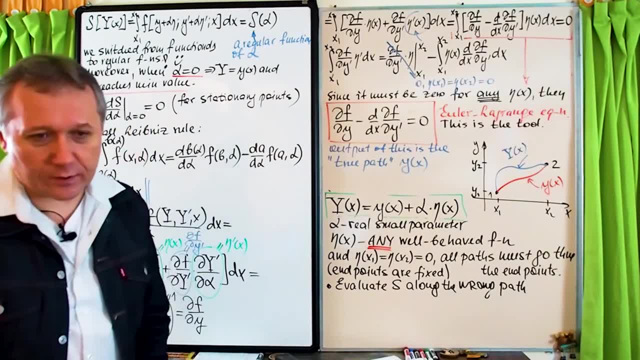 Because, again, we just use the stationary condition Condition for stationary points, So that equation cannot guarantee that we are going to reach Functional. Functional is going to reach minimum. It can be minimum, It can be maximum. There are some situations where 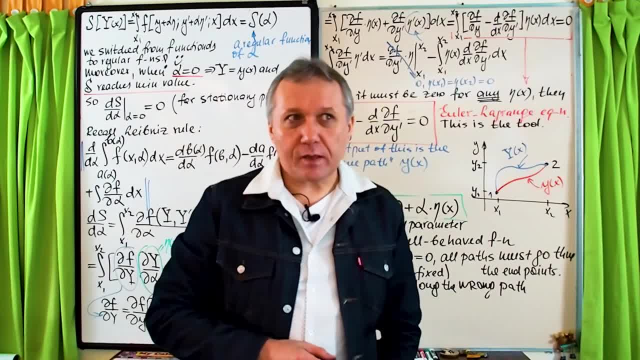 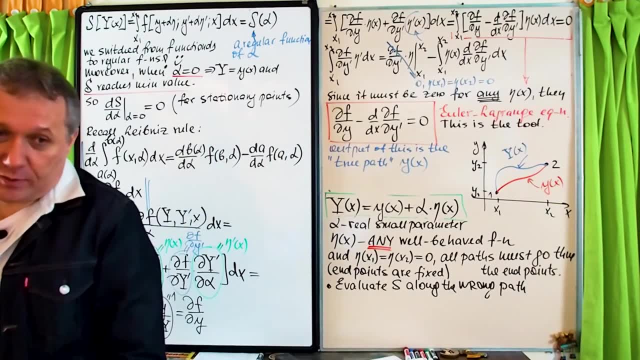 If you want to, If you deal with money, with profit, of course you don't want to minimize your profit, right? Of course you want to maximize. So sometimes there are situations where you have to maximize something right. 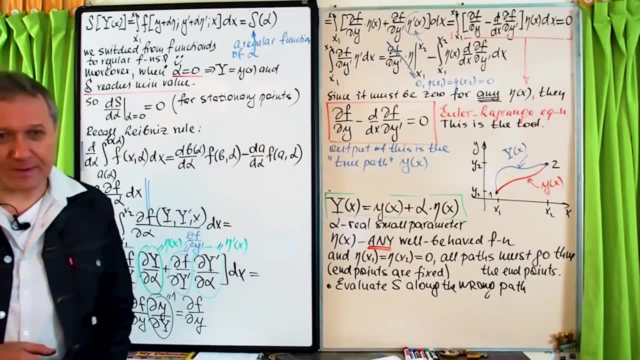 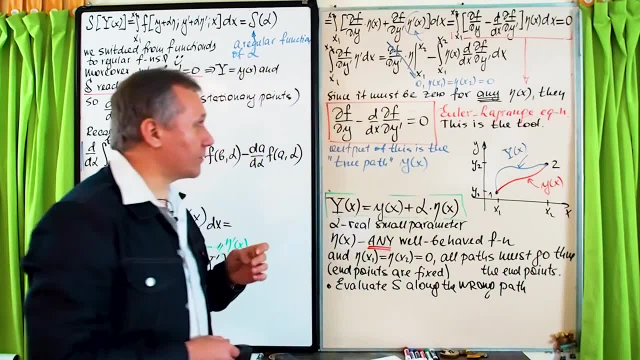 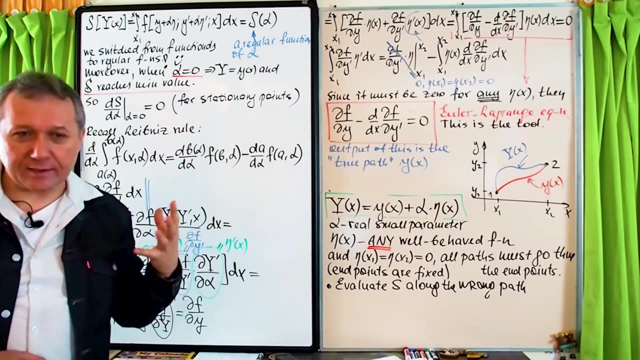 You might want to minimize your expenses, right? Okay, so this is the Euler-Lagrange equation And, of course, when we get to the Lagrangian formalism, this equation will be reused. We will slightly adjust it and that will be our Lagrange equation. 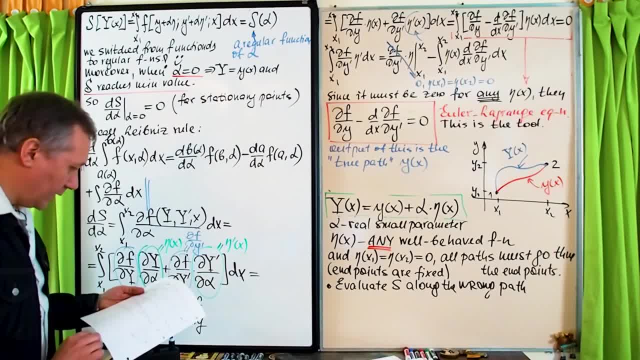 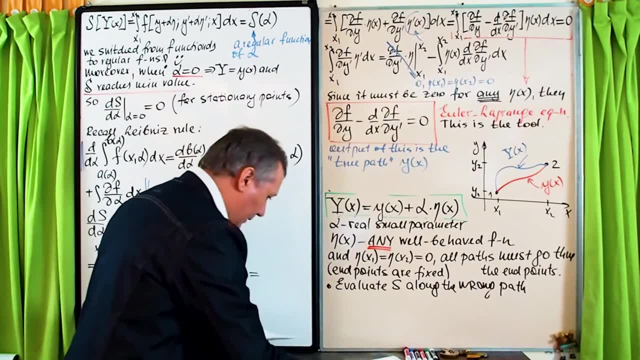 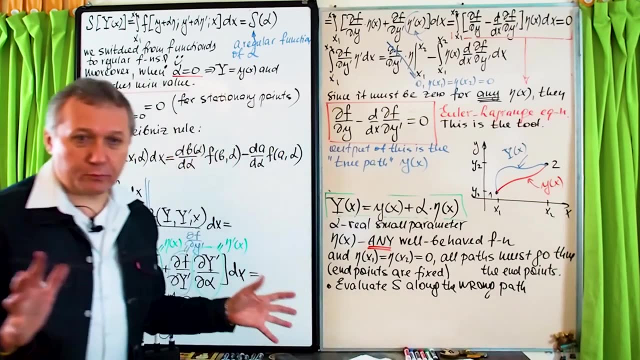 Okay, let me check if I mention everything. Let me quickly. All right, Ah, yes, So now what's the procedure, How we can address problems of this type. So first of all, you need to state the problem. 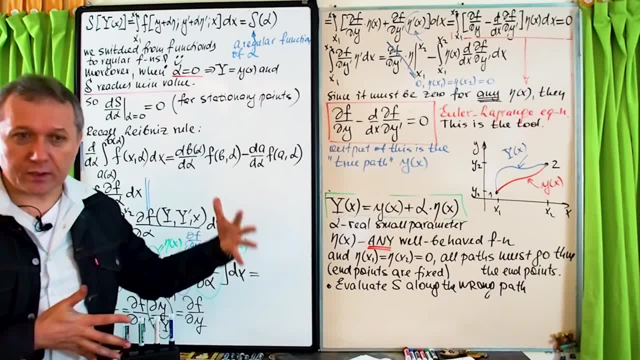 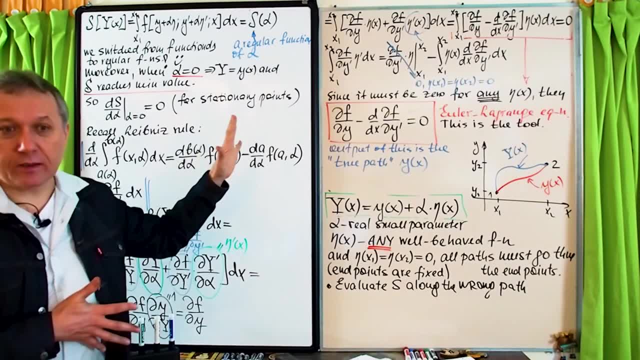 Like we stated those two examples at the very beginning, right The shortest distance between two points, or Fermat principle. First you need to write those integrals, Which What do we call now functionals? First write them down. 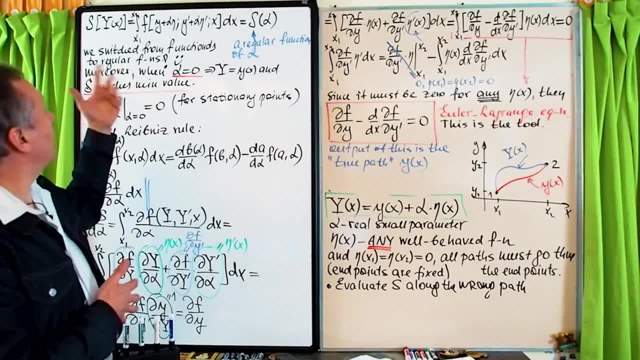 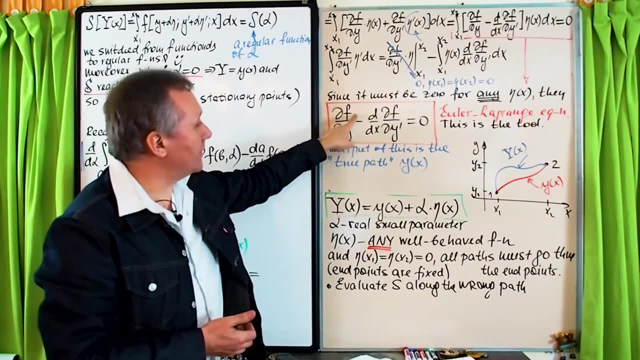 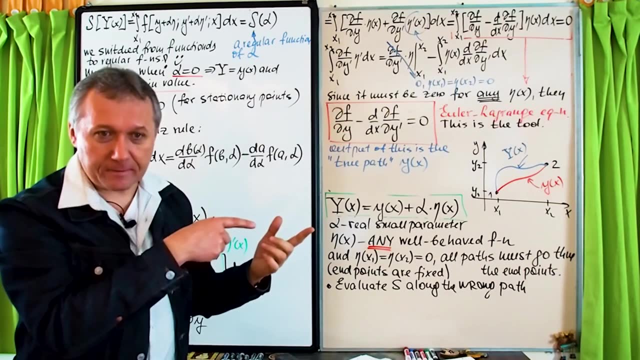 Then, inside of the functional, inside of the functional, that integrant, that integrant, that's what function F is. That's why now I regret that I don't have that original functional right. You remember, we have S right. 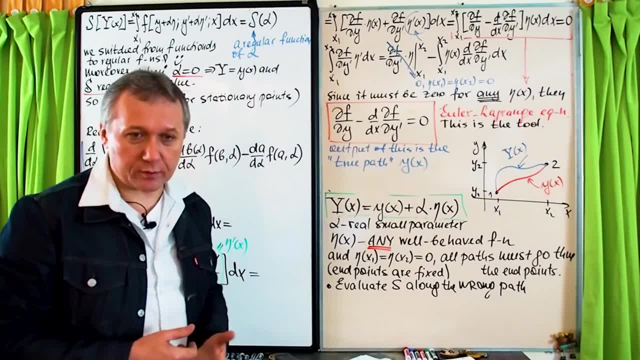 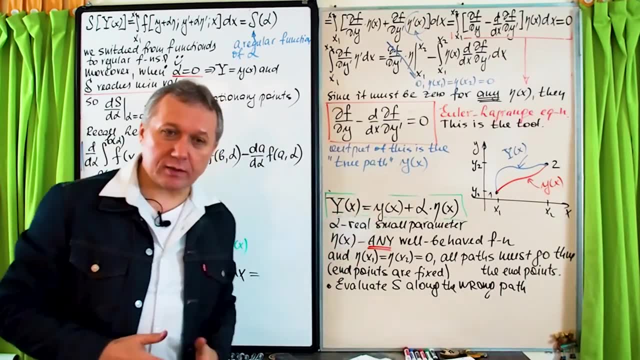 And that function F. you can. you have your notes right, You can see. you can look That function F is the integrant And that functional. So write down that integral which is functional. Look inside of the integral. 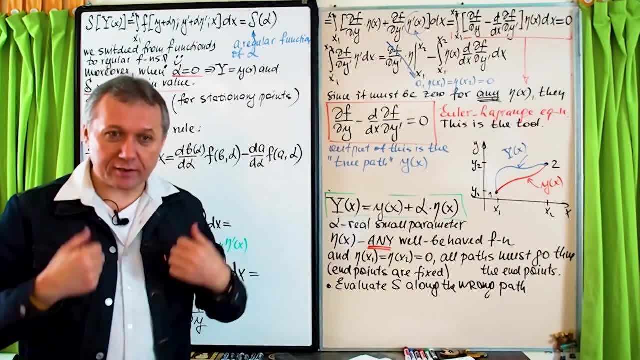 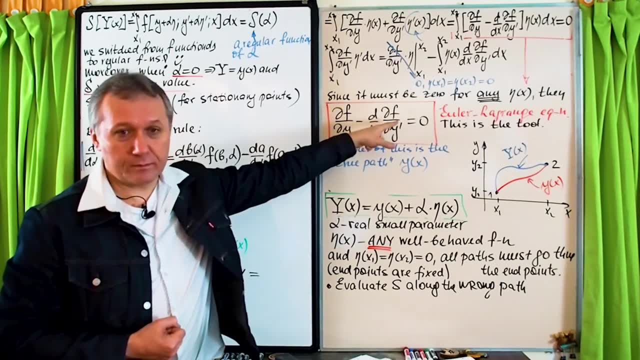 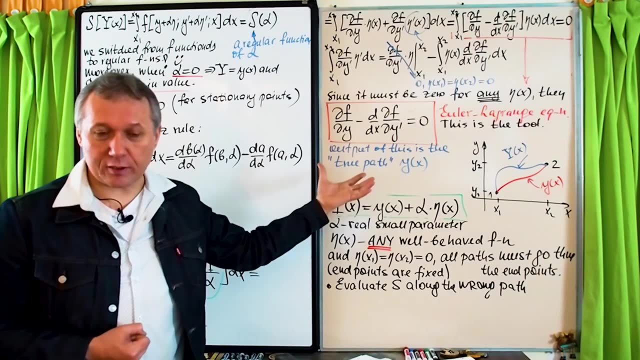 That function F is an integrant. Extract it from there And plug it into this Euler-Lagrange equation F And start differentiating. First you differentiate And then, of course, you will start integrating. Once you solve this equation, once you integrate it twice, 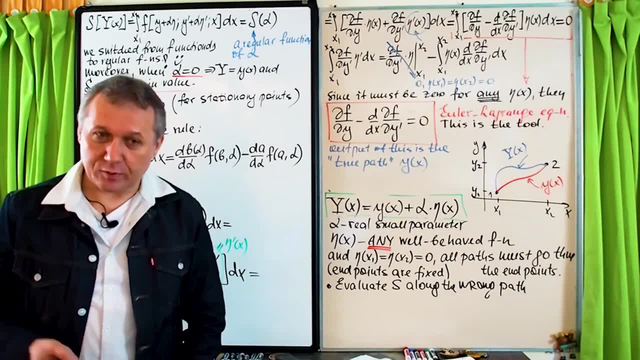 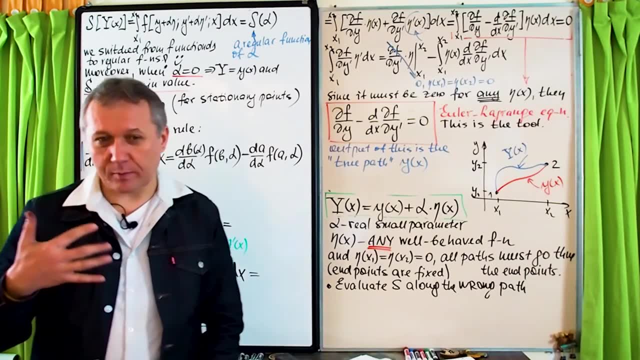 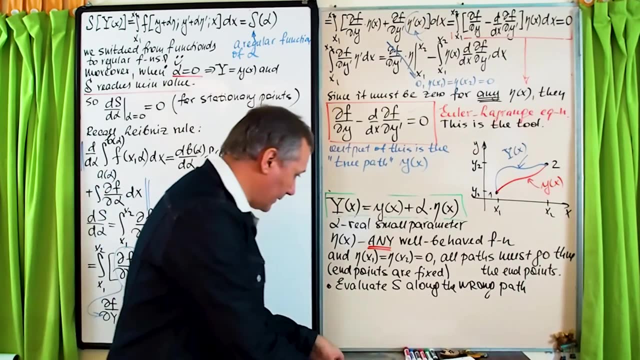 you will get the true path Which is going to make your functional stationary, But again, most of the time it will be minimization. Okay, So that's the procedure again, And now let's finish our first example, which we stated and I promised that we are: 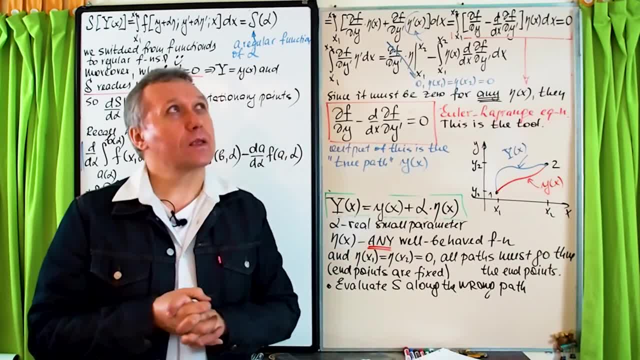 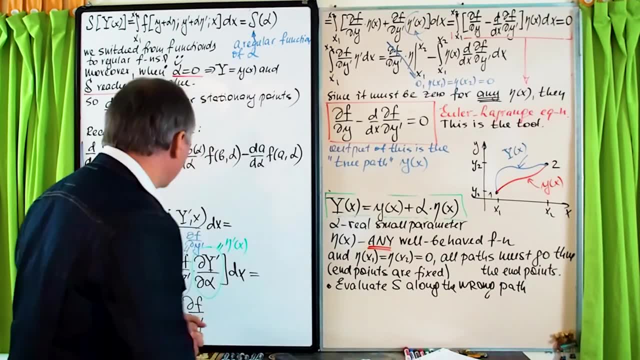 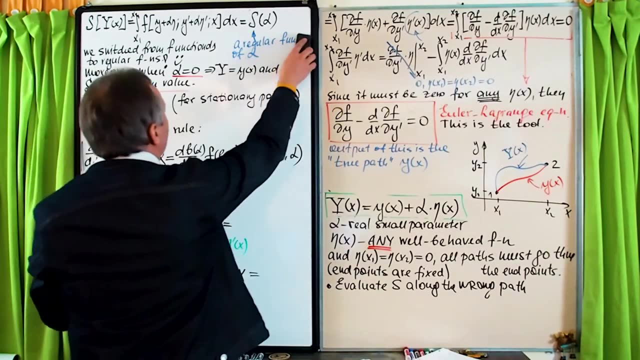 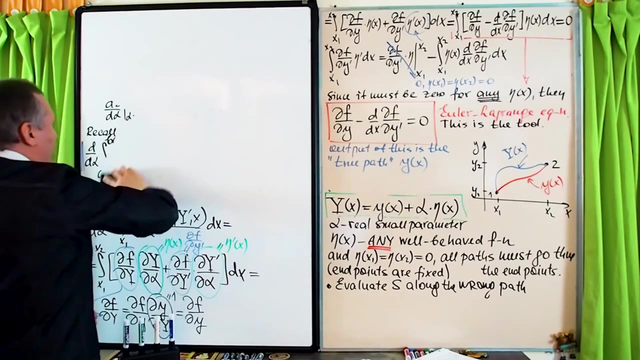 going to look at that. Let's look at that example: Finding the shortest path between two points in a plane, In a plane plane. okay, so now you know we derived so i can erase it and maybe i will be able to finish, although i doubt. so we're going to look at, uh, this example. next class, we will look at brachistochrone example. 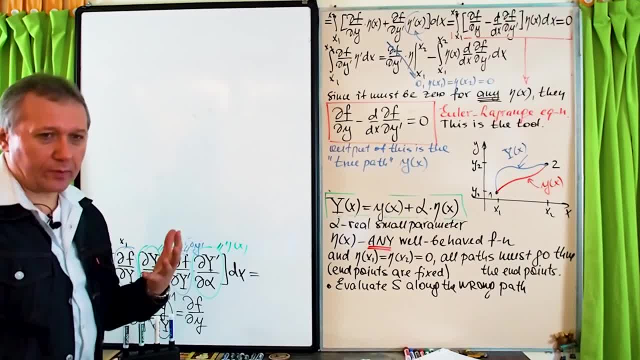 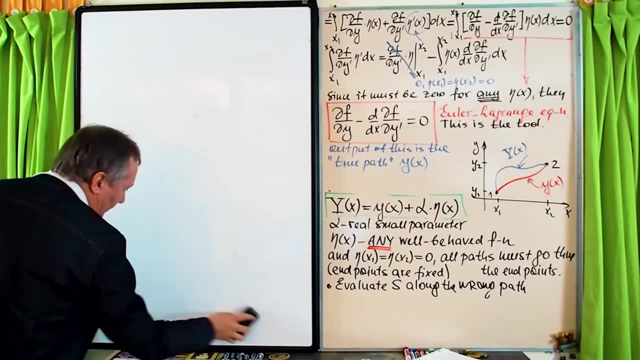 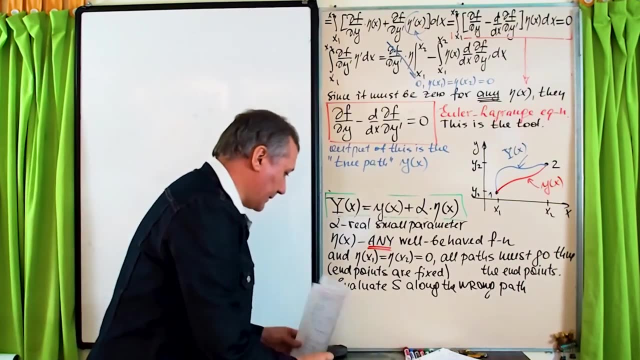 and then i will state another problem, right, but you will finish it in your homework, right, and this will be the end of this chapter. um six, it's reasonably short. it's just a review of calculus, of variations, right, and then lagrangian formalism. so next week, definitely, we will start. 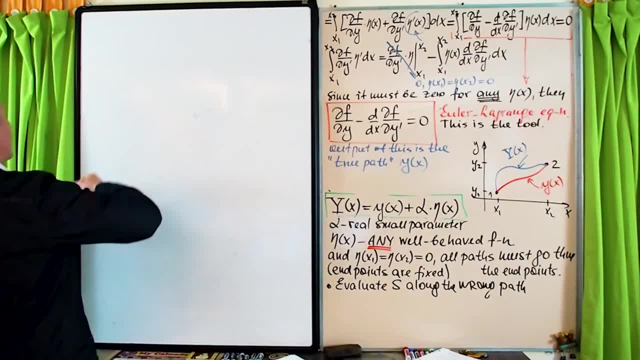 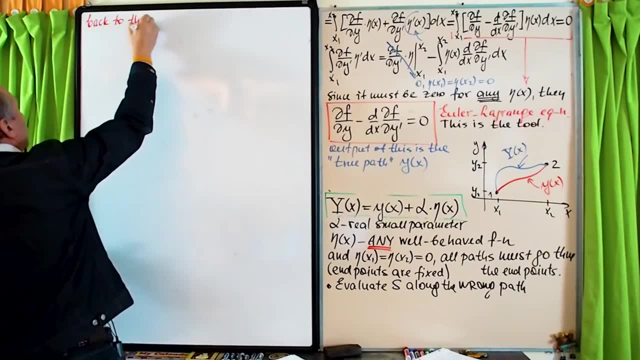 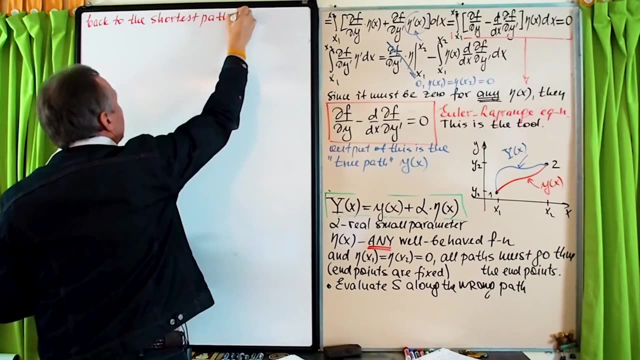 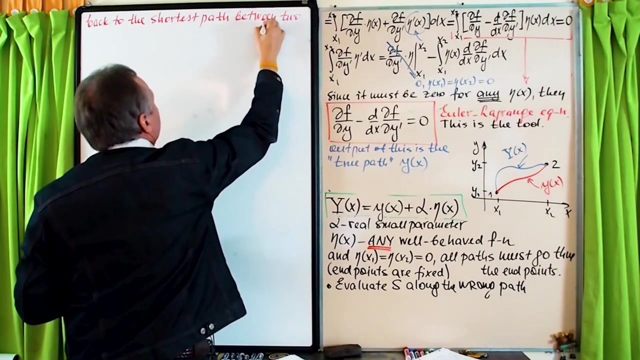 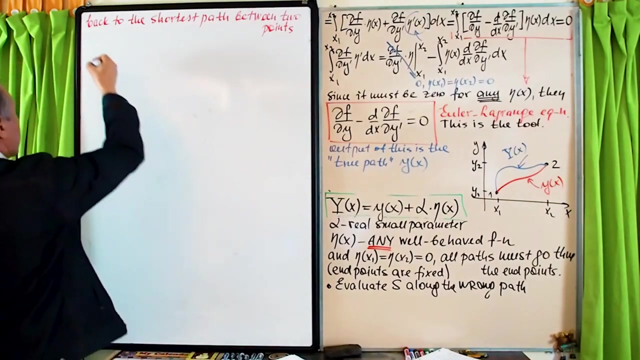 discussing lagrangian formalism. so, uh, back to our example, all right. so let me write back to uh the uh shortest, uh the shortest path between two points, path, path between, uh, two points. so basically, this is an example. probably i should, i should have written: so it's an example, right. 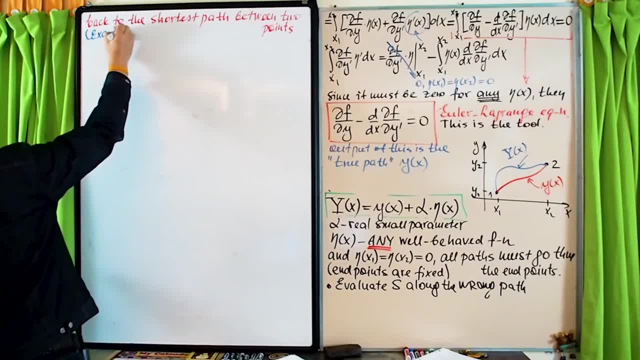 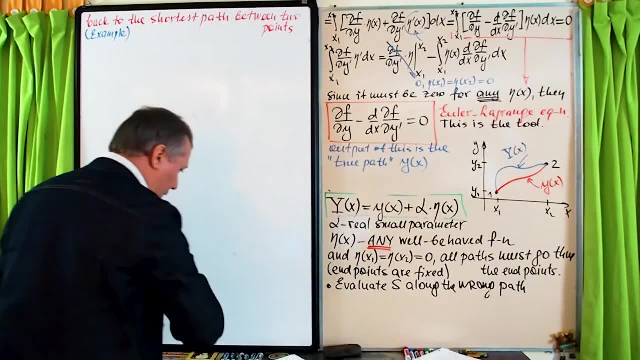 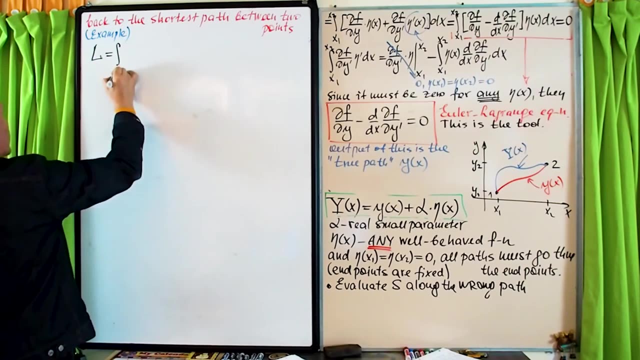 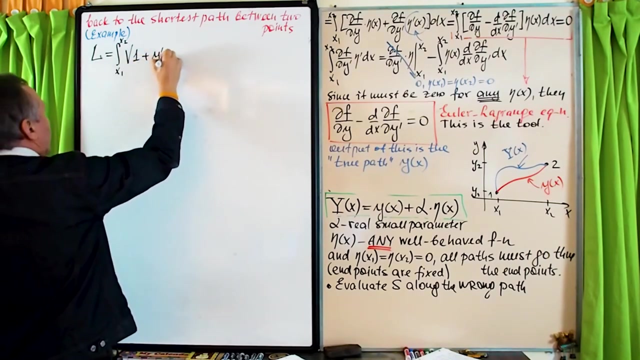 so we already set up the problem right. you have in your notes. i have in my notes, right, the problem that dating जेहं planted right there. uh, is that the śrg of logic? xon Kaštel're, you got to give the first side. okay, this is مت्रोसा web. 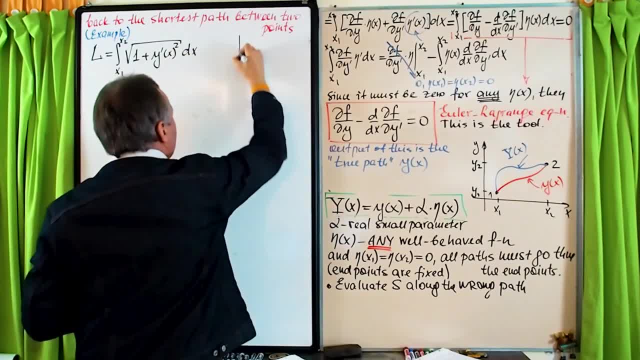 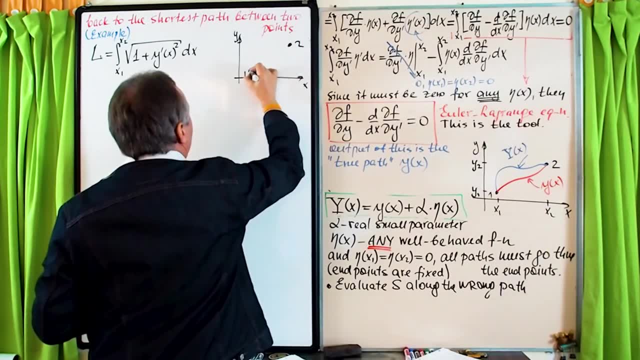 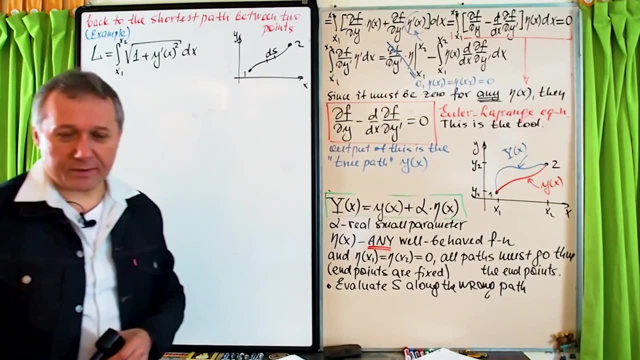 this is student, perhaps all right. and elsewhereوي have anregry all r d s, right. so all r has anregry dx. and again the situation was this: so Y, X, this is 1, this is 2- right, and we picked an arbitrary path. this is ds, which is dx, dy as components, right, so we? 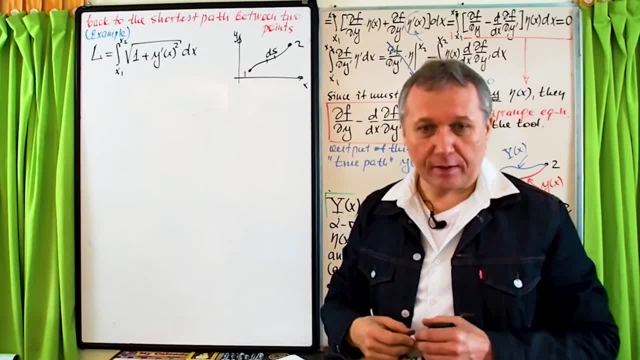 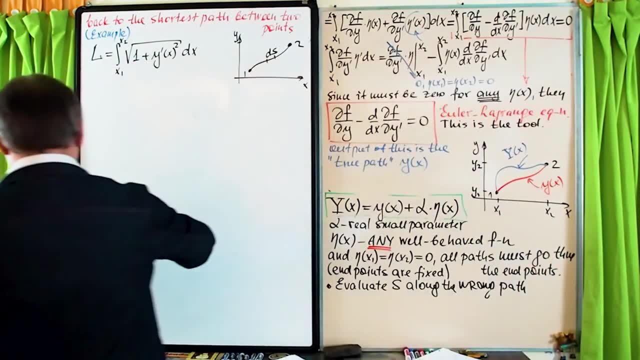 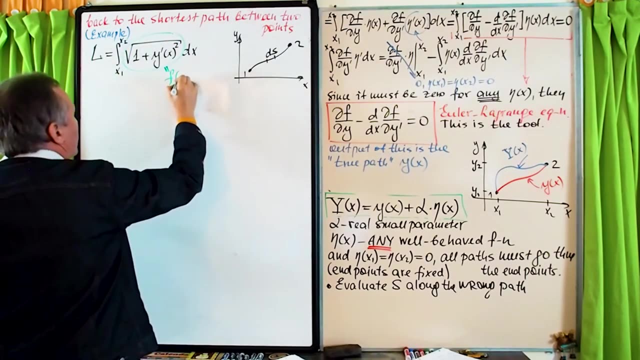 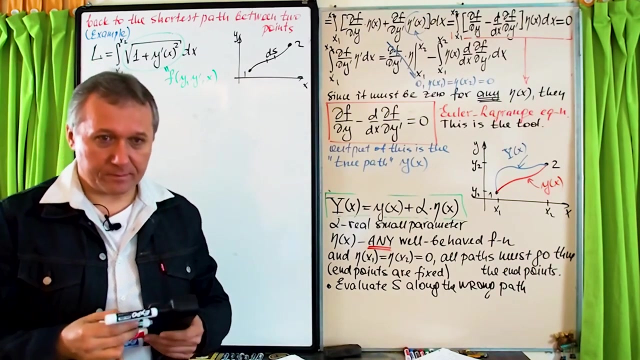 stated the problem. so now we need to find our function F, which is, as I said, just an integrant. so this is our F. so that is our F, which is usually a function of Y, Y, prime at X. so now that is the function. shoved it into the. 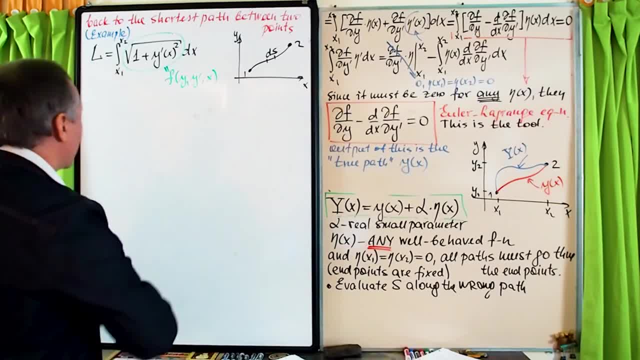 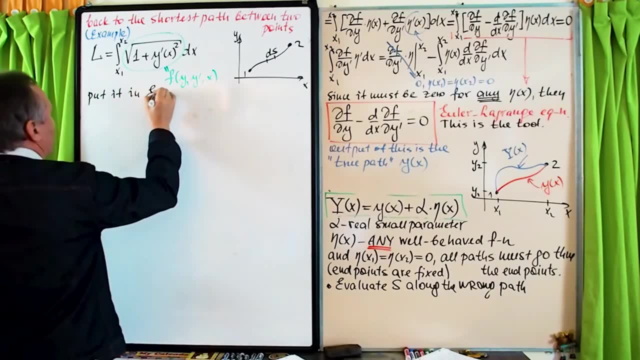 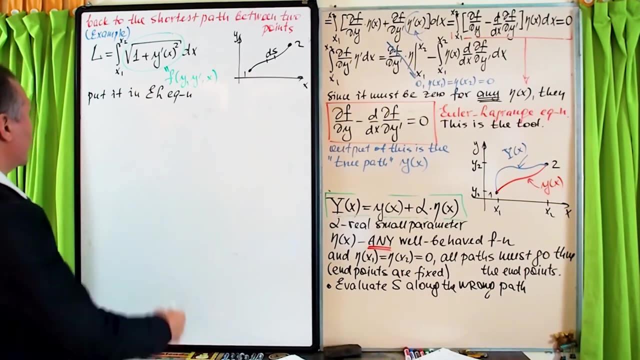 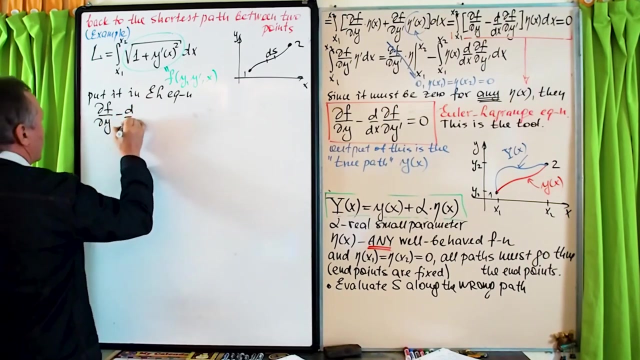 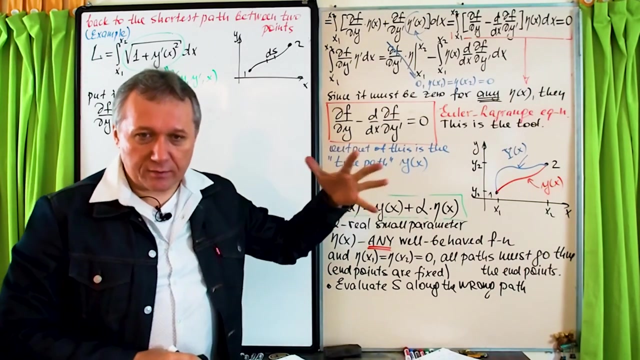 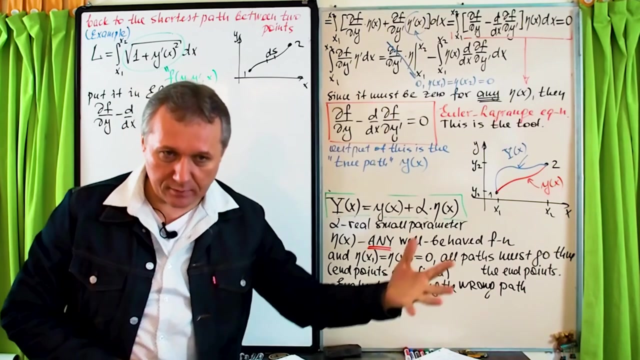 Euler Lagrange equation and massage it right, put it in you, you O'Neill, okay. so now let me rewrite it so it will be DF over D, Y minus D over DX, and, and emphasizing your variable of into your independent variable, is here D over DX, here this Y prime and this white dependent variable, right, independent. 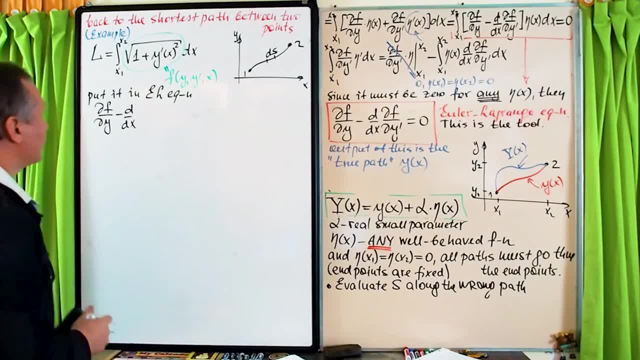 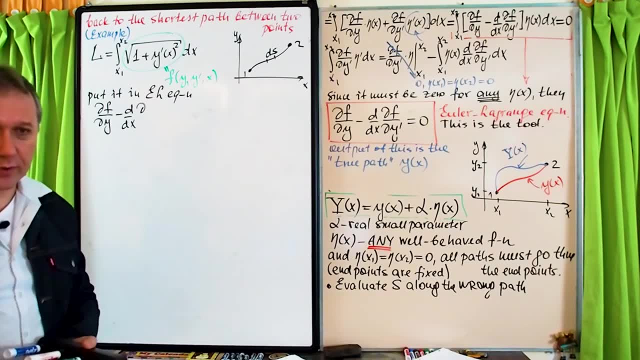 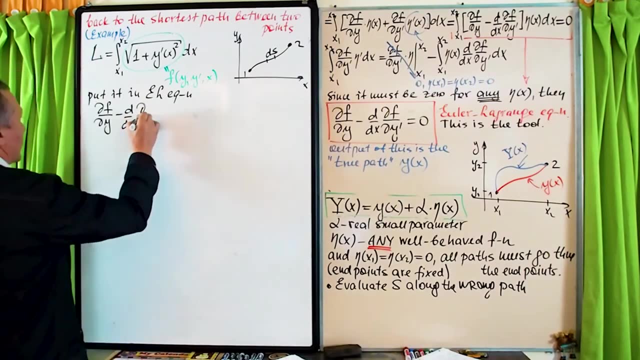 over here in D over DX in the second term, D you will understand next class because this class are most likely. I wouldn't be able to get to that point right, but you all understand why I emphasize on that. this is dependent, that is independent variable. all right. so D F over D Y prime equals to 0. so let me say: 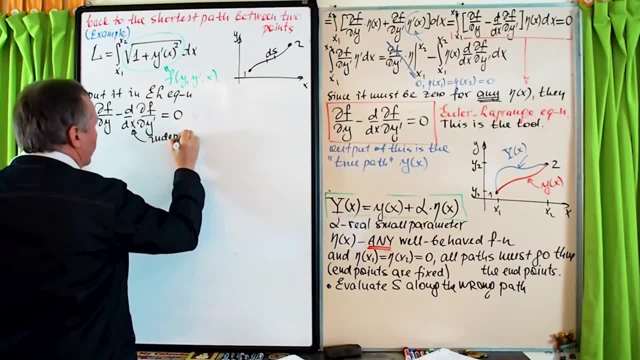 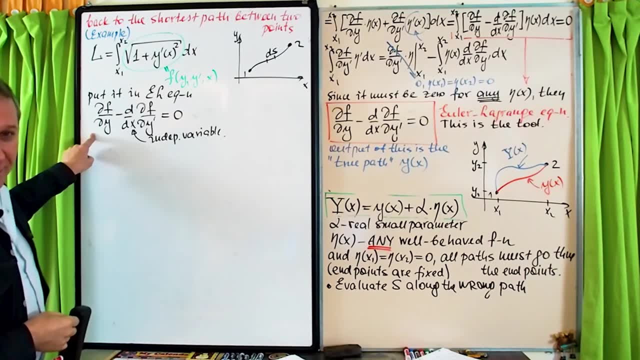 that this is independent, independent variable. okay, first of all, D F over D Y. if the depicted remains 1 as a symbol of щ, okay, first of all, D F over D Y. our function F doesn't depend on Y, it depends on y prime. again, you see, we are looking at the partial derivatives. so 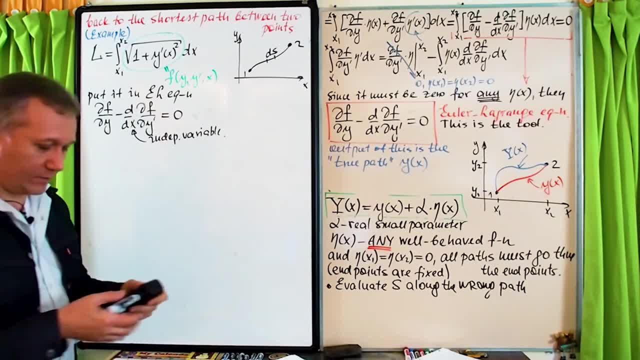 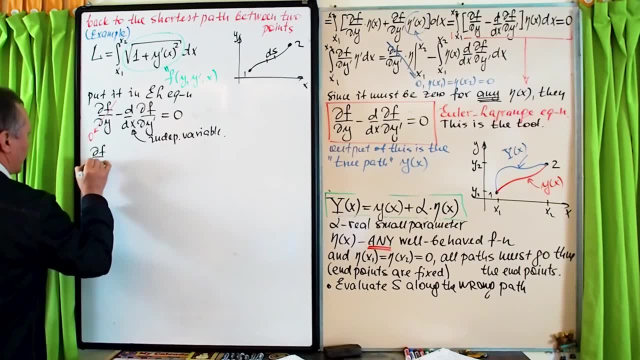 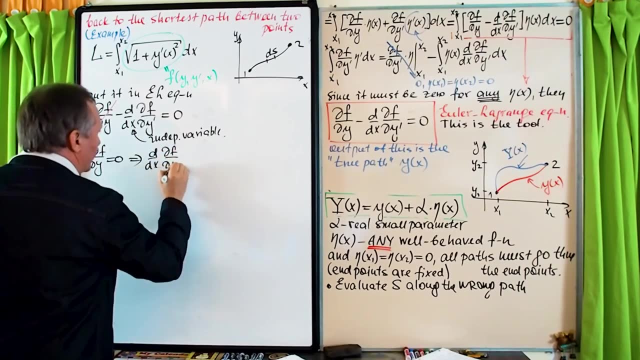 immediately. DF over D Y is 0, and so this is immediately is 0, right. so DF over D Y: iero, and so this is immediately is 0, right. so DF over D y equal 0. as a result, result: D over DX, DF over dy. prime equals zero. warning, especially at the very. 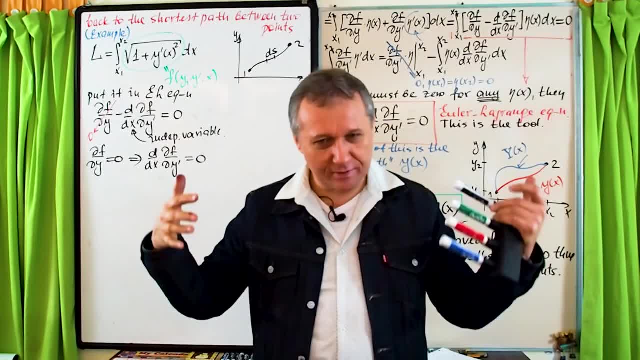 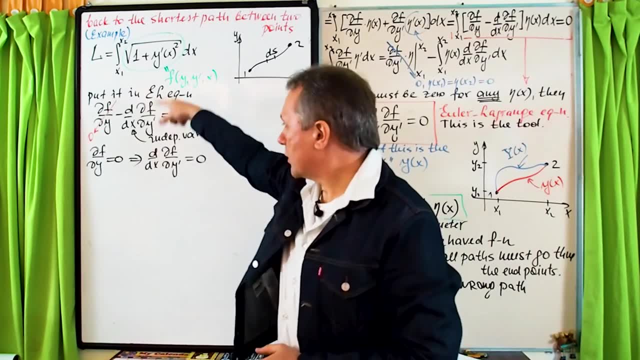 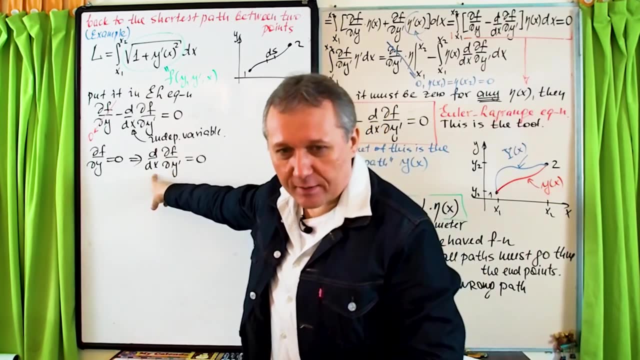 beginning. plenty of students did this in homework. this silly mistakes mistake. they differentiated this function. of course, here you can. you can differentiate DF over dy prime. you will get the function and then they differentiate it with respect to X. as a result, here they got it, they got the. 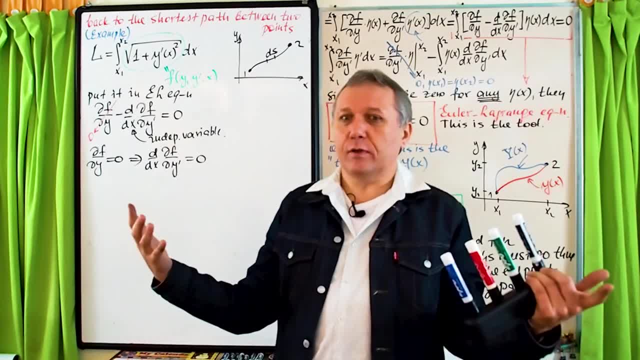 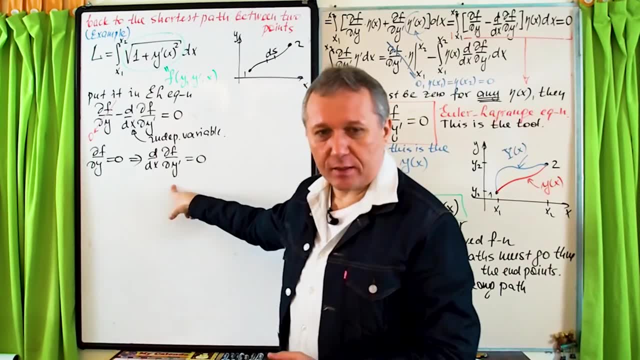 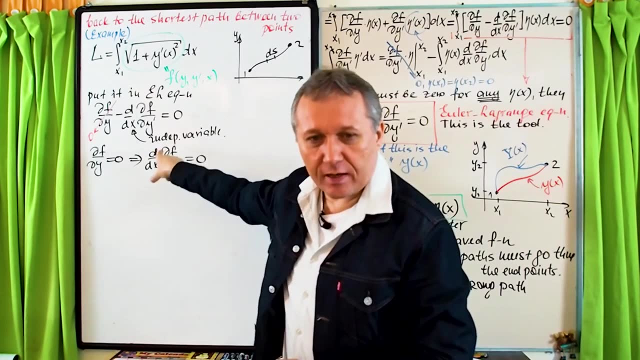 second order differential equation. it's not wrong, but then they will. they would stare at that second order differential equation without knowing what to do. you don't have to differentiate this because you can see immediately. since the derivative equals to zero, this function is constant. DF over dy prime is: 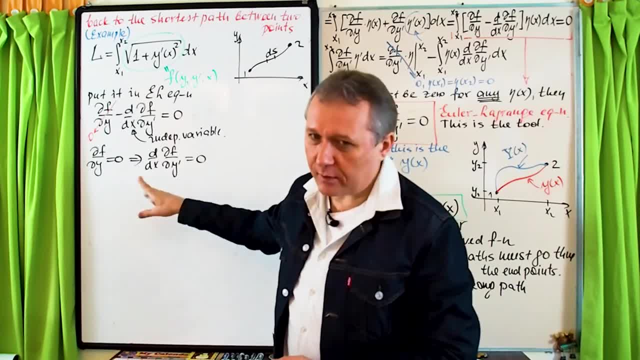 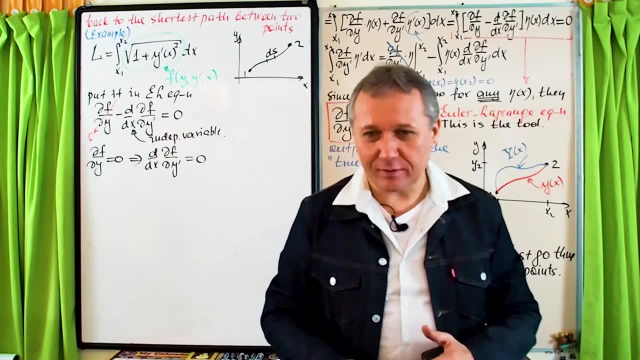 constant. it happens almost still, occasionally, with some students right and then they sent me a mail. what to do? what? this difference between the derivative and the derivative is not wrong. it's not the average expression. oh, you are right. but, with respect, this is true. so let's. 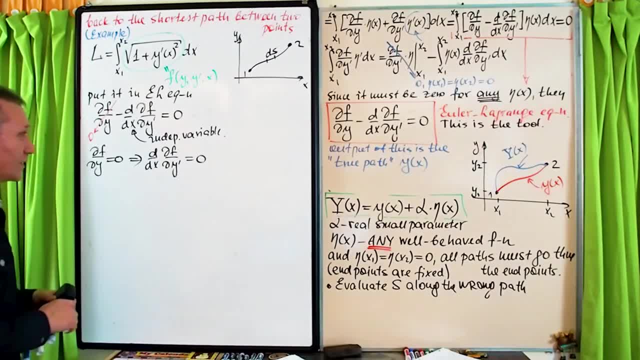 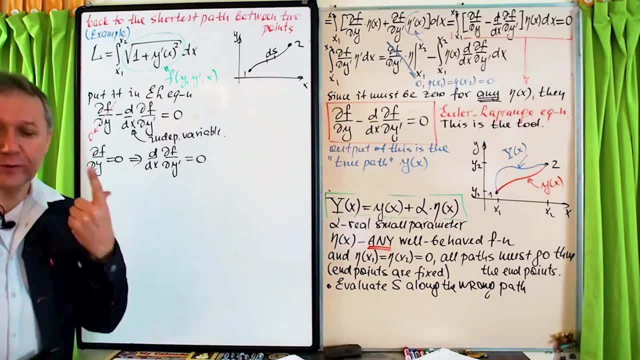 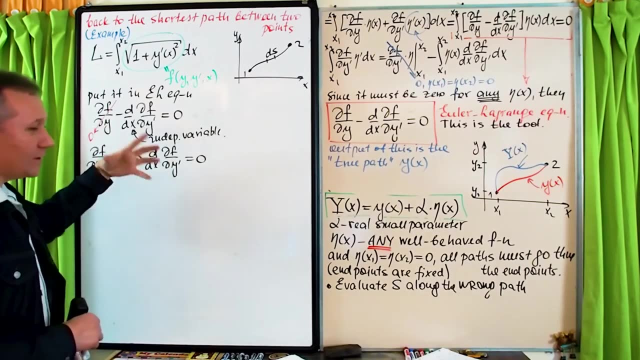 differentiate this again. this differential equation looks crazy. yeah, because you've done an unnecessary thing, right, which is not needed, right? so in this case, immediately, the nature gives you integrated for you, did the first integration for you, right? so don't go into that math. so, since this is zero, the 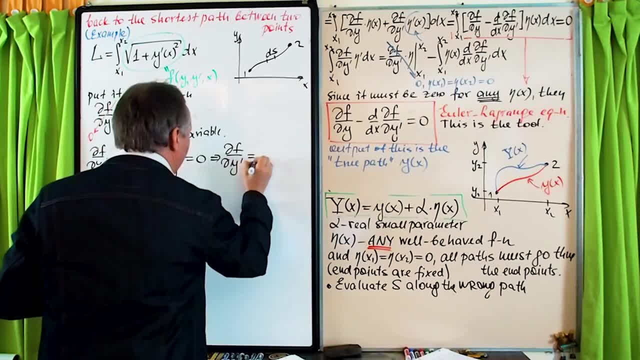 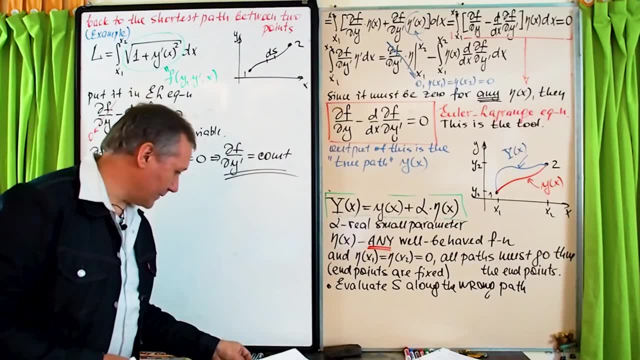 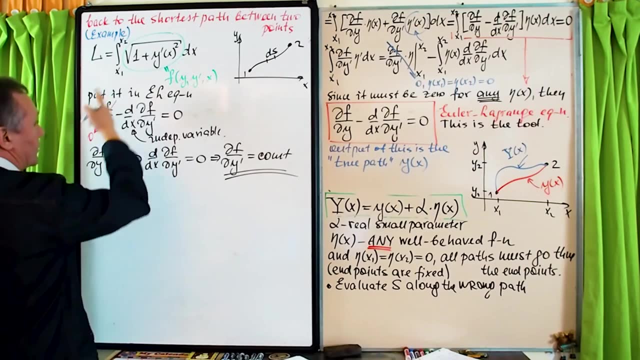 first, integration in your automatic right, so you'll get DF over dy prime and equals constant. don't differentiate this with respect to x right. okay, so now, as a result, df over dy prime, df over dy prime. so let's differentiate it, so it will be one over two. 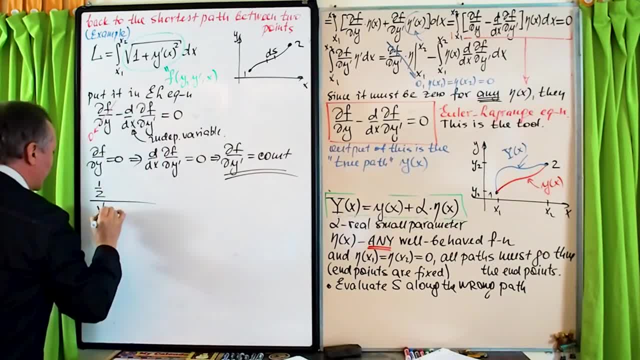 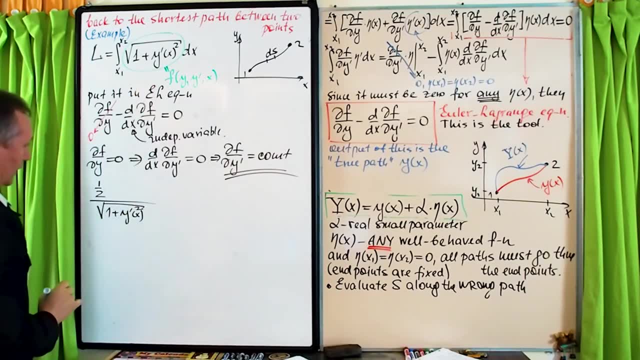 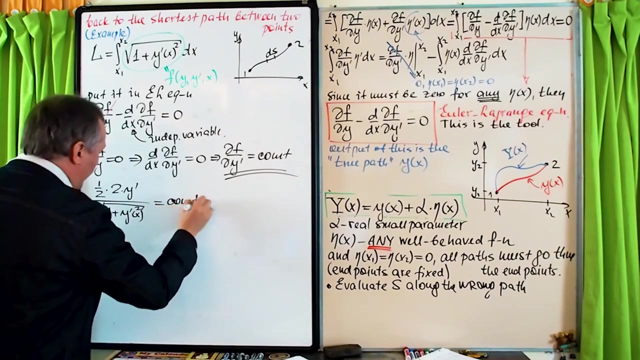 then this will go downstairs: one plus y prime of x, squared. all right. then we have to differentiate this again with respect to y prime partial derivative. so it will be times two y prime and it is equal to this constant right. so two goes and we have this. so let's of course square it. 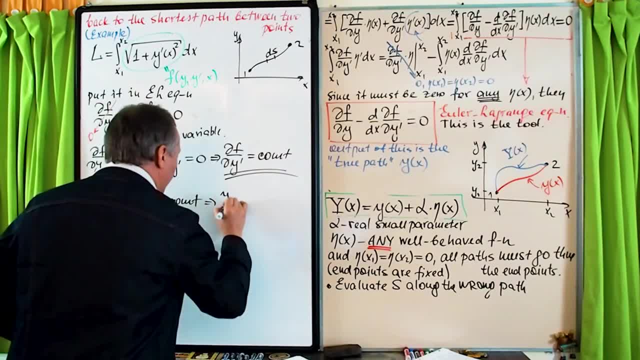 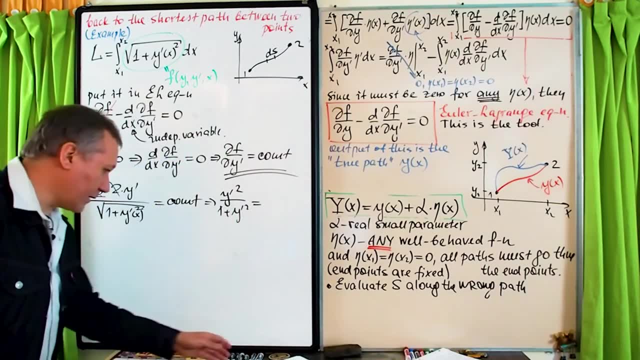 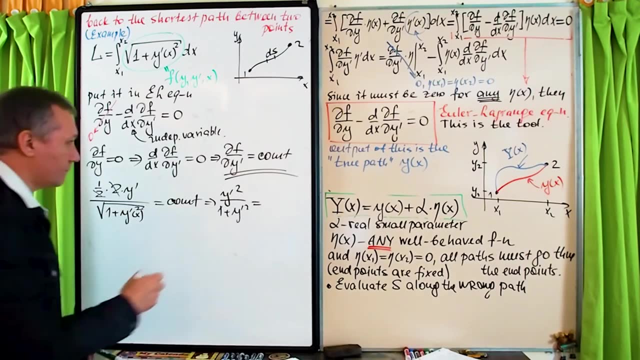 just a little bit left. let me just quickly do it. so of course you will get y prime squared divided by one plus y prime squared equals two, and now i think i will introduce the constant okay c. so i call this constant labeled. i call this constant c. 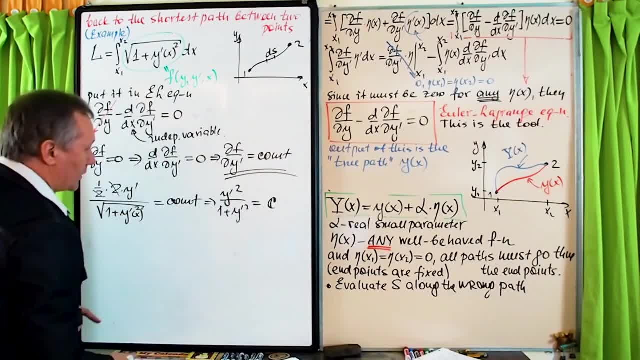 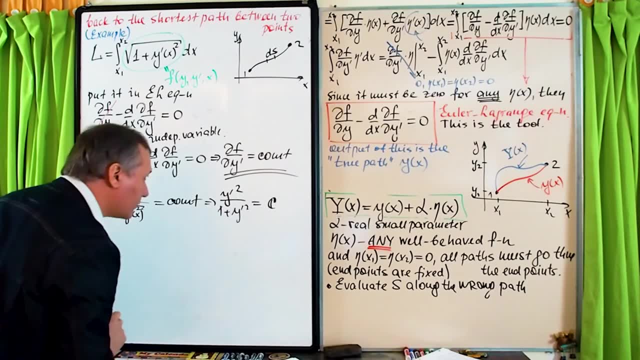 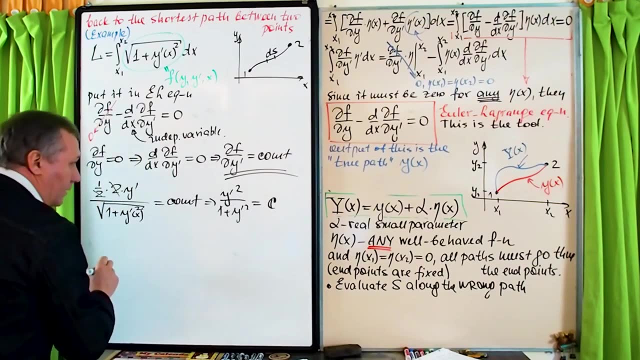 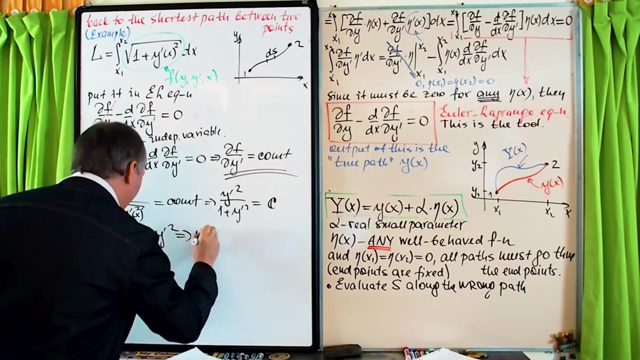 okay, so of course you can move terms around. so you will get uh, one minus c, one, really, one minus. how come? oh yeah, yeah, it's good, right. y prime squared equals c plus c y prime squared, so we can move terms around. all right, so it will be y prime squared. one minus c equals to c, right.